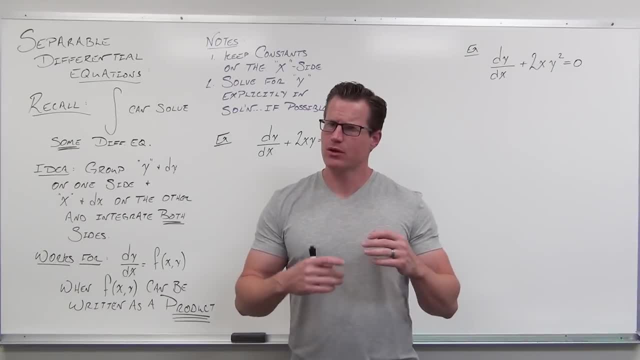 them at least an approximation. We've learned a lot of things about differential equations, but we haven't learned really how to solve them. The only thing we really know is that if we have some very basic differential equations, an integral can undo a derivative, and so an integral can solve. 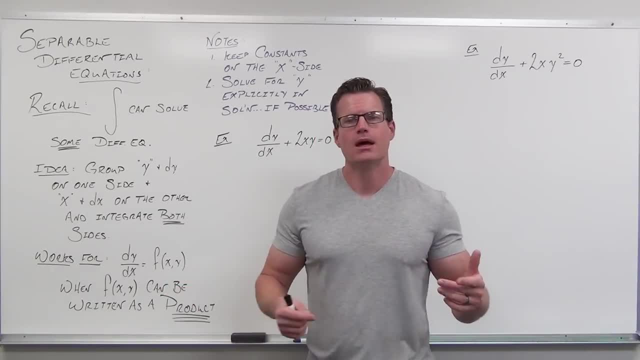 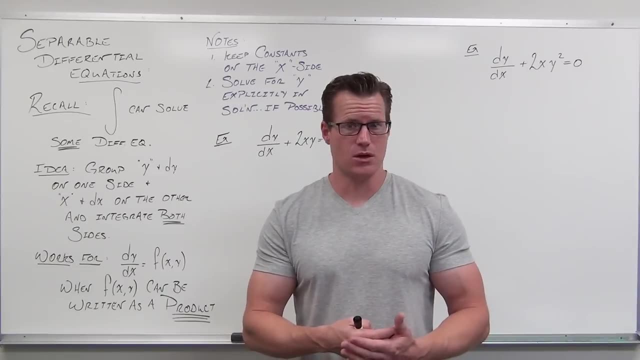 some very basic differential equations for us. No problem, Now we're going to learn about this technique, that is. it's the most fundamental. It's the one that you try to use as often as possible because it's the most straightforward. So there's lots of techniques on how to solve differential 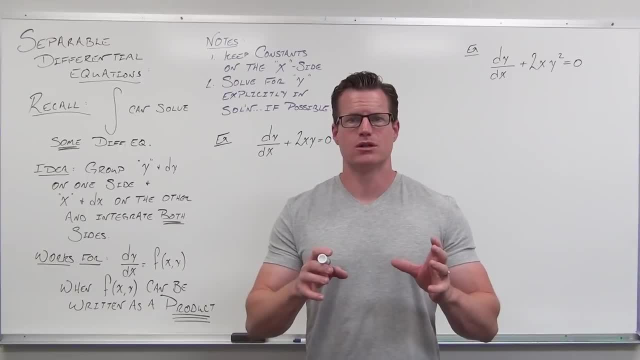 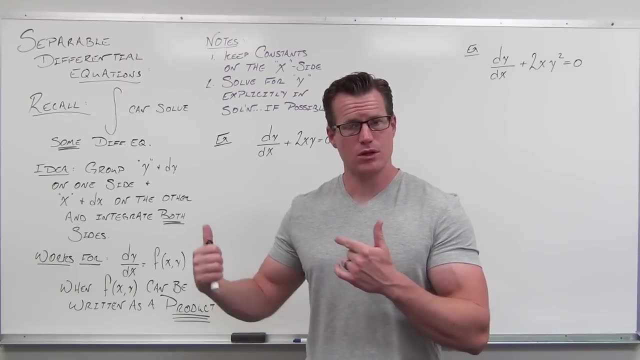 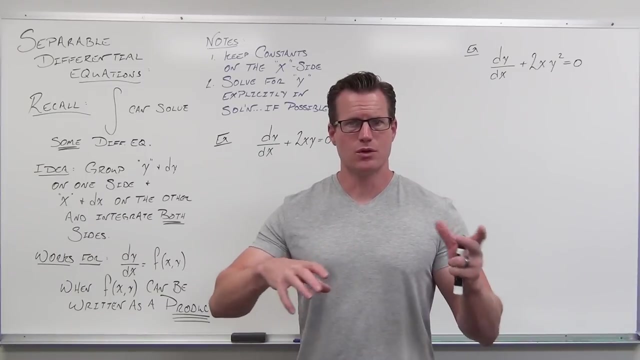 equations for ordinary differential equations, first-order differential equations like we're dealing with. So there's some very basic differential equations. We're going to learn about things like separable differential equations that we're going to talk about today. There's homogeneous differential equations. There are Bernoulli- if you can make a Bernoulli substitution. 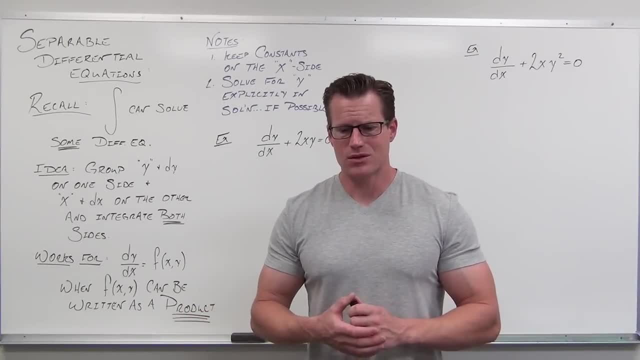 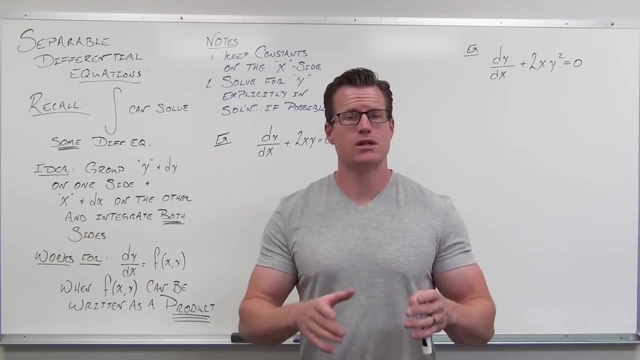 There's a substitution technique for differential equations. There's some other ones as well that we'll explore. So my point is that we're going to get in in the next several videos on lots of different techniques and at the very end I'm going to wrap up and say, hey, here's how you. 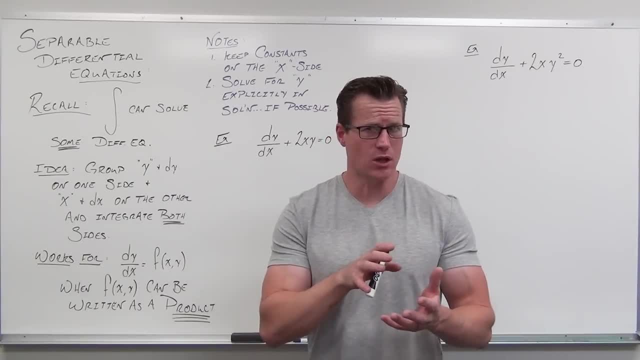 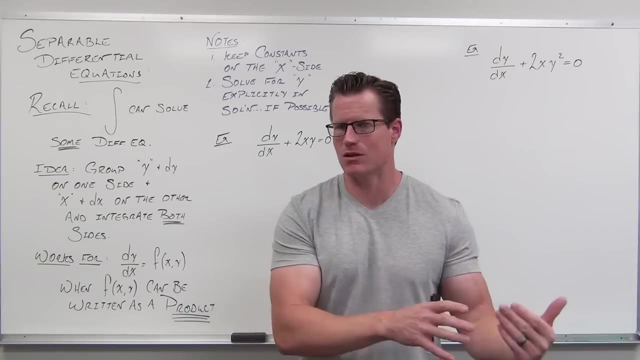 should approach these differential equations. Here's what you should be looking for, Maybe, maybe, try this first technique and then, after that, see if you can make it to this, and then see if you can make it to this, and I'll give you a list of a thought process on how we would go. 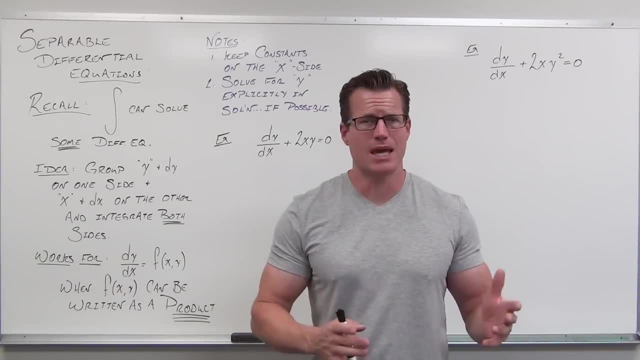 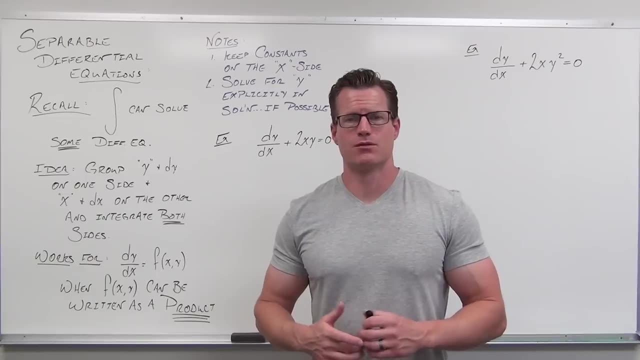 about it. The first one that we should try, like all the time, if we can- and it's it's pretty easy to see when we can use it and when we can't- is if we have a form of a differential equation that is separable, where we can separate the variables and the first about five minutes of this video. 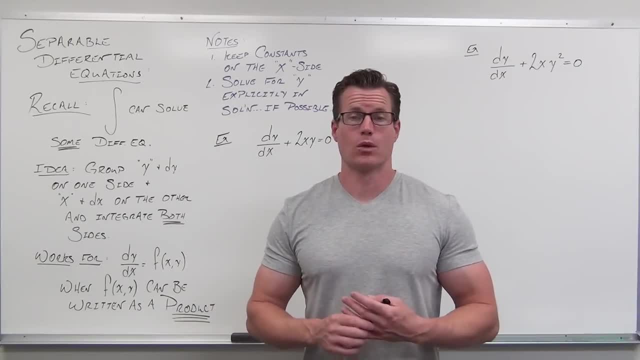 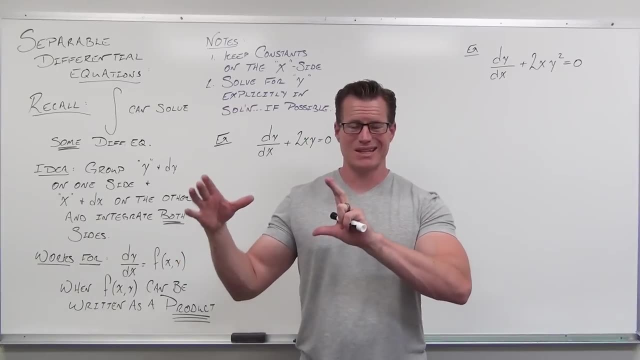 I'm going to explain exactly what we're doing, why it works and what we're going to do next. So we need to remember that integrals can solve differential equations, because a differential equation is basically this equation with a derivative in it and, if I can get it into, 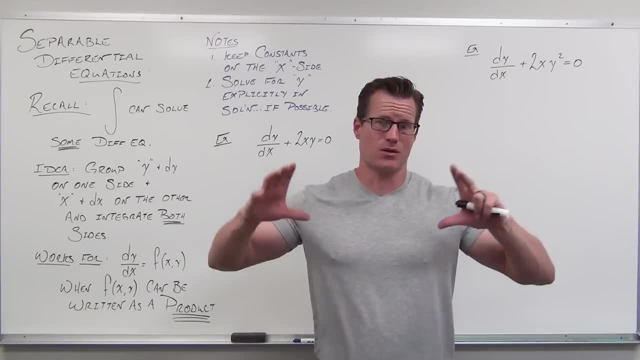 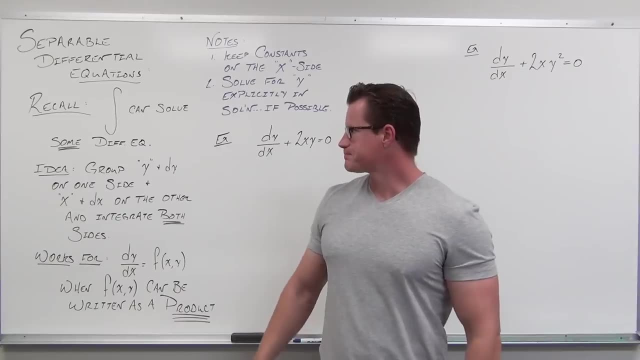 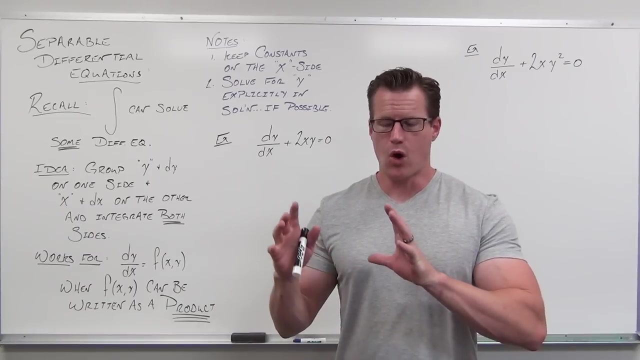 proper form. I can just integrate both sides and find my parent function or the, the anti derivative. so that's what integrals do. is they find that? so we can do that. so here's our idea: if we can, if we can write our differential equation where we can group all of our- let's call it y stuff all. 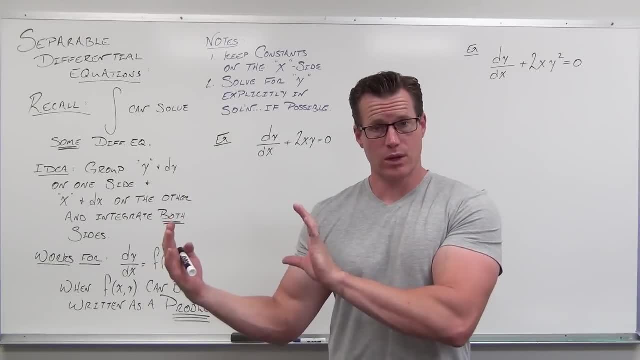 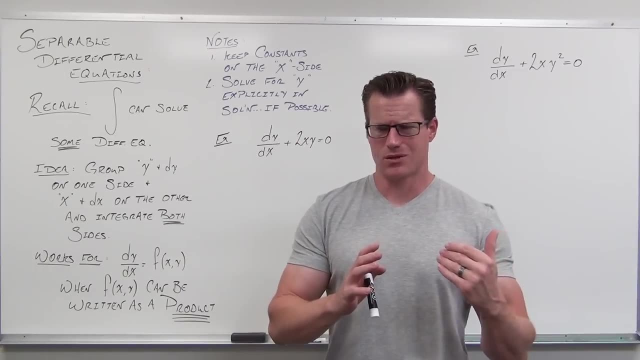 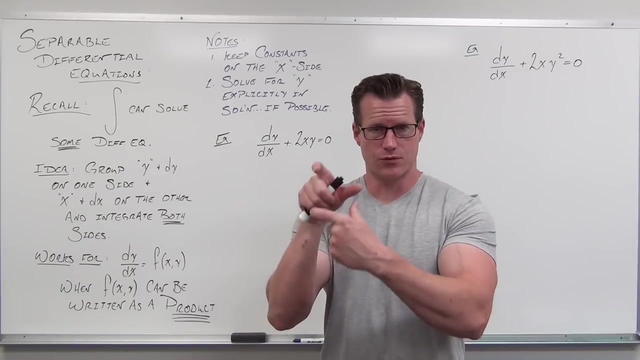 of our functions with y in it and the dy on one side, and all of our junk with constants and x's and the dx on the other side. so wait, wait a minute. I thought we had dy, dx. we do, but those differentials, we can put this in what's called differential form. and well, similar differential form, we can. 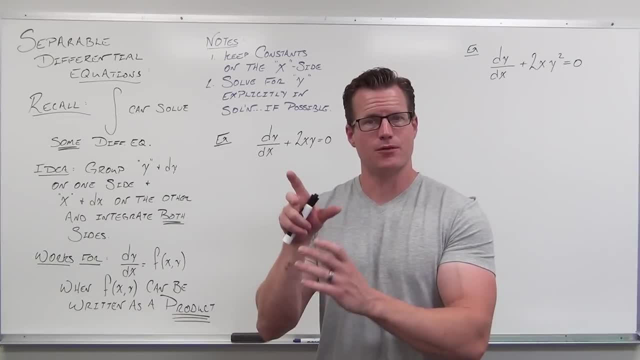 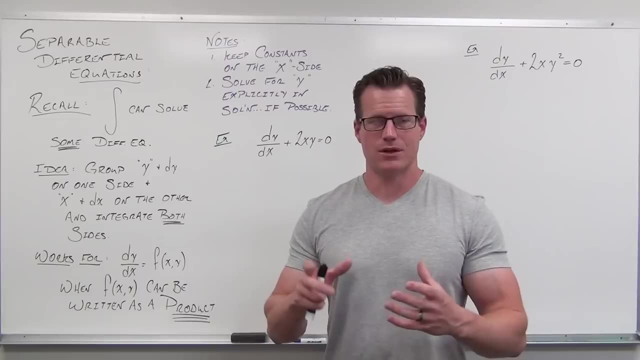 split up that dy and dx. we can treat it like the fraction that it is. it comes from that. if you remember, like back in way a long time ago in calc one, I have a video on actually where we talk about how you can really sort of separate that dy, dx. 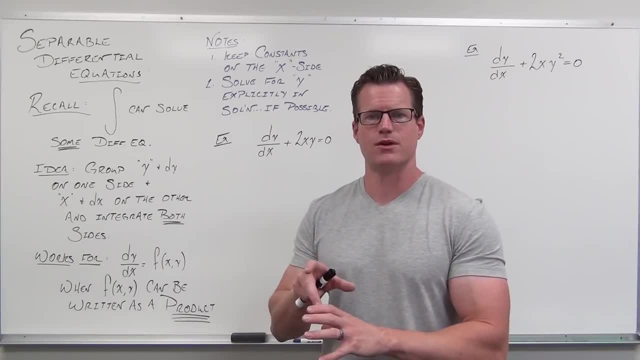 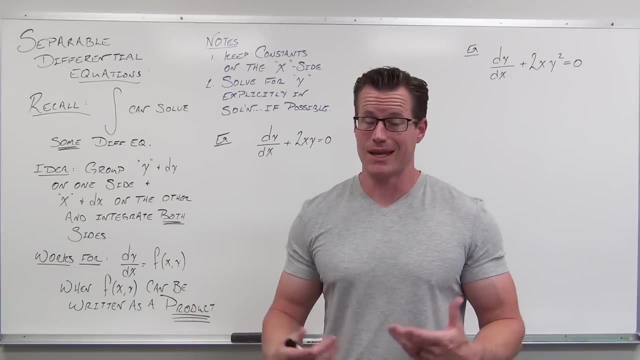 because of how it's created. when we first create the derivative, we we put a dy and a dx together and we can actually pull it apart and it works for us mathematically and that's pretty awesome. I will show you another way to think about it if you really need to. that's okay too, so I'll. 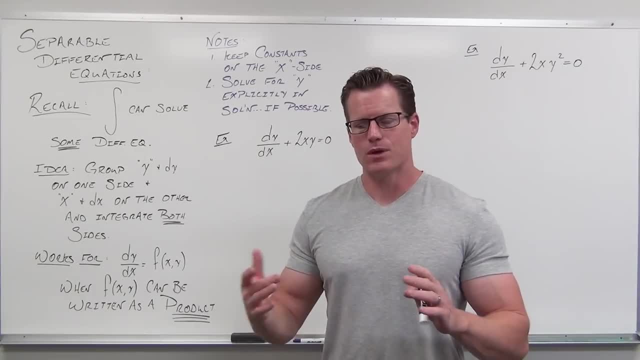 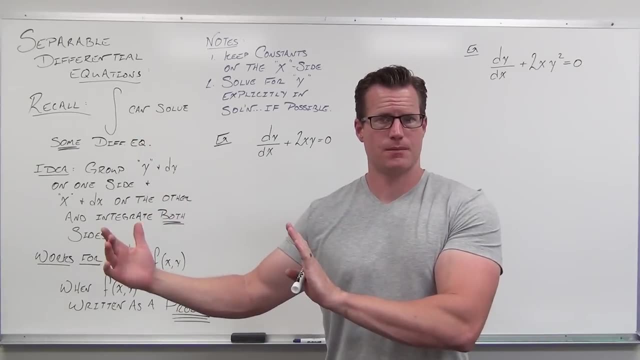 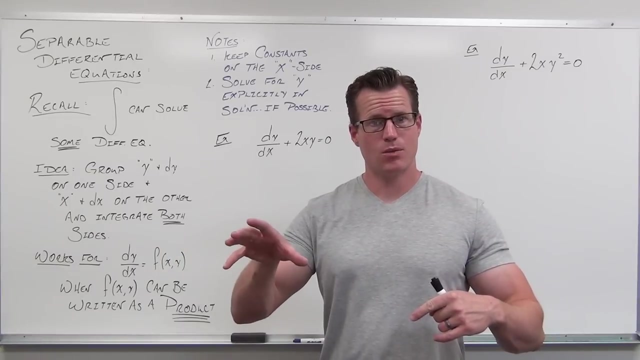 show you two ways to approach this. but the plan is, if we know integrals under derivatives, let's try to put all of our y stuff and dy on one side, x stuff and dx on the other side, and then when we integrate, we'll integrate one side. hey, we got a dy. oh my gosh, that matches up an integral. 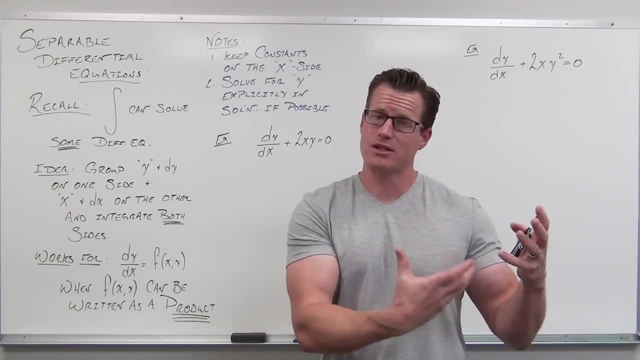 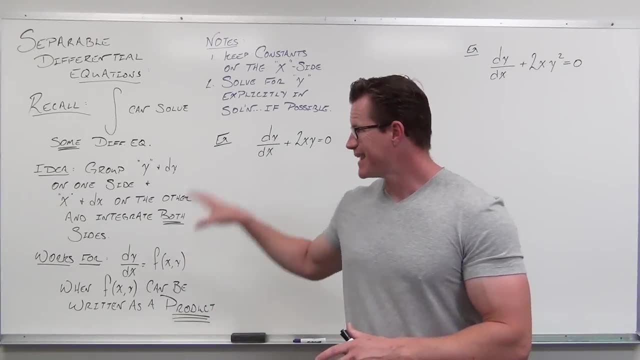 with all the y stuff. and then we have another integral with dx oh, and that matches up with all the x stuff and we can just take two integrals. and then, if possible, we can solve for y explicitly, and that's what we're talking about here: group your y stuff and dy on one side, group your 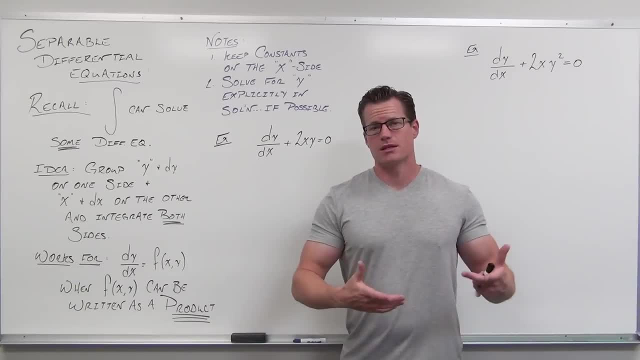 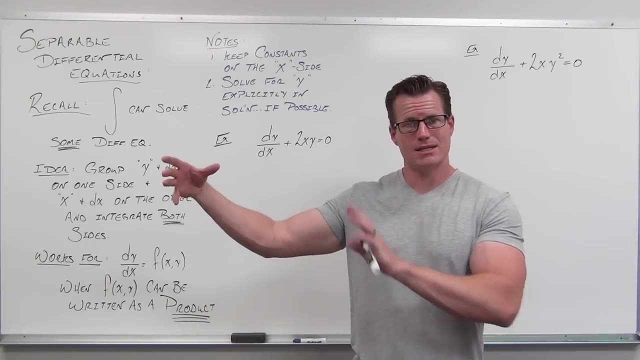 x stuff and dx on the other side and then integrate both sides. what we do to one side in an equation we've got to do to the other, so that's why we're integrating both sides. the reason why we have Y's and dy on one side is so that when you integrate dy your variables match up. we have 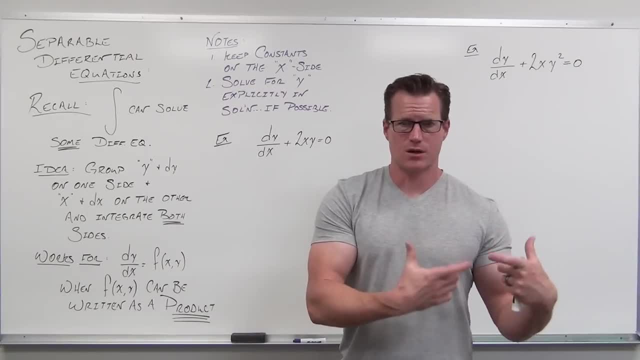 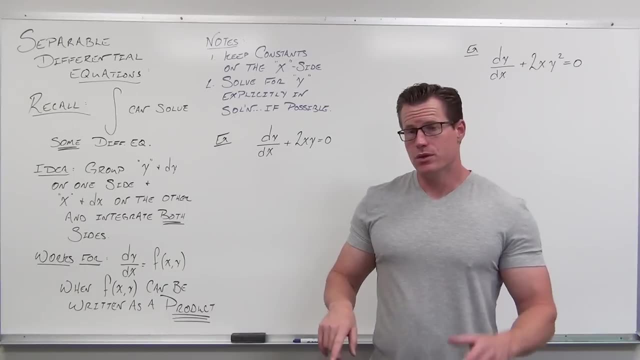 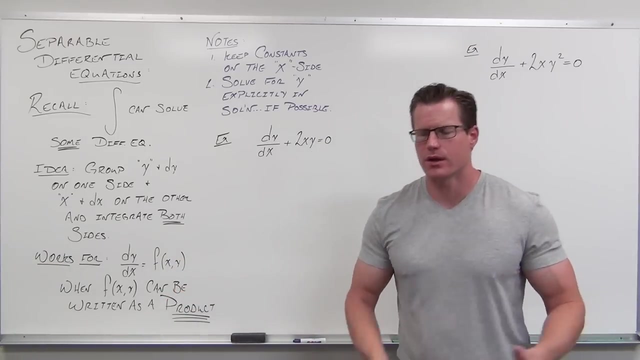 X's and DX. that way, when you integrate the other side, your variables match up. that's the plan. this works for any sort of differential equation where you can solve for the dy, dx, and then this thing is a product. what why a? why a product? well, if we want to separate our variables and 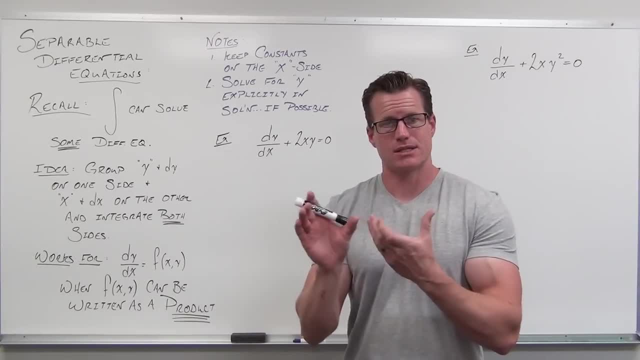 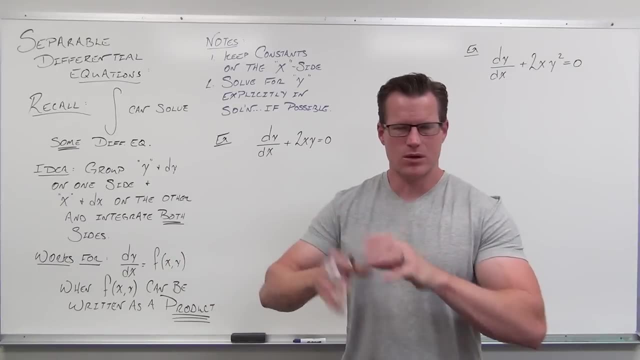 have the ability to do an integral. we need the X's and Y's to somehow be multiplied together. that way we can easily divide or multiply or move our, our X parts and our Y parts, our factors, to one side or the other and separate. if we have stuff added and subtracted, we either have to 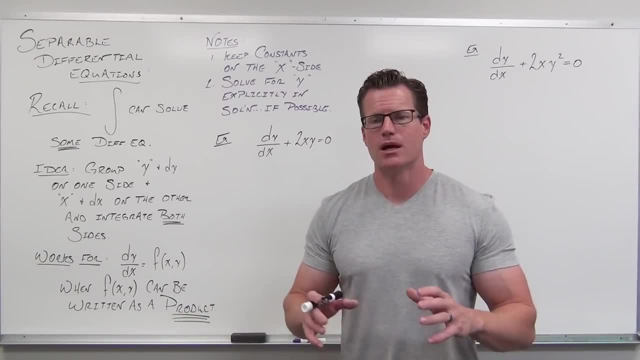 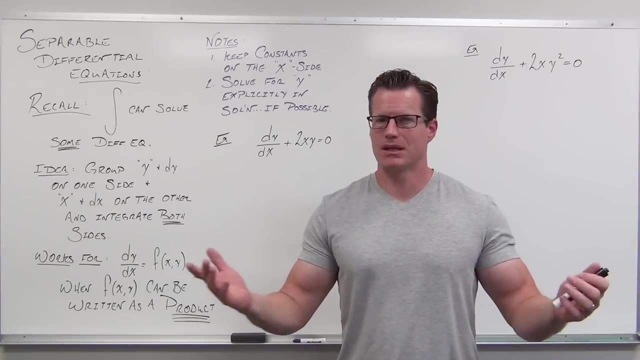 be able to factor that which we're going to get in our second. the last problem which we have to solve is is the original equation. so we need to solve that to create this product, or we have to have some other technique, like linear. there's linear differential equations. that's another. 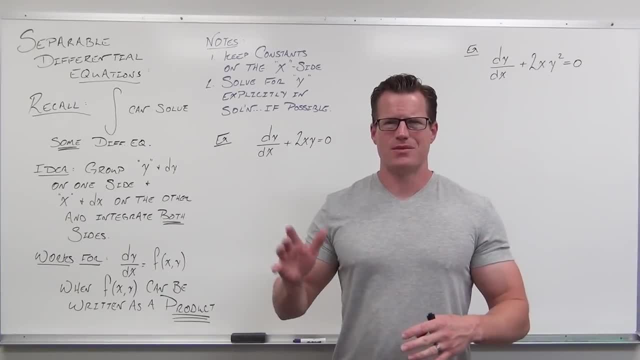 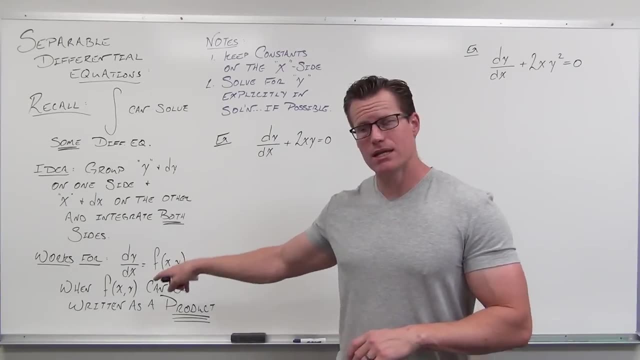 technique we're going to use figure out how to solve linear differential equations. so a little bit of a recap. I said about five minutes, I don't know if I've made it that long, but the idea is we've got differential equations. if you can write it as dy, DX, your derivative equal to a function in: 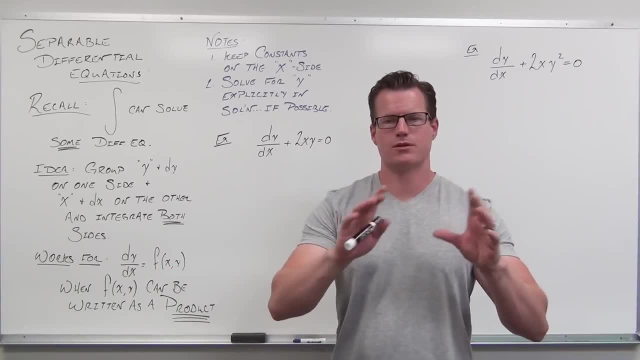 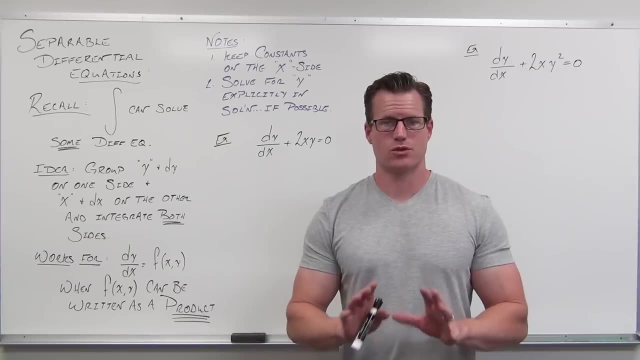 X and Y, where your stuff is multiplied, can separate our variables. We put our y's on one side with dy, our x's on the other side with dx. We integrate and we try to solve for y. So a couple notes, One thing that's going to really 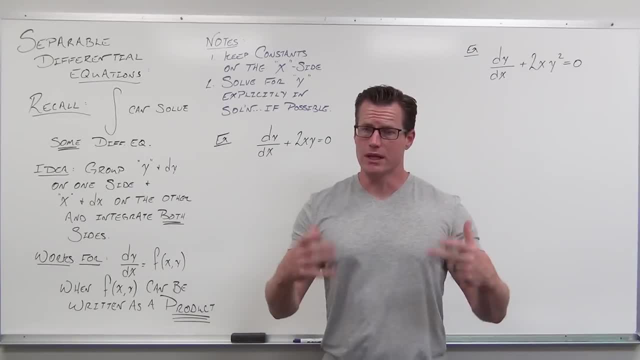 help you, keep all of your- I'm going to call them constants. they're really coefficients because we're multiplying. So keep your coefficients, your constants, all of that stuff, the numbers. keep it on your x side, The y side. it gets a lot more difficult to solve if you've moved your. 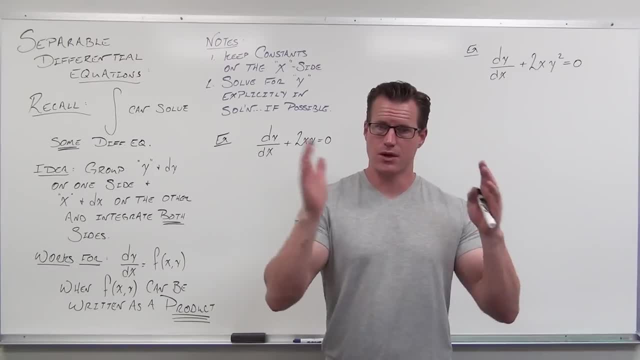 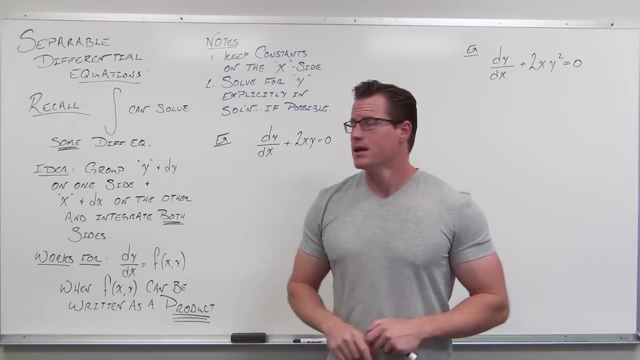 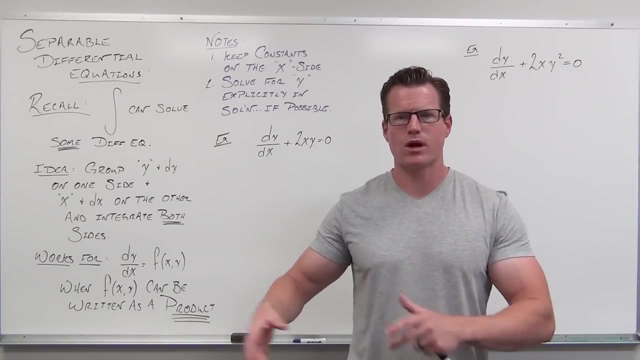 constants coefficients to your y side. So keep your constants on your x side. We're trying to solve for y, So that would save us some work if we keep our constants on our x side. Secondly, if you can, when you do your integrals you're going to have a y function somewhere and you're 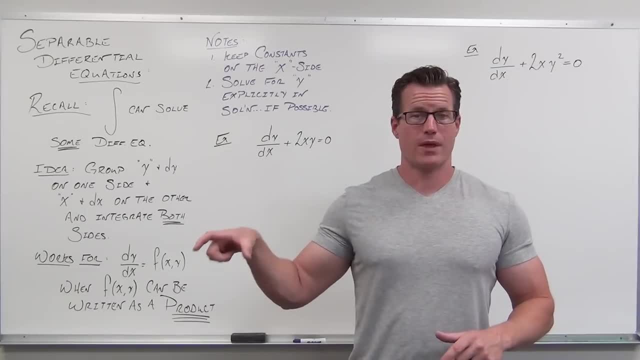 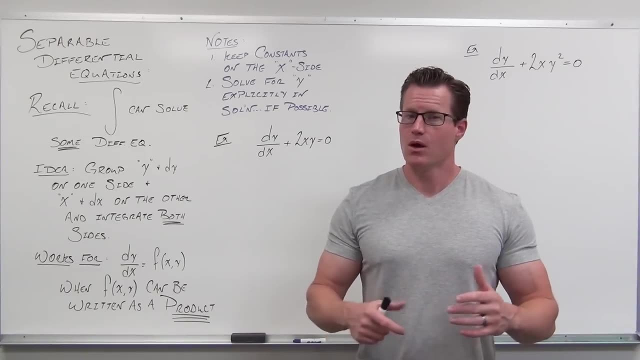 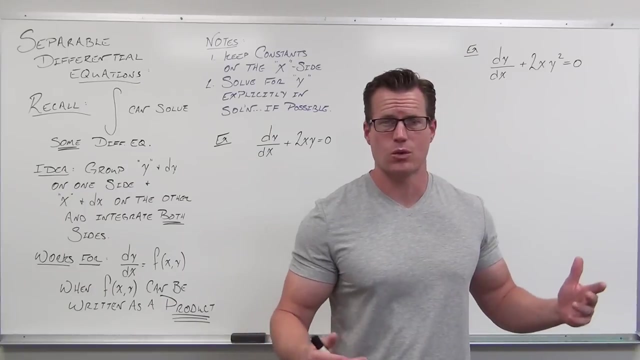 going to have an x function somewhere. Try to solve for that y explicitly. Sometimes it's not possible. A lot of times it is with separable equations. So we're going to- I'm going to show you that We are going to do just an absolute gob of examples here. I think like 12 examples. 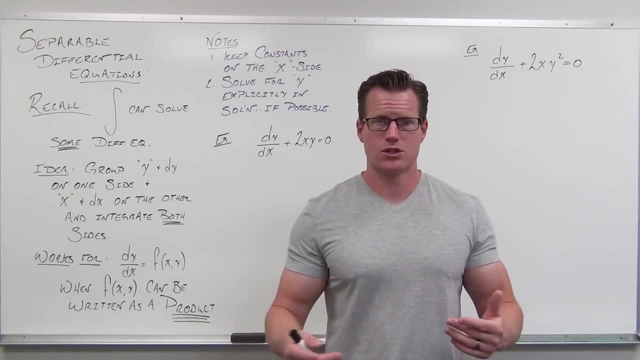 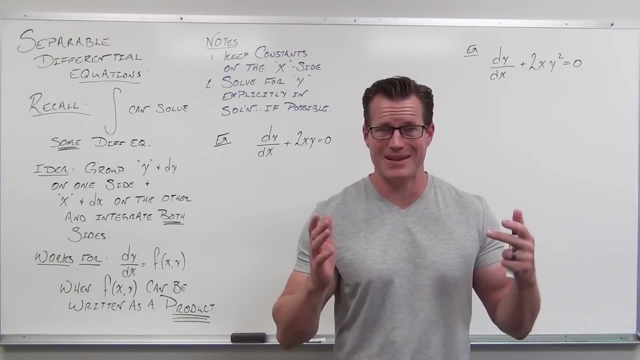 11, 12 examples. If you are getting the point after the first two and you want to just go and try stuff, that's fine. What I'm trying to do here is for those of you who- man, it's been a while. 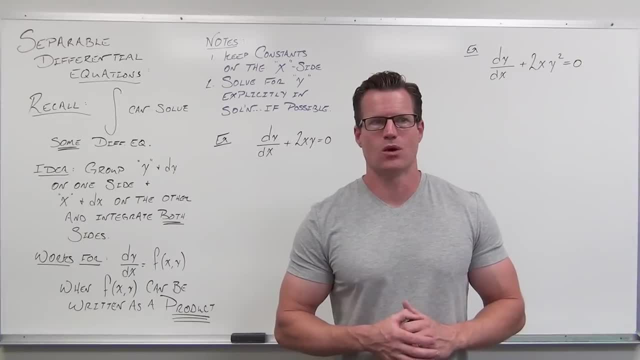 since you take calc two or even calc three and you're like: I don't remember how to do partial fractions. What do those look like? I don't remember how to use integration table or trig, sub or substitutions, even, or integration table. I don't remember how to do partial fractions. 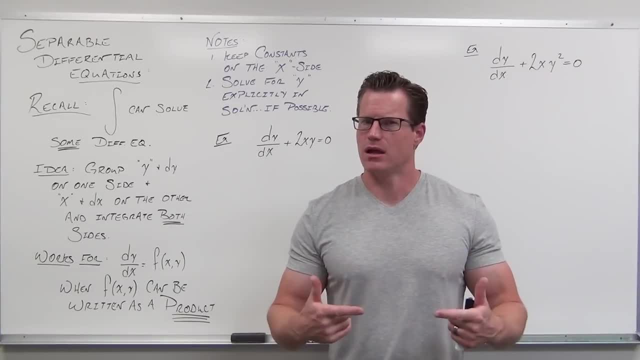 I don't think we have one of those, But if you're not, if you're not familiar with that stuff, that's okay. That's what this is for. Okay, I'm going to do like 11 examples to make sure that. 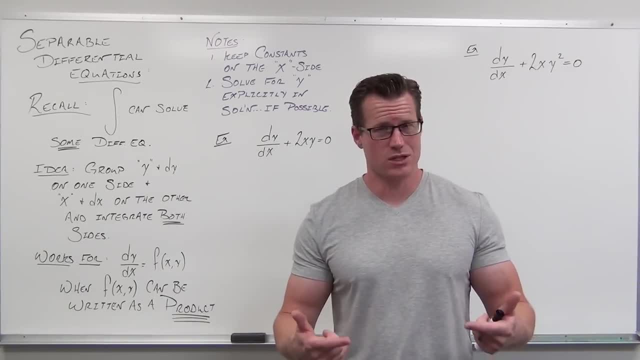 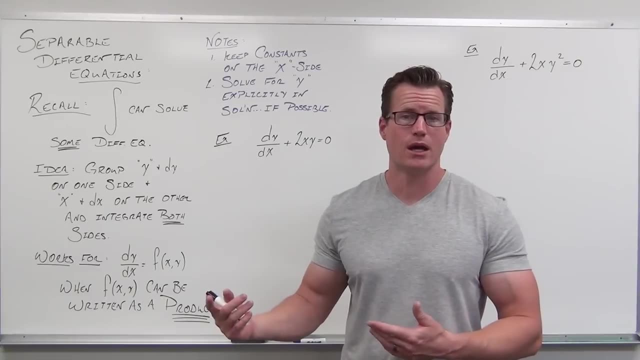 our integrals, our integration techniques are still there. If you're fine with that man, skip through a few of them, That's okay. I mean I don't care if you watch the whole video or not, I want you to learn it. So the basis of separable differential equations, our very first technique. 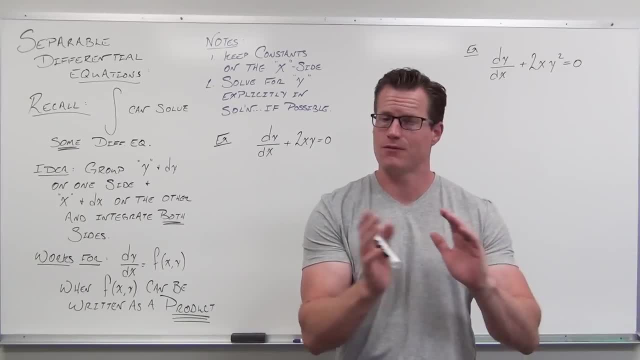 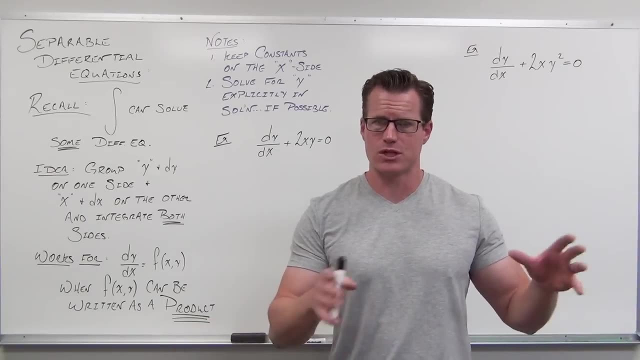 is, if you have a product can write it as a product factor it So that's a product. Get your Y stuff on one side with DY X stuff in the other and integrate. That's it. I'm going to show you a couple of them. I want you to hang on for the first two And then 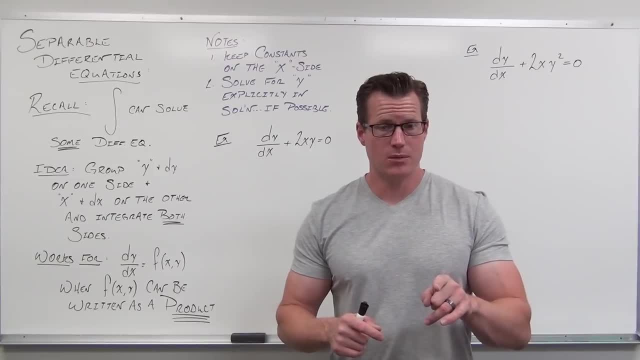 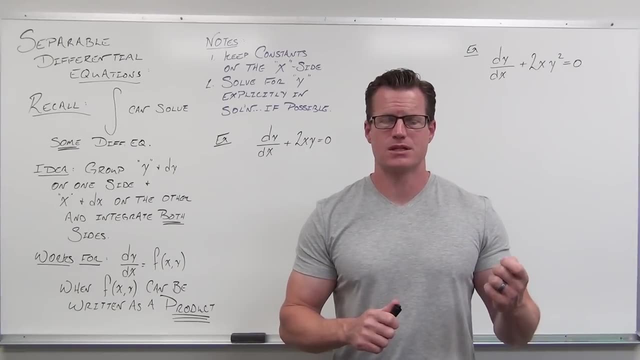 if it's making sense, cool, If it is making sense to you and you don't need any more. skip to the last example, please, in this video and at least watch these singular solutions. The very last one talks about a singular solution, And you need to. you need to understand that this technique. 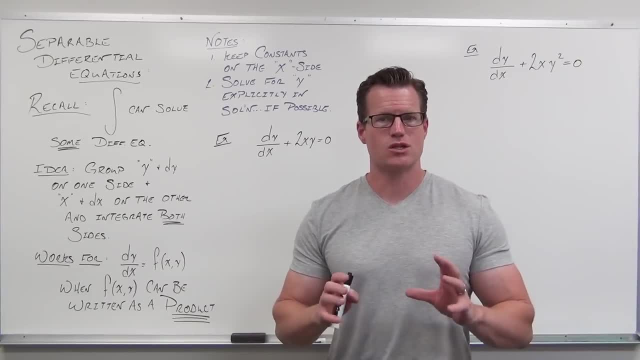 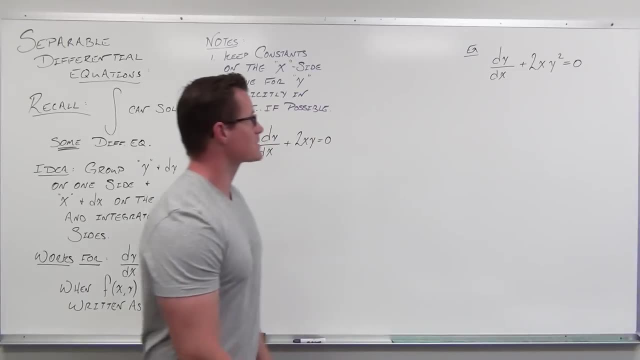 while awesome sometimes doesn't give us these things called singular solutions, It's a solution that doesn't show up by just integrating. So check that out. So let's give it a try, Let's see how this stuff works. So we're going to do two that look very, very similar. They're 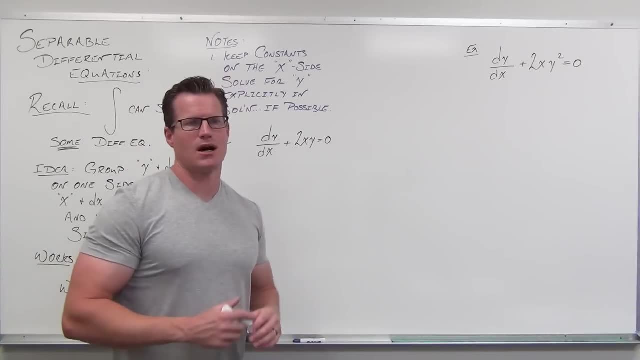 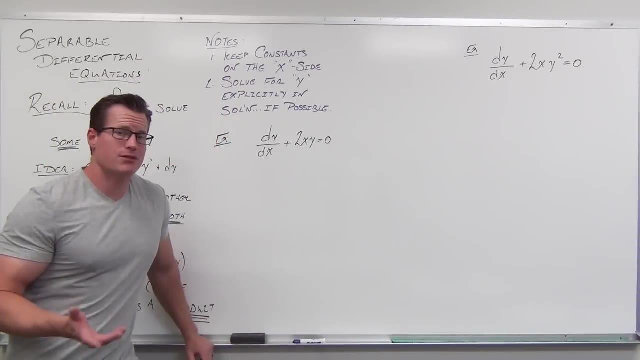 slightly different, And the point is that that slight difference causes us to get a nearly completely different type of a solution here. So let's look at this first differential equation. We have a derivative and, right off the bat, that doesn't look like that. Let's make it look like. 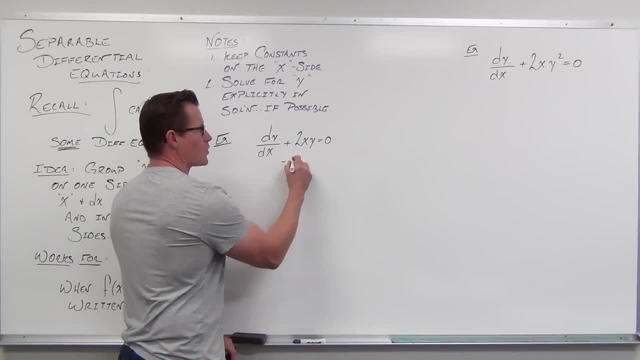 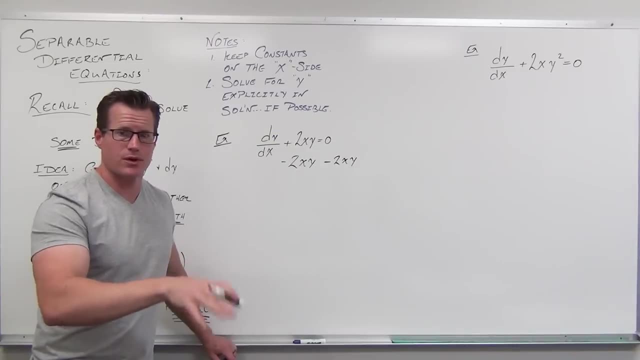 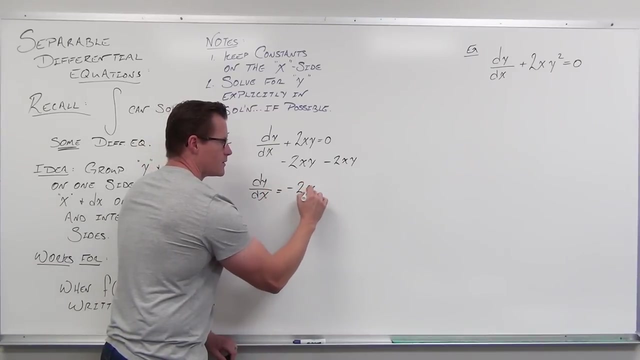 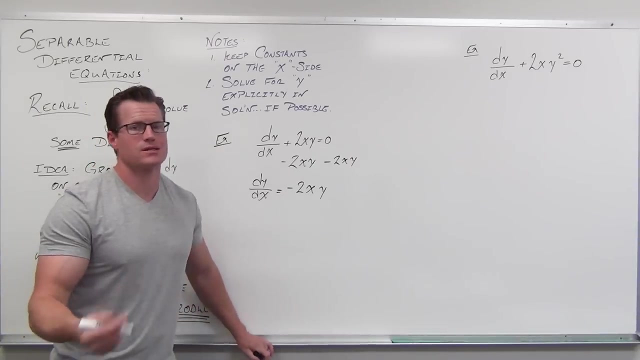 that. So sometimes in our differential equations we have to do some work Just to make it fit our model of being able to separate our variables, this model of I want a derivative that's equal to a product, a product of some x stuff, a function of x times some y stuff. 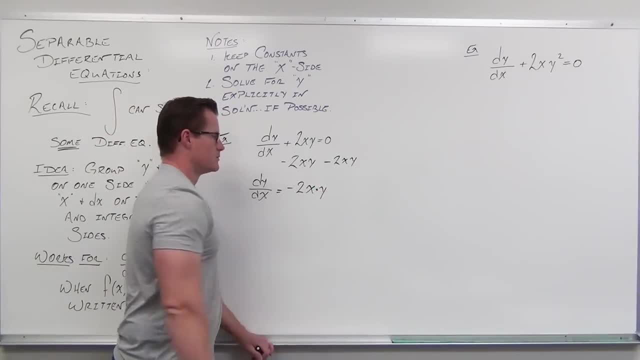 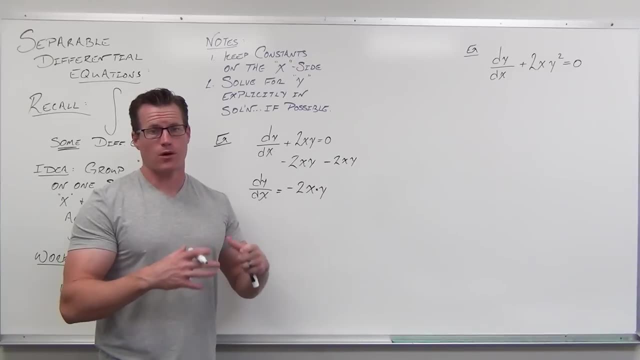 a function of y. Well, I'm going to look at it like that: There's a function of x negative 2x, and there's a function of y, just y. So we are going to to move our variables. What we're going to do? because we have a dy on the numerator of this. 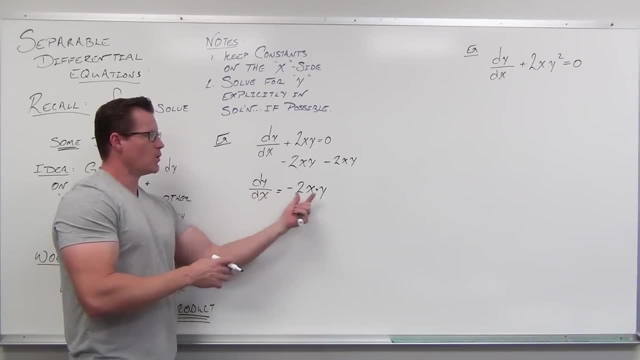 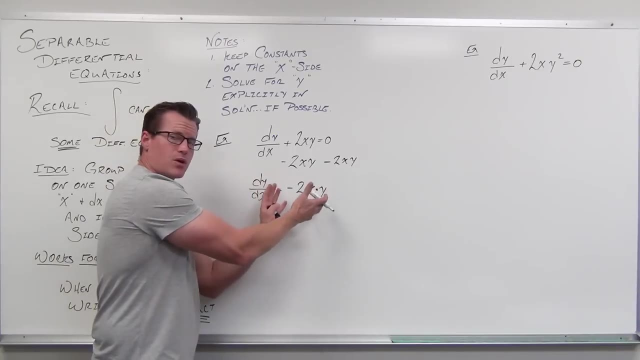 fraction here this dy, dx and dx on the denominator. we are going to want to move our y variables to the left-hand side of our equation by multiplication or division. Obviously, we're going to have a product over here, so it's going to have to be multiplication. 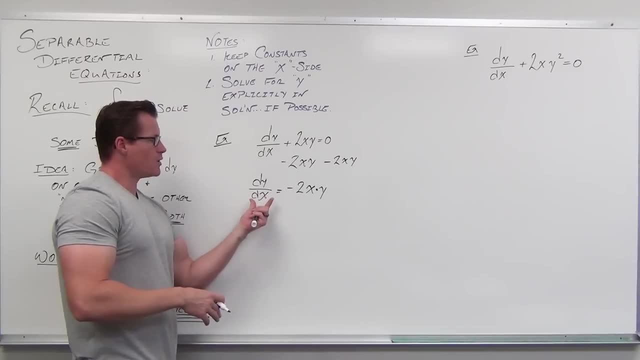 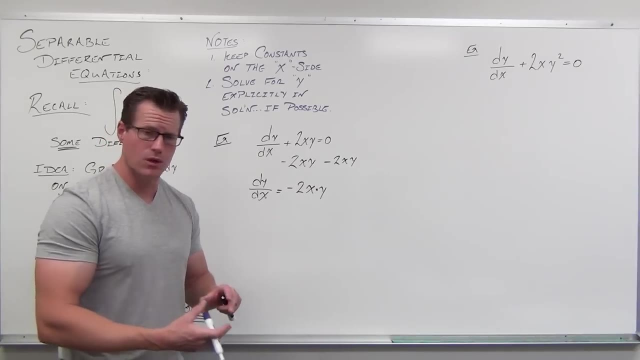 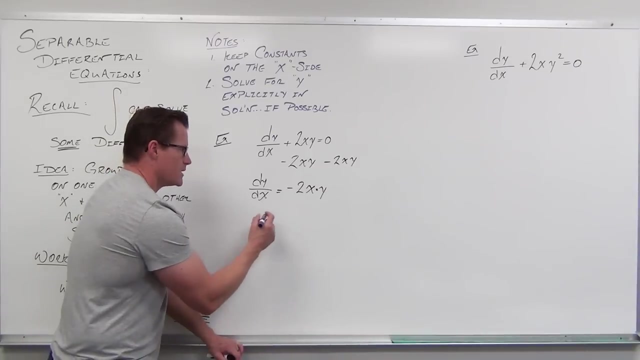 or division to move our stuff. And we're going to move this dx to the right-hand side. It might seem a little weird, but we haven't done this since Calc 1.. It's rare that we do, but you can separate that fraction. So if we divide both sides by y, I'm going to be getting 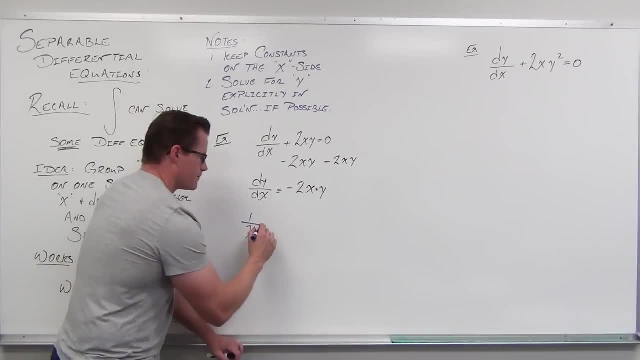 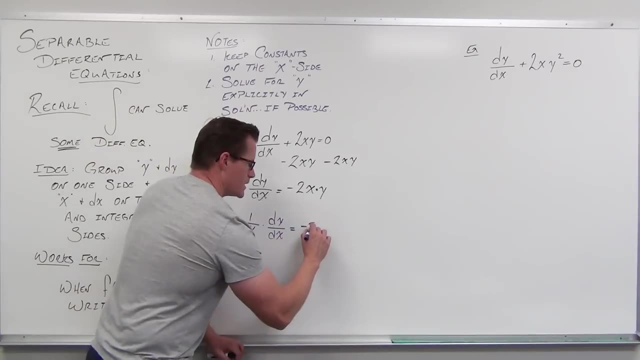 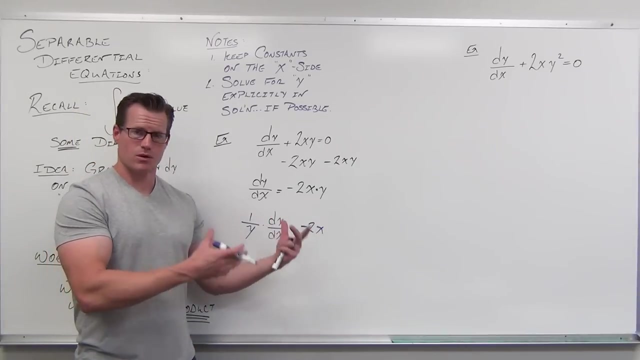 1 over y. dy. dx equals negative 2x. Notice how I'm moving my y. Sure, I'm moving my y and my dy. I'm keeping my constants, my coefficient. it really is what that is: constant factors on the right-hand side. 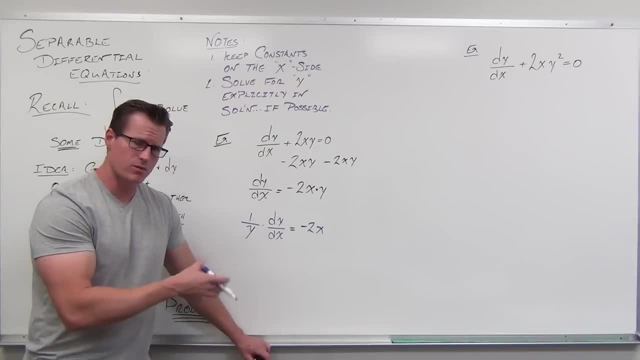 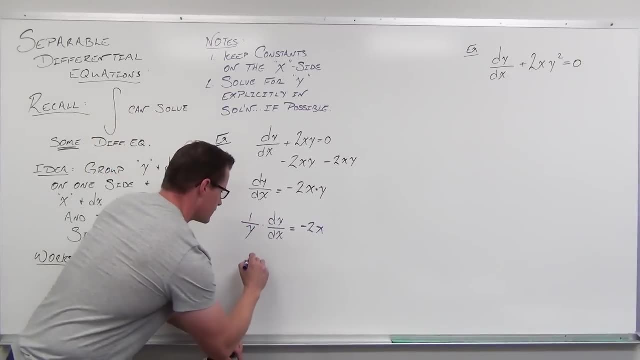 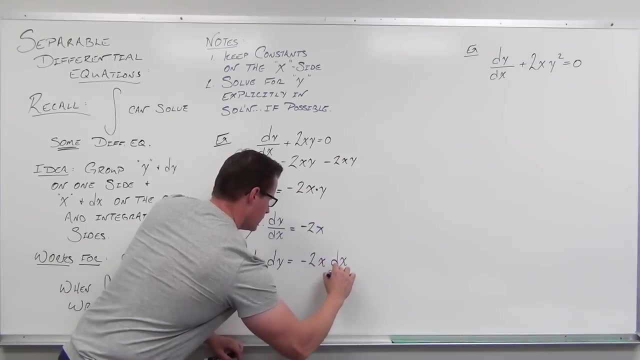 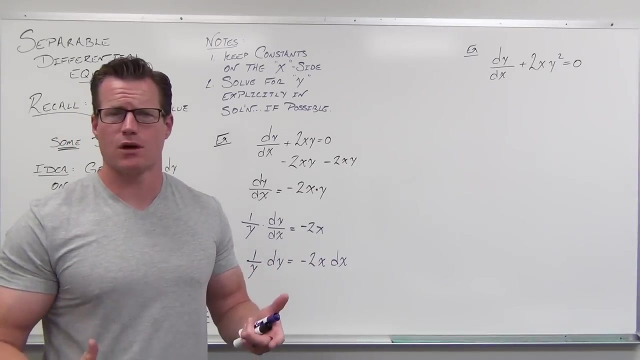 on my x side. Now one last thing we are going to do: before we integrate That dx needs to be on your x side. So if we do that, multiply both sides by dx. this gives us something that we can integrate on both sides, So that man, one of the fundamental ideas of solving equations is: 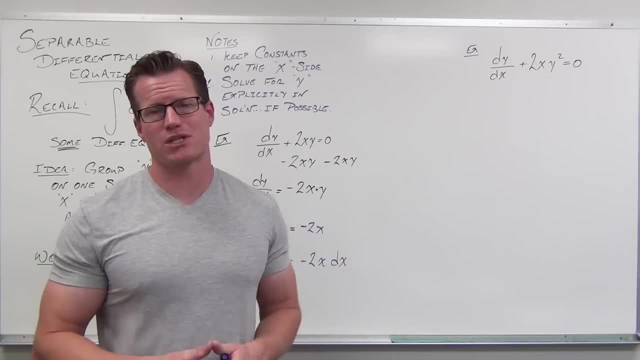 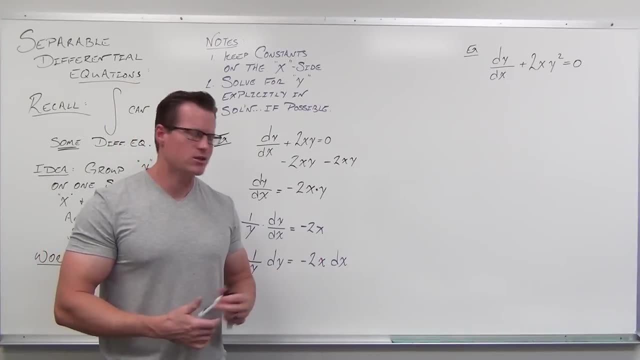 you can do almost anything you want, as long as you do it to both sides. So if we say: well, I want to perform operationally, well, we've never performed operations on equations on both sides, shouldn't you? you do a logarithm on both sides, you. 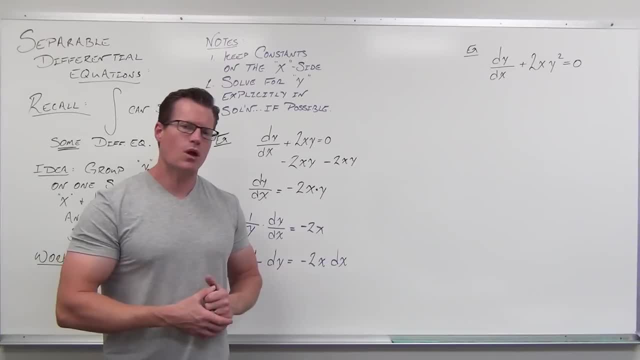 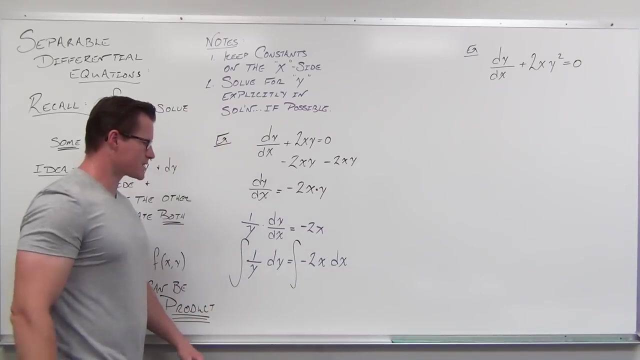 take both sides as an exponent. like exponentials, we do lots of operations on both sides and integrals is an even derivatives with implicit differentiation. you take derivatives on both sides. integrals is another one that we can do this operation on both sides. so if we integrate on both sides, we have this. 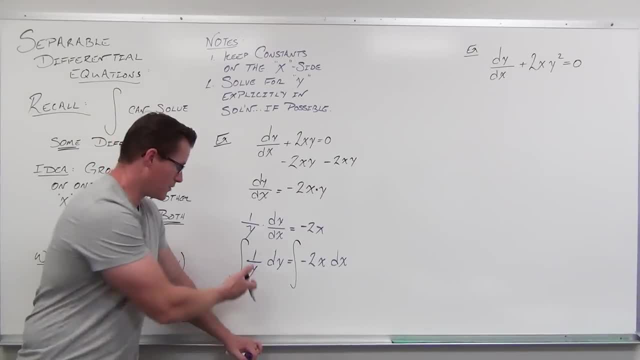 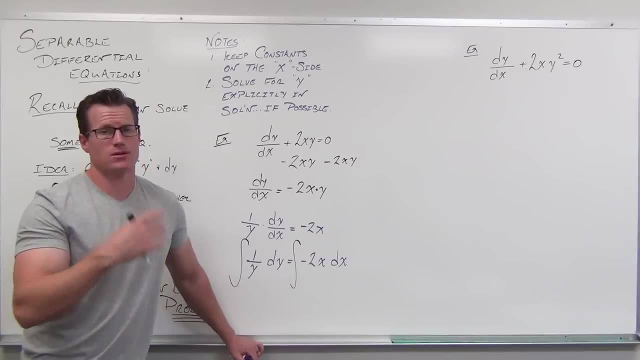 idea of I'm integrating 1 over Y dy. oh my gosh, the variables match up. that's awesome. that's a very easy integral. on the right hand side integral of negative 2x, DX- that's an even easier integral. then the variables match up. so I told. 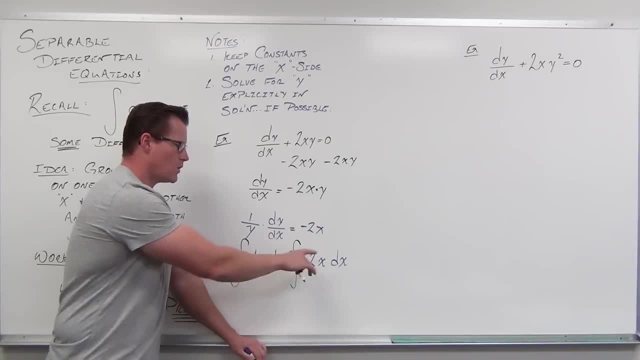 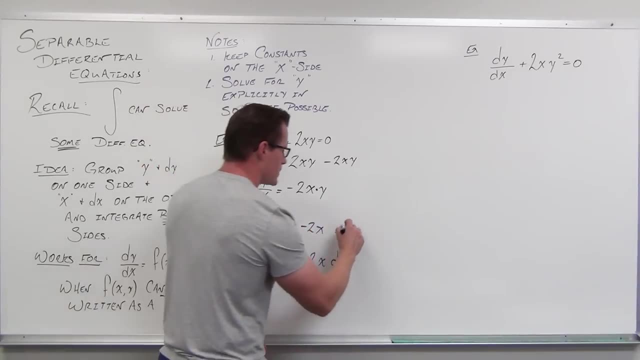 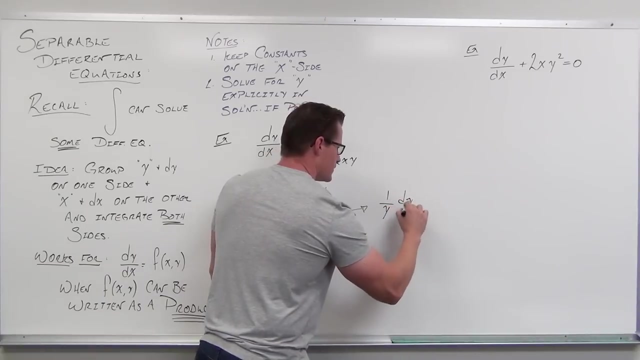 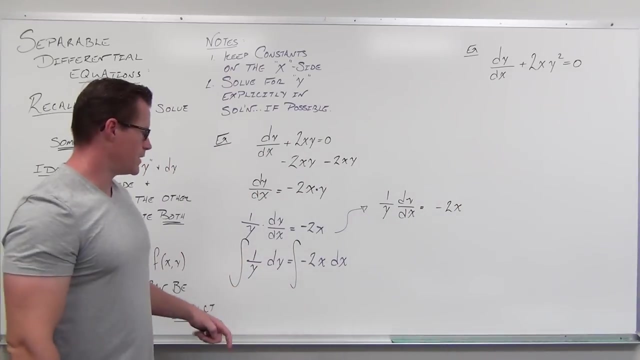 you that I would show you this, I'm sure this one time- that if you don't like this, here's kind of the root of this, this idea too. you can think of it this way. it's a little weird, but if you kept it like this, some people don't like the idea that you are integrating with respect to two. 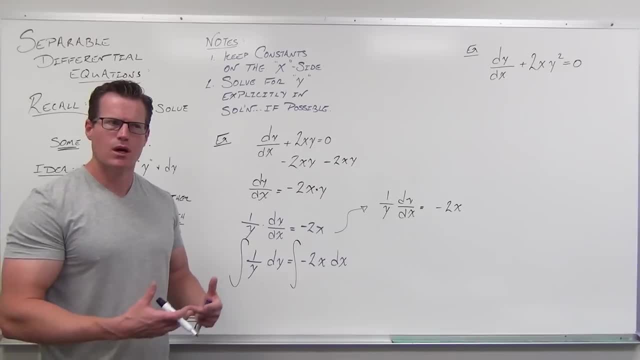 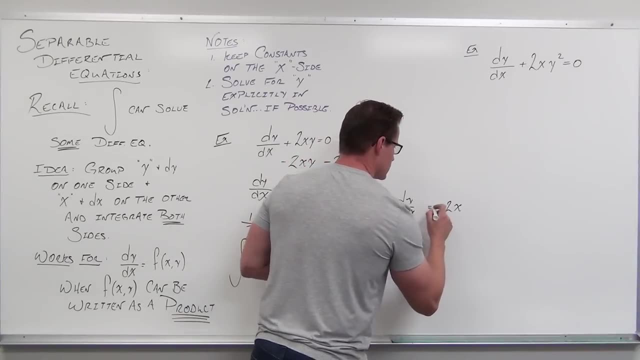 different things. here they: well, this is why that's that's X. so you're not really doing the same thing if you think about it this way. well, what if I integrated one side DX and integrated the other side DX? these DX is actually do cancel out. these DX is actually do cancel out. 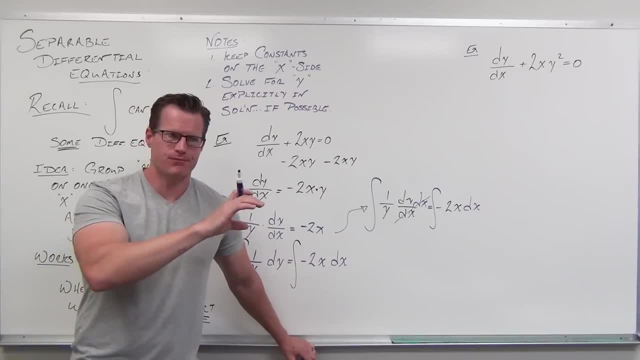 from the root of where they came from. on the definition, what a derivative is, we have those like Delta X in a limit. so where that comes from, you can actually remove my showed in a video in calc 1, but that's, that's possible. so if you, 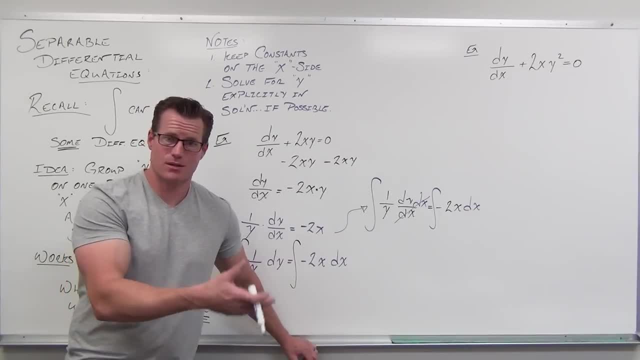 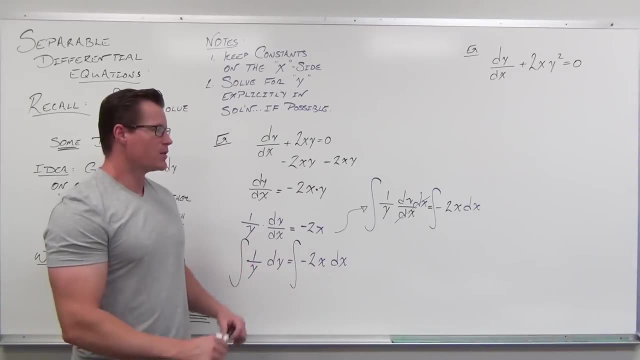 want to think about it that way, like, hey, you are integrating with respect to X on both sides. it's just that this X and X go away and you have the dy. still, you integrate respect to Y. think about it that way if you want to, I don't care. the. 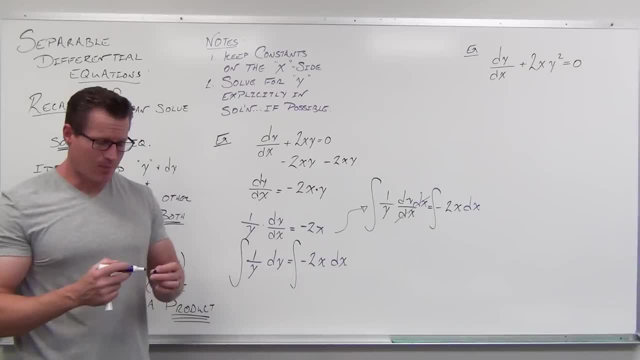 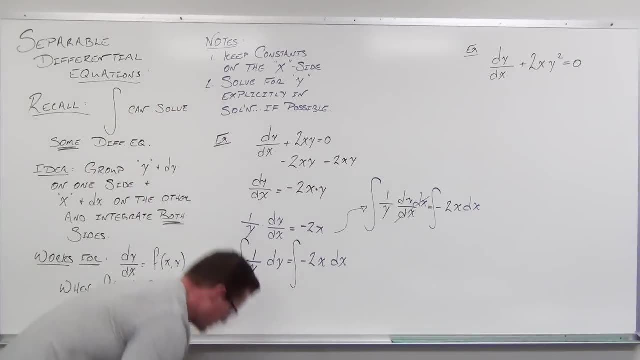 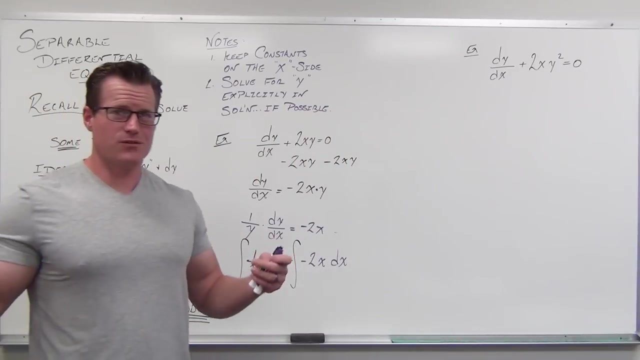 point is that, but these, this actually does work. we can separate the dy DX and integrate both sides, and mathematically that's a nice tool for us to be able to rely on, so let's use it if we integrate. and again, most of this this video is about integration techniques. the idea 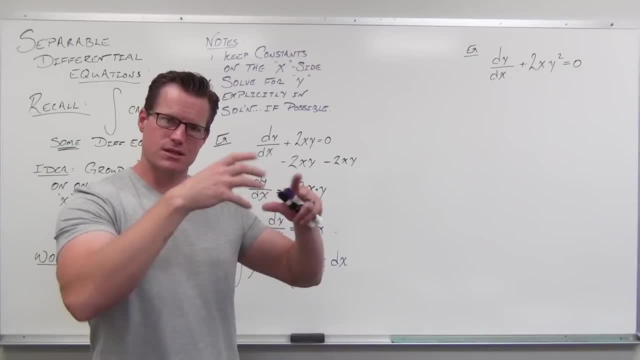 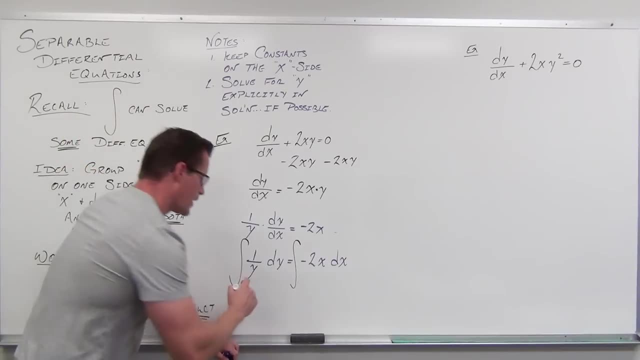 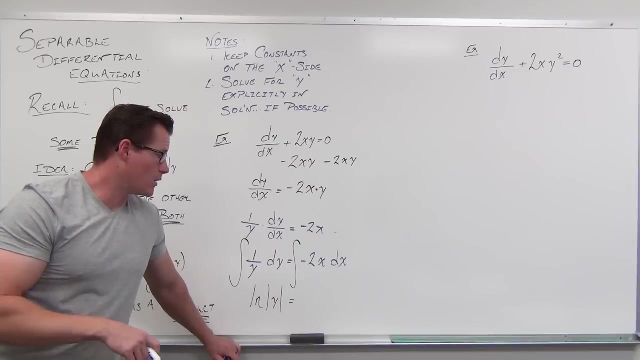 really basic: move your Y's, move your X's dy, DX, group them and then then integrate. so we need to remember that things like integral of 1 over Y dy and be able to arrange that시면 Willa is an absolute value of Y on the right-hand side when we integrate this. 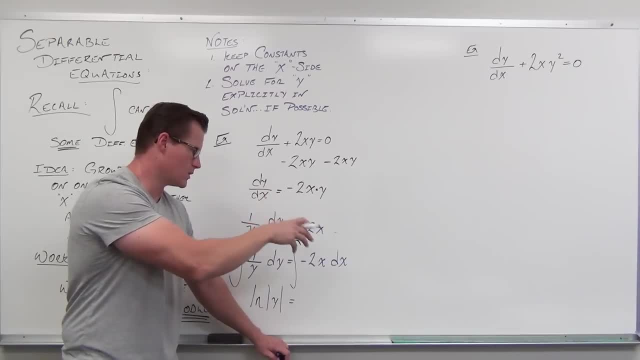 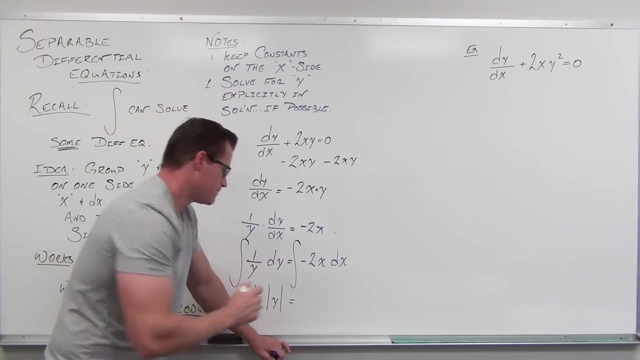 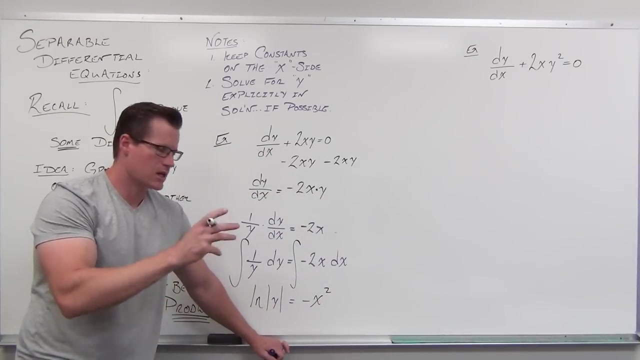 negative 2x. you can pull your negative 2 out as a constant, so a coefficient can move out in front and we integrate. or just think about just a negative, if you want to. this should be negative X squared. so when we integrate that, we get this negative X squared. if you want to do the derivative real quick, 2 and so we negative 2x. 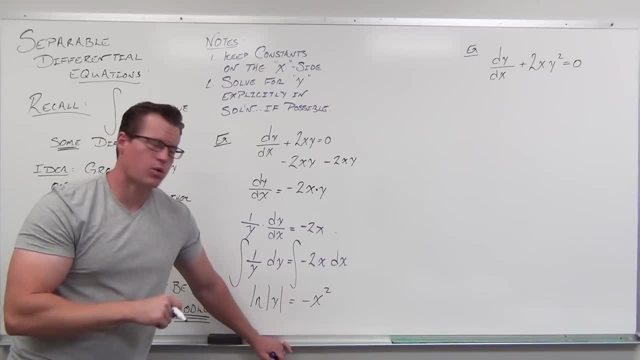 that's great, Importantly, like really important, you're always going to get a plus C. Now, it should be in your head right now. well, wait a minute, I'm doing an integral on both sides. When I get a plus C on both sides, the answer is yeah. 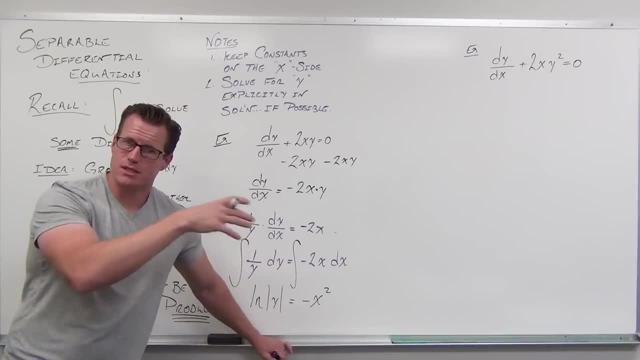 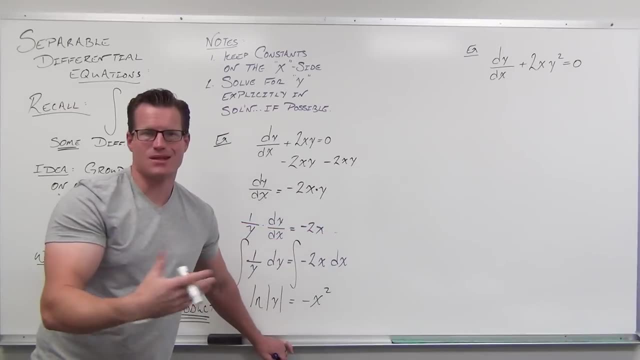 you could make that argument, but because you get a constant on both sides- this plus C- on both sides, you could add or subtract one of them to the other and you'd get this other arbitrary constant. So we really only need it on one side. We choose the x-side because we're trying to solve for y. I hope that. 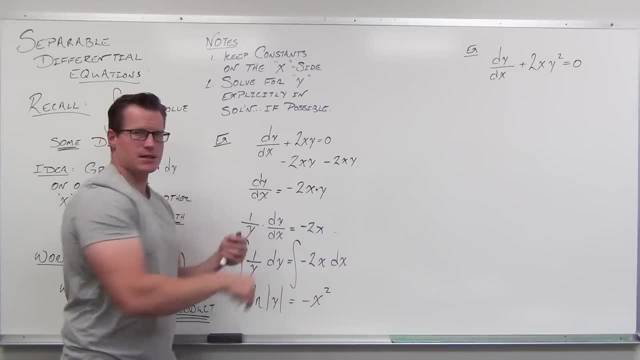 makes sense. So make it fit. separable equations, if you can, separable difference equations, separating the variables. so make it look like a product. Get your x's on one side. with a dx, I pointed to the wrong type. Get your x's on one. 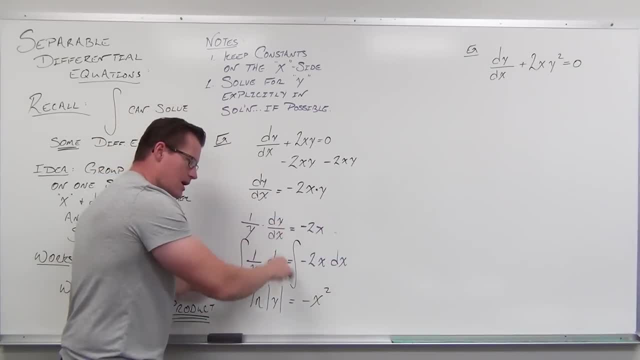 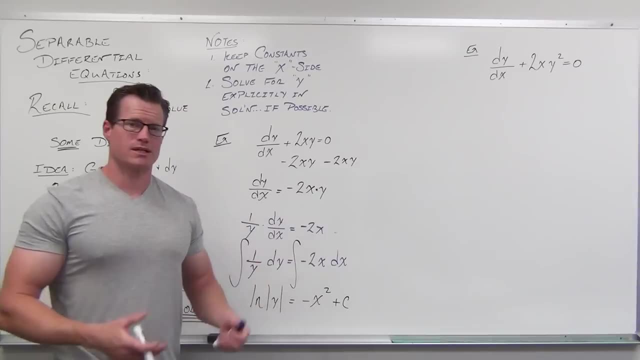 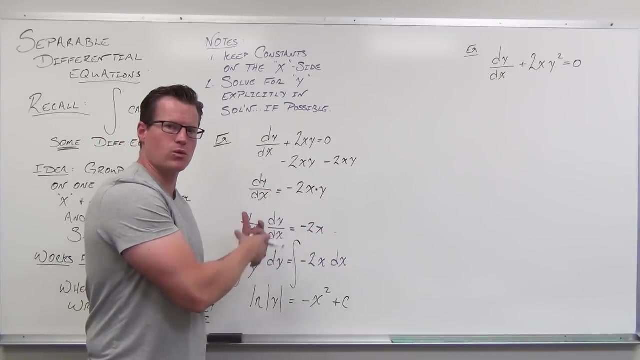 side with a dx, your y's on the other side with a dy. Integrate both sides and try to solve for y. You only need one plus C, because if you had two plus C's, like minus two and plus three, you could group them on one side You could just add or subtract one. 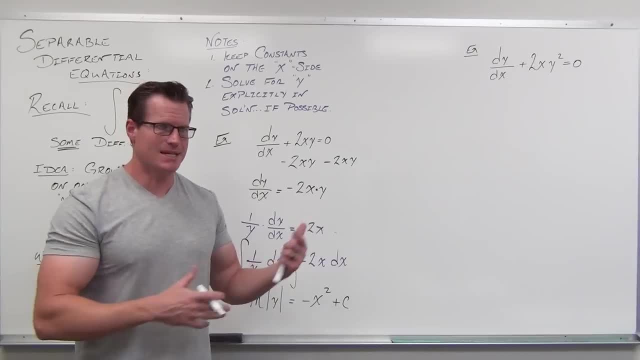 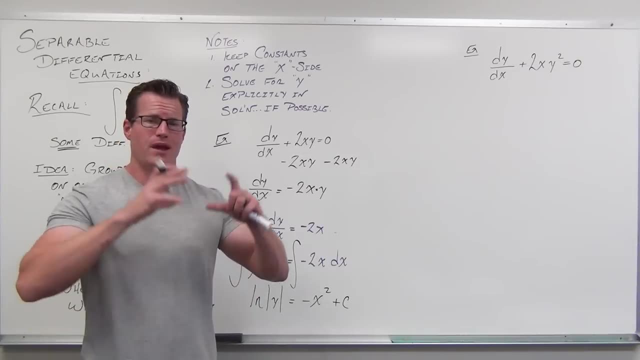 constant to the other. And remember we're talking arbitrary constants, So it doesn't matter what it is, It's creating this general solution for us. Do you remember general solutions? The general solution is this family of curves that has an arbitrary constant in it that says you could plug. 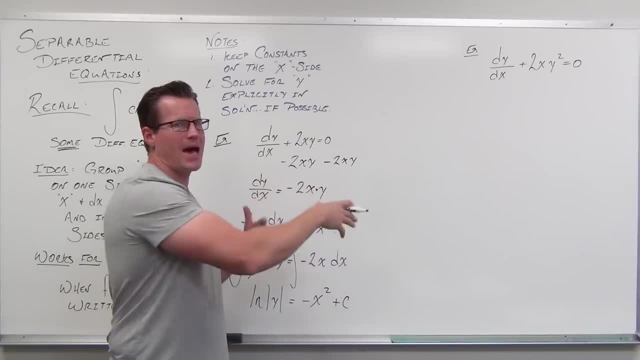 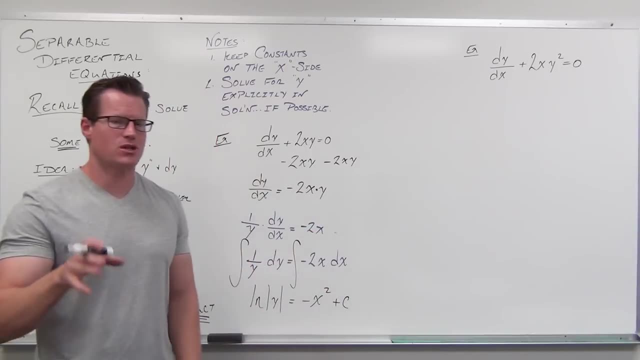 in any number and it would still work. So it doesn't matter that we have a plus C here and here. we would just subtract or add an arbitrary constant and group it on one side. Now I'm going to do something weird. I'm going to call this C sub one, because what's going to happen is in our 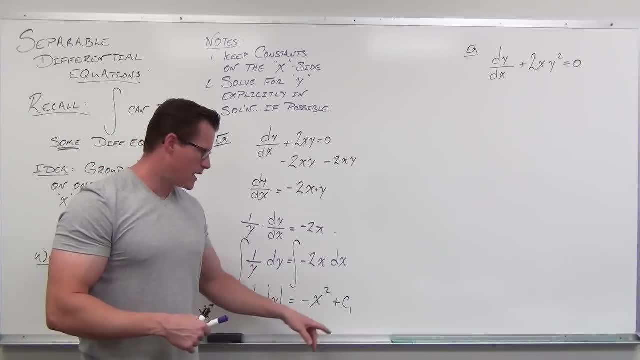 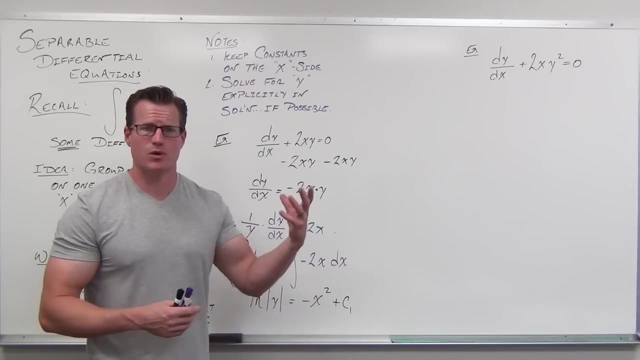 process of solving for Y, we're going to start multiplying that number, whatever that is, times other numbers And we're going to take it as an exponent on E in just a little bit, because we've got a natural log. So I'm going to call it C sub one for a little bit And this is: 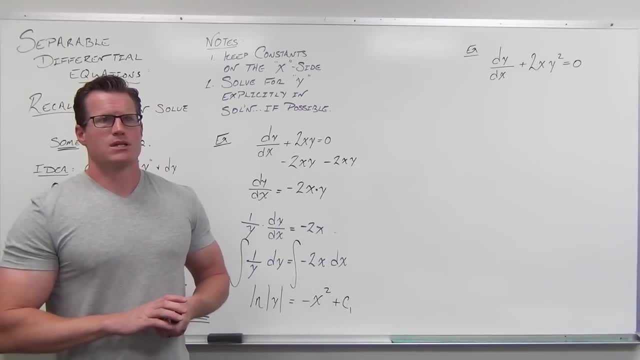 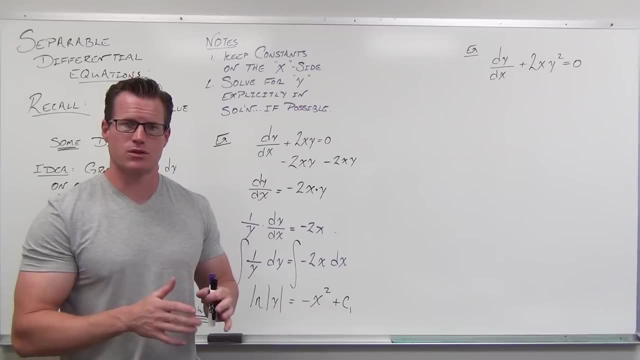 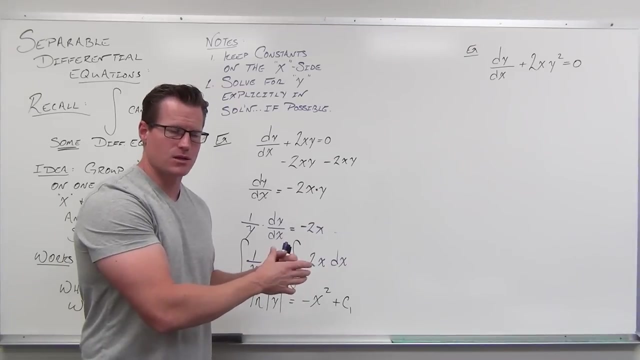 um, man, I don't remember When it was- I think it was calculus two that we started talking about this, One of the first few videos. there's a section on simple, simple differential equations, separation of variables idea where we have an arbitrary constant. Now that constant when you multiply it by another. 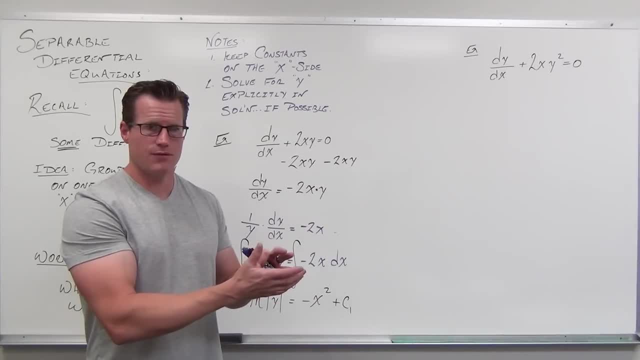 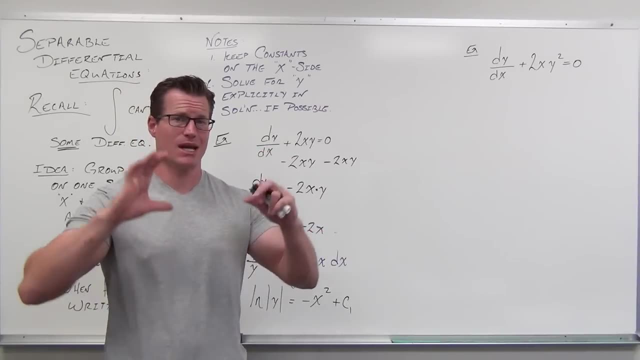 number like a factor, it's still a constant. And if you take it to an exponent on E, it's still a constant. So we're going to allow that to happen And at the very end we're going to say, Hey, this thing right here, that looks really nasty. 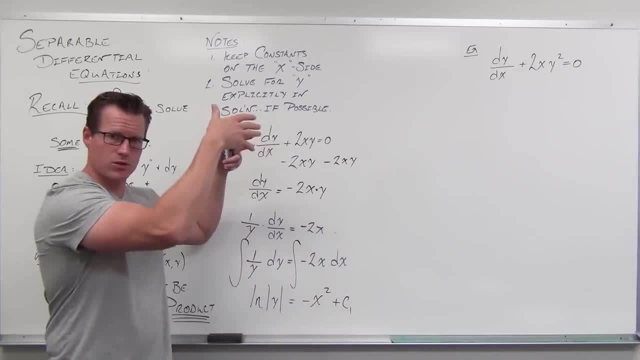 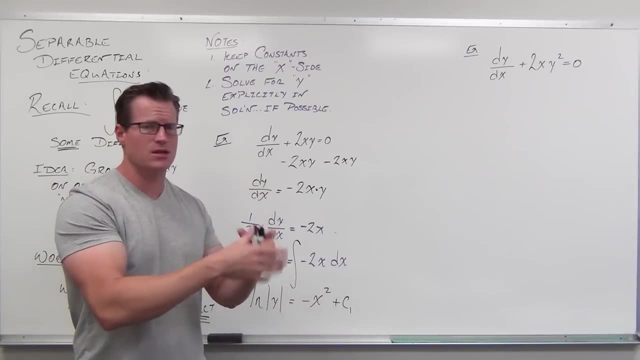 That's just a constant. So we're going to leave that for just a bit. As we work through our examples, it's going to happen to like every example we do, And then at the end we're going to say: this thing, that's got the C one in it. That's still a constant. We're going to call it. 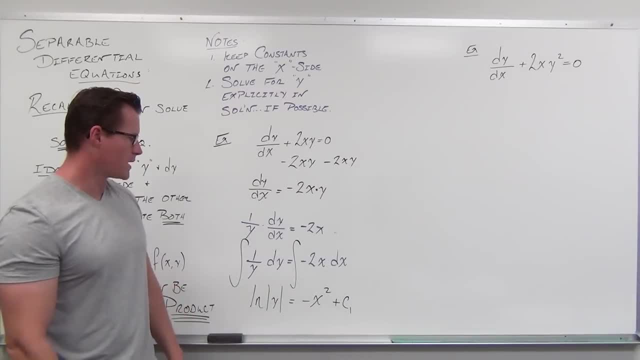 the arbitrary constant. I hope that makes sense. Just just watch out for it. So let's go through the process of solving this for Y. We need to solve explicitly if we can and we can. So what undoes a natural algorithm? Well, we're going to. we're going to take E on not going to take E. 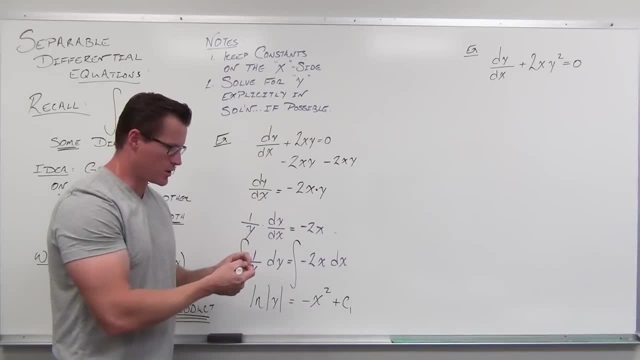 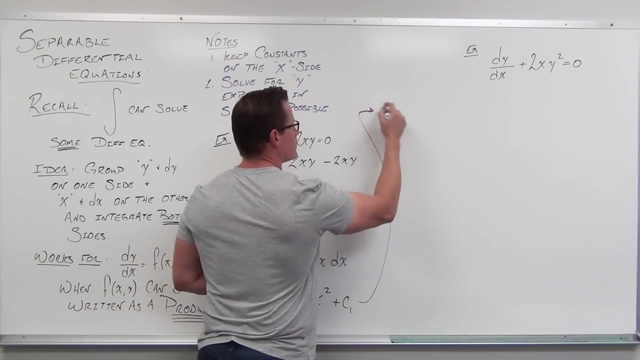 but like we're going to put an E on both sides and treat both of these as an exponent, So ln absolute value Y equals negative X squared plus C. We know that the exponential, that is, the inverse of this, is E, So you can show it this way. You really don't need to go all that in depth and 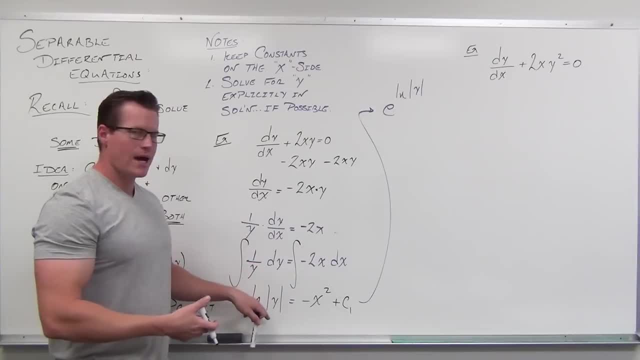 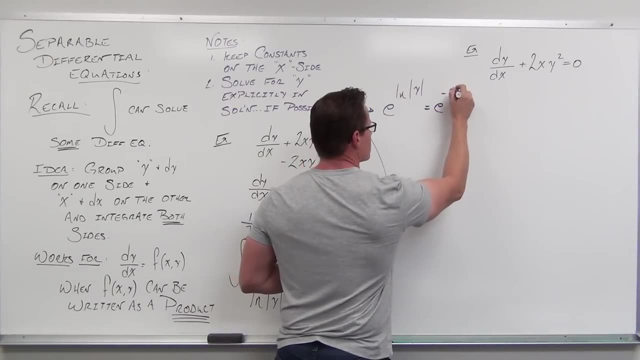 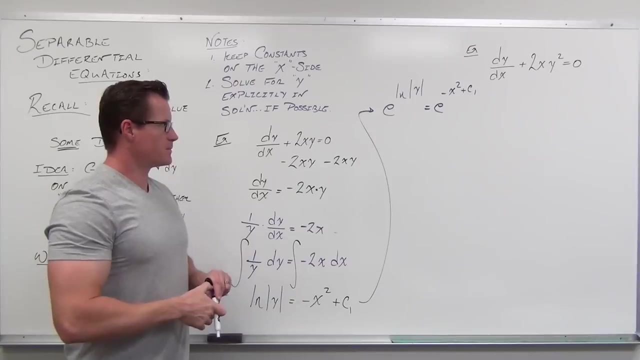 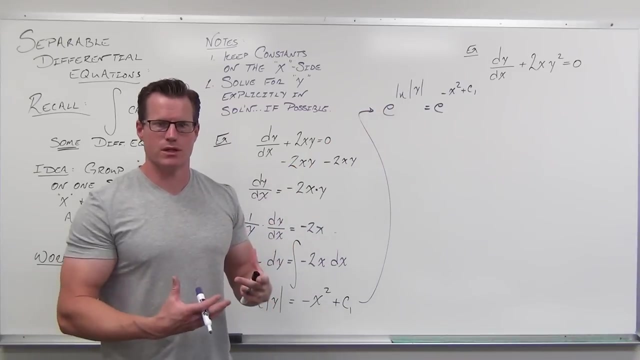 show that You can just say: man, yeah, Y. absolute value of Y is going to equal E to the other side. So raise both sides to the exponent as an exponent on E. These are a composition of inverse functions. They're always going to cancel out. That's going to leave you absolute value Y. 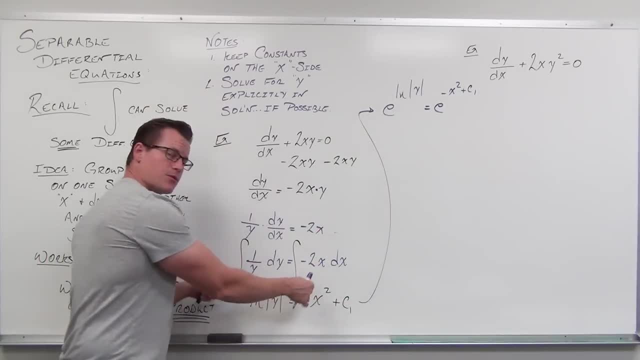 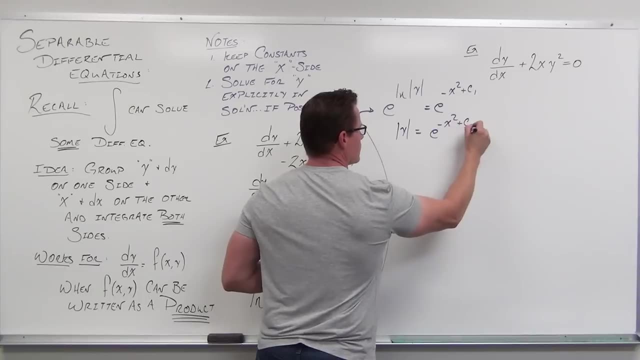 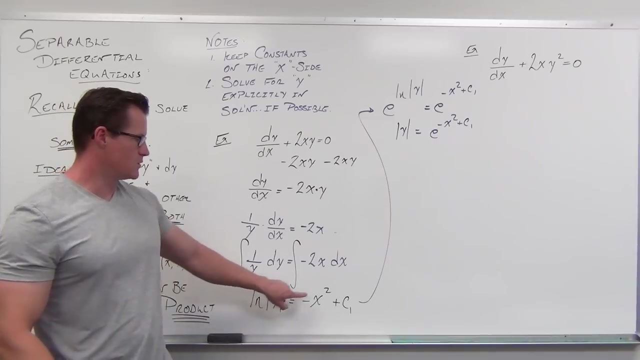 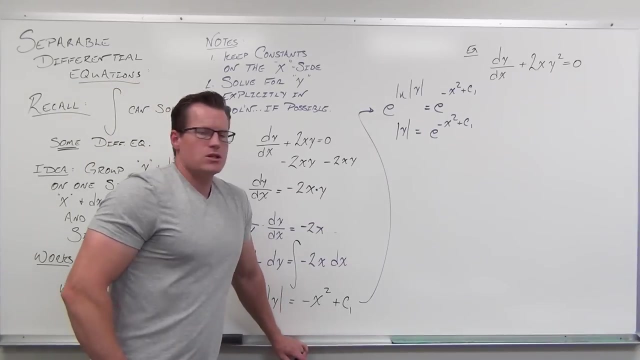 Most people don't even write this. Most people go directly from here to here. They go. yeah, this is a base of E. E to the other side equals argument, And that's how this, these logarithms, work. Now, I was mentioning to you a little bit before that we're going to 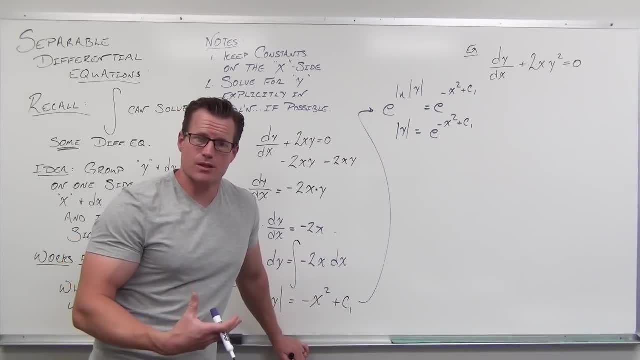 have C sub one as an exponent on something else, And then we're going to have it multiplied by another number or another positive or negative, And so here's- here's how that works. If you want to solve for Y, you need to get rid of this absolute value, And this doesn't look all. 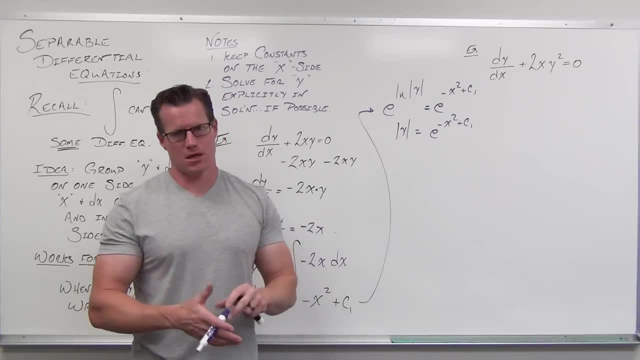 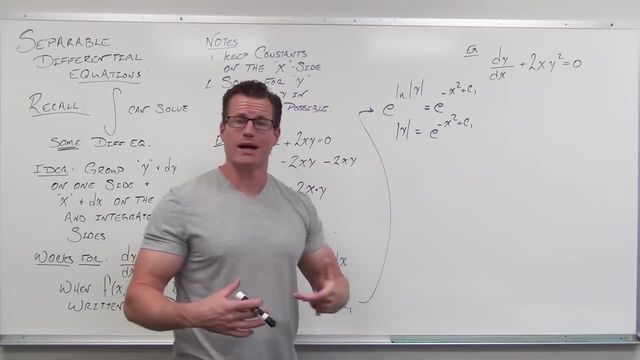 so good over here. So here's some ideas that commonly come up in solving for Y explicitly. A lot of times if you have E to an exponent where there's a plus or minus, do you remember that when you have a plus or a minus in your exponent it came from common bases being? 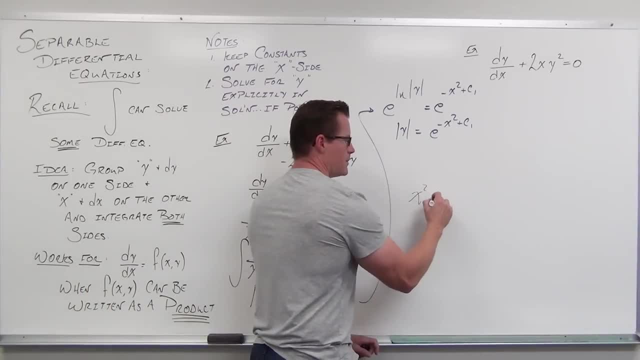 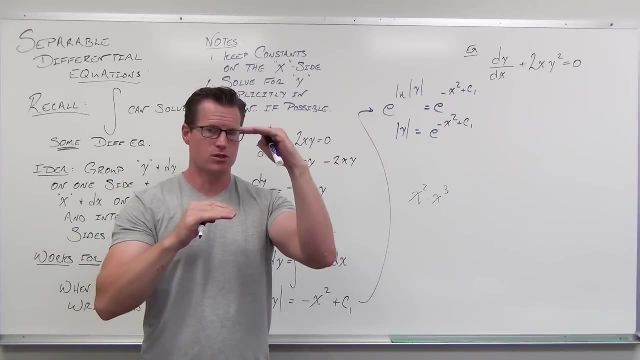 multiplied. If you have common bases being multiplied, what you do with exponents is always one operational level below what you see. So if you see multiplication that involves exponents, what you do with your exponents is: let's see what's one below multiplication. 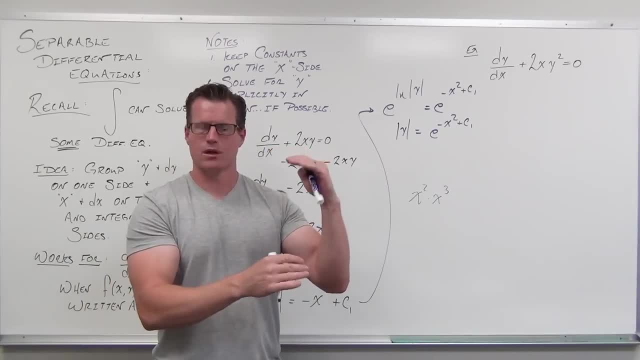 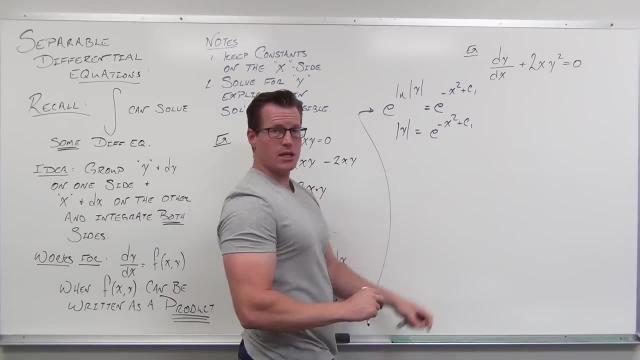 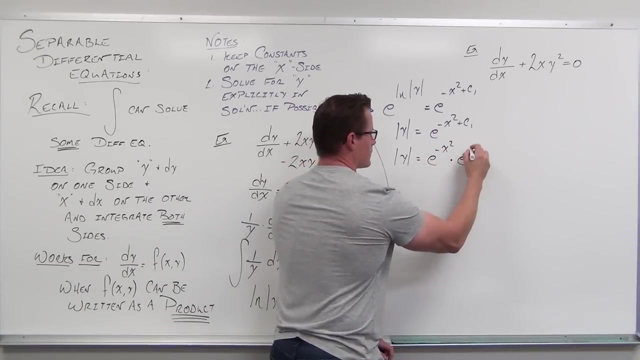 Addition, What's one below division, Subtraction? So when we see that what we're going to do is imagine that if we have addition in our exponents, we could actually write this as common bases, It's going. it's going backwards. If you had common bases, you add exponents. If we 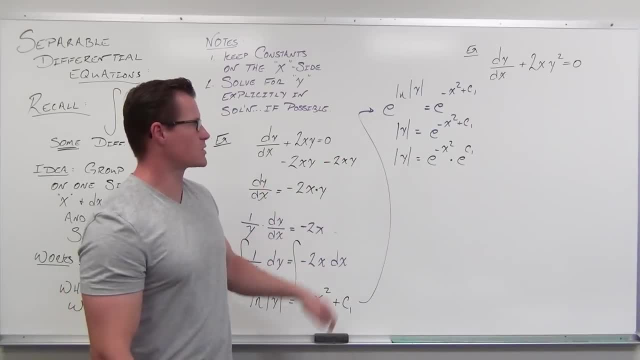 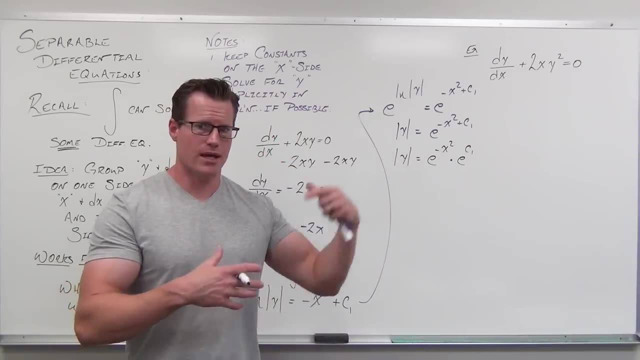 have adding exponents, we have common bases that are multiplied. So that's what's going on. Notice how we have E to the C1.. E to the C1,, ladies and gentlemen, it's still a constant. If you take E to that C, whatever it is, any number in the world. 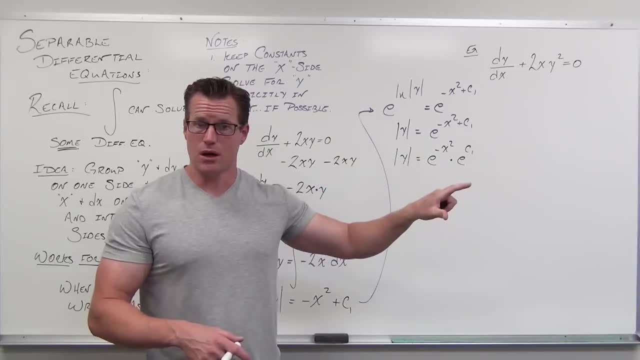 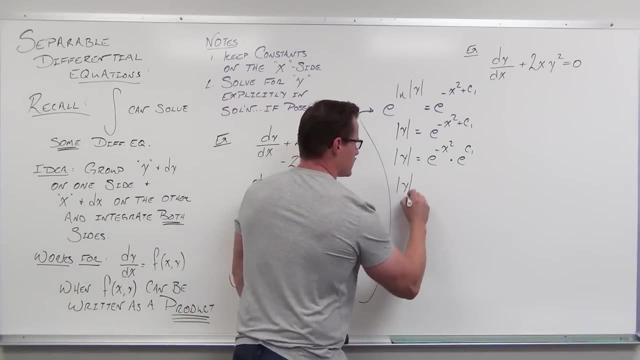 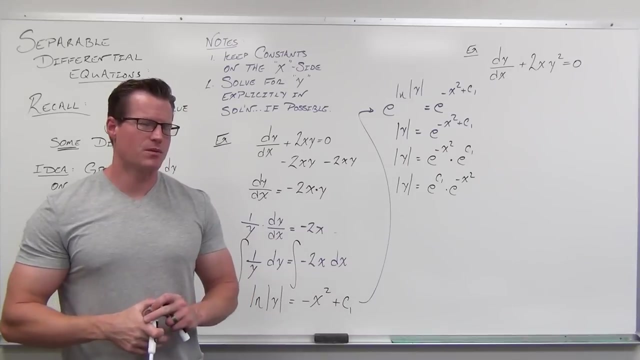 it's going, because the domain is anything, you're still going to get a constant out of it. Now the idea of absolute value. this also happens a lot. Let's move this around for just a second Here. The idea of absolute value: do you remember the definition? 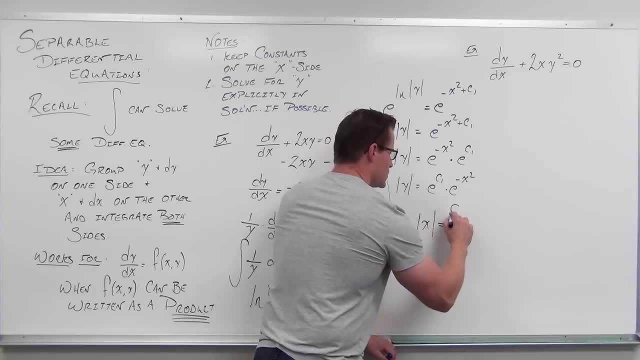 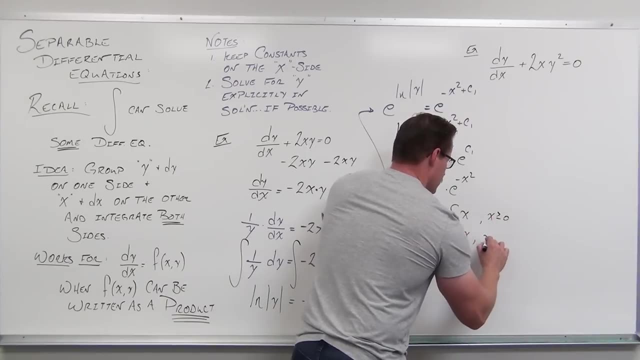 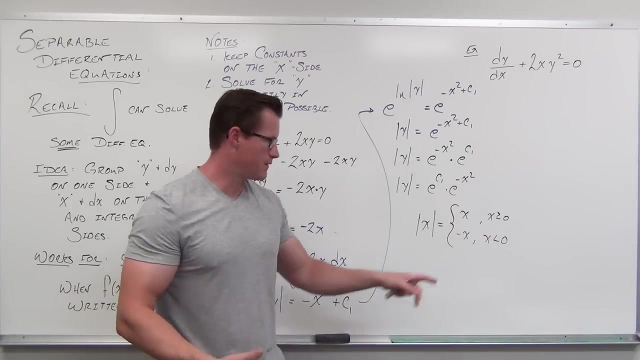 The definition of an absolute value says you get X if X is positive and negative X if X is negative. That way we always get a positive out of it. If that's a negative number, you say: well, I'm multiplying by negative, It's going to end up being positive. 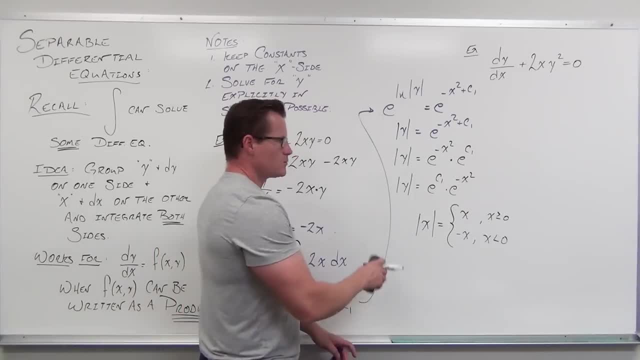 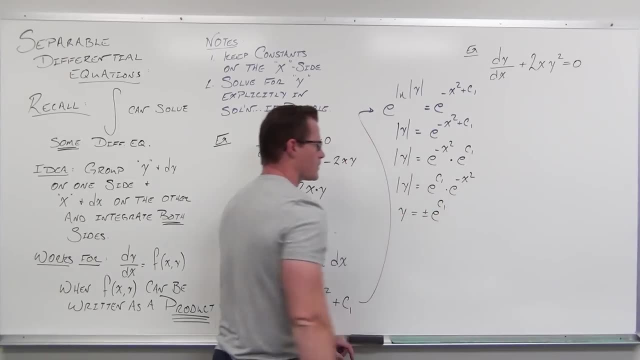 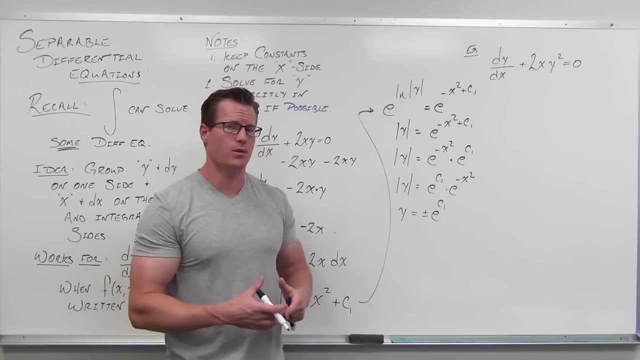 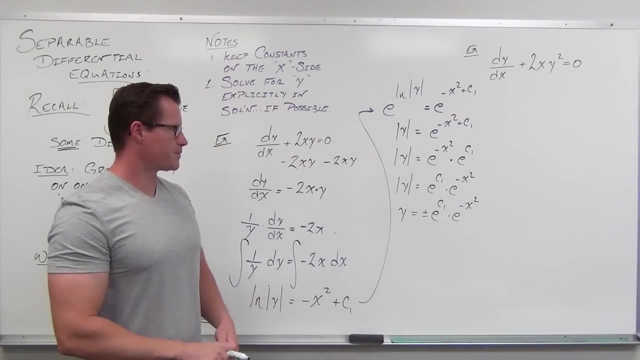 That's how absolute value works. What that means is that whatever we have here, we can always change this to the absolute value of Y equals plus or minus whatever Y is. So that's something we can always do with that absolute value. It's kind of nice If that happened to be positive, we'd keep the 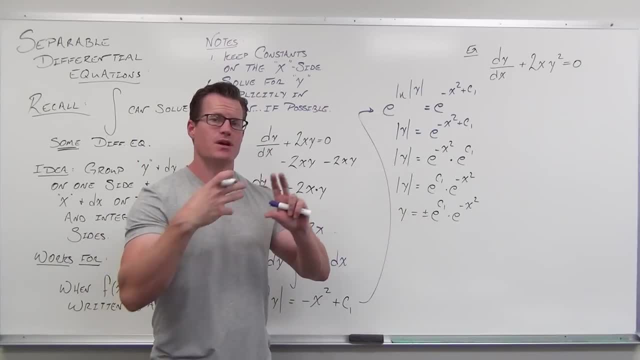 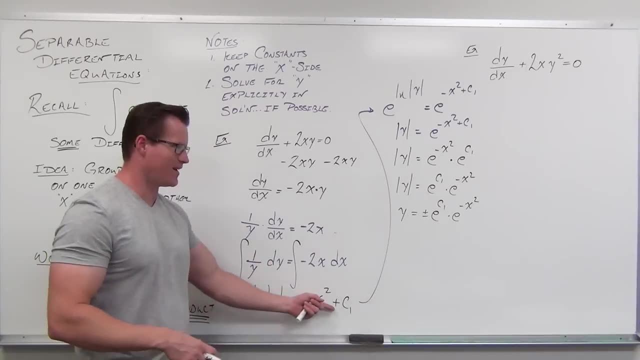 positive. If it happened to be negative, we'd keep a negative, and a negative times negative would give us the positive Why we're doing all this and why we call that C1, because if you still didn't get it, you're like what? 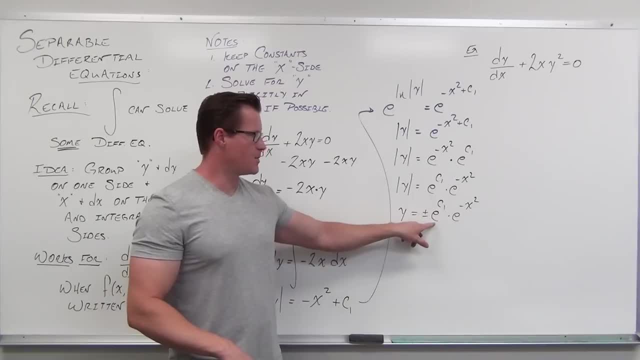 Right now. I want you to think about that, because you have this number- E, 2.7, something, blah, blah, blah, blah, blah- forever natural number. You're going to raise that to a constant. This is still a constant right here and it's based on whatever that is In fact, you could. 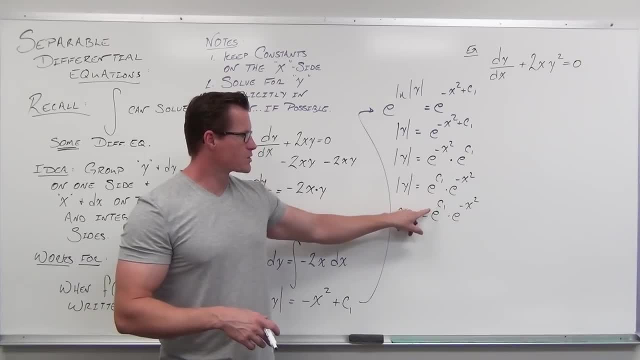 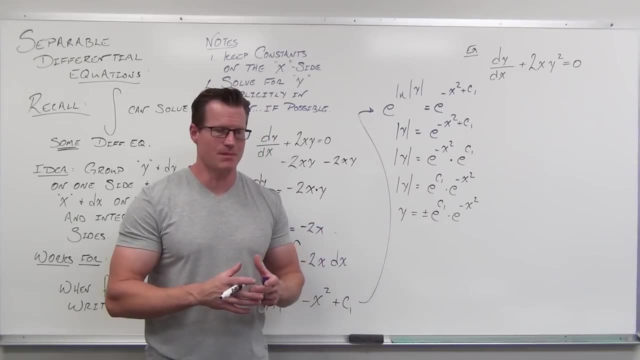 get back the first constant by plugging something else in, But you're also going to have either positive or negative. The point is, this whole expression is still a constant. It doesn't matter what it is. No, it's an arbitrary constant. 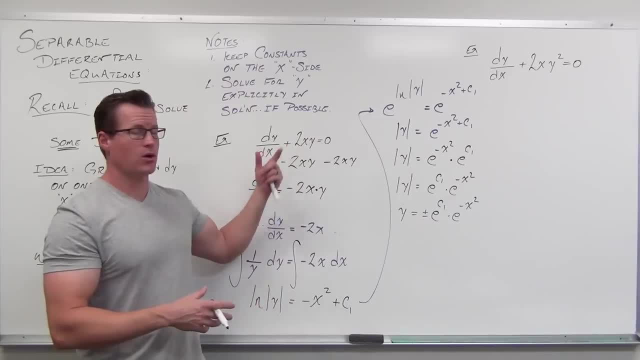 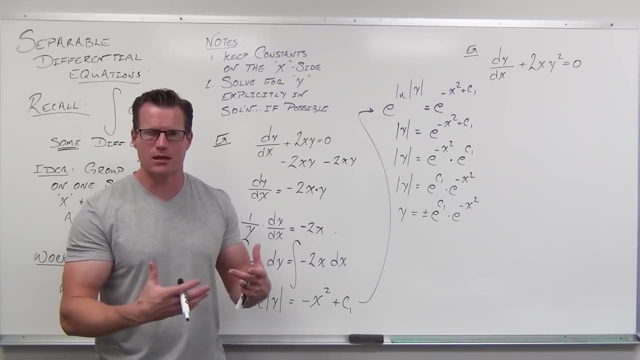 The point of that is the derivative of that is going to satisfy our original differential equation. Remember what we're trying to do. We kind of get lost in some of this. We start crunching the numbers. You're not really thinking about what we're doing. We're finding a function. 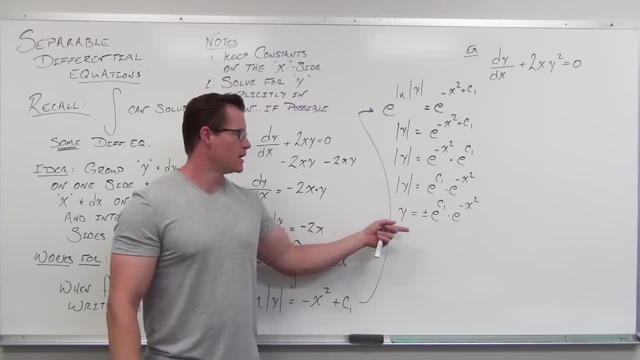 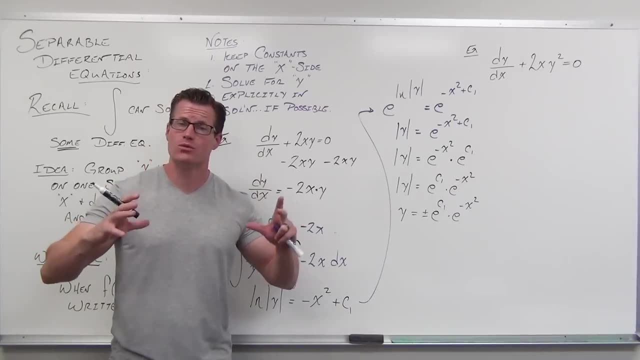 so that when you take a derivative of it, it's going to satisfy this, which is really cool, And any arbitrary constant is going to work. We're creating a general solution here. We don't have an initial value, so we can't find a particular solution. 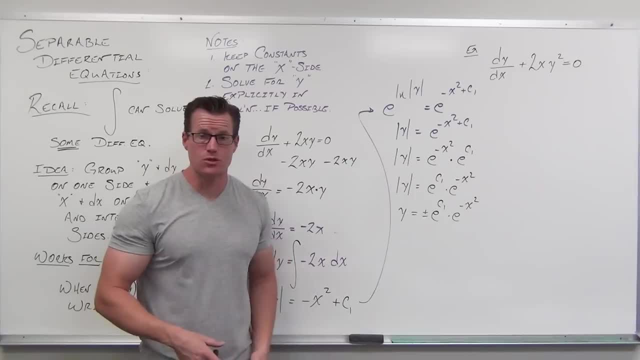 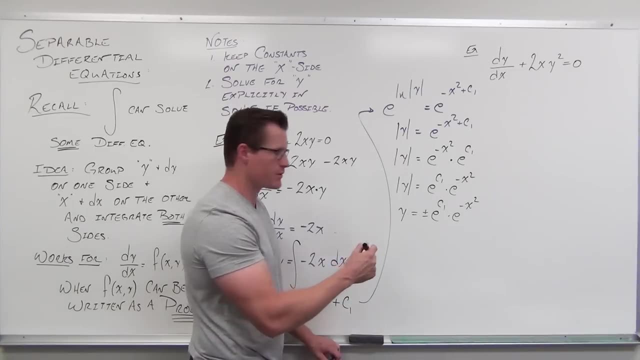 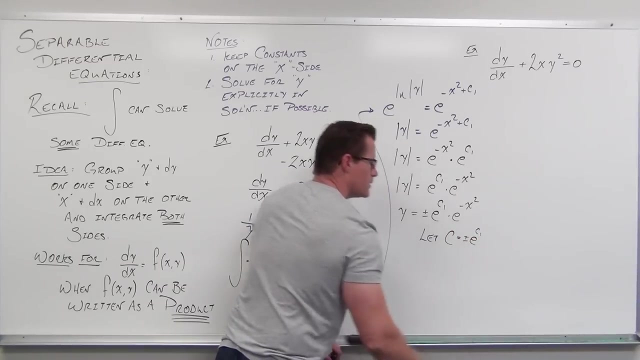 That's something that's going to come later in another video, Next video, I'll talk about particular solutions. So what we do, what we often do- and we don't even really identify it sometimes—we should every time—is we say: let's let C, this arbitrary constant, equal that constant there. 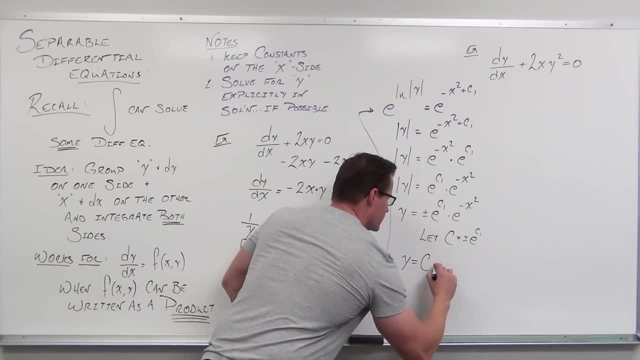 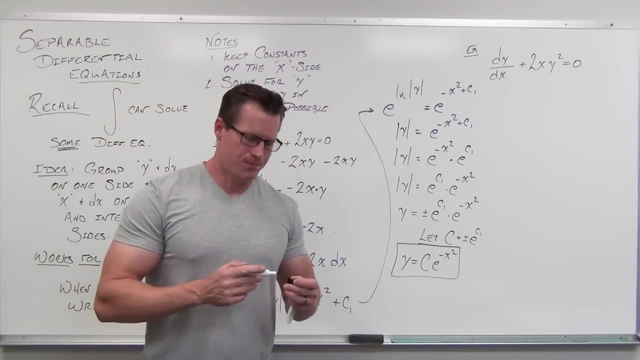 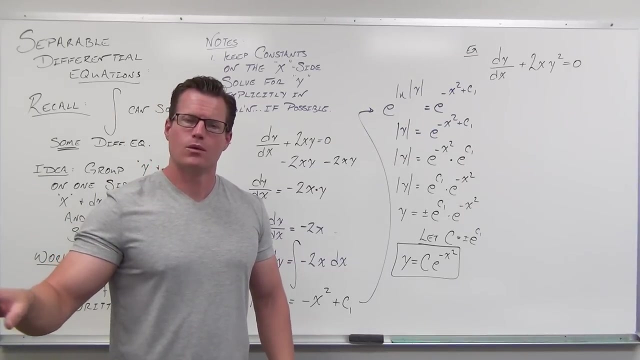 And when we solve for y, look at that. That's why a lot of times we're going to get this from the answer. You know you're going to think about it several times on your homework, when you're going through it, or your practice and you go, man, my answer doesn't look anything like. 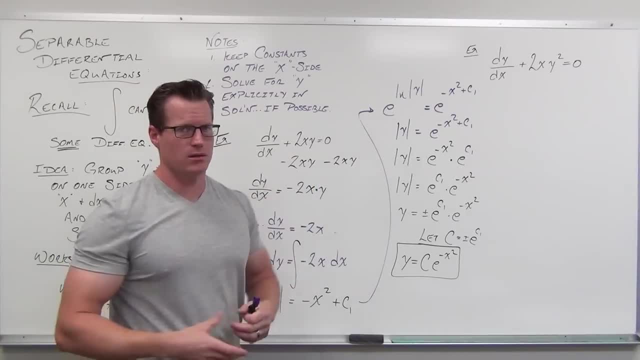 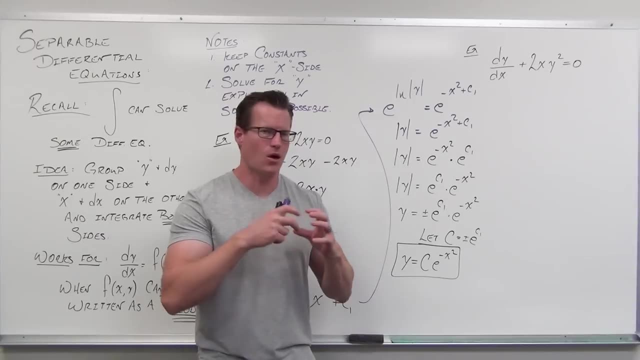 what they're doing. It might be—if you're not making a fundamental mistake, an integral mistake, sine error, something like that- it might be that they're moving around their constant and adjusting for it and taking that whole garbage out at the end and saying: that's still a constant, Let's call. 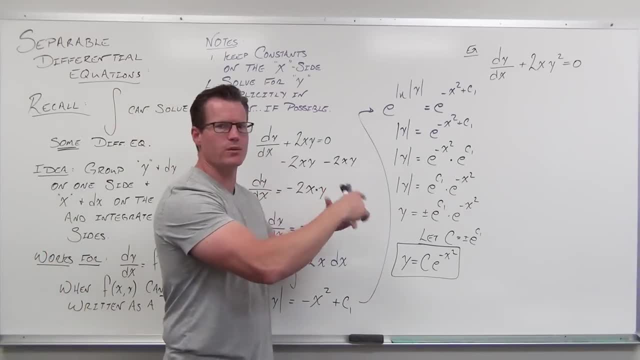 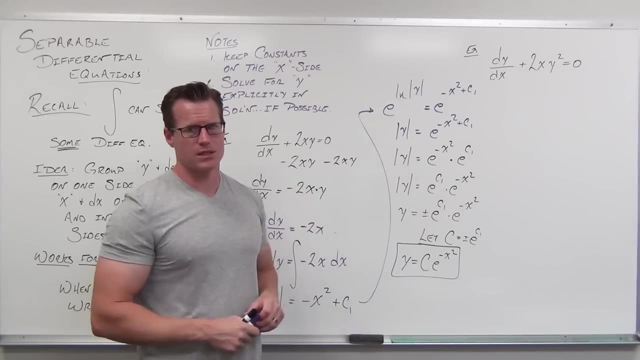 it a constant. That's the reason why we write the C sub 1, so that later on, when we do multiply it plus and minus in front of or positive negative in front of it, we can call the whole thing a constant of n. I wish I could ask if that makes sense, but I hope that it does. This is solved. 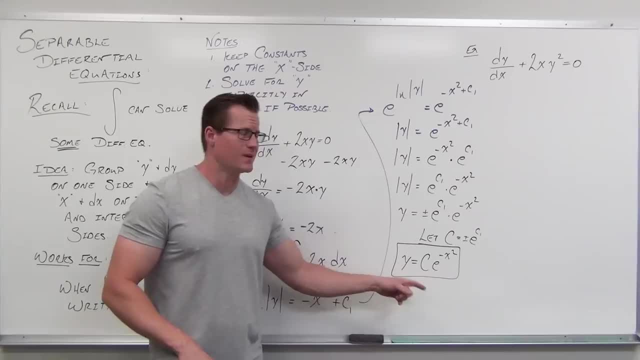 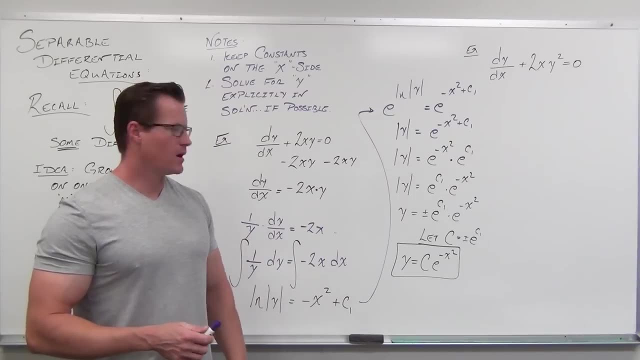 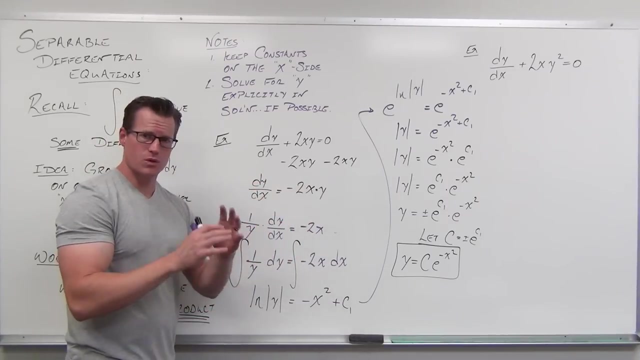 explicitly for y. This is the general solution to that differential equation. That's pretty cool. We had our first technique. The next one's really really similar. I'm not going to show you a lot of the options. Basically, most everybody does it this way: We separate the y dy. the x is dx. 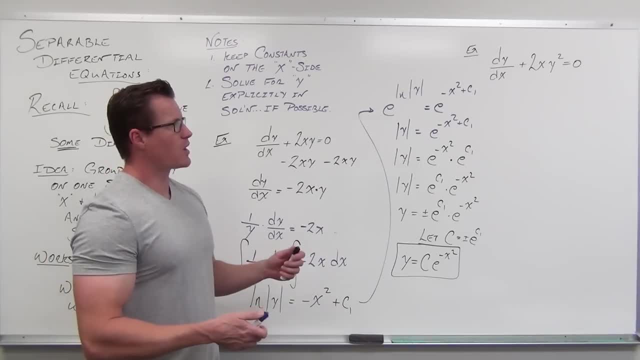 and we integrate. We take that, but that's okay, So let's give it a try. Of course, we need to write this in this form, if we can, in all possible Man. separable equations are really nice. Let's. 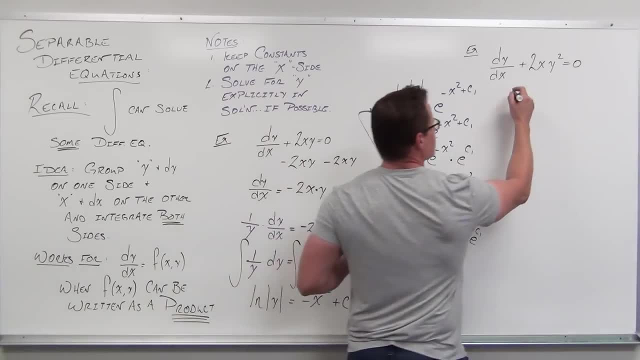 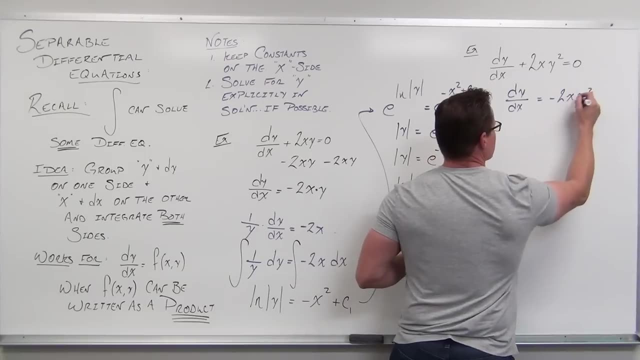 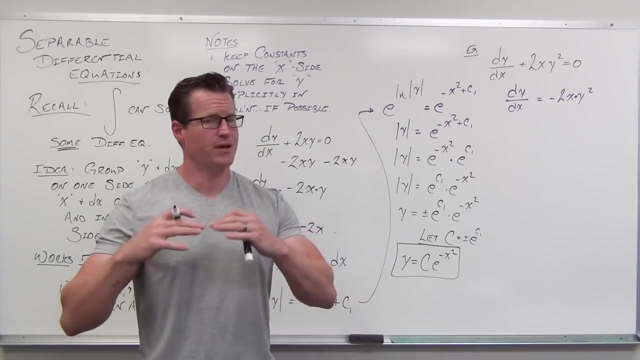 separate our variables out. Let's write this As a product of a function of x and a function of y equal to our derivative, our first derivative, if at all possible, that allows us to move things, these factors, by multiplication, division. So 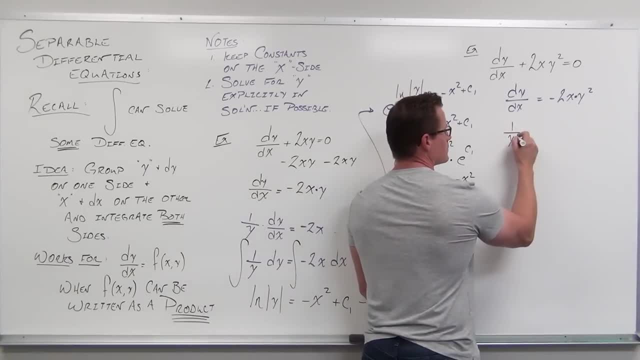 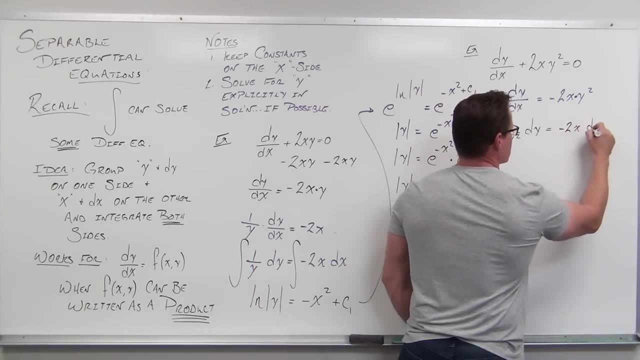 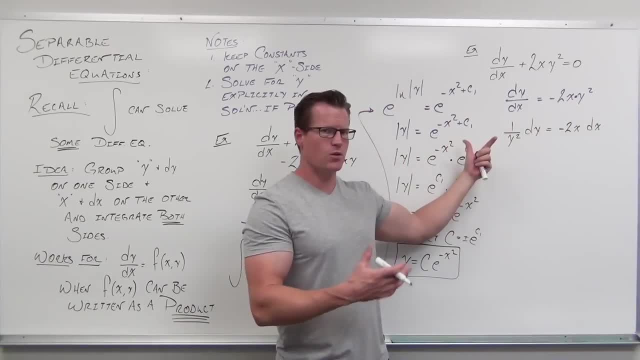 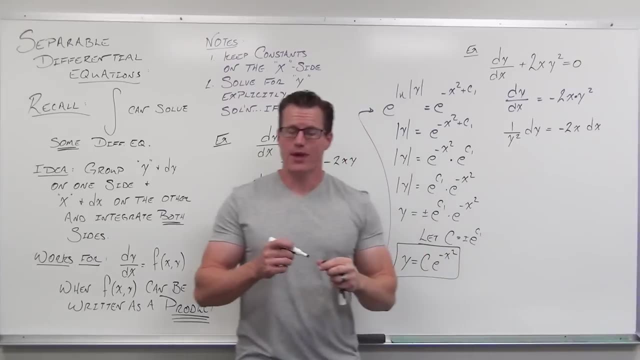 understand that, yeah, you're dividing both sides of a y squared, It's going to give you 1 over y squared and a dy. We're keeping our constants and our x's on one side and multiplying by dx. Then that allows us to take an integral on both sides, which is a really cool idea. 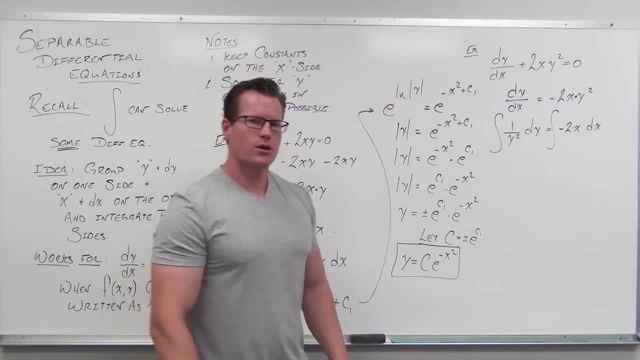 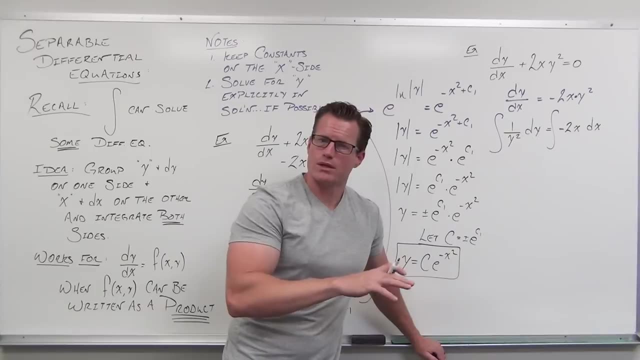 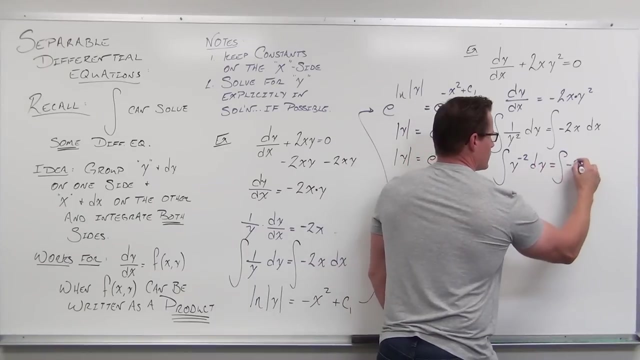 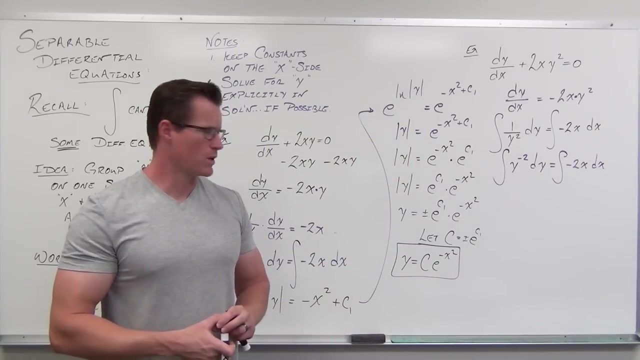 And look at the difference. Look what that y squared does for us. Instead of having 1 over y and yielding this ln of absolute value of y- that's not what's happening- We really have an integral of y to the negative 2 power dy. So we have a completely different answer. We're not going. 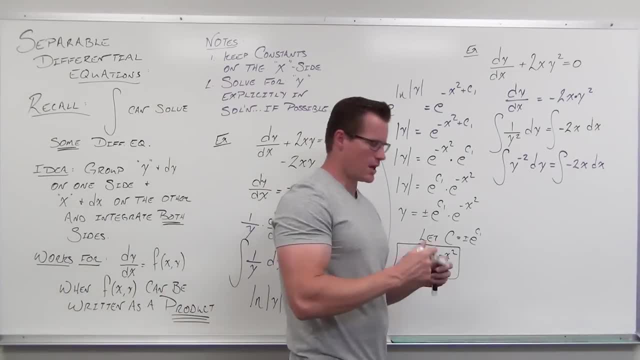 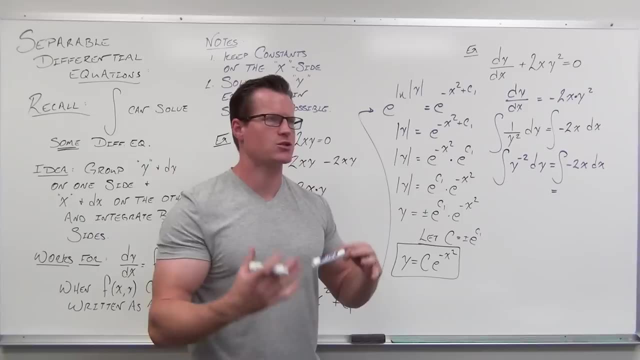 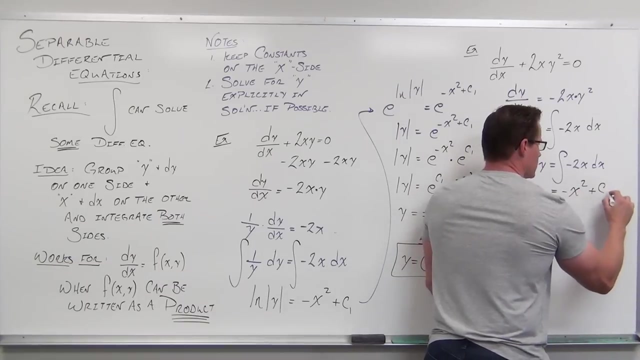 to have an e to anything on this On the right-hand side. sure, we've got the same exact stuff going on. So remember, on the right-hand side, that's where our constants are going to lie, That's where our plus c is going to lie, which is an arbitrary constant. We're going to have this negative x. 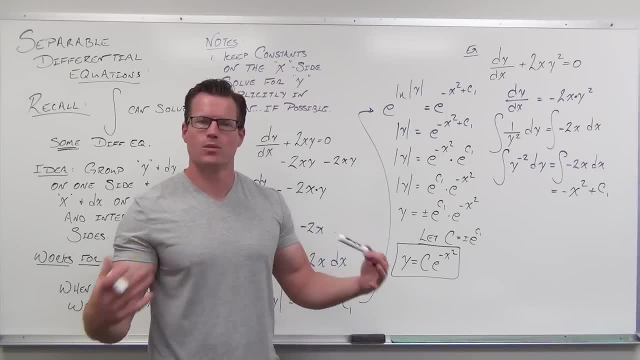 squared plus c squared. So we're going to have this negative x squared plus c squared. So we're going to have this negative x squared plus c squared. So we're going to have this negative x squared. So we I'm going to write the plus c1, just in case I multiply by any other number. this in case I take: 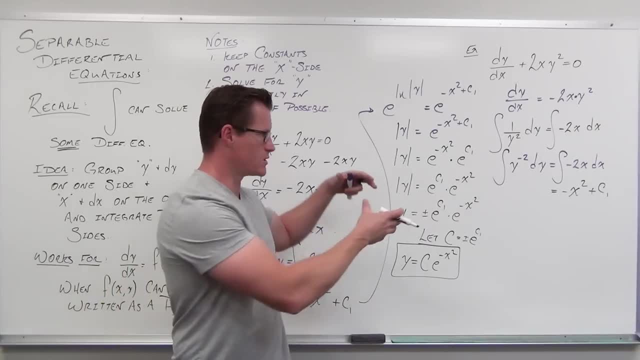 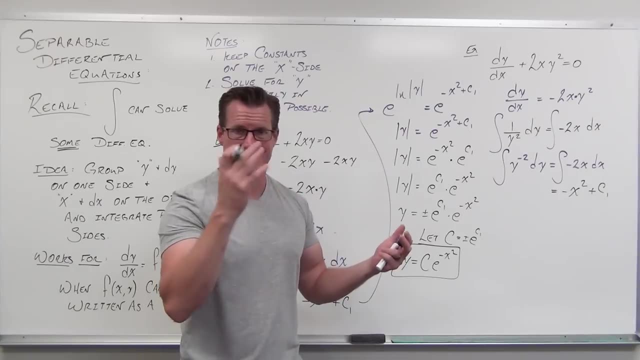 it to an exponent. This can be a little bit more easy for us to show that we're changing that to another constant. If we don't have to change it, we're just going to erase the plus 1 and call it the arbitrary constant. On the left-hand side we've got y to the negative 2.. So do you remember? 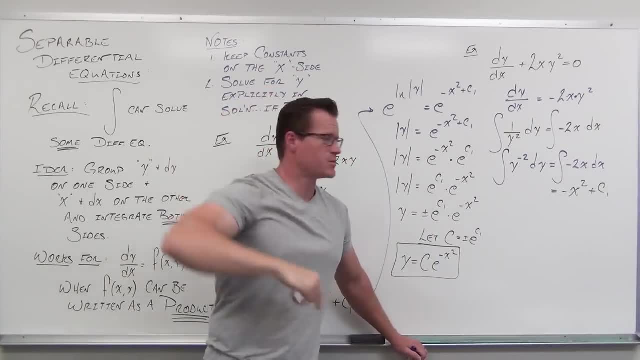 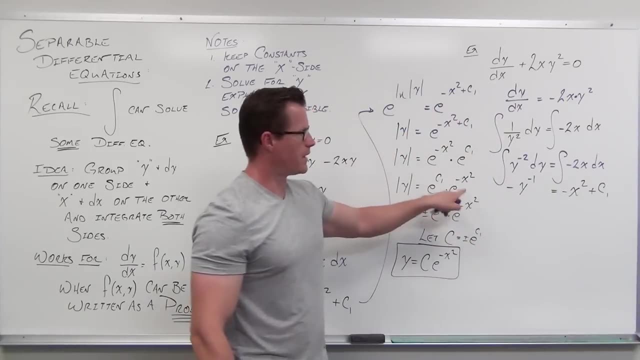 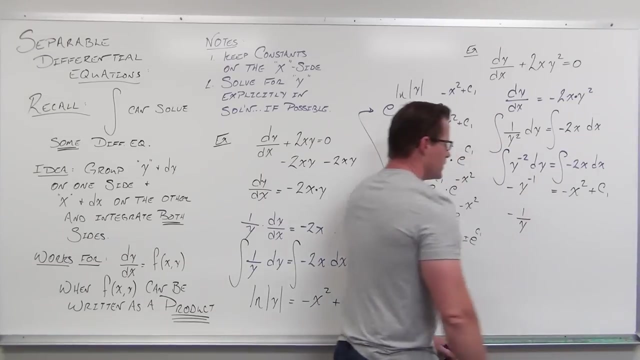 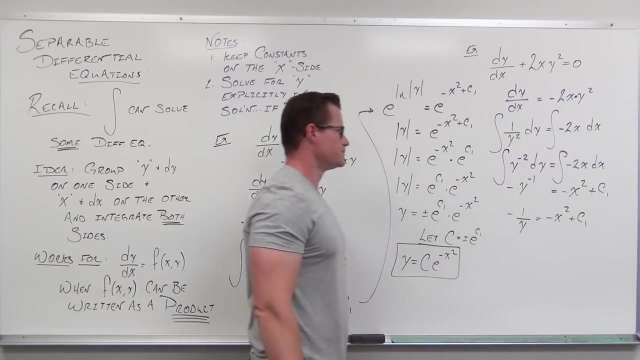 those We add 1 to the exponent, divide by the new exponent. So add 1, divide which gives us a negative y to the negative 1.. Or we can think of this as negative 1 over y. Let's multiply by negative. 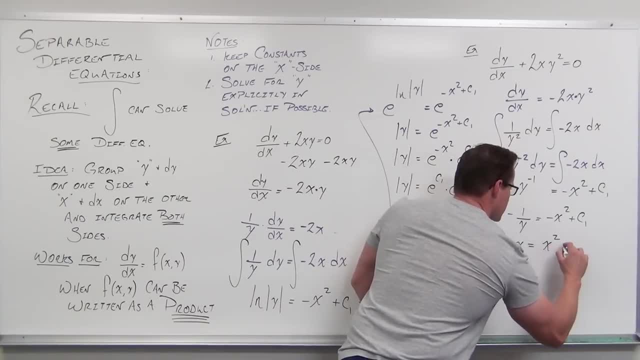 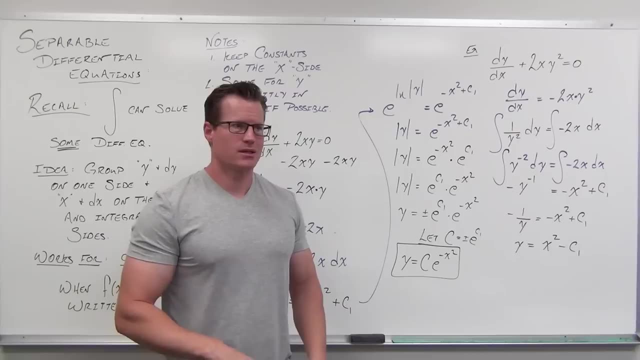 That gives us this: positive y equals positive x squared minus c1.. So, right now, if you did this problem on your own and you checked- I don't know if this came out of a book or not, but if you checked in the back of your book- 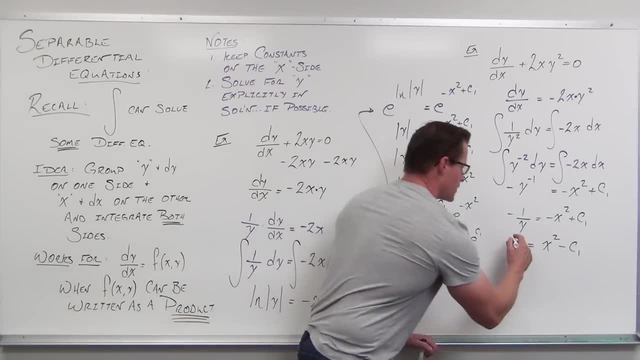 and you said: well, they have x squared. well, I'm sorry, I'm making a mistake. I was thinking about the next thing. I was saying 1 over y. They've got x squared plus c. You know what? 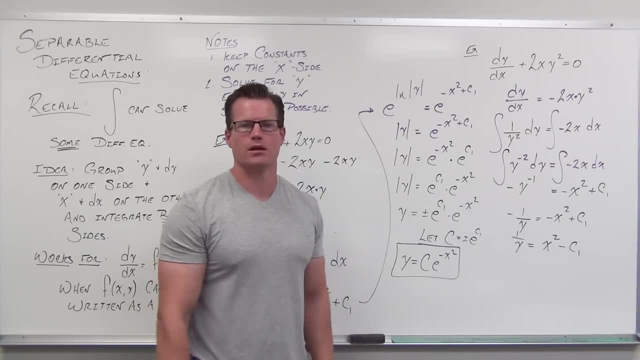 Maybe they defined c as equal to negative c1. And that would change that sign. If it's arbitrary, it doesn't matter, So that's not a big sticking point. The point is that can you get down to 1 over y equals x squared minus c1,. 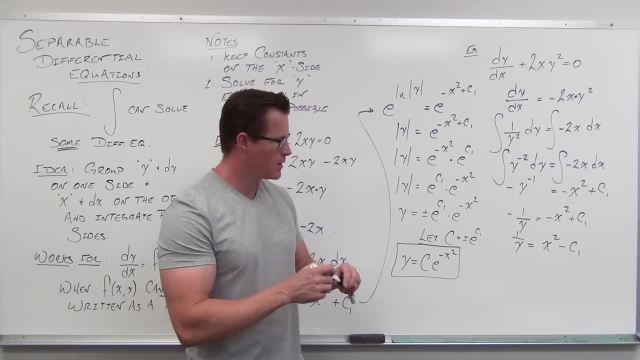 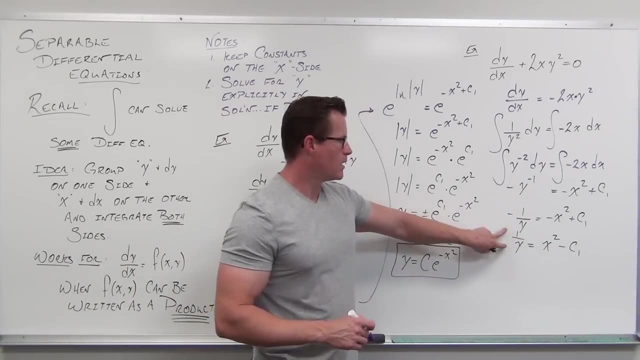 or plus c, a different constant, It's the same thing. Well, that's great if you can. Now we're almost done. If we have 1 over y equals x squared minus c1, then y equals the reciprocal of that. 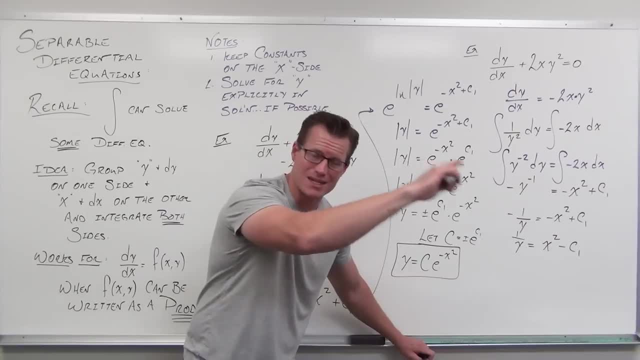 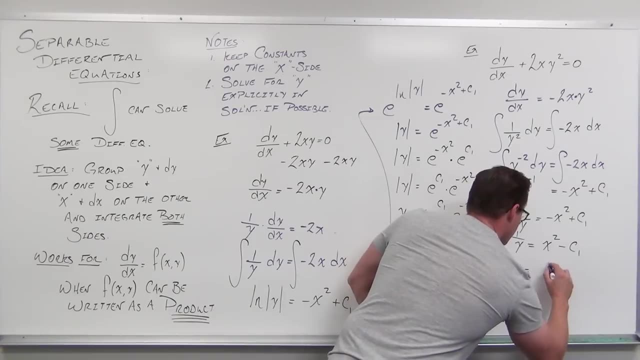 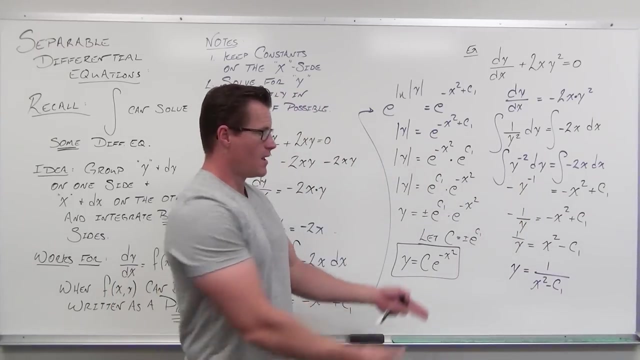 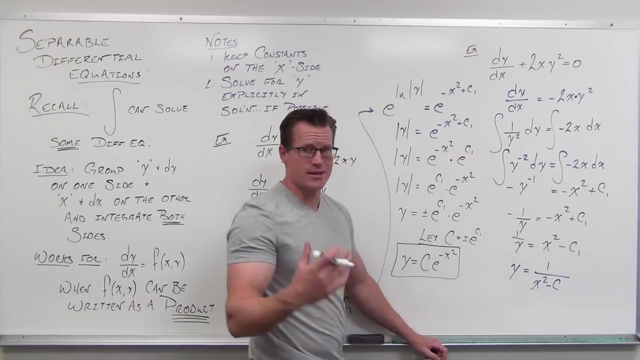 So you can think of it as multiplying both sides by y and dividing by x squared minus c1, taking reciprocal And, as I was saying just before that, right there, that is a solution, That's a general solution. We can either erase the c1 and just take this as y equals 1 over x squared minus c. 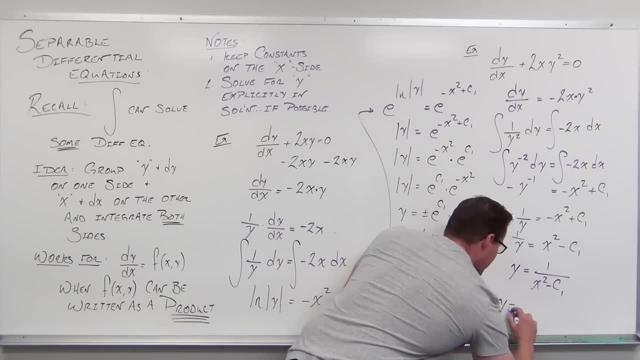 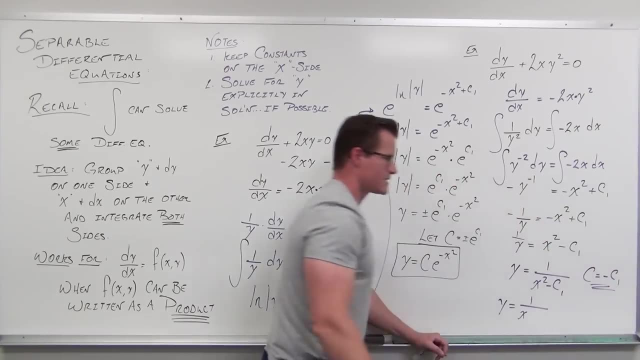 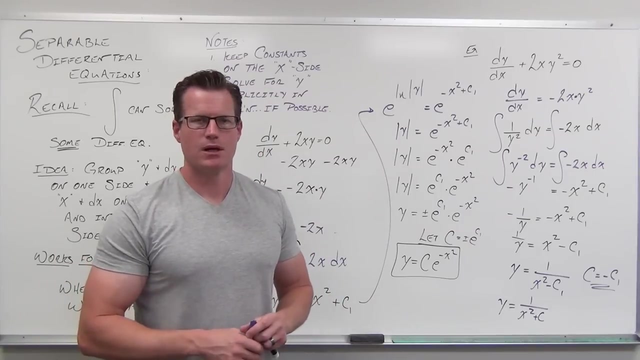 or if you want to keep the c1, you can redefine it. Let c equal negative c1. Then you could write this as x squared plus c. Is it a big deal? No, it's not even a big deal, Not to me at least. 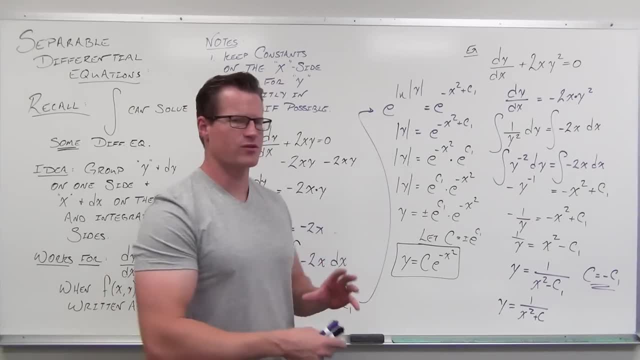 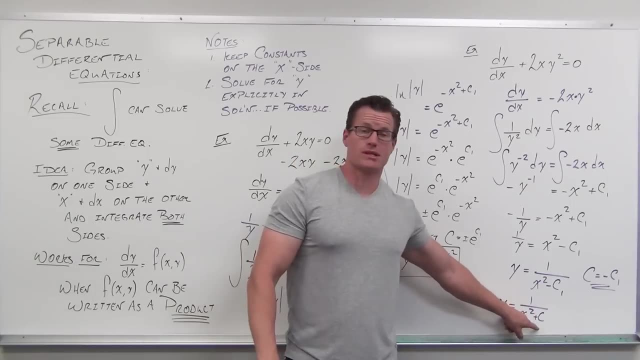 It's still the function that has an arbitrary constant in it. It's in the correct form, We've solved it explicitly And this function is a general solution. Why general? Well, it has a plus c in it still. So this is a family of curves, an infinite number of functions. 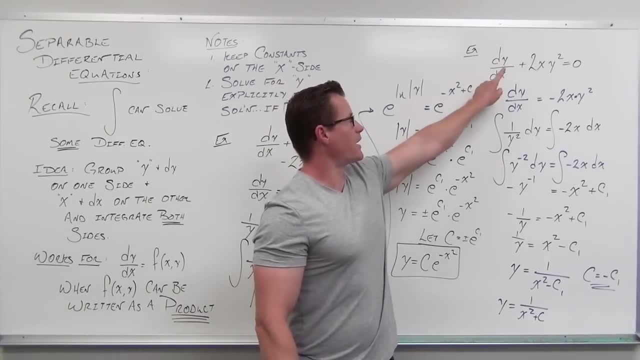 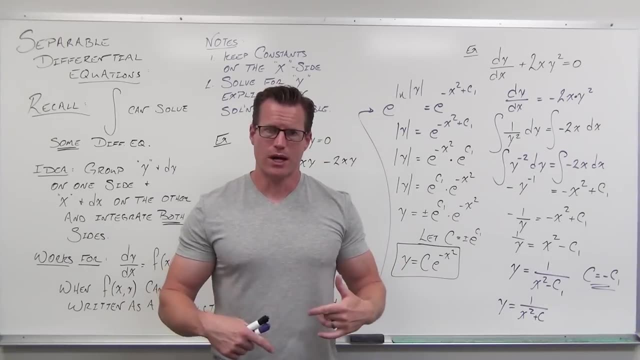 that when you take a derivative, a first derivative of it, it will satisfy our differential equation with that other stuff in it, which is really awesome. It's pretty cool that we can do that now From scratch. If you wanted to look back at the first few videos: 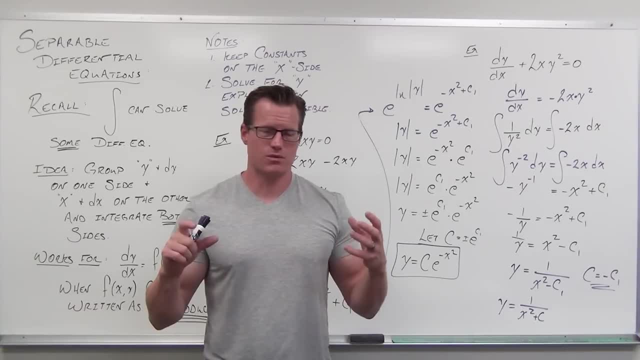 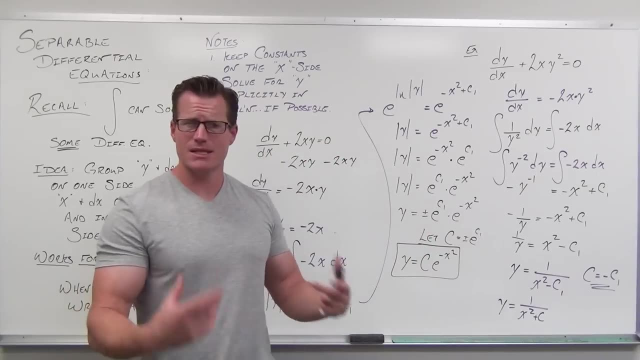 there were some problems that we could have solved this way. There were some basic problems that we could have solved with separable equations. So we're going to do a whole lot more. If this is making sense to you right now, like I really get this, try some. 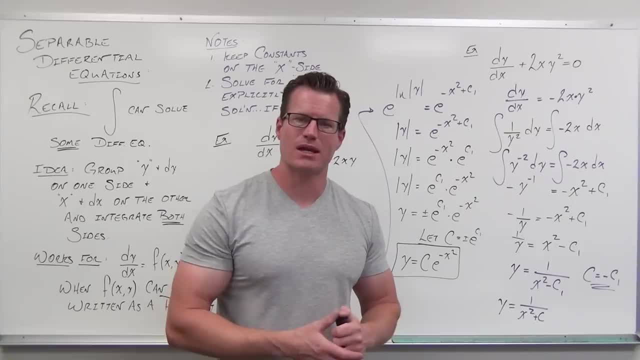 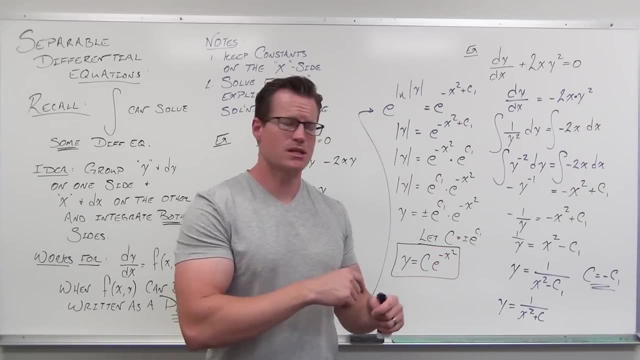 And if you're not familiar on some of the integration techniques, then check back into the video Again. though, skip to the last problem, where we talk about singular solutions. So I'm going to erase this. I'm going to come back in just a minute. 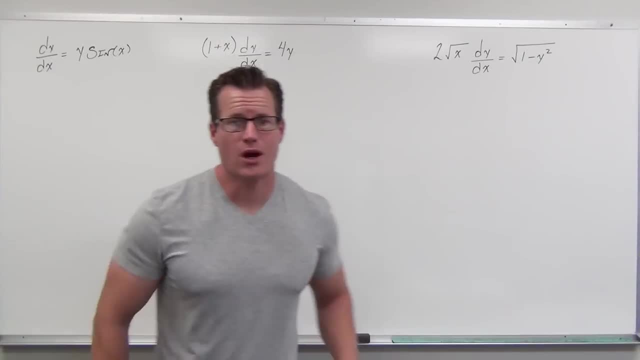 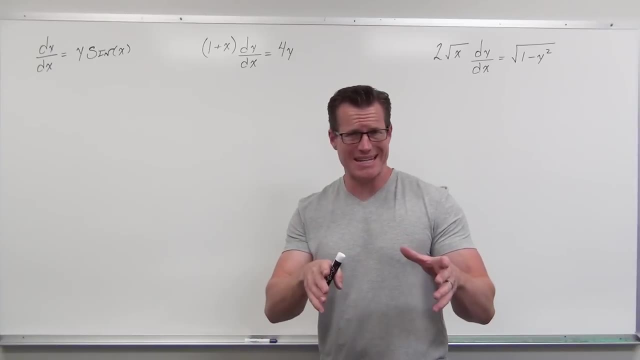 Let's get some more examples. Let's give these a try. First one: remember what we're trying to do with separable equations here, separable differential equations. We're trying to see if the function fits the model of. could you write it? 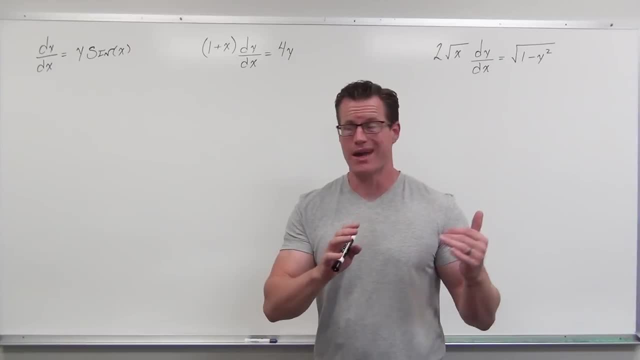 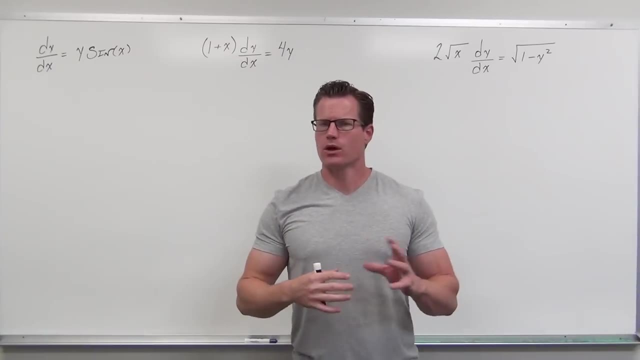 as a dy. dx equals a function of x times a function of y. Sometimes they're written like that. That is great. Sometimes they're not. But if you divided this you could write it. So we're going to get to that where we're thinking that. 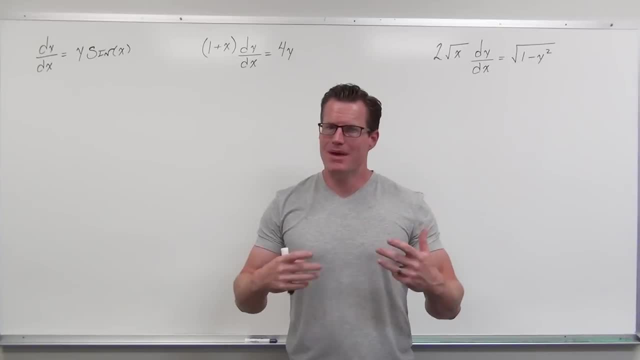 but we're not actually doing it. We're actually showing that in particular steps. So the main idea is: can you get your? y is dy, x is dx. That's the main idea, Whether you go through the actual process of writing dy. dx equals a function of x times a function of y. 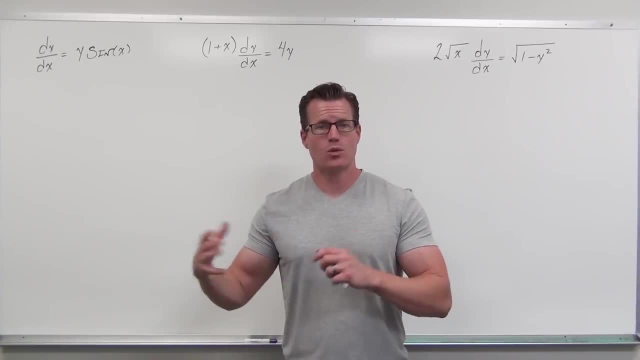 And now I'm going to move the y. It doesn't really matter. The idea is: can you write it like that? If you can, great, do it. That's your first goal. First goal in differential equations is if you can get it that way. 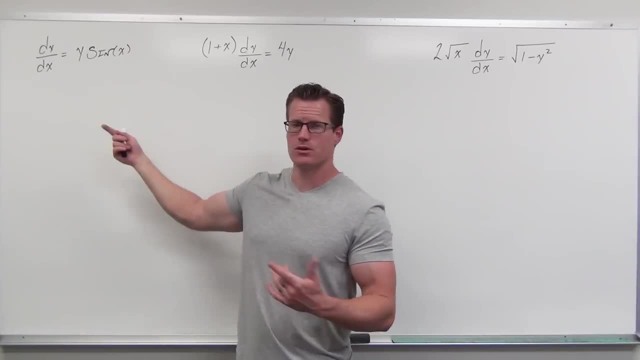 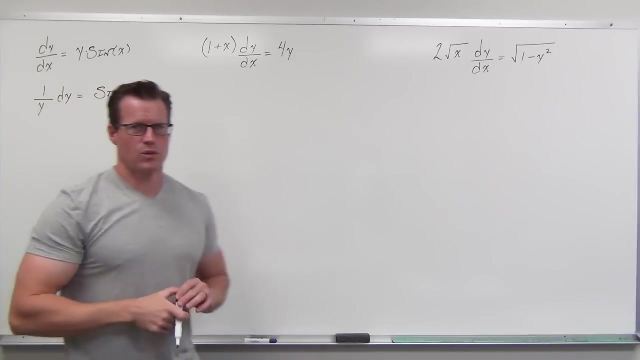 Here we can. We've got dy. dx equals a function of y times a function of x. That's perfect, Because we know that we can divide and get. the y is on one side, dy, x is on the other side. dx. You're going to get really used to the whole 1 over y thing. 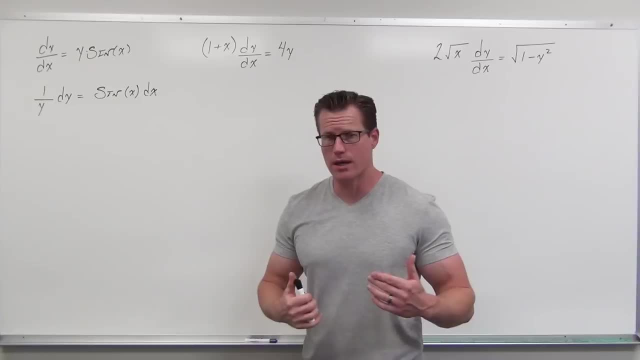 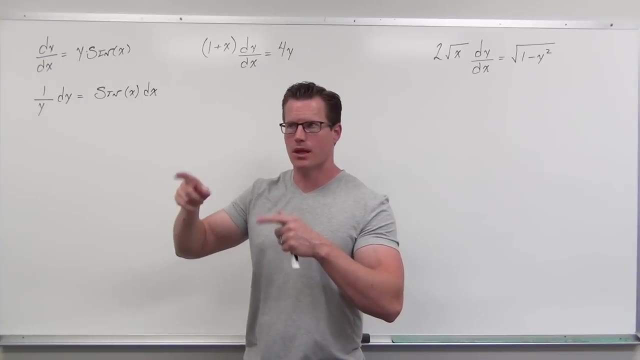 1 over y, dy happens a lot. You're going to get a lot of ln, absolute value y's. You're going to get a lot of e to this side, Whatever that integral is, And then we're going to get a lot of that plus or minus e to the c1 equals that c. 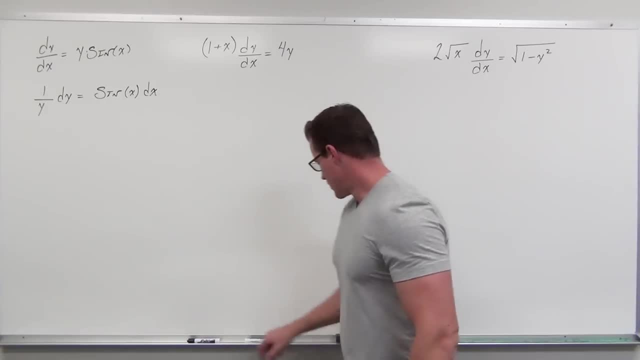 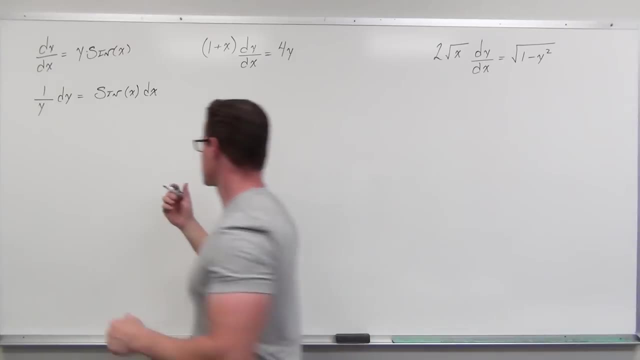 It happens quite a bit with some basic differential equations. So we've got this down. We say, all right, we grouped our y dy, We have our function of x, dx. Let's integrate both sides. That's great. On the left-hand side, we know that integral. 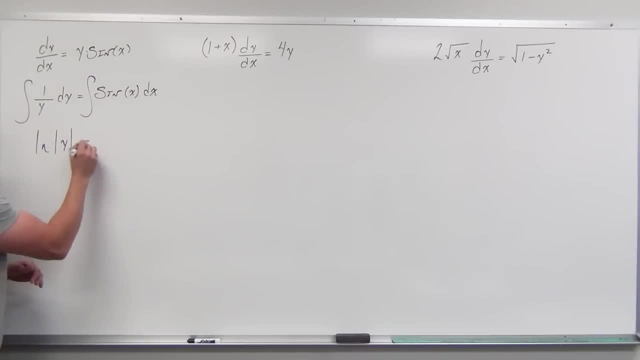 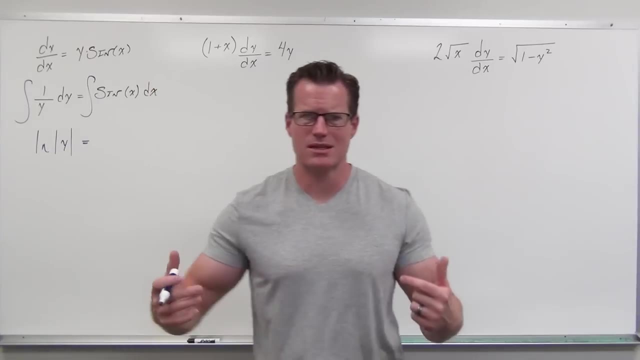 This is ln absolute value of y. It looks pretty good. We know what that was. We had an example like that before. Integral of sine x. Let's remember what that is. Remember. most of this lesson is just repeating some integration techniques. 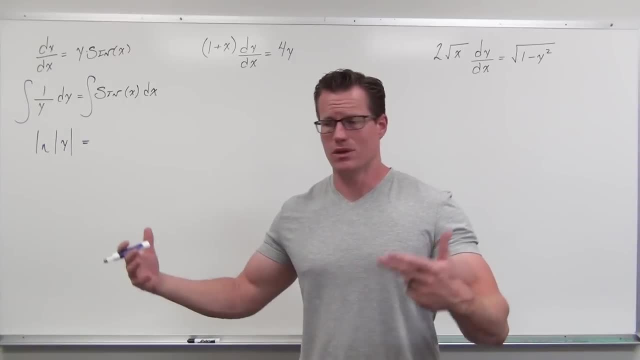 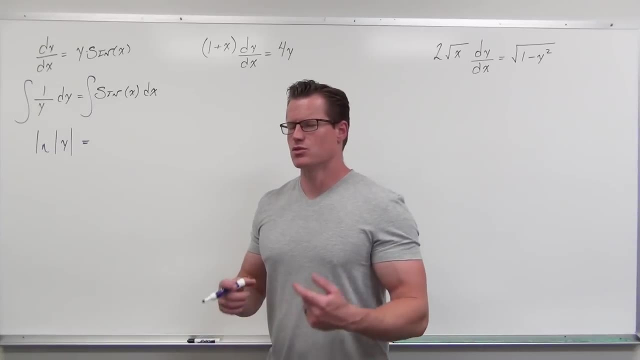 and just getting that back in your head, Because if you can't do this then it doesn't matter that you understand separation of or separable equations here. So on the right-hand side let's see: the derivative of cosine is negative sine. 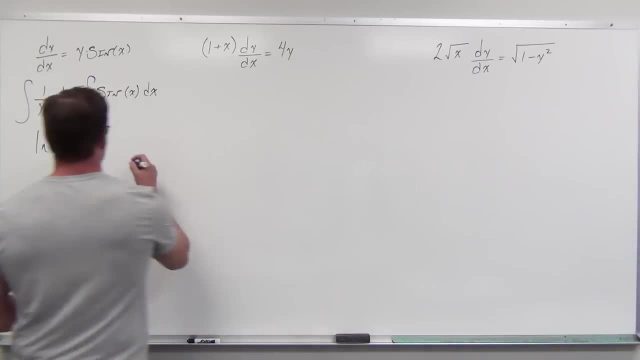 So the integral of sine is negative cosine x, And I might want to just take a moment to think that through The derivative of cosine gives us negative sine. So the derivative of cosine times negative 1 gives us positive sine x, And that's pretty good. 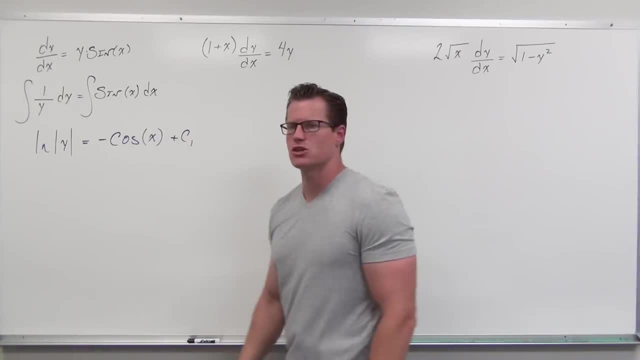 I'm going to add my plus c. I'm going to give it a little 1 because I expect this thing to be changing a little bit later. So I've grouped them. I've integrated both sides. Easy integral. Had to think about this one a little bit. 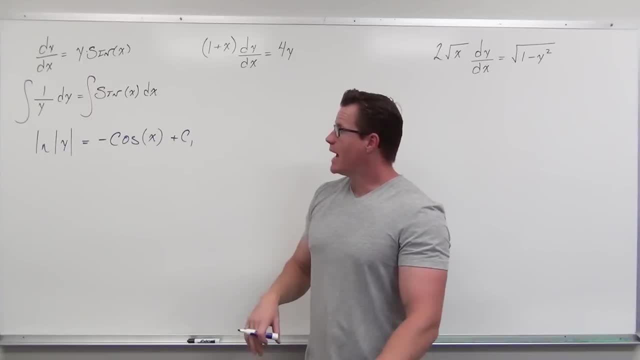 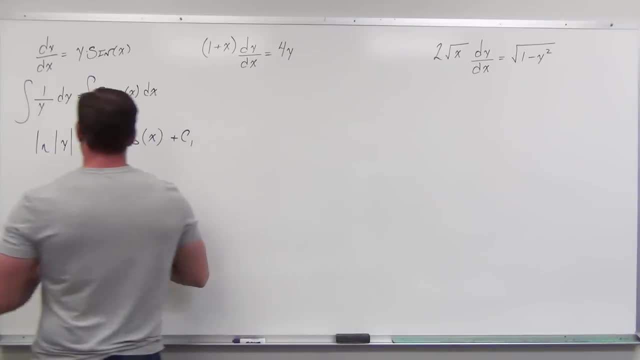 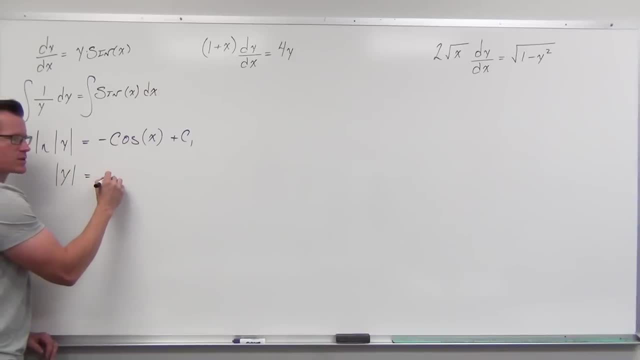 That means y at least. the absolute value of y equals e to the negative cosine of x plus c1. And we go through this process a lot. We know the absolute value of y is going to equal If we separate this. I'm going to move my factors. 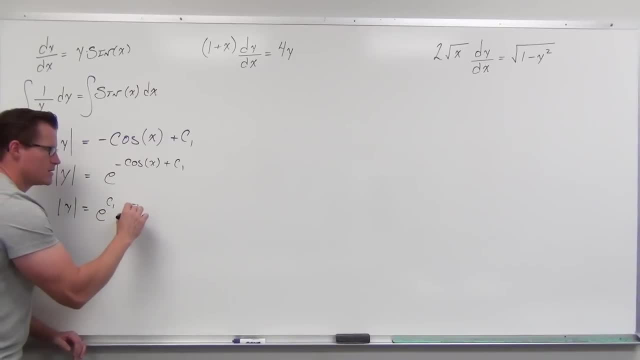 This is e to the c support. This is e to the c sub 1 times e to the negative cosine x. We know that any time exponents are added together they came from a product of common basis. I just moved the e to the c sub 1 first. 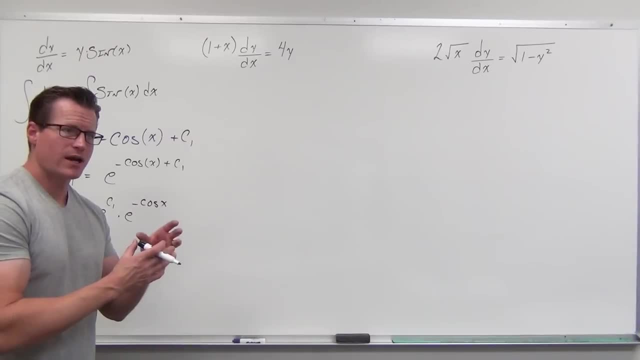 We also just explored what absolute value is. Absolute value takes a positive when the expression is positive and a negative when the expression is negative, which means we can write: y equals positive or negative. Now, the fact that that's never going to be negative because we have this e to some power. 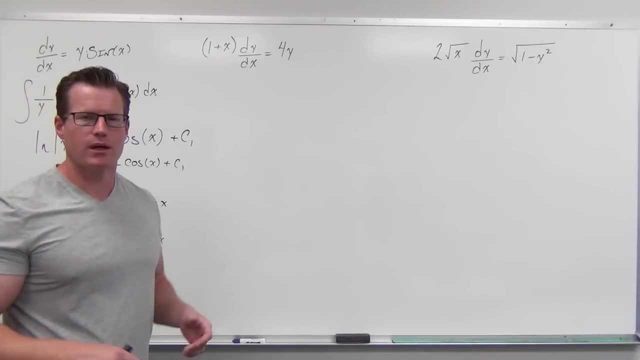 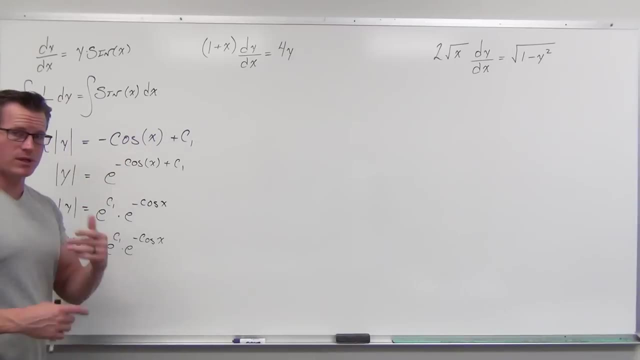 this might be a little redundant On some cases. we can do it anyway. It doesn't really matter as far as the long run, but sometimes e to anything is not going to give you this negative, So that we're going to redefine. 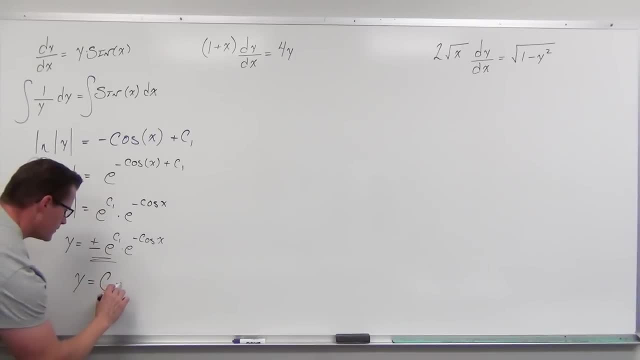 We're going to call that c. So sometimes we show this off to the side and we say: let's let this. I would show that if I were you, but sometimes that's not shown. So if you're wondering where that garbage goes, 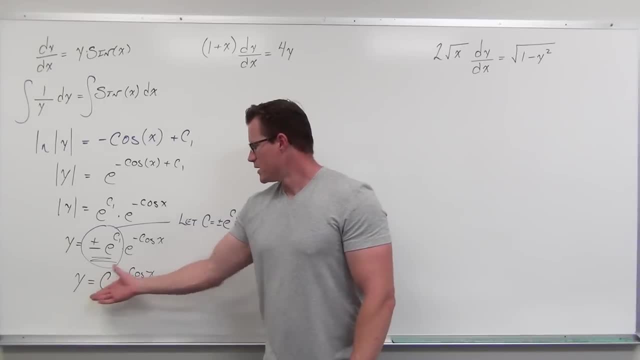 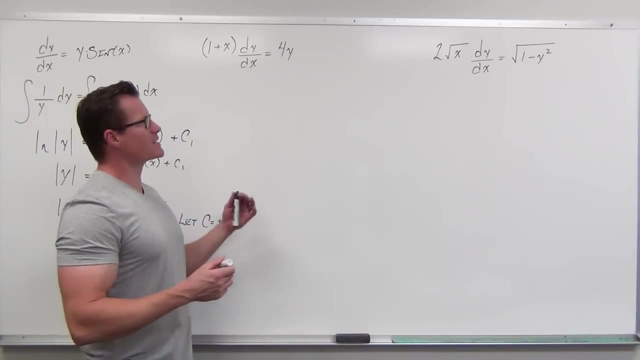 they're wrapping this whole thing up and calling it the arbitrary constant. So that's our solution, That's the general solution of that differential equation, which is pretty nice. Let's try the next one. So the next one doesn't really look like like what we had. 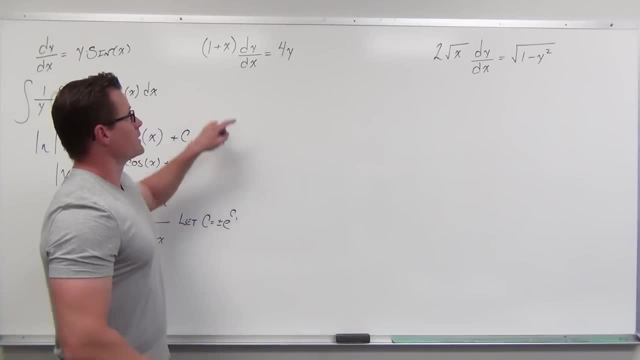 It doesn't look like what we had before either, where it was added. But can you imagine, if I divide this over here, you would get 4y over 1 plus x. Well, since division can be defined as multiplication and multiplication is division, 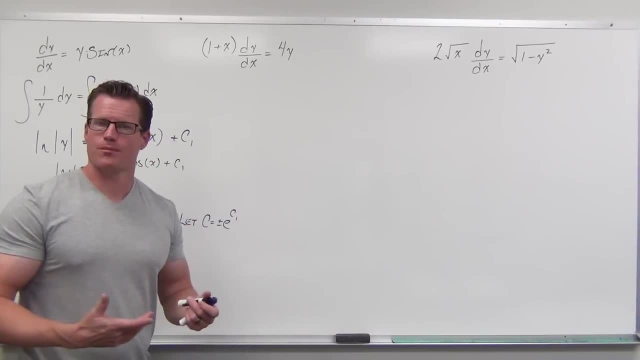 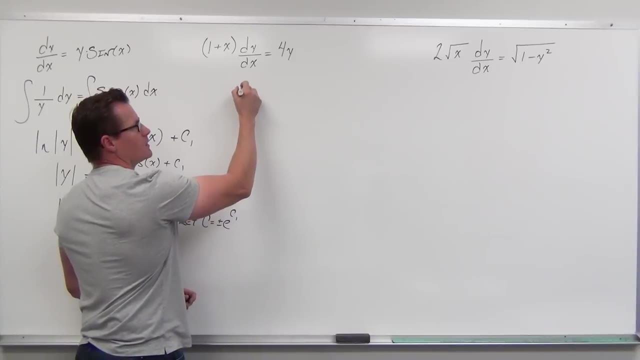 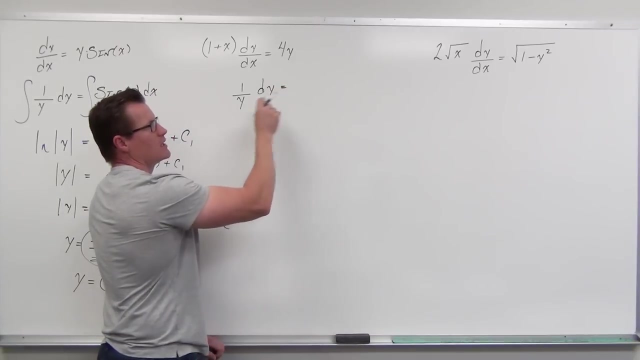 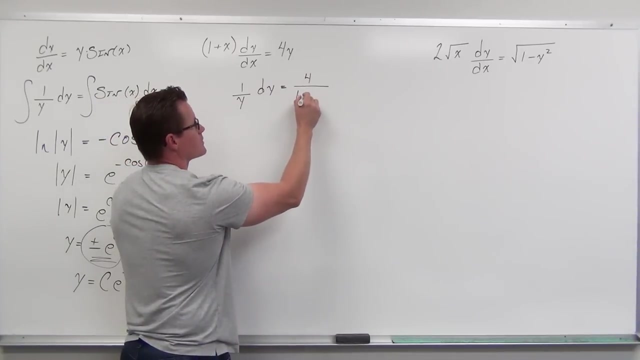 they're the same level of operation. This acts like that form. All we're really concerned about is: can you get your y on one side by dividing by y? Can you get your x's on the other side with your coefficients that are constant factors? 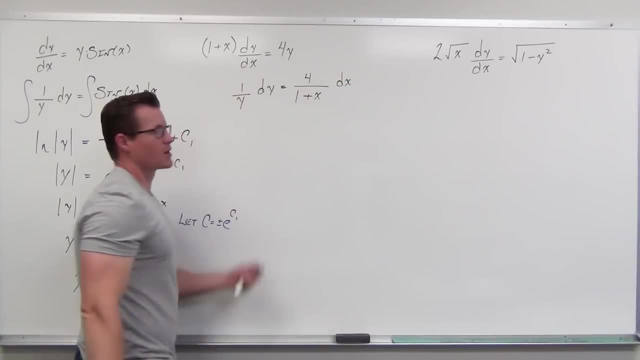 by dividing by 1 over x with your dx, by multiplying by dx. Can you do that? Because if you can, then you can integrate both sides. If you can't, then there will be another technique for us. So we divide by y. 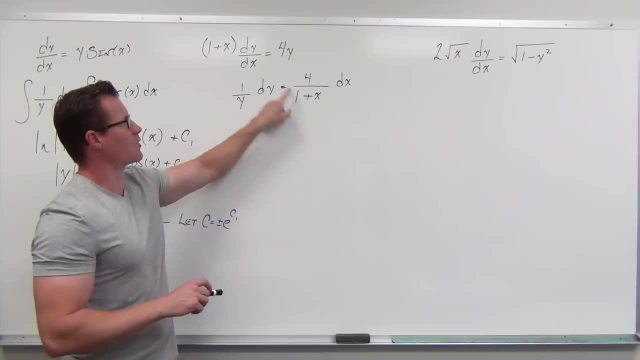 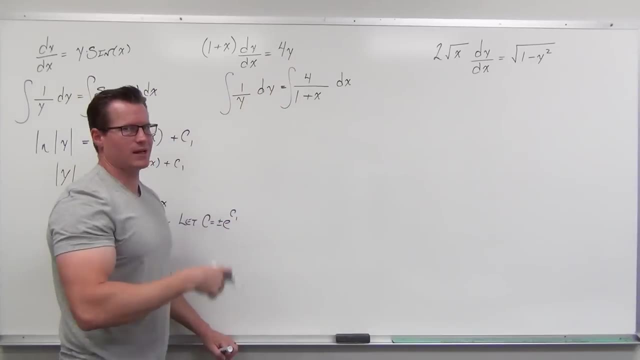 Keep the dy, Divide by 1 plus x. Keep the 4. Multiply by dx And now we're looking great for integrals. So, left-hand side, again, you're going to get really familiar with this ln absolute value of y. On the right-hand side. 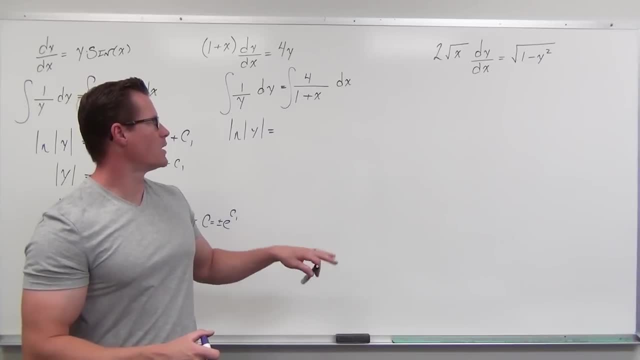 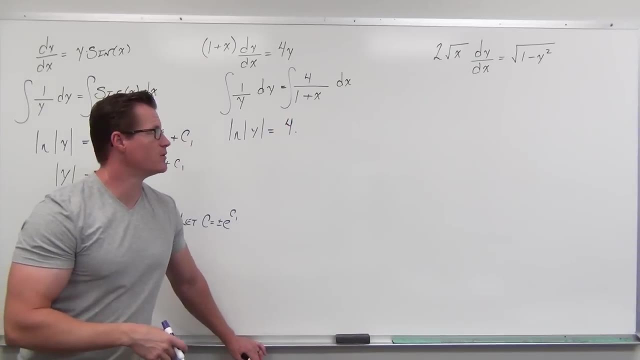 well, we have 4 over 1 plus x. Now the 4 is a constant, so we could pull that out and multiply by whatever the integral is going to be of 1 over 1 plus x. So do you remember what the integral of 1 over 1 plus x is? 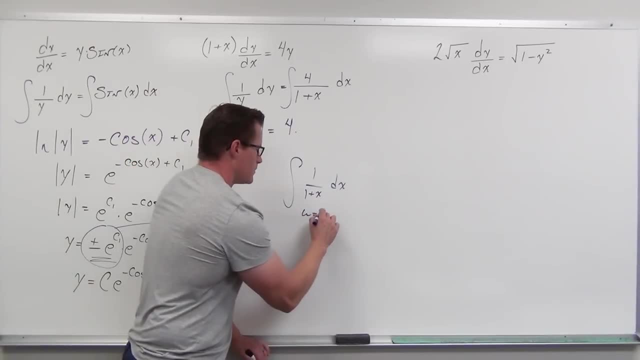 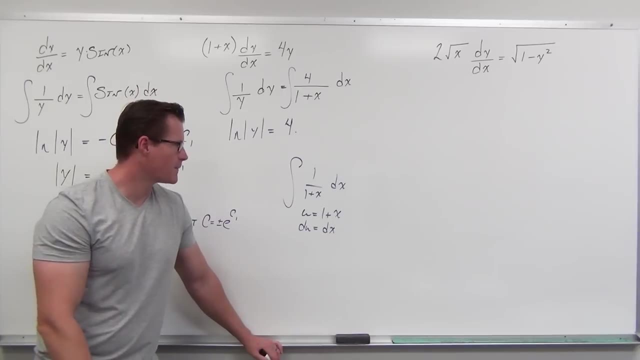 If you need a substitution, you could do that. It's a direct substitution. There's not even a coefficient that comes out of that. So we would have this whole integral of 1 over u du Ah, another ln of absolute value, of whatever that is. 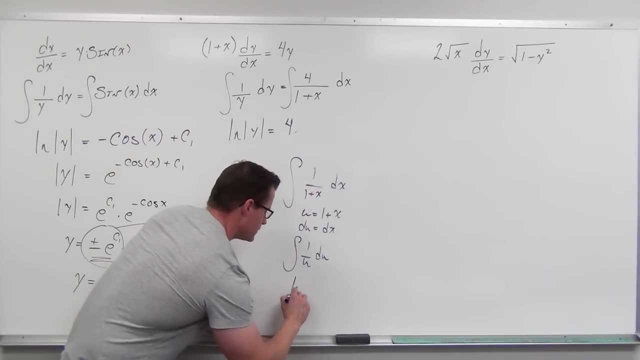 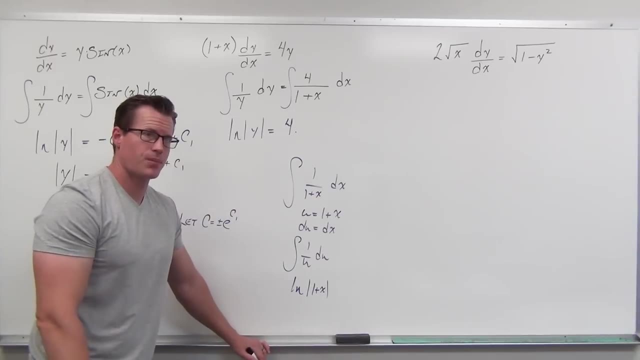 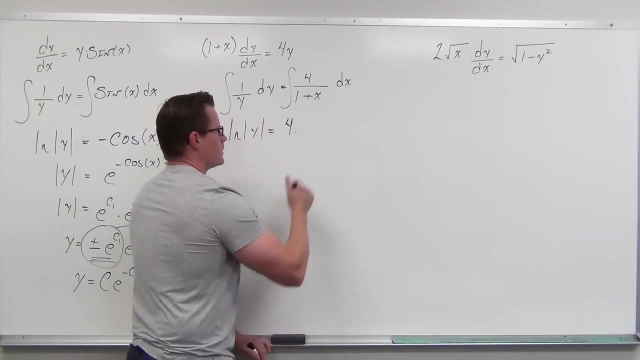 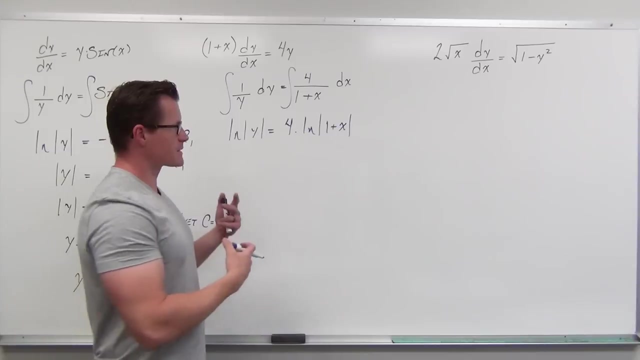 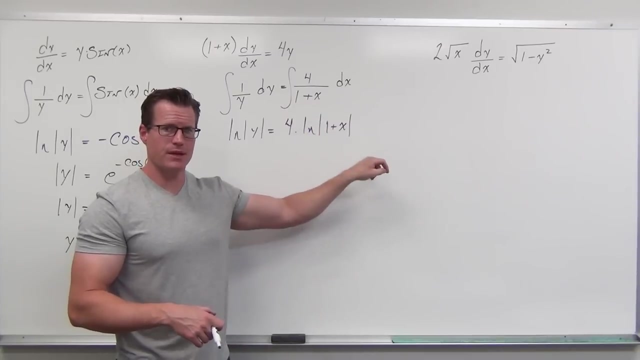 So this whole side over here comes out to ln absolute value of 1 plus x. We can say 1 over x somehow, And if you're not sure, if that's not making sense, go through the derivative. The derivative of natural log would be 1 over inside times, the derivative of the inside. 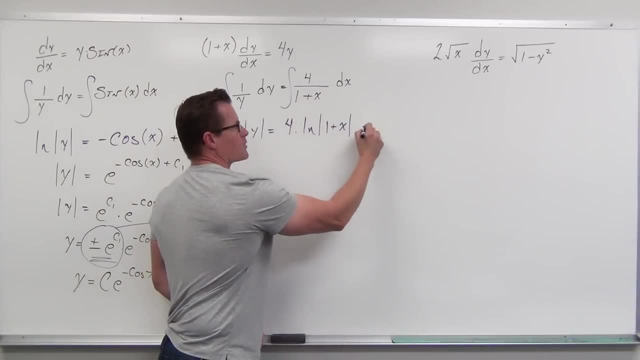 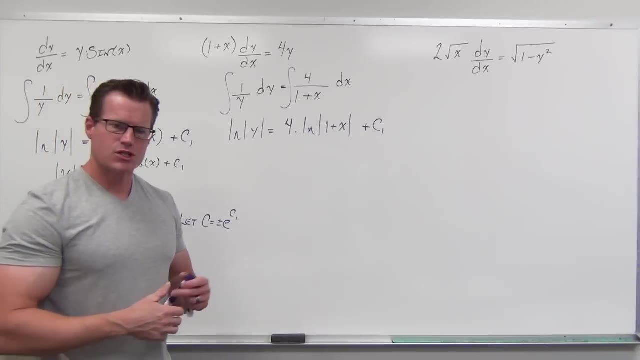 But then we have that 4.. It's the same thing as what we have right there, And we're going to put that plus c1.. So next thing, just so we recall, do you remember that with any coefficient in front of the natural log that acts as an exponent? 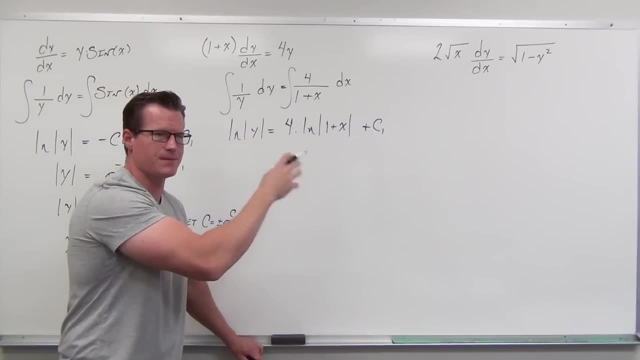 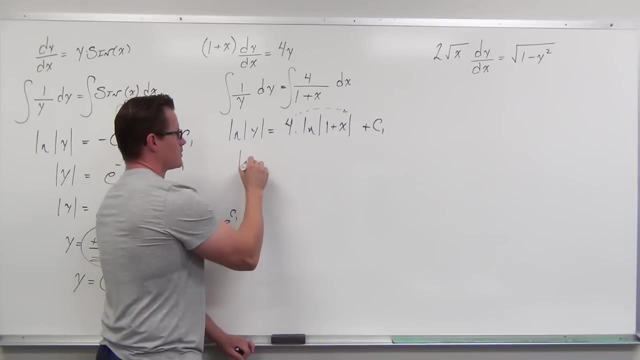 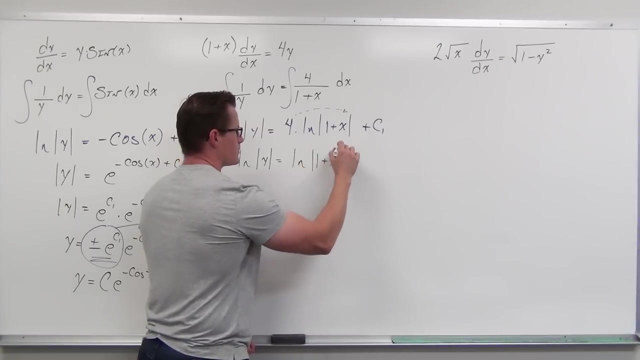 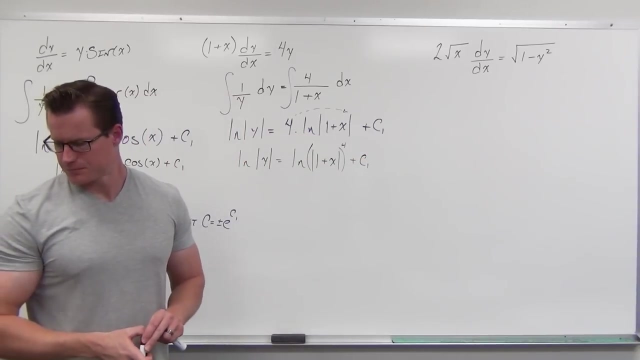 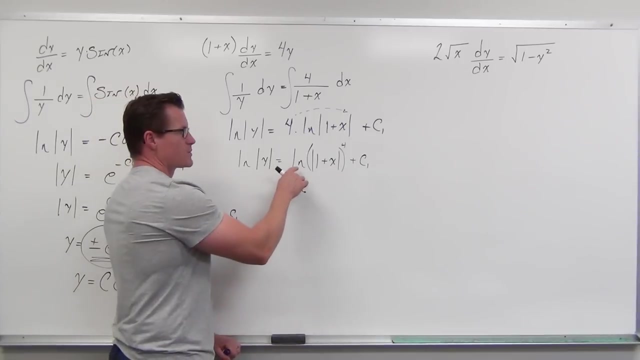 So, before we touch this with any sort of e to that power, we're going to move this and create an exponent. So let's keep on going Now, because we have a natural log of something that cannot possibly be negative. whatever this is, we're going to get that to the positive. 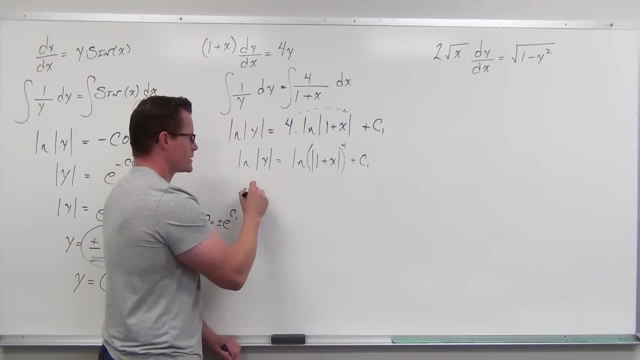 We don't even need that absolute value there, So we're going to take this: e to the left side, e to the right hand side. Show: absolute value: of y equals 1 plus x to the 4th power plus c sub 1.. 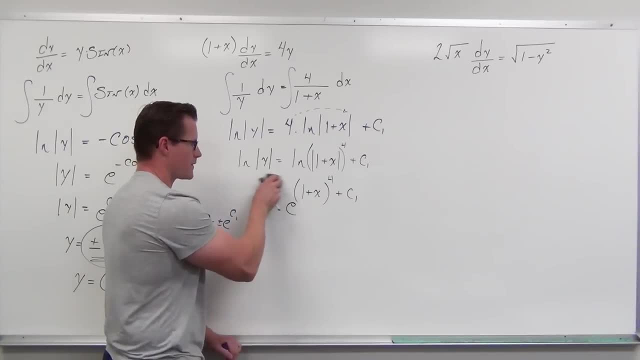 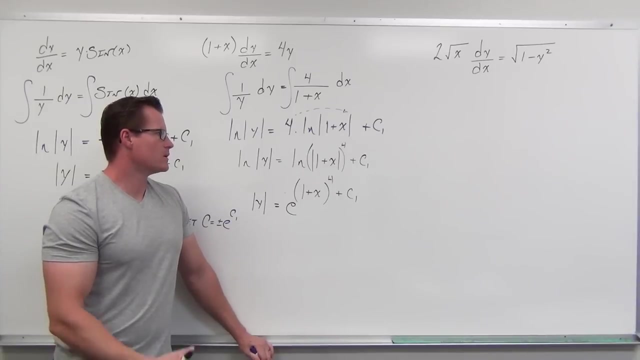 And e is to all that stuff that I wrote, with that little pun in it, to rewrite that. So e to the other side equals our argument of natural logarithm. So that's kind of nice. Now let's do the same exact thing we did before. 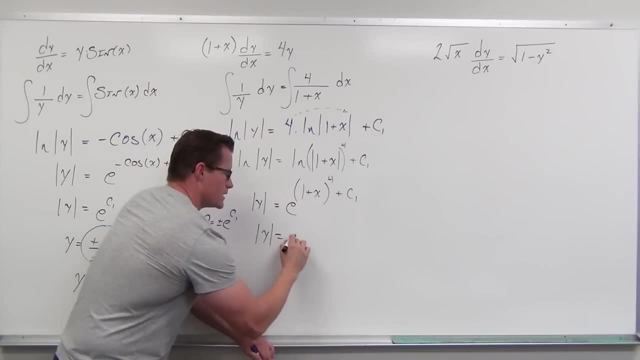 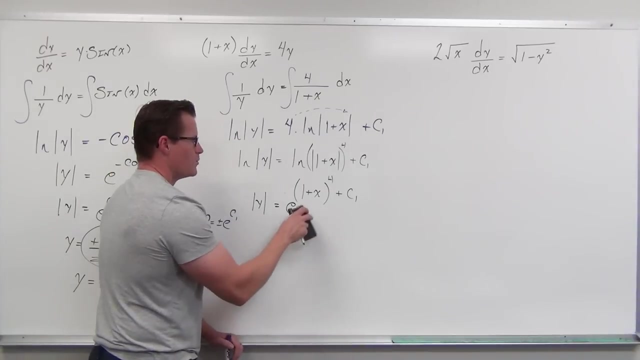 Let's do: absolute value of y equals e to the c, sub 1 times e to the 1, plus x to the 4th power. You know what I made a mistake. I hope you saw the mistake. I kind of went a little too quick here, maybe for my own good. 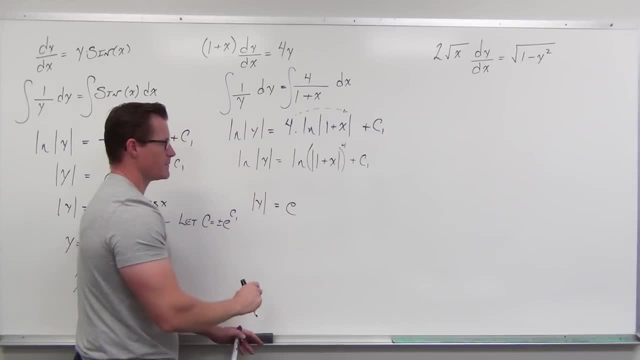 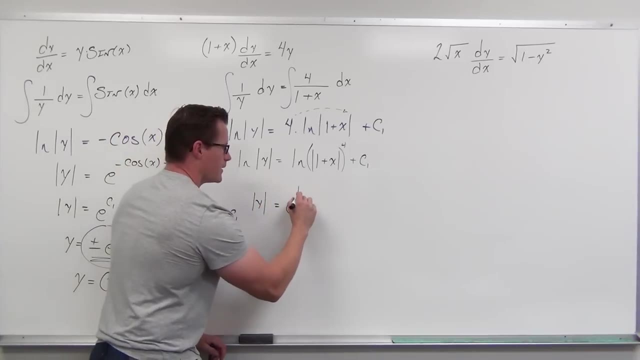 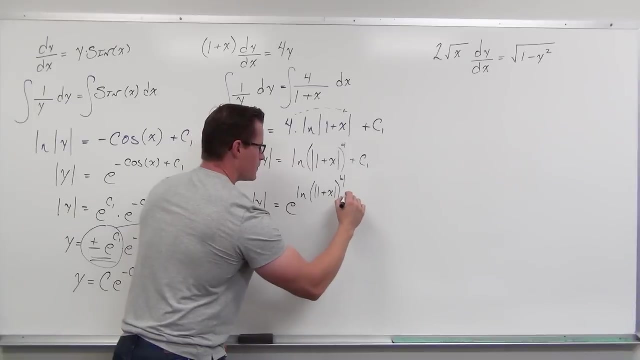 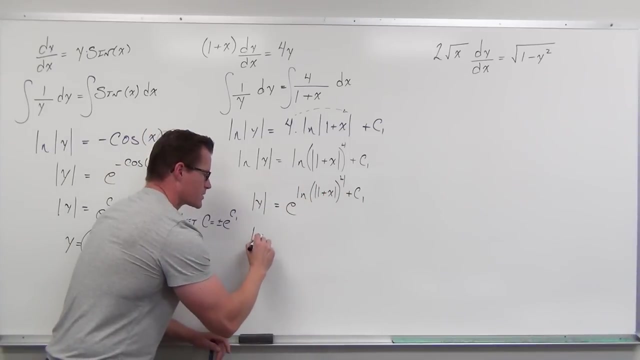 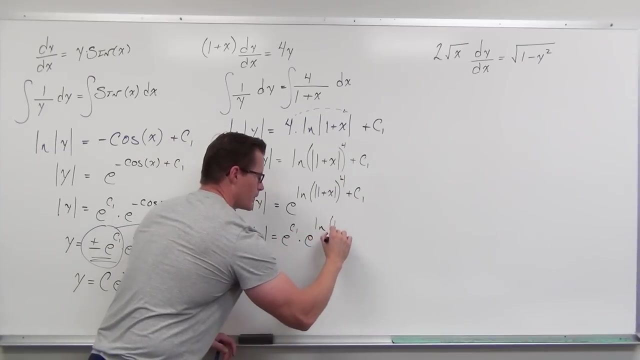 But I forgot something here that I really need to see When we do this whole removing the logarithm by using the exponential. I forgot about the ln. So that's true, but then when we separate this, when we have the absolute value of y equals e to the c, sub 1 times e to the ln, 1 plus x to the 4th power. 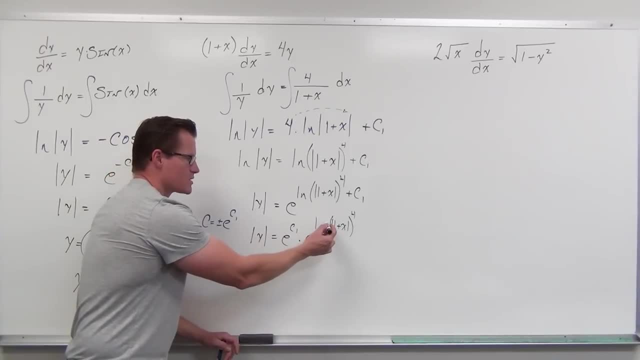 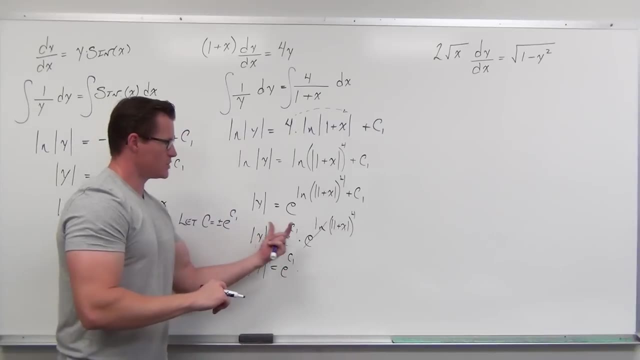 well, now you have a composition of inverse functions. These things are going to be completely gone. So we have the absolute value of y, We have the e to the c sub 1.. But because you had e to the ln of an argument, right there. 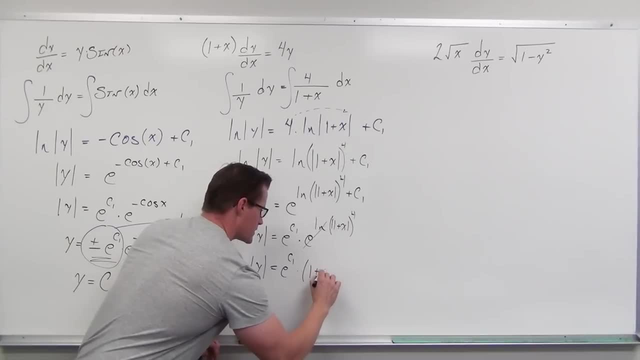 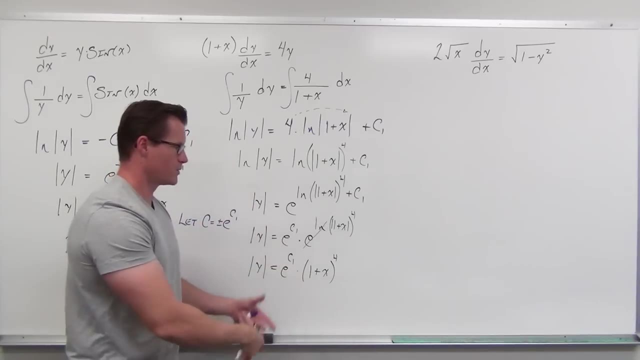 we've got this 1 plus x to the 4th power. That can't be negative. So whatever that absolute value would be, we're taking, the 4th power can't be negative. This plus or minus is going to be wrapped up in the e to the c sub 1.. 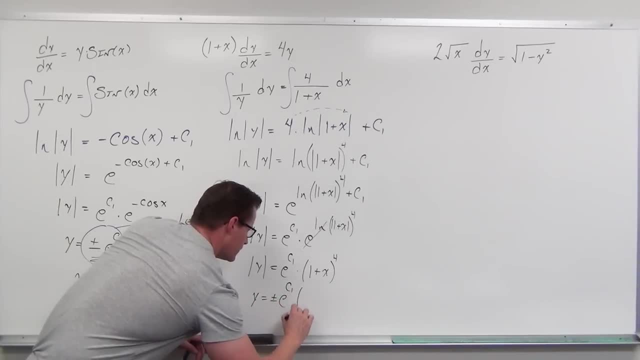 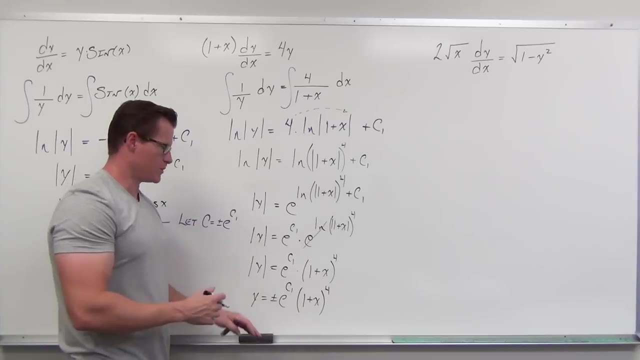 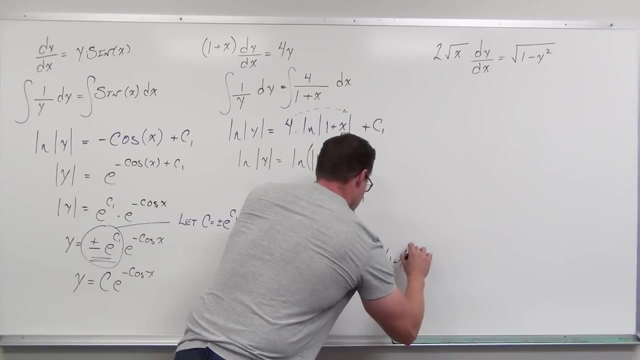 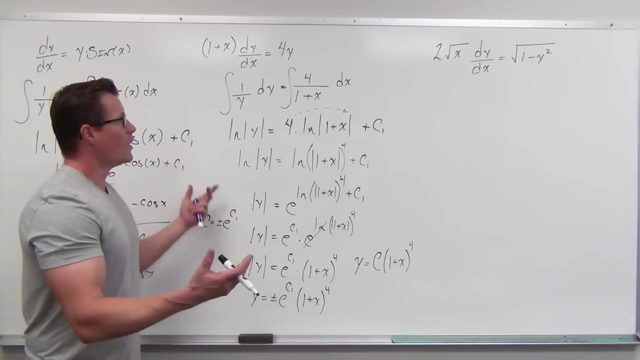 And now we can call that whole argument c. That's our general solution to that differential equation. Sorry about that, I completely forgot the ln. Hopefully you don't do the same mistake. So, walking back through, sometimes they don't look like what we want them to look like. 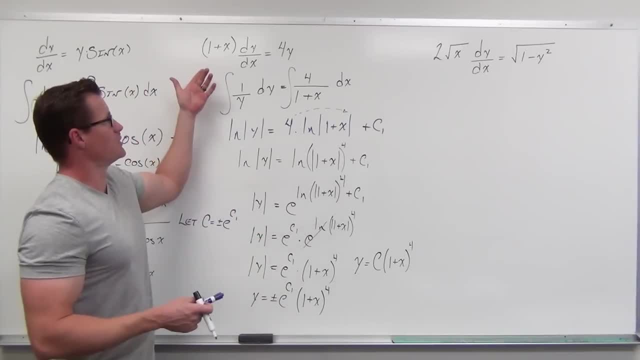 as far as these separable equations go, But we can always see if we can do it. Let's move our x's to one side, keep our constant y's to the other side and then keep our dy, move our dx, integrate. 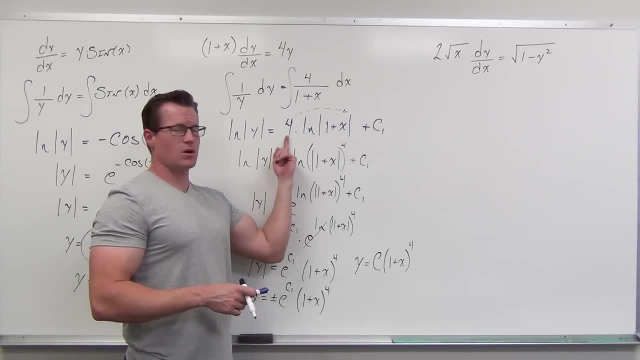 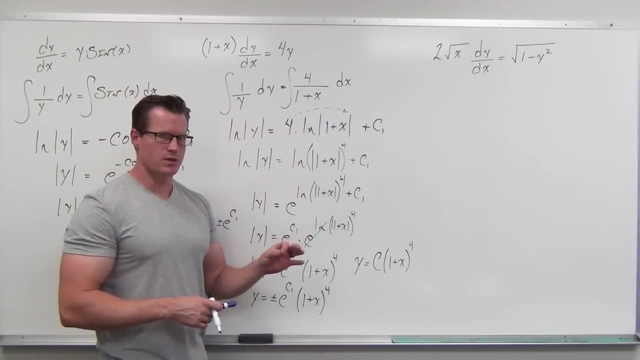 and then start moving these coefficients, if you can, for ln. So we move that up. We recognize that, hey, there's two ln's, They should both disappear when I'm doing an exponential with them. So absolute value of y equals e, to this sure. 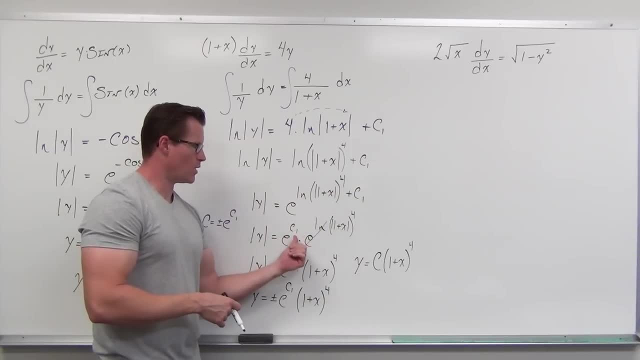 We have a c1.. Let's separate that out: e to the c sub 1 times e to the 3rd power. That's where ln's go away, So this whole thing disappears. We have a composition of inverse functions. We'd have 1 plus x to the 4th power. 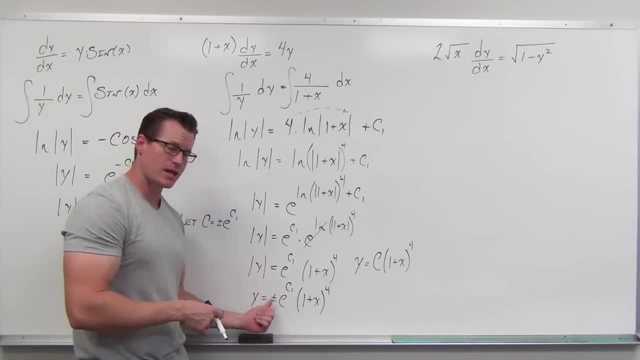 We're going to take away our absolute value by calling that positive or negative, And that becomes our general solution with an arbitrary constant of c. So the next one works very similar. If you haven't done so already, pause the video. See if you can just write it in the right form. 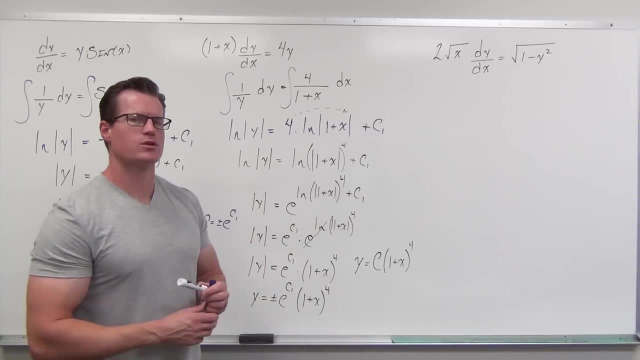 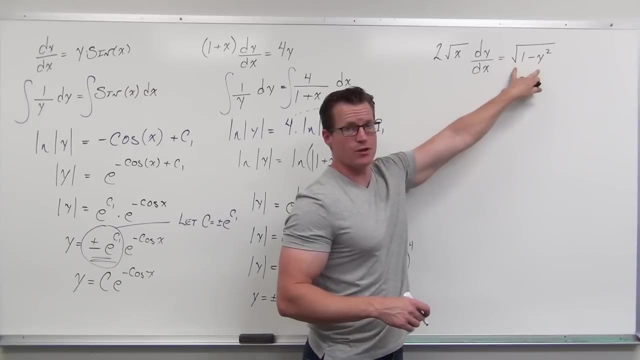 If you get stuck on integration. that's what this video is for is practicing integrals, But see if you can do that. So we have x's here, We got a dy dx. We have y factors over here. We need to move this to the left, this to the right and our dx has to fall away. 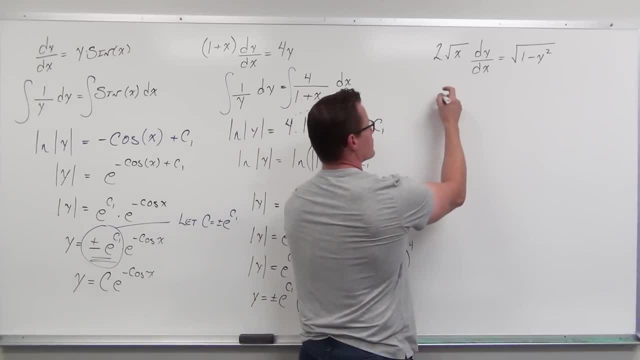 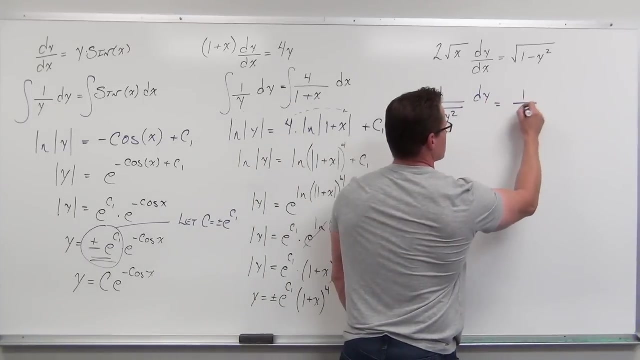 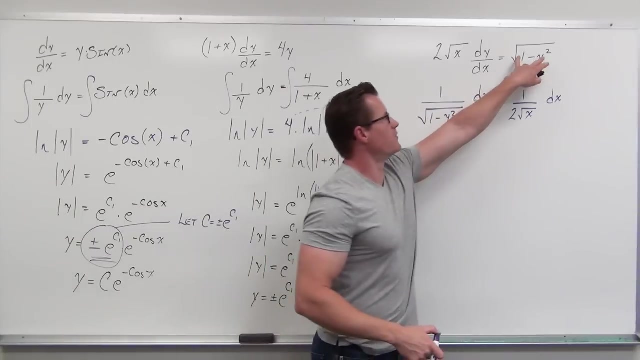 So if we divide both sides by the square root of 1 over y squared, 1 minus y squared, and we keep our dy, and we divide both sides by 2 square root of x and we multiply by dx, So we've divided both sides by the square root of 1 minus y squared. 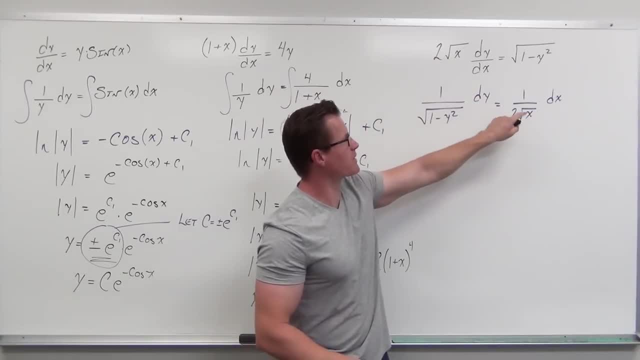 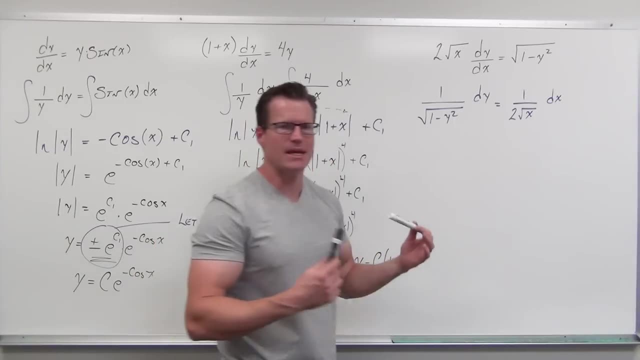 We've kept our dy. We've divided by 2 square root of x. We've moved our dx. Now we're ready to integrate. Hopefully you got the same thing, or at least thought about it and said, yeah, that makes sense to me. 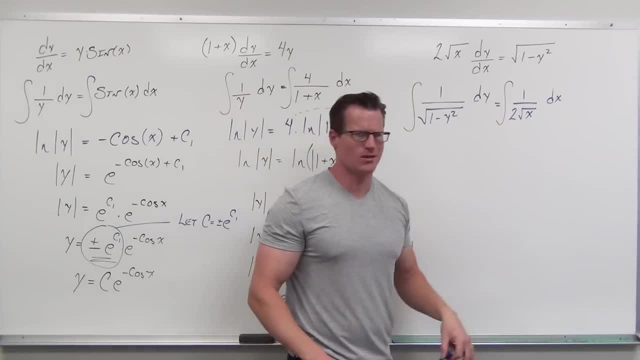 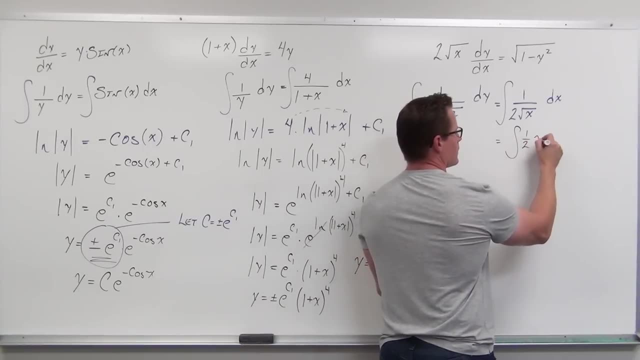 Let's look at that one. I don't want to do that, That's easier. Let's do the right-hand side. So on the right-hand side we've got an integral. We've got an integral of 1 half x to the negative 1 half. 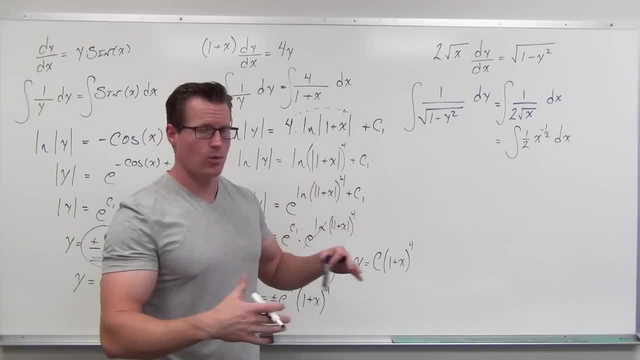 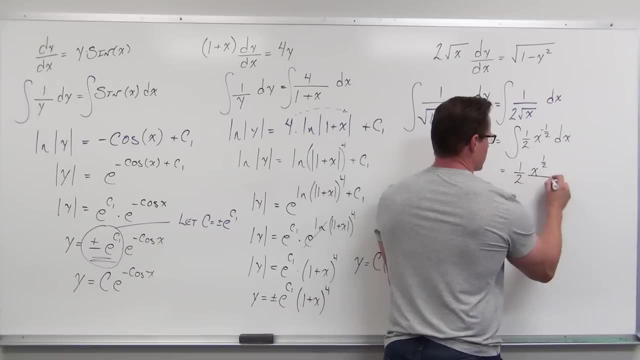 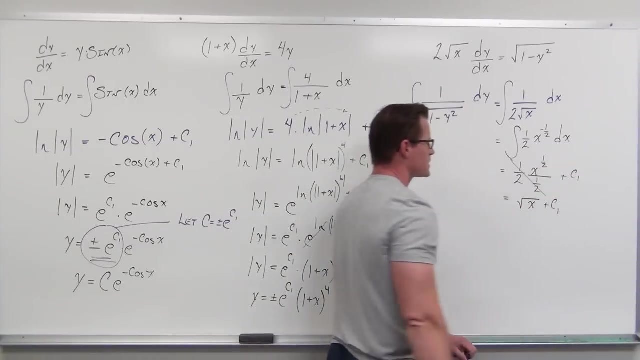 We can do all of our integrals with exponents the same exact way. We add 1 to the exponent and divide by the new exponent, 1 half, and 1 half are gone, Plus c sub 1.. So that would give us just this square root of x plus c sub 1.. 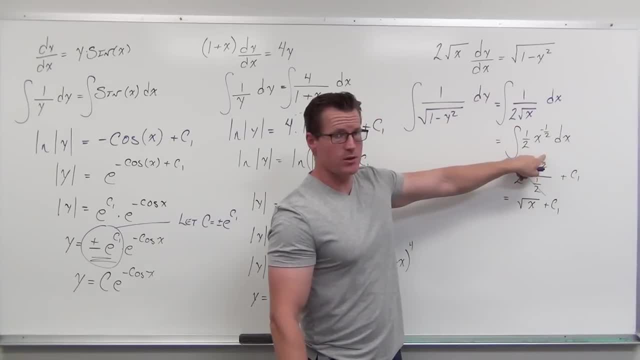 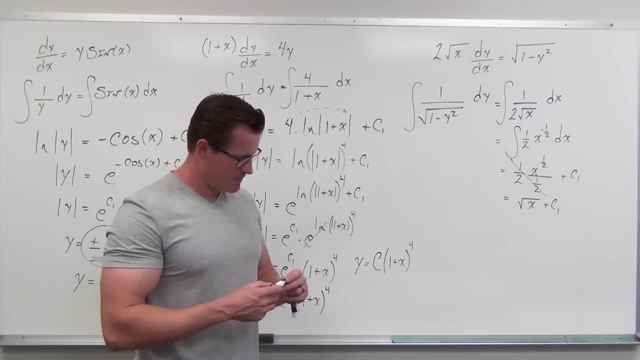 We've added 1 to our exponent 1 half Divided by new exponent 1 half. We already had 1 half It gone And now we just have square root of x plus c 1.. On the left-hand side, there's two ways that you should approach this. 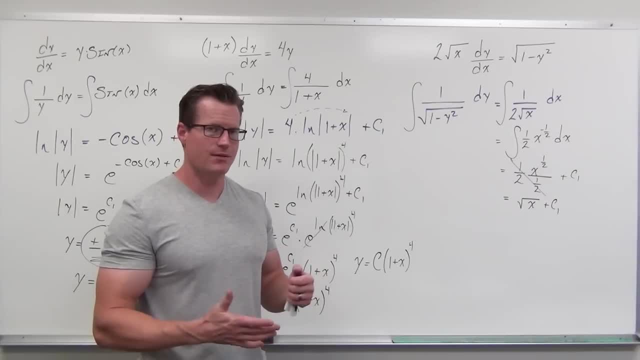 Number one way, if you're allowed to, or if you remember it, or if you have it, or if you've used it before, man your table of integrals. that's why they're in most every differential equation textbook, because of the back or the front. 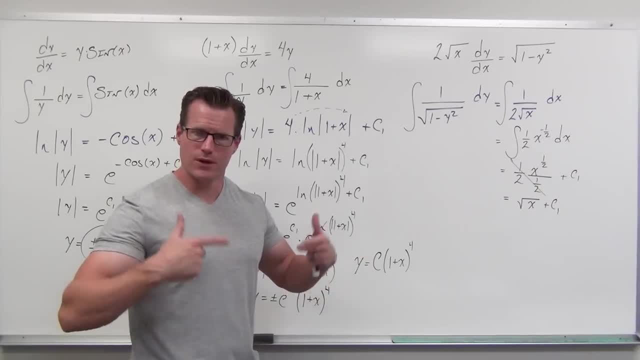 You go: yeah, you're going to use this a lot, So these are things that are very common, that when they come up, here's what our answer is: That's fine. This class shouldn't just be a repeat of Calculus 2, where you learn all of your integration techniques. 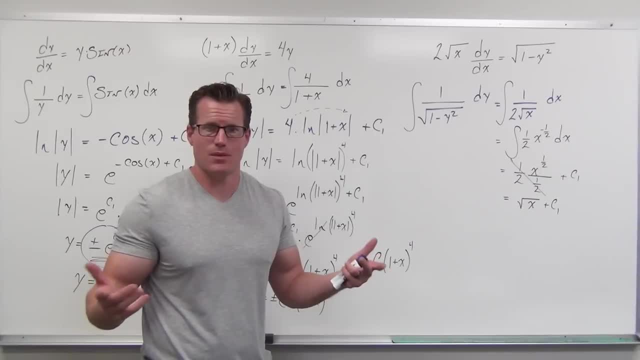 I'm showing it to you as a courtesy, And thank goodness that we have lots of time. You're my class, So you are my students. I'm taking the extra time to make sure you know it If you don't. if you do know it, great. 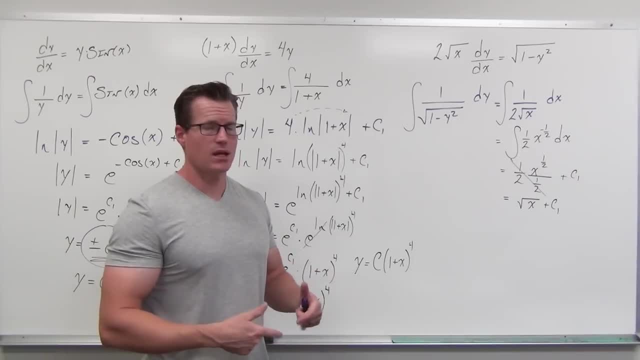 Use your table of integration. If you don't- and you forget it, or you're not allowed to, for some odd reason, do a trig sum, You could do a trig sum on this. In either case, you get sine inverse, Or maybe you've memorized that. 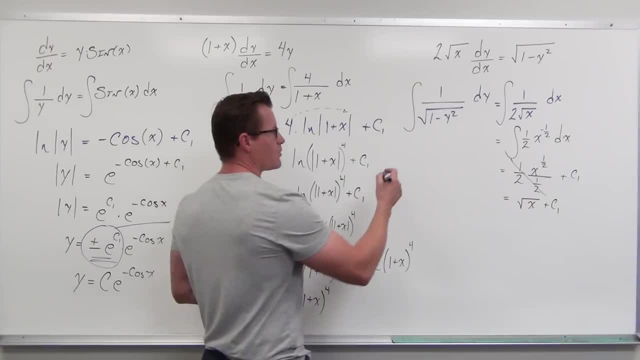 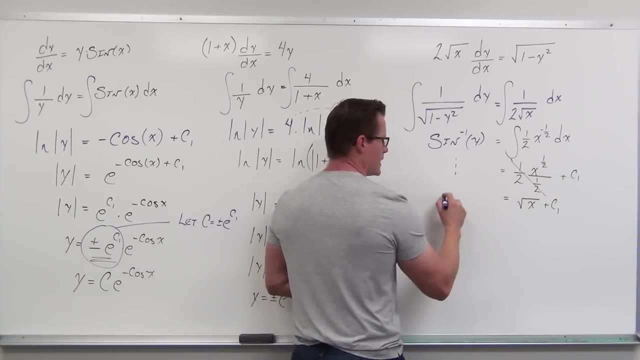 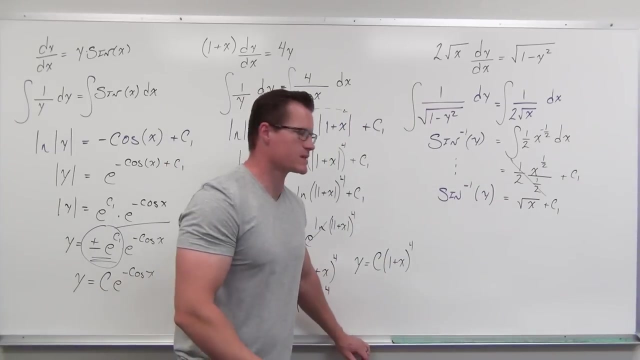 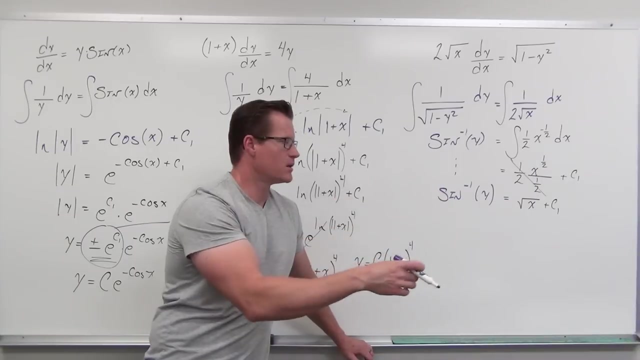 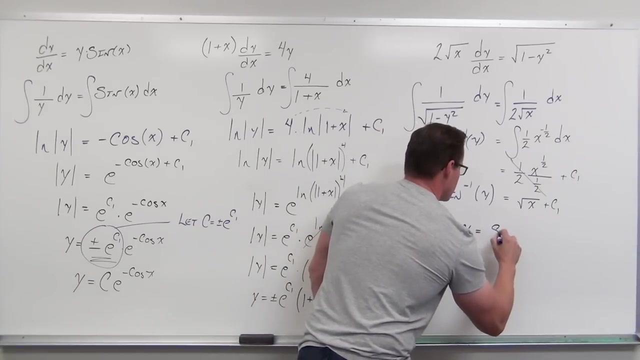 So we get this whole sine inverse of y. I'm dropping that down. Sine inverse of y equals the square root of x plus c1.. Remember that with inverse trig functions, if sine inverse of y equals something, then y equals sine of that something. 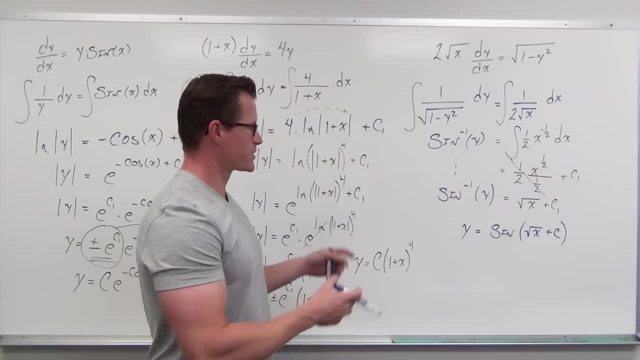 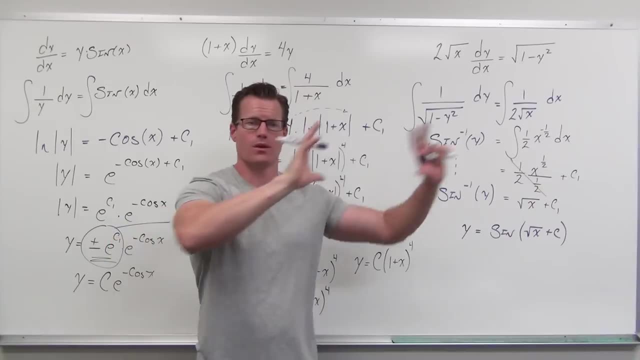 I'm going to drop the c1.. We don't have to change that constant at all. That's an arbitrary constant And that is the general solution to that difference. So we're always trying to group x's, dx's on one side, for you on this side. 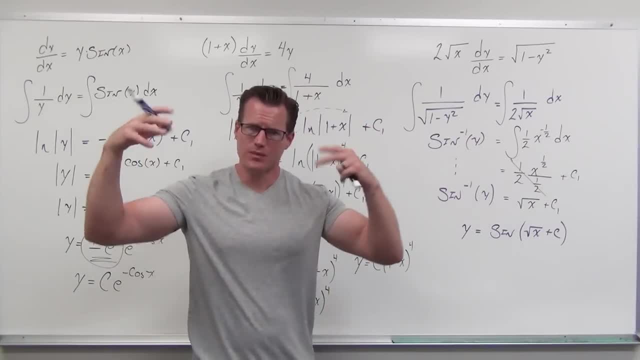 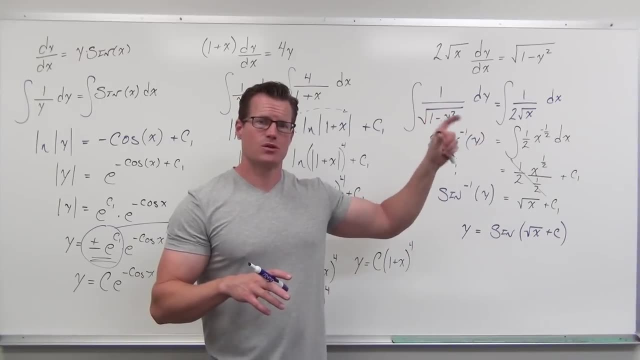 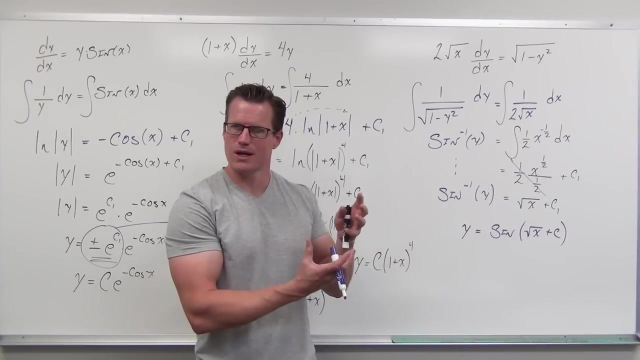 Y's dy's on the other side, Integrating both sides and then doing our very best to do two things. Number one: don't forget about your constant, Always a plus c, Making sure that we, if we can simplify that so it looks nicer as a maybe larger or different form of an arbitrary constant. 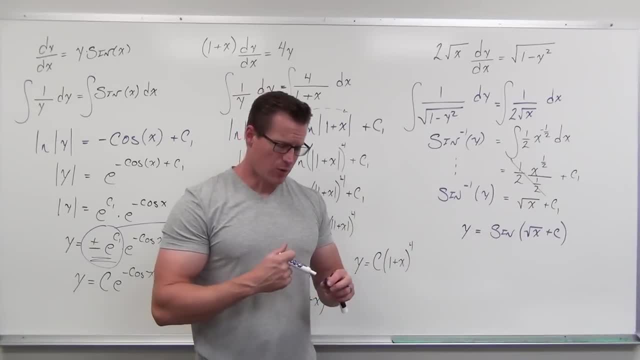 And solving for our y explicitly. We have several more examples. I hope this is making sense to you. If it's not, if you're not quite getting it- our integrals- it might be time to go back and watch some Calc 2 videos about how integration works. 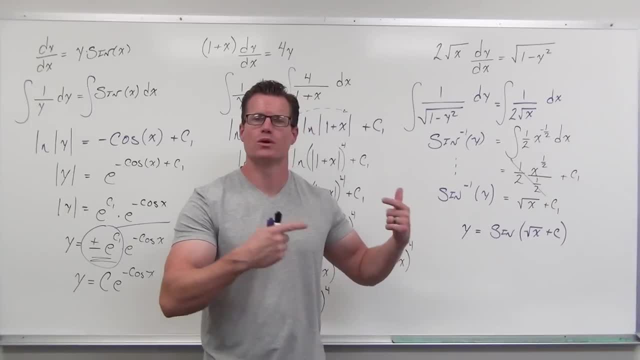 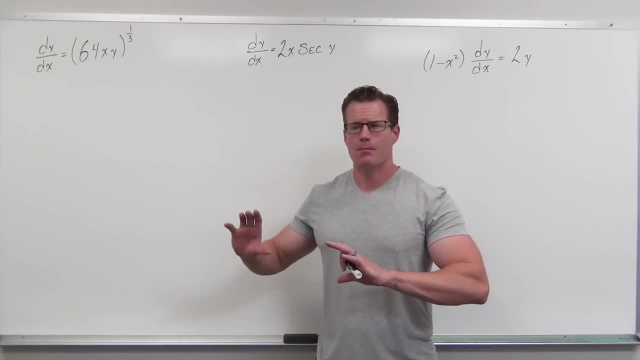 I'm trying my best to explain it quickly, but we're also looking at the form of differential equations here. We've got a few more on the board. Let's go through them. Make sure that we're understanding what's going on. Again, there's some techniques here that you might have forgotten about in integration. 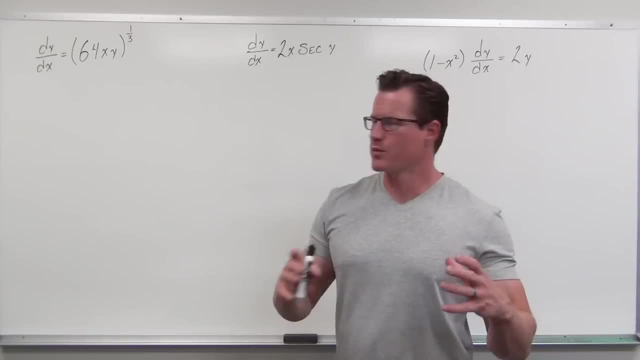 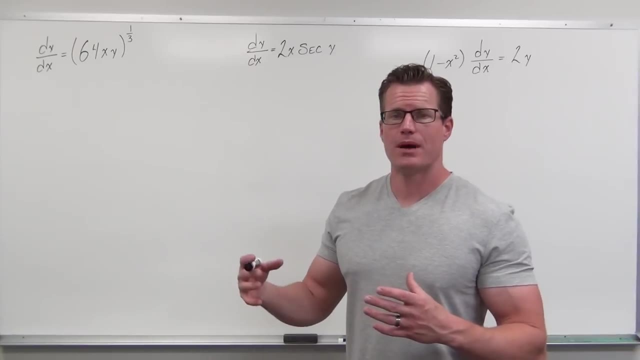 So first one: this is really close to fitting our form. We see a product on one hand side, on one side, the right hand side- We've got our derivative on the other side, But it's all wrapped up in that one-third power. 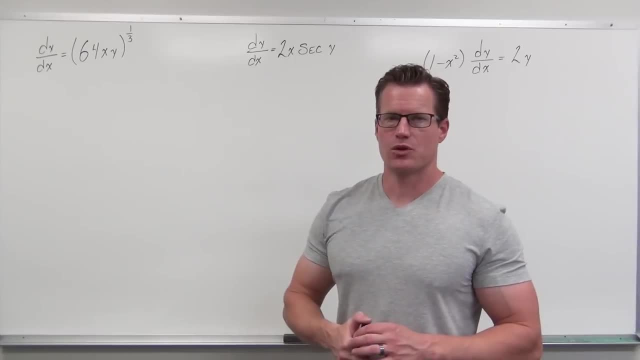 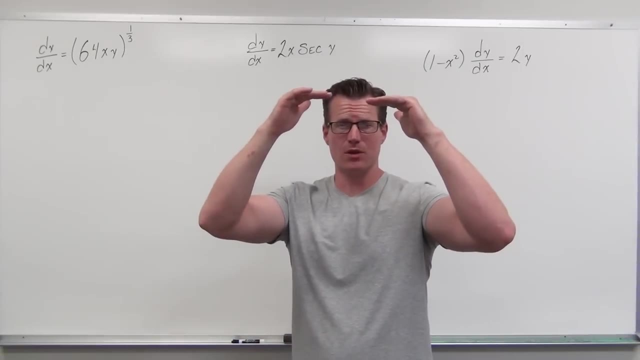 So sometimes all it is is a matter of distributing that exponent across multiplication and division. That's fine. We know that exponent rules work one level below what we have, So you can distribute exponents across multiplication and division, but not two levels down, not addition and subtraction. 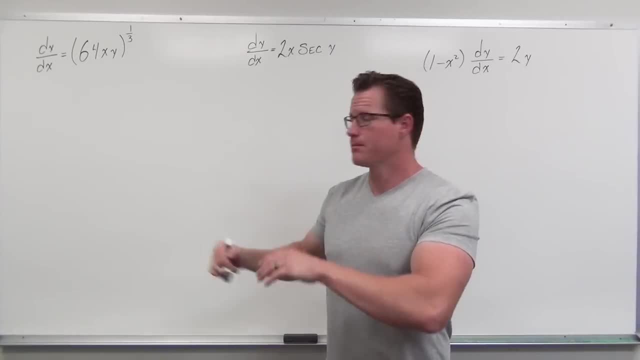 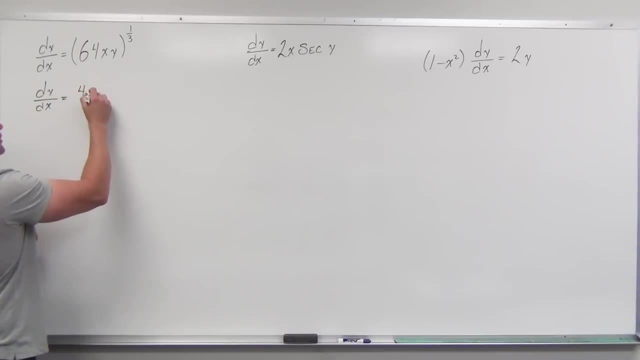 So we're going to take the cube root, or the one-third power of 64.. Not bad, That's 4.. We're also going to have x to the one-third power and y to the one-third power, And now we see that, yeah, that's some factors that are multiplied together. 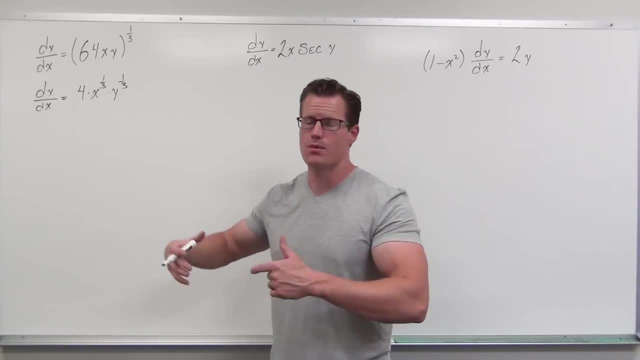 We can move our y, We can keep our coefficient of 4. And we can keep our x and move our dx. Let's go ahead. Let's write it as something that we can integrate. So 1 over y to the one-third power looks pretty good. 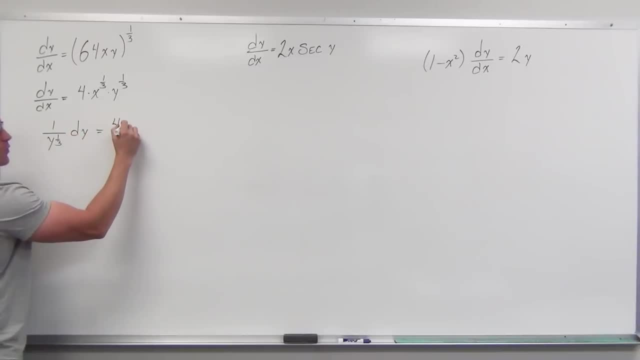 We're going to keep our dy Right hand side, we're going to keep our 4.. We're going to keep our x to the one-third And we're going to have our dx. We just multiply on both sides to get that. 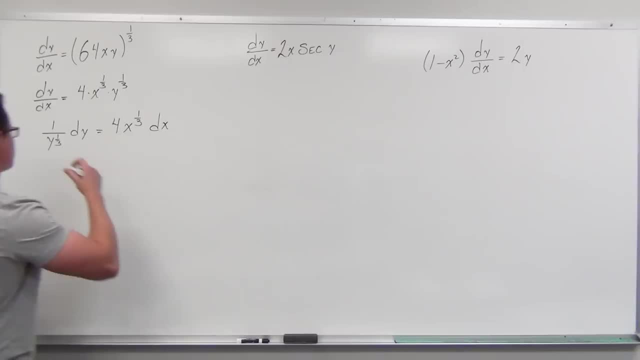 Now we're able to integrate, So let's try it On the right hand side. that's pretty nice. Our coefficient of 4 stays, Remember, with our exponents, we add 1 and divide by our new exponent And we're going to have a plus c. 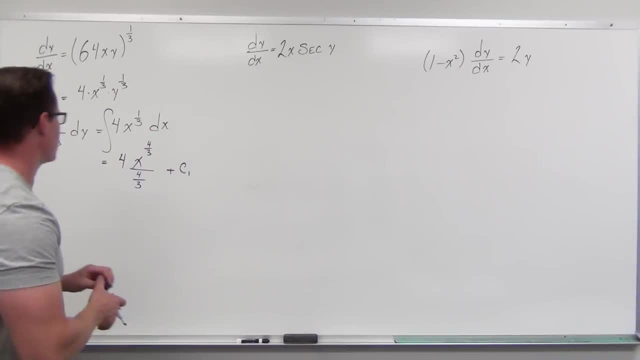 We're going to call it plus c1, sort of expecting that we're going to change that later. On the left hand side, well, this is the integral of y to the negative one-third dy. So y to the, let's add 1.. 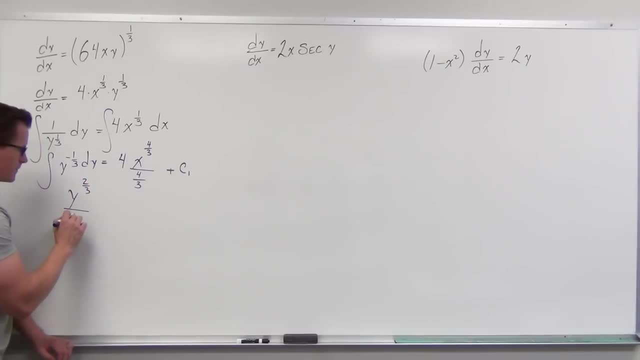 That's positive two-thirds divided by two-thirds. On the right hand side, our 4s are gone And we can move our 3 to our numerator. So we're going to get 3x to the four-thirds plus c1.. 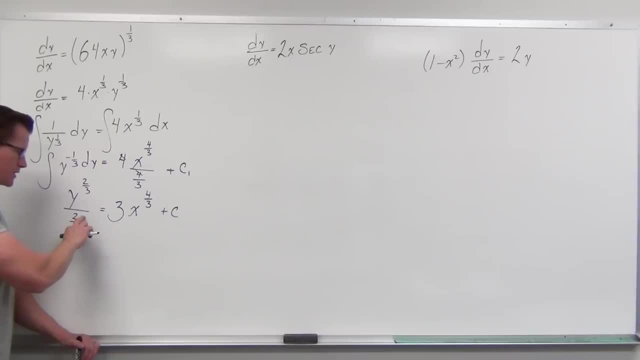 Now a couple options. You can move this first and just get 3 halves y and divide everything by two-thirds. Or well, multiply everything by two-thirds. Or you can multiply by two-thirds now. So either one of those is absolutely fine. 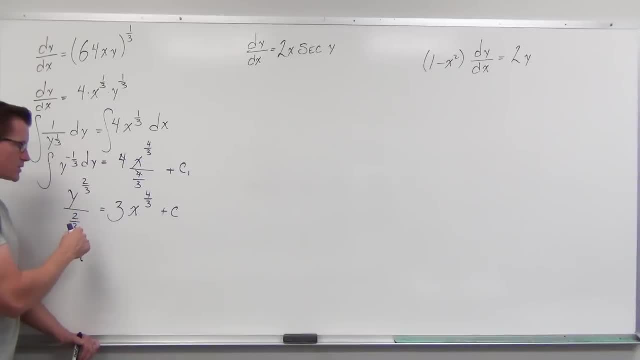 So if we do that, if we multiply by two-thirds, then we're going to get Just y to the two-thirds On the right hand side. when we distribute that, our 3s are gone, We're going to get 2x to the four-thirds, plus two-thirds c1.. 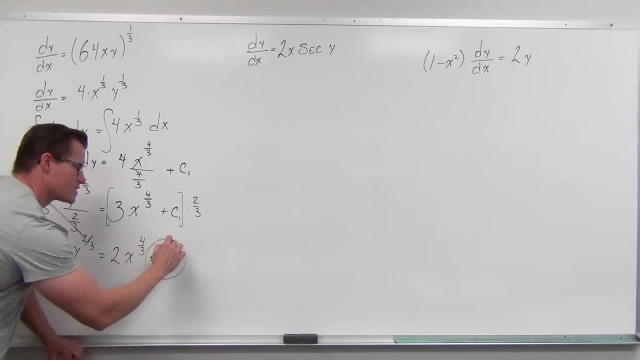 We're going to wrap all of this stuff up And we're going to say: let's just let that become our arbitrary formula. This is our arbitrary constant. That way it's a little bit cleaner. So if we have y to the two-thirds, then essentially we can raise both sides to the three-halves power. 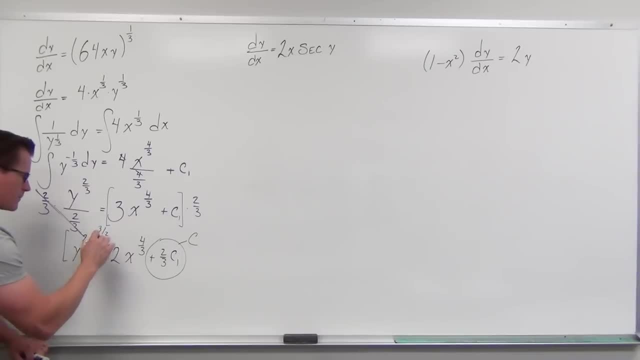 So if we do that, raise both sides to the three-halves power, exponents raise to exponents multiply. One of the low exponents raising to exponents is multiplication. That's what we do with our exponents. This is completely gone. 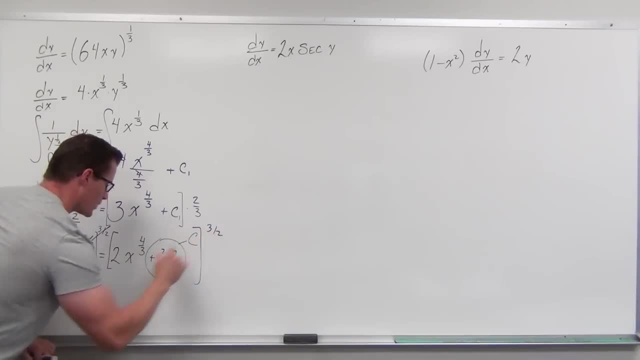 On the right hand side. we raise all of this to the three-halves power as well And we get y equals this 2x to the four-thirds- looking good- plus a big arbitrary constant, And then this is just raised to the three-halves power. 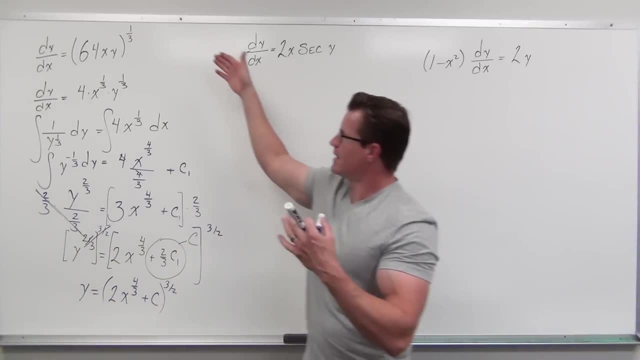 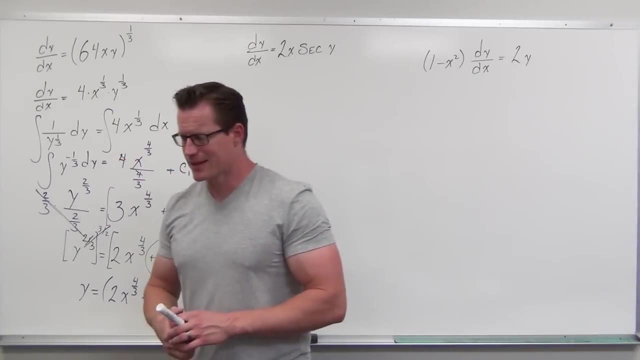 So we've grouped our x's, grouped our y's. We had to distribute an x node. That's fine. And then we do an integration And then the hardest part of all this stuff is just solving for y. That's like the most challenging part is just doing that. 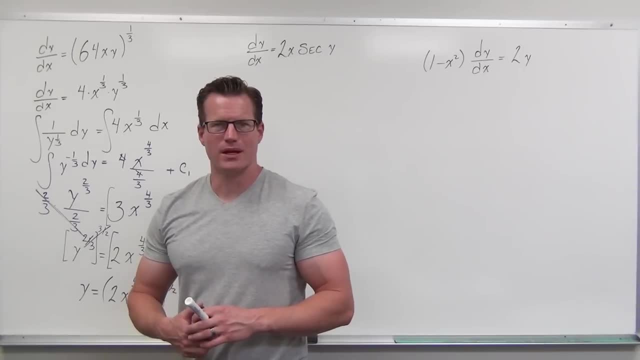 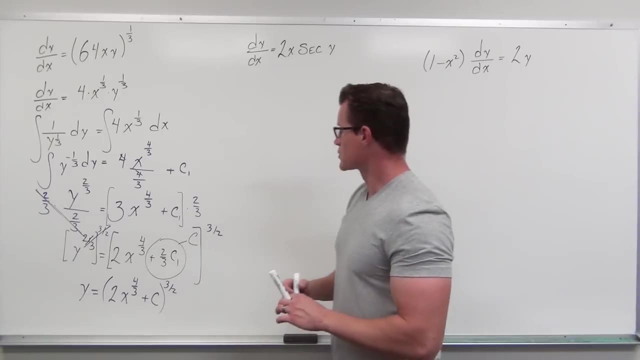 So make sure that we're doing it right, Make sure that we're not making little teeny errors- and hopefully I didn't making little teeny errors on that, So let's go on the next one. That looks good already. So this is a differential equation. 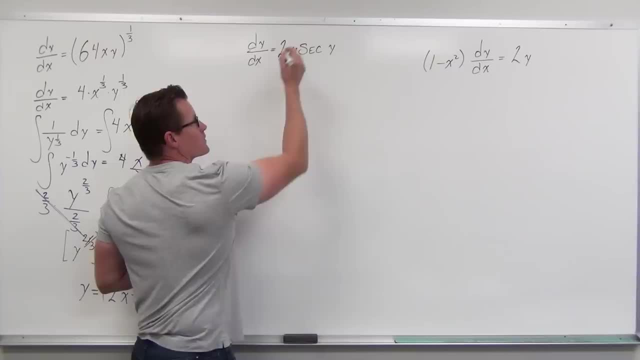 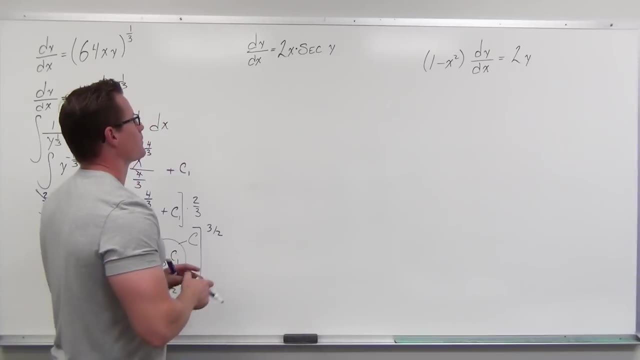 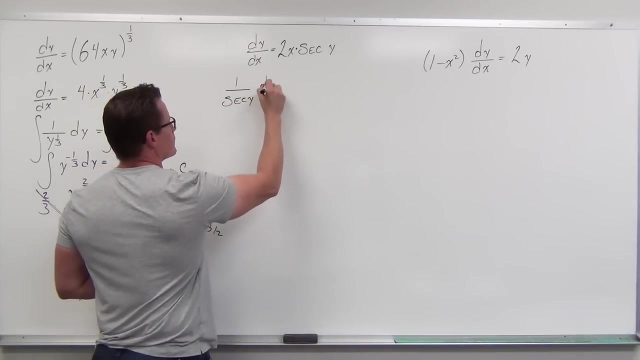 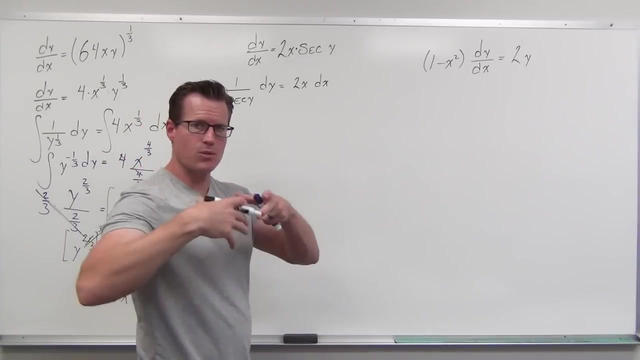 We have this function of x, this function of y. It's multiplied together, It's really solid. Let's move our y's, Let's move our x's. Try that now, Do it on your own. if you can, Group my y's dy, Group my x's, dx. 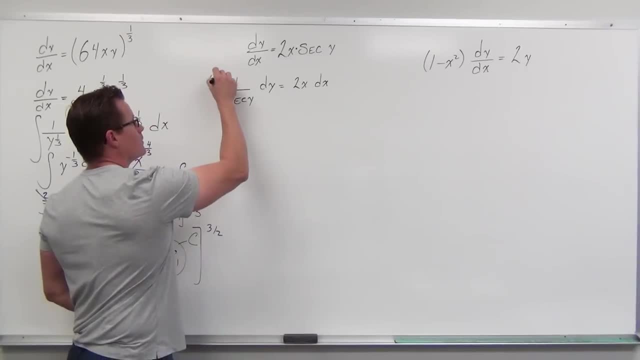 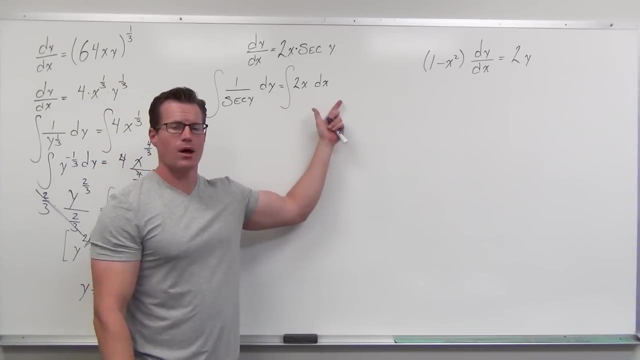 Take an integral on both sides. Try that if you haven't. Well, that was easy. Now, on the right-hand side, that's a piece of cake. That's going to be x squared plus c1, no problem On the left-hand side. don't overthink this stuff, okay. 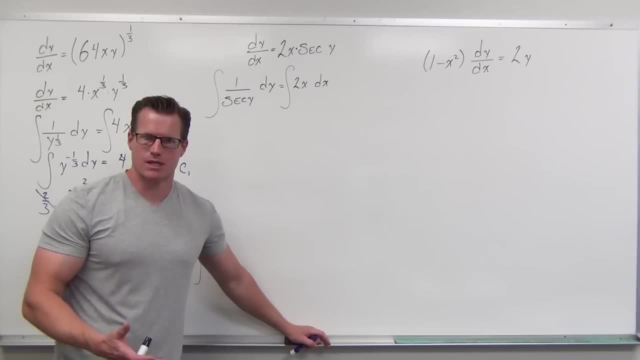 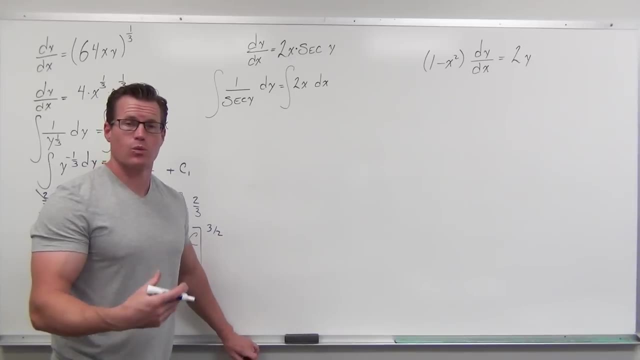 Don't try to make it harder than it is right now. It's harder than it is, is what I'm saying. So when we have this 1 over secant y dy and you're struggling to figure out what that is, think about what 1 over secant y really means. 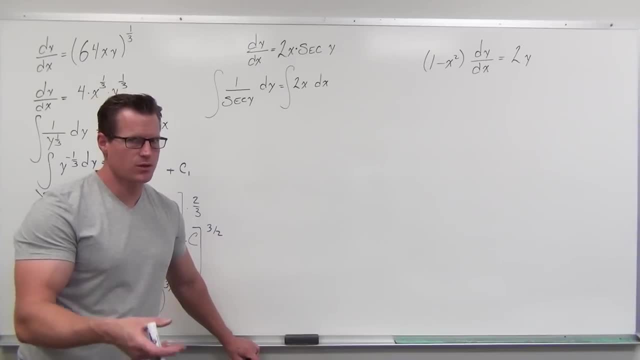 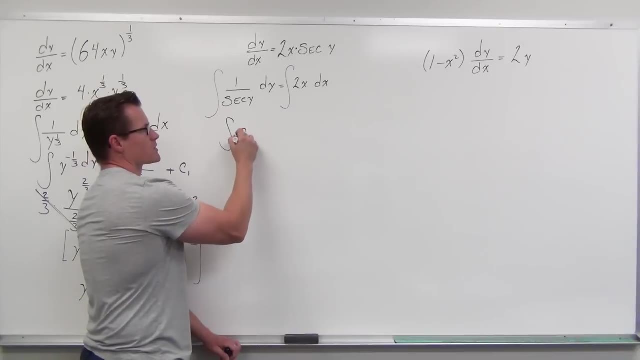 1 over secant. well, let's see, secant is 1 over cosine, So if we have 1 over secant, that's just cosine. This would be integral of cosine y. dy equals integral of 2x dx. 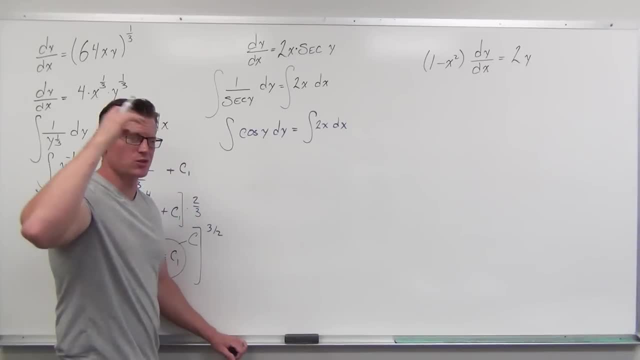 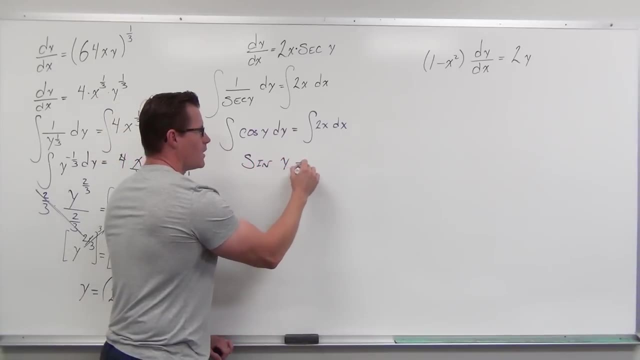 And that gives us something really nice to integrate The integral of cosine. well, the derivative of sine gives us cosine, so the integral of cosine gives us back sine of y. On the right-hand side we have x squared plus c1, as expected, 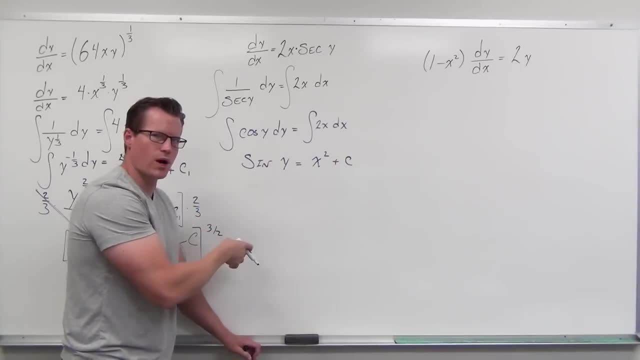 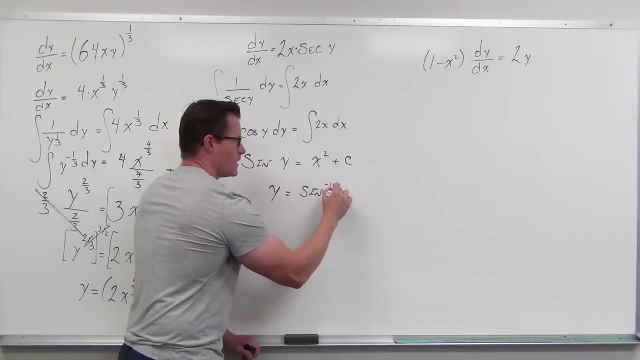 Let's just call it c. There's nothing fancy when we're going to solve for y here with an inverse. If sine of y equals x squared plus c, then y equals sine inverse of the same. And we're good, That's our general solution. 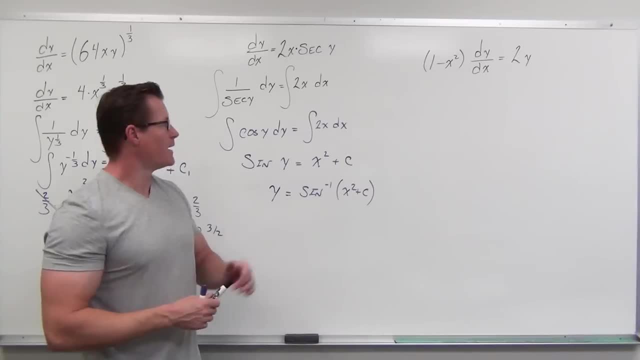 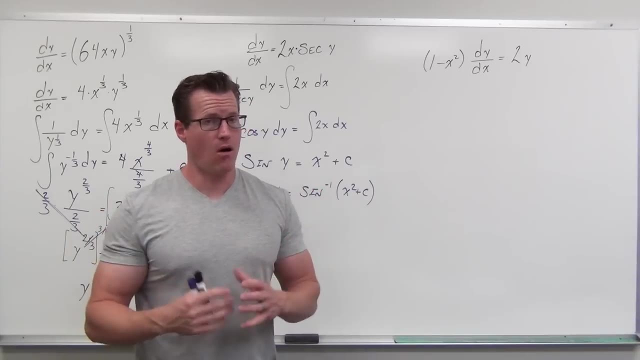 It's got a real nice plus c in there, Not as hard as you might have thought. It's just a matter of recognizing what you're doing with your integrals. So separating your variables, these separable equations, they're not hard as far as typically the setup. 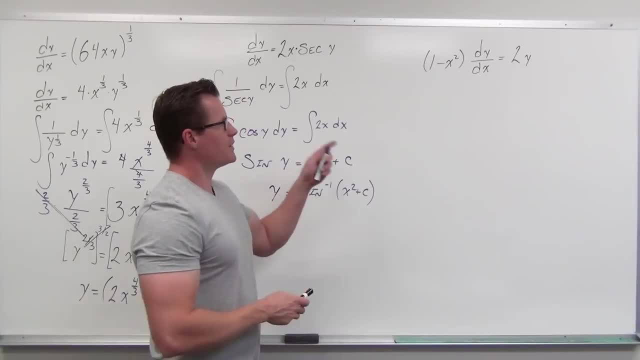 They're not bad, but the integration techniques might get you On the next one, so let's try it. If you haven't done it right now, I would really recommend pause the video, see if you can group your y's on one side with your dy. 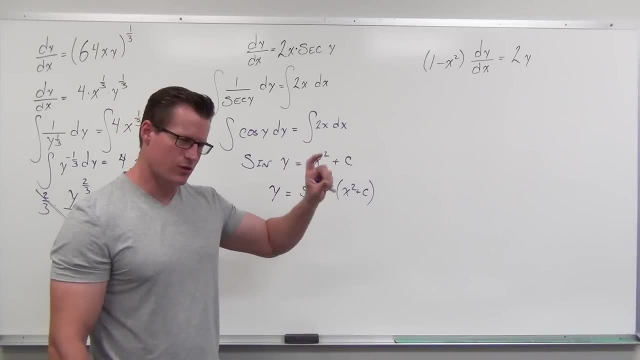 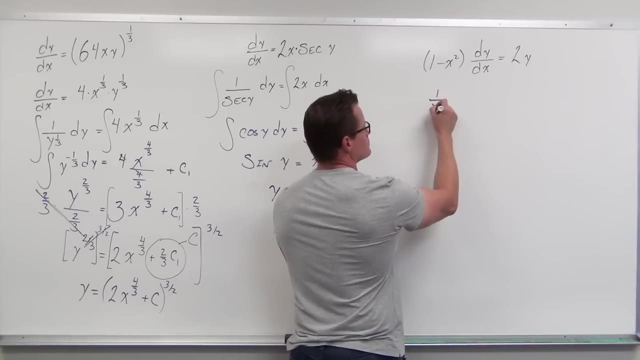 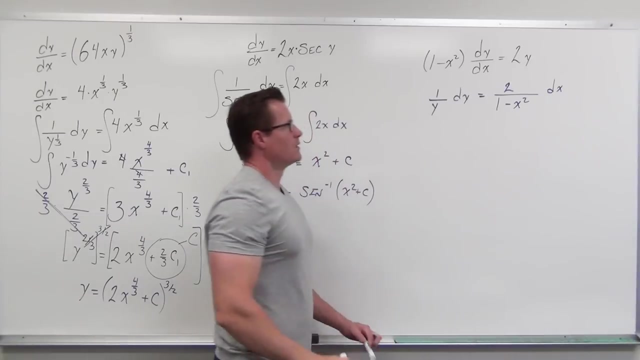 group your x's on the other side with any constants, coefficients that are constants, and dx. My y's got to move 1 over y. we keep our dy. Our x can stay there. We have to divide by 1 minus x squared. 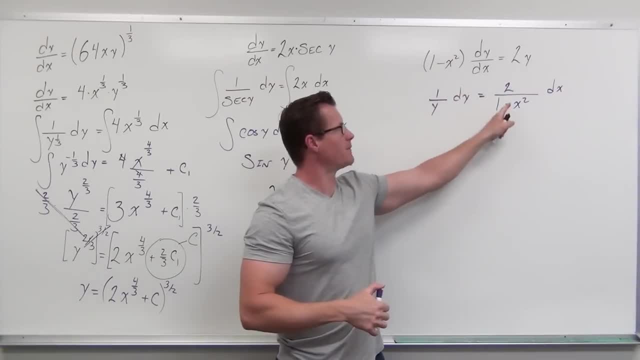 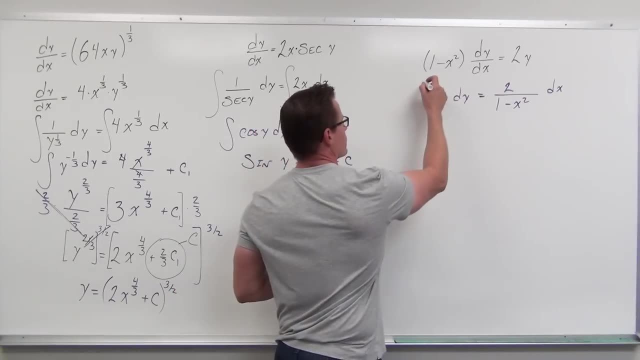 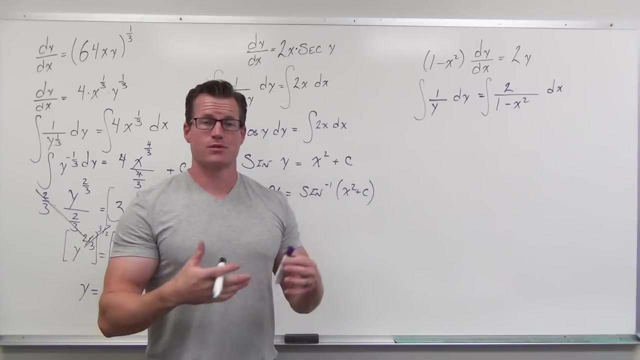 So we get this 2 over divided, that 1 over y divided, that keep our dy, move our dx, and now it's time for us to integrate Left-hand side's- really a non-issue. We have this absolute value of ln, of absolute value of y. 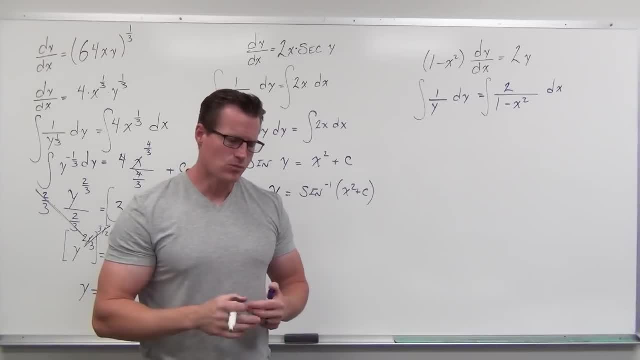 We've got it several times before. On the right-hand side, 2 over 1 minus x squared. there's a lot of people who just really, really, really, really want to do like a trig sub on this. This is not a trig sub. 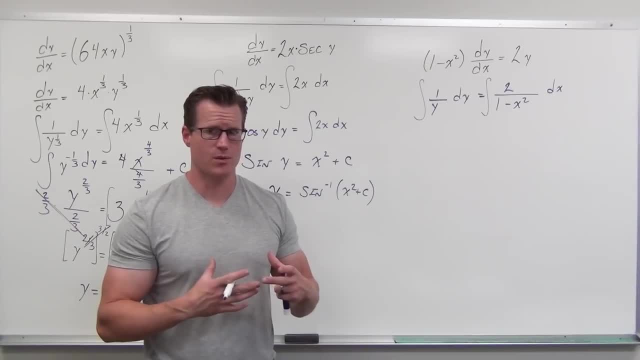 It's not going to work out for you. There's no square root there. It's really hard to represent that. We don't want to try it, because what you end up getting is, if you do force this thing, to do a trig sub. 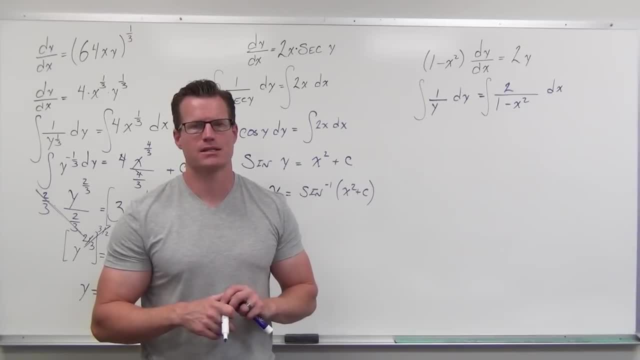 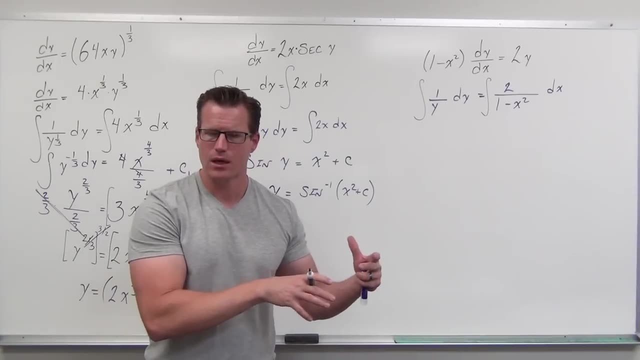 I think it's like secant theta d theta and that's a nasty integral. It would work, but there's an easier way to go around doing it. So instead of going about that way, let's see if maybe we can revert back to something a little bit nicer. 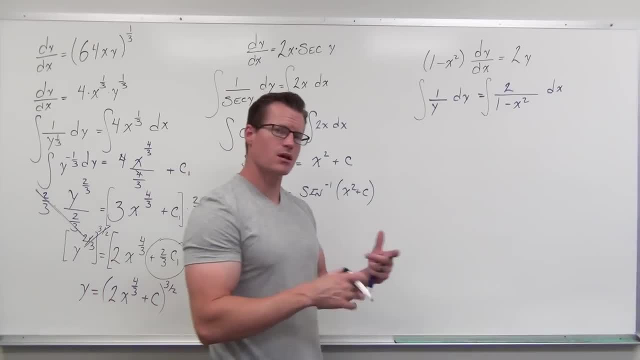 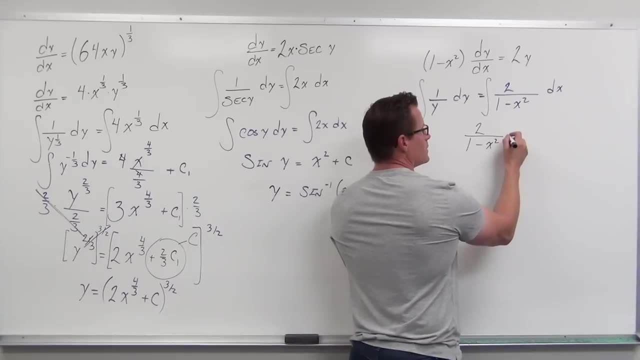 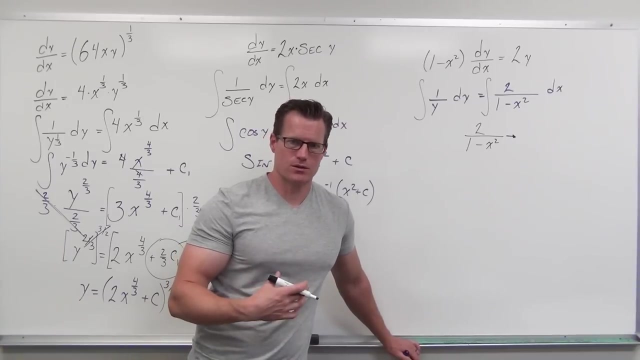 like: how about partial fractions? So let's take a moment and review that. So we have 2 over 1 minus x squared. If you remember how partial fractions work, they rely on your ability to factor into linears and irreducible quadratics. 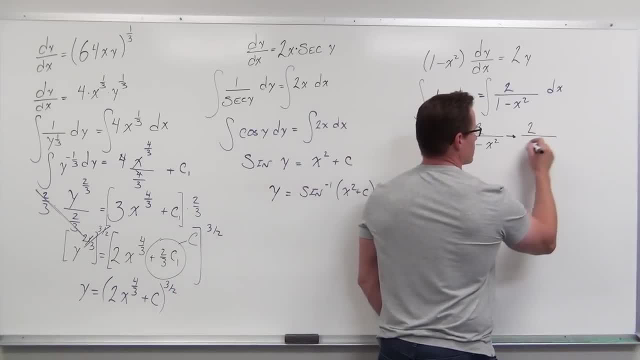 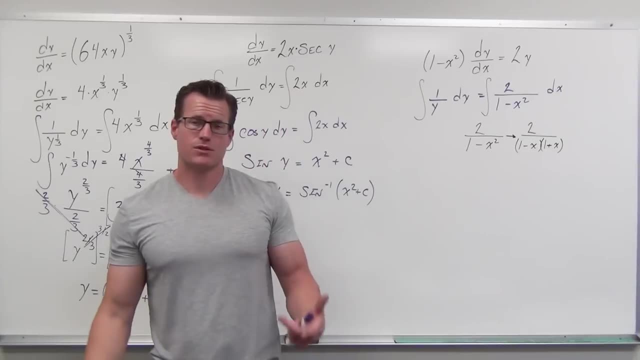 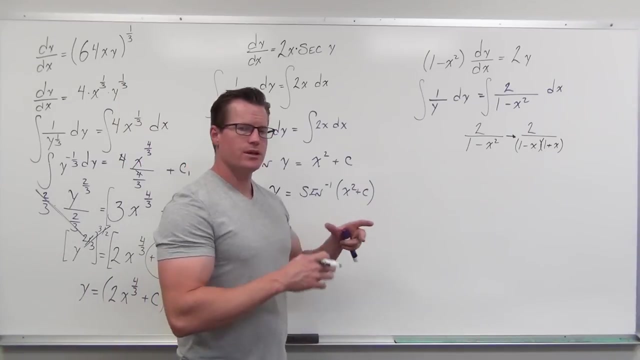 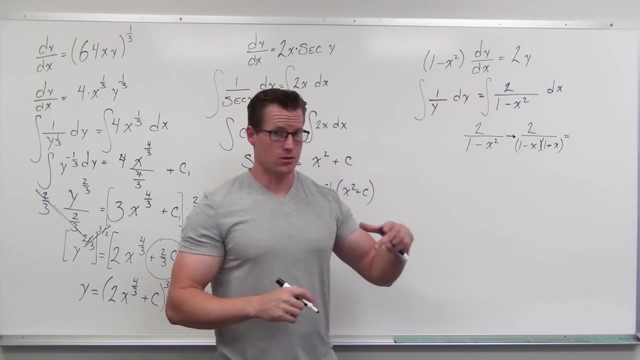 So what that means is that we can write that as a difference of squares, So 1 minus x and 1 plus x, And now we do our partial fractions, So partial fractions, say, for any linear factor that you have on your denominator. 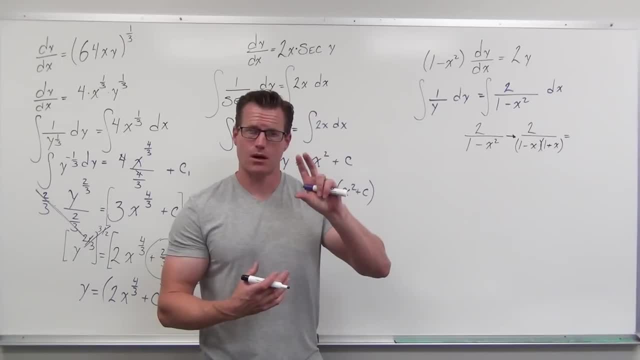 you're going to create a fraction for that with a constant on the numerator. The numerators on partial fractions are always 1 degree less than the denominator. So if your denominators are linear, your numerators are constants. If your denominators are quadratics, your numerators are linears. 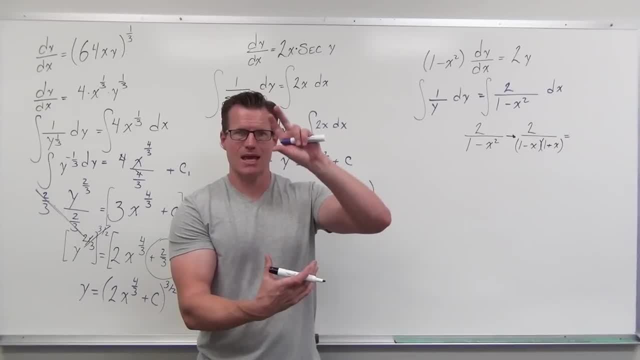 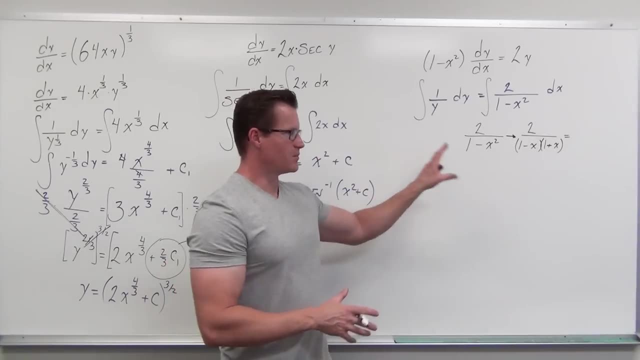 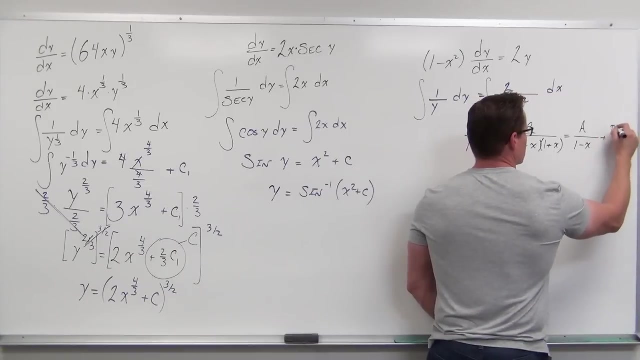 So like x squared plus 1, then you get ax plus b or cx plus d or a linear over that. So that's how those work. We don't get a whole lot of that. We get some basic ones like this, though a lot: 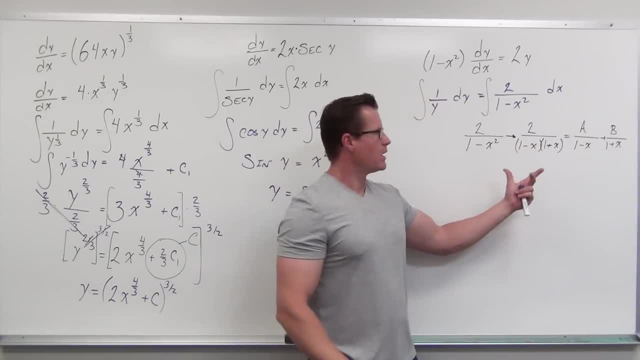 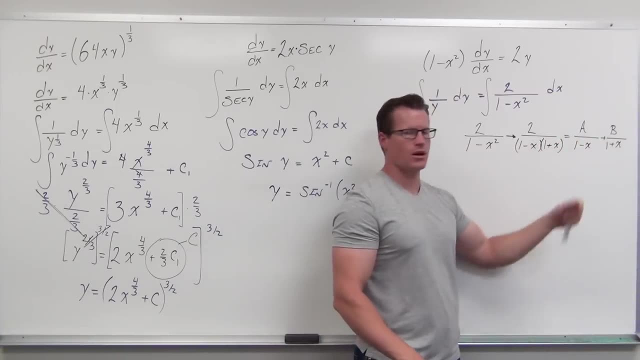 So we know that we can split this up somehow, as long as we have our same two factors. That's a linear, I have a constant, That's a linear, I have a constant- and they're added together. Now the whole idea of where you go from there is basically just. 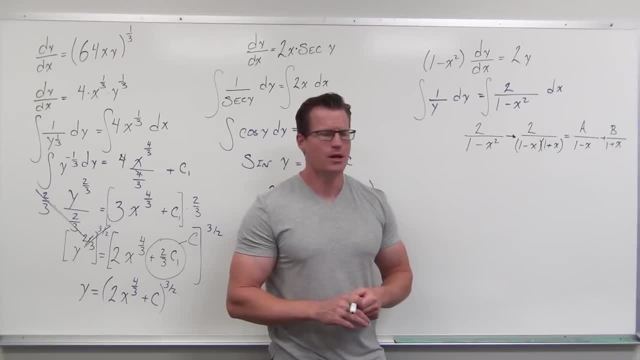 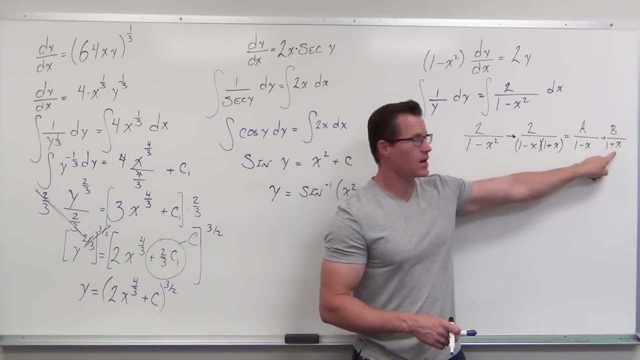 I call it a cover-up method, but it's basically just finding a common denominator. So if we found a common denominator, what would happen here? You would have to multiply this times 1 plus x. You'd have to multiply this times 1 minus x. 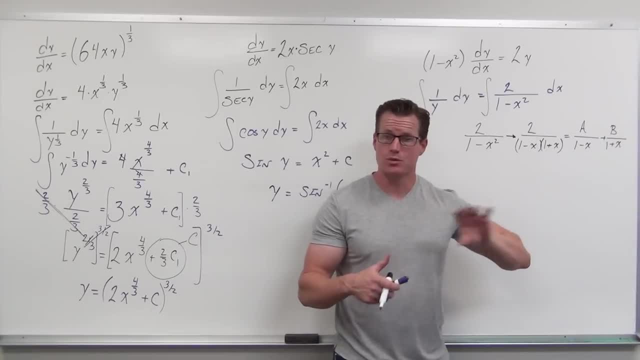 And then if you were to add the fractions, your denominators would be the same. That means that your numerators would also have to be the same. Now that all boils down and that's not really explained very often in a Calc 2 class. 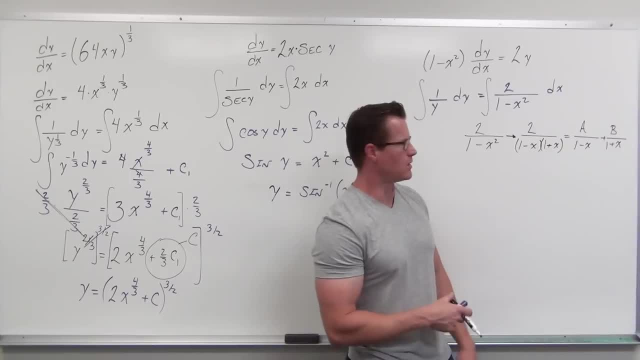 where you learn about partial fractions. You might explain and say: oh, just do this, Cover this one up, put this here, cover that one up, put this one there, and then just make sure it's equal to 2.. Why? 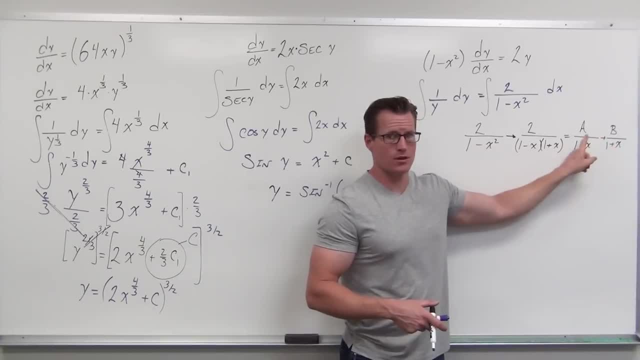 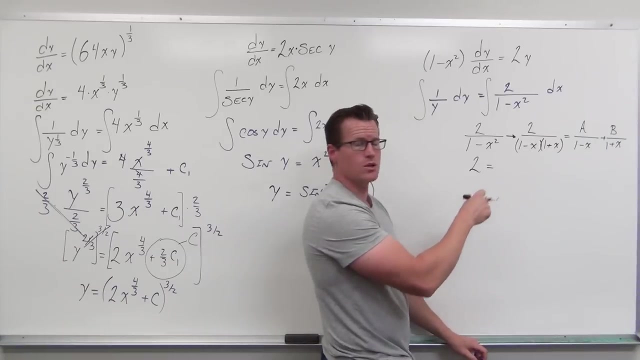 Because you're multiplying a times the factor that this needs and b times the factor that this fraction needs. this, 1 minus x, That's creating a common denominator. When you add your fractions, 2 will be equal to the numerator that you're creating. 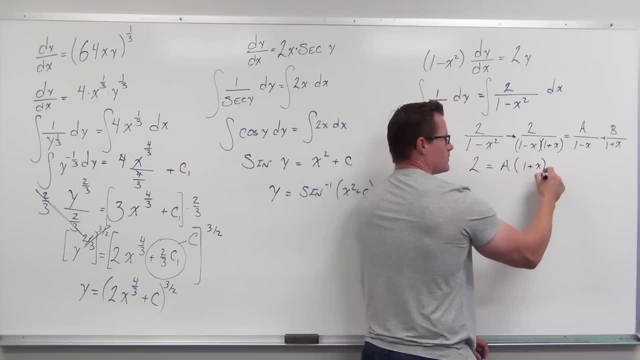 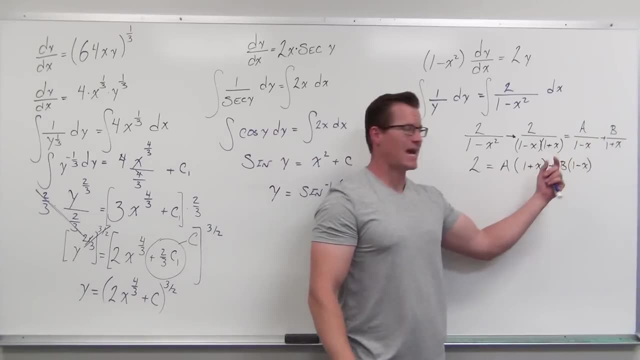 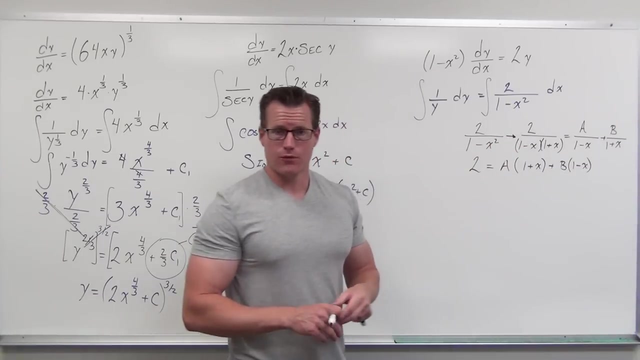 by finding a common denominator. If you went and found a common denominator for these two fractions and added the fractions, that's your numerator. That's the numerator we had. They've got to be equal. Now, how we go about solving for a and b. there's some nice stuff. 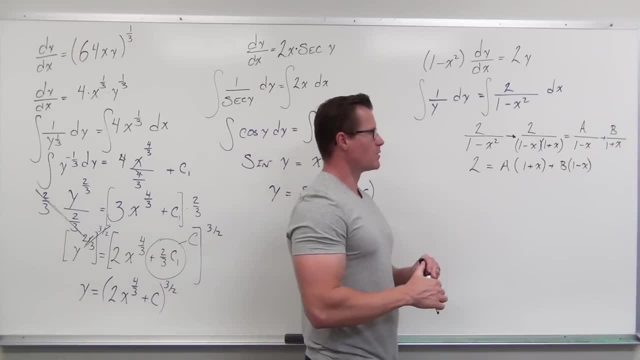 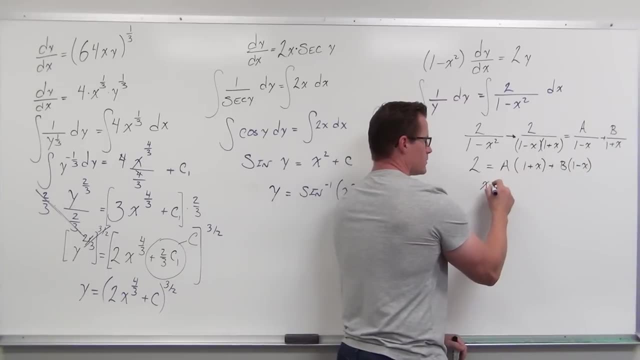 when you're dealing with just linears, Plug in a number that's going to create these factors as a 0. So, for instance, I'm going to plug in 1.. If x equals 1,, I'm going to plug in 2.. 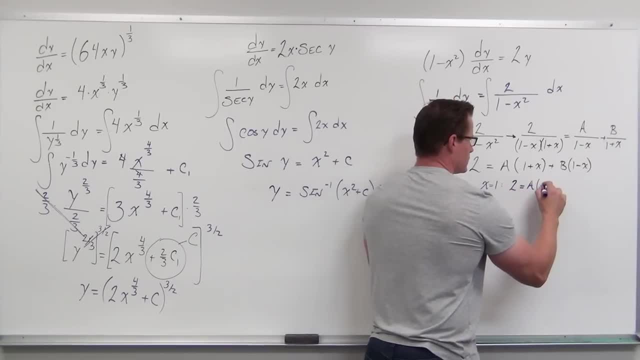 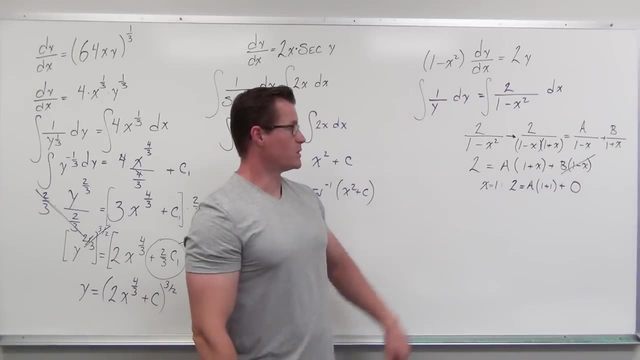 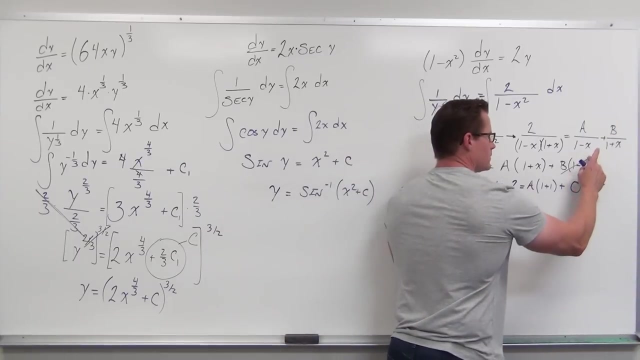 If x equals 1, that factor would be 0.. If x is 1, this factor goes to nothing. 1 minus 1 is 0. That's a 1.. Cool, So we would get b equals 1.. 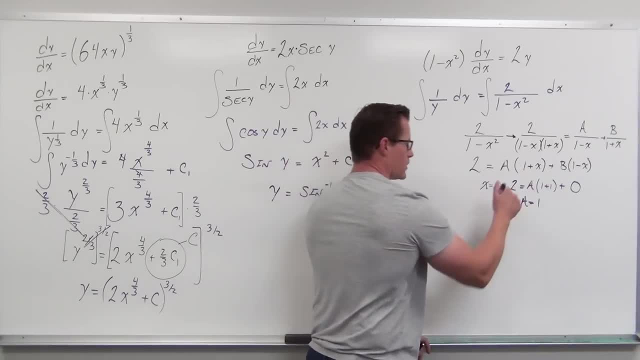 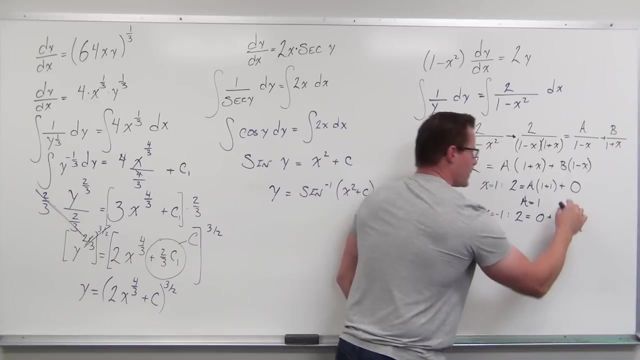 2 divided by 2 is 1.. Now plug in negative 1.. 1 plus negative 1 is 0. But 1 minus negative 1 is 2, which means b is also 1, which is kind of nice. 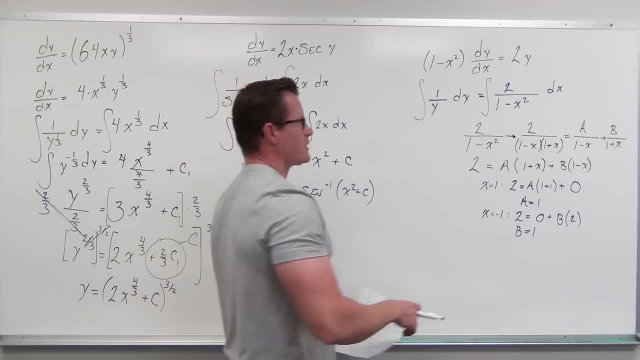 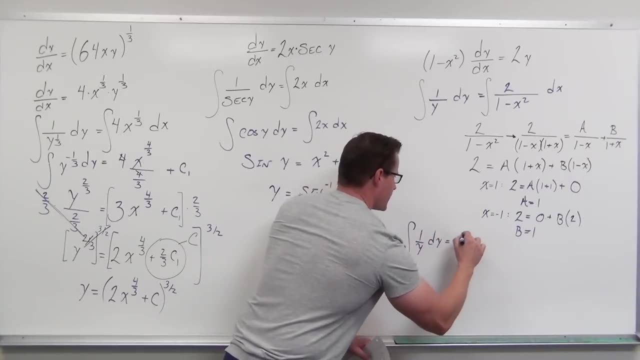 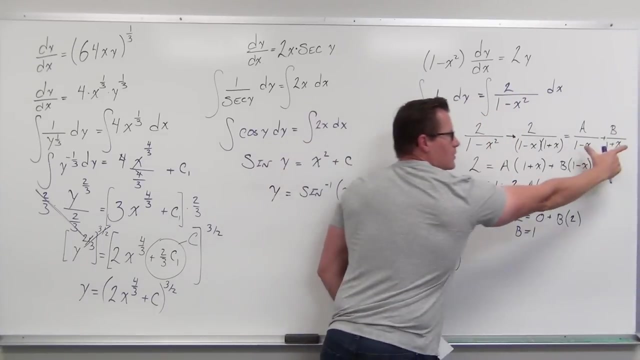 So, moving on from there, if we wanted to go ahead and write these fractions out, our integral changes a bit. We have an integral of 1 over y dy. We've got an integral now of: instead of all this stuff, we've used some partial fractions to say that this is now this, right here. 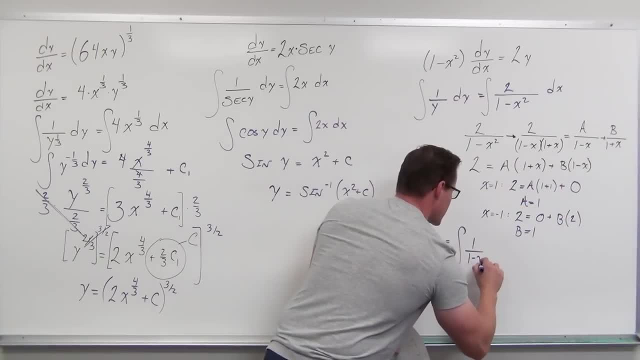 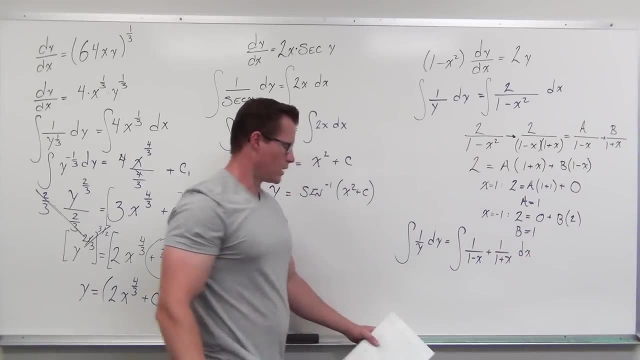 where a is 1 and b is 1.. So that's 1 over 1 minus x plus 1 over 1 plus x dx. And if we integrate after that, let's just use the same thing we've been doing. 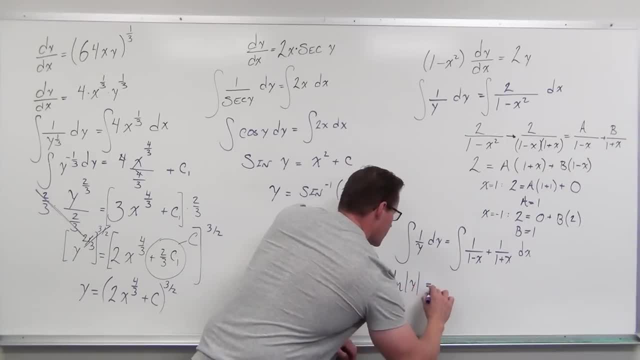 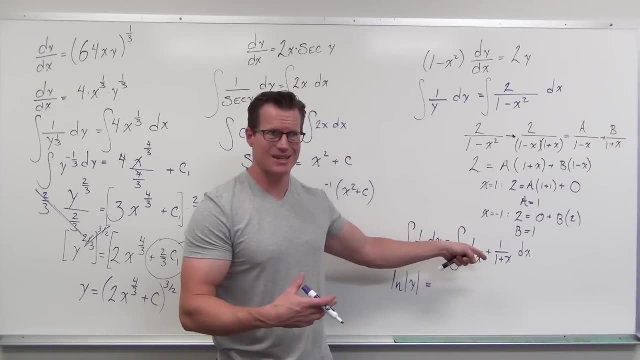 Well, we've got ln of the absolute value of y On the right-hand side. these are both ln's. We had something very similar in one of the first examples where we did, hey, 1 over 1 plus x, That's just ln of 1 plus x, an absolute value. 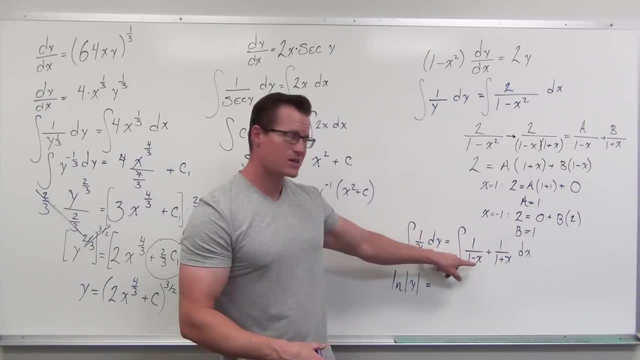 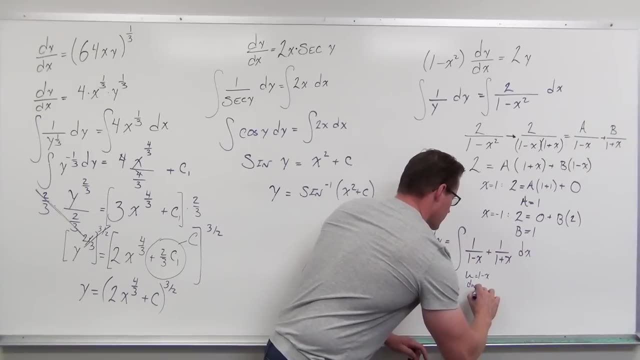 ln of 1 minus x, but we have a negative in front of it. Do you see why? If you had to do a U-sub, you would get negative dx. It's going to have a negative in front of your ln right here. 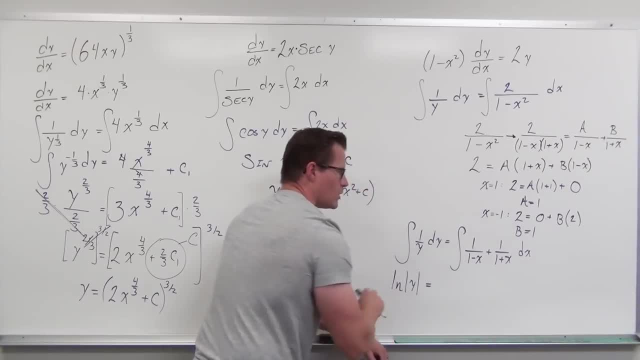 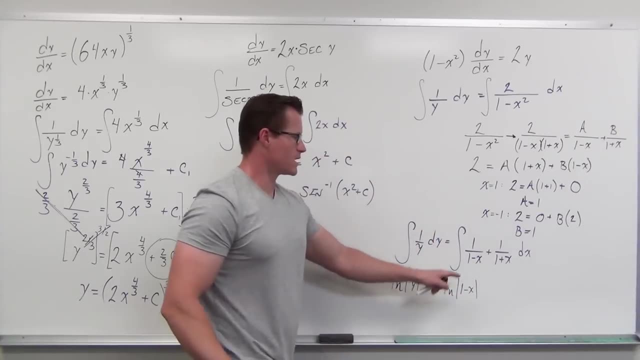 So we get integral of 1 over 1 minus x. That's ln, That's absolute value, That's 1 minus x. Yes, but it's got a negative because the derivative of this inside part, if you will, is negative 1.. 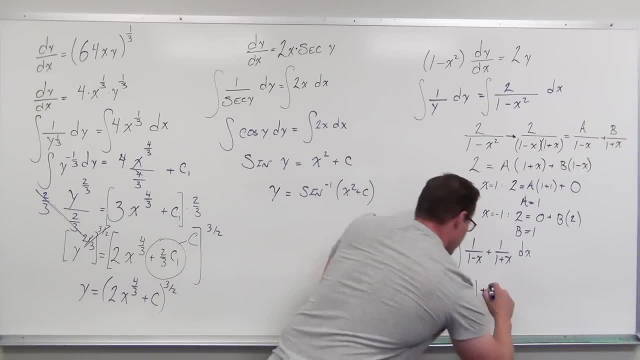 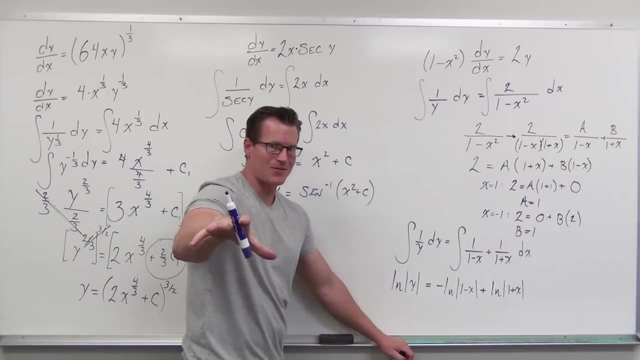 Plus 1 over 1 plus x. Well, that's ln absolute value of 1 plus x. And you all say: what do I need after this? Let's call it C1.. We know that we're going to be changing that. 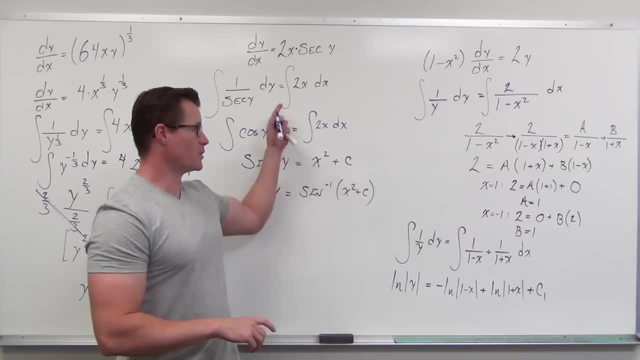 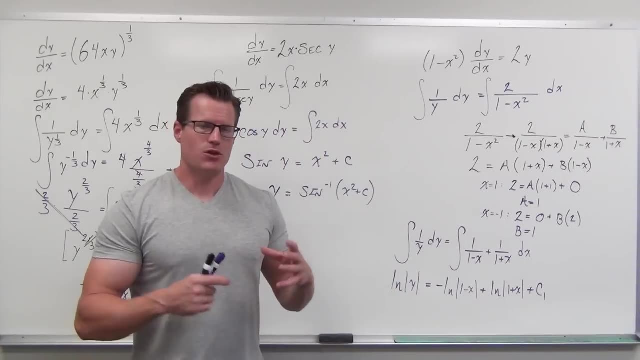 Now, before we go any further, I'm going to have to move over here, so I'm going to erase it. But before we go any further, we need to know some properties of logarithms, stuff like if you are adding logarithms together or subtracting logarithms. 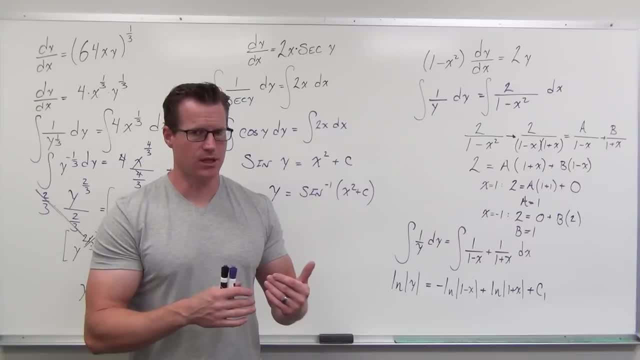 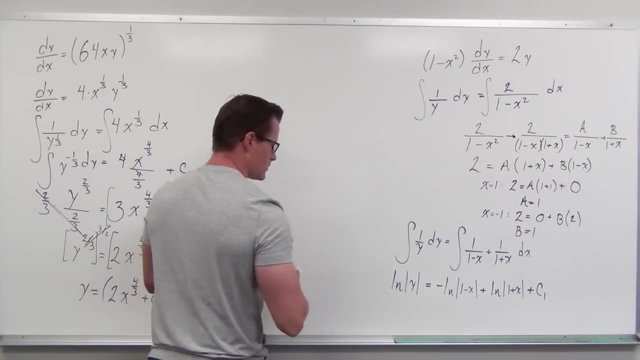 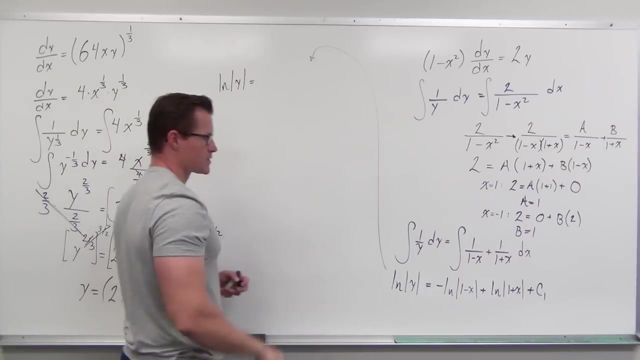 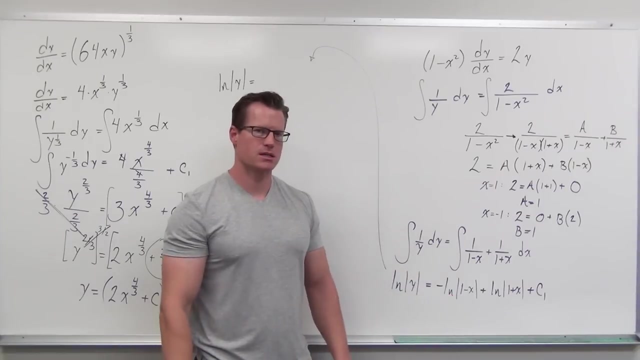 they create a product or a quotient respectively. So when we're doing this, ln absolute value of y. there's not much we can do, But can you think of this as ln of 1 plus x, minus ln of 1 minus x? 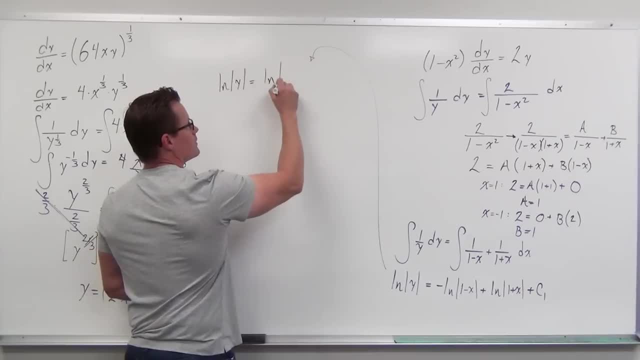 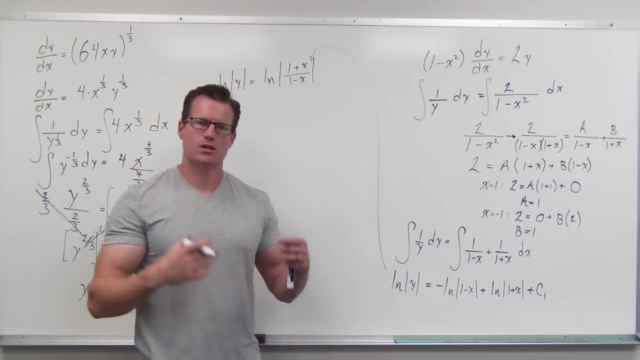 Because, if you can, then we can write this as ln of 1 plus x over 1 minus x. Two logarithms added or subtracted. Two logarithms added or subtracted create one logarithm with a product or a quotient respectively. This is technically subtraction. 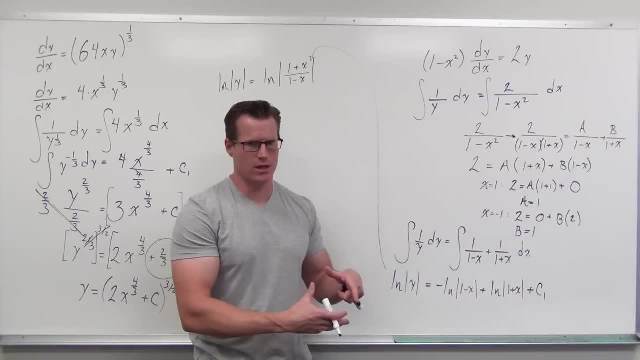 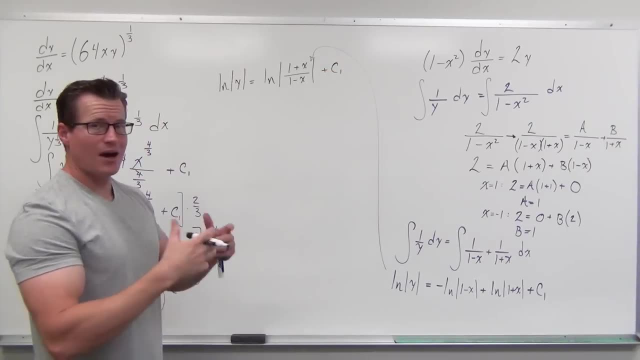 You have a logarithm minus another logarithm. Create a quotient out of that Plus a C1.. Now let's see if I don't forget my ln this time. So now that we have this written, we're going to try to solve explicitly for y. 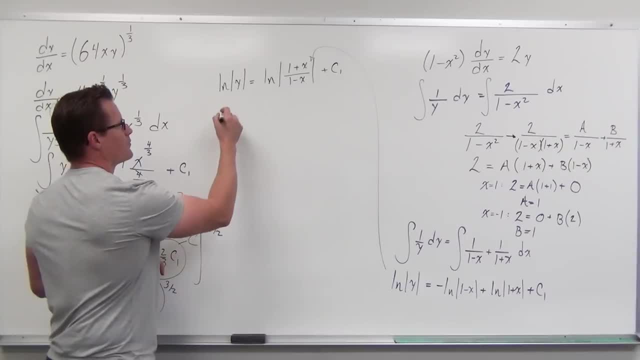 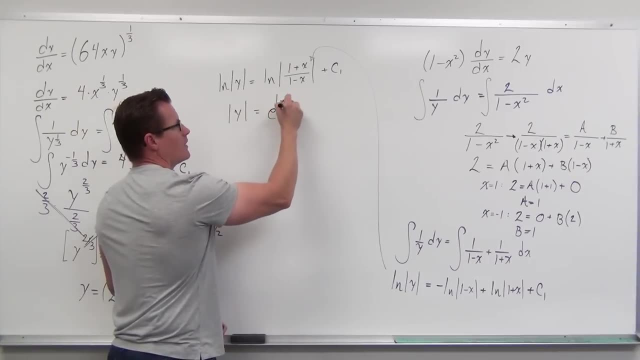 We're going to do that e to both sides. Well, we have e to ln of absolute value of y is just absolute value of y. e to the ln, absolute value of 1.. Oh my gosh, this is getting messy. 1 minus x plus C1.. 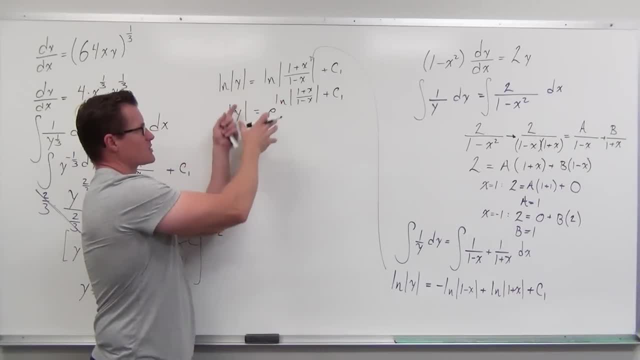 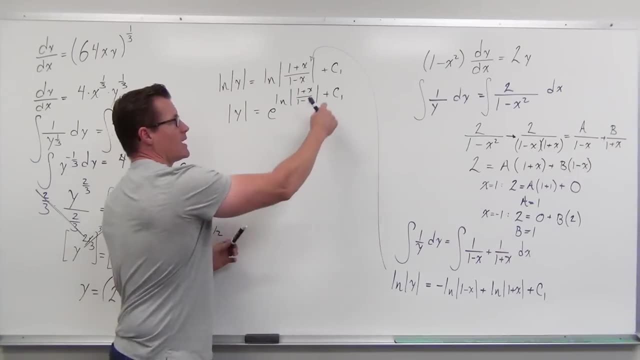 Let's go piece by piece through it. We did e to both sides. That's great. This is just absolute value of y, e to the right hand side. I've shown exactly what that is. Now you have this whole hey added exponents. 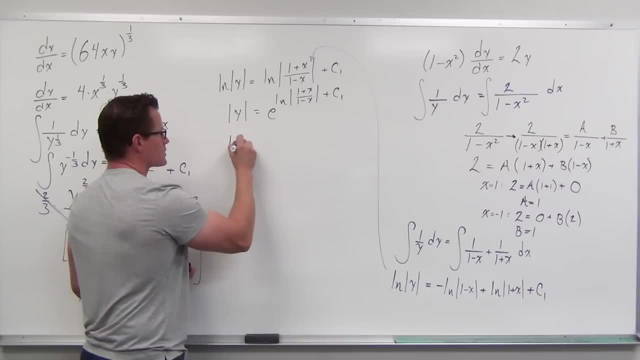 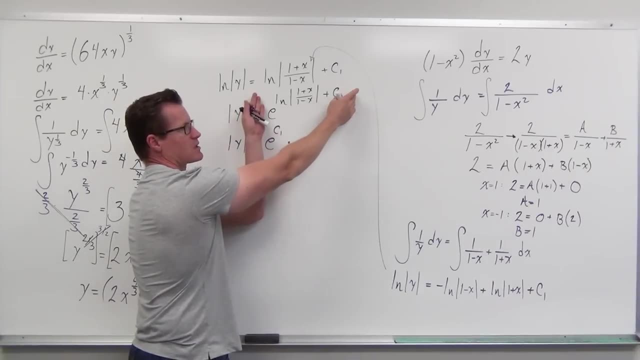 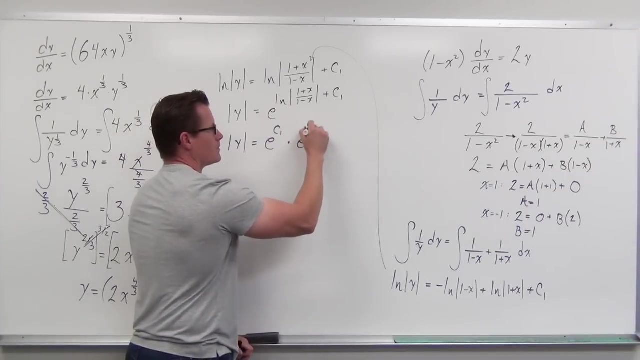 That's these common bases that are being multiplied. So absolute value of y looks good. We're going to get e to the C1.. No problem Times, because addition of exponents means that it came from multiplication of common bases. But we also have a composition of inverse functions here. 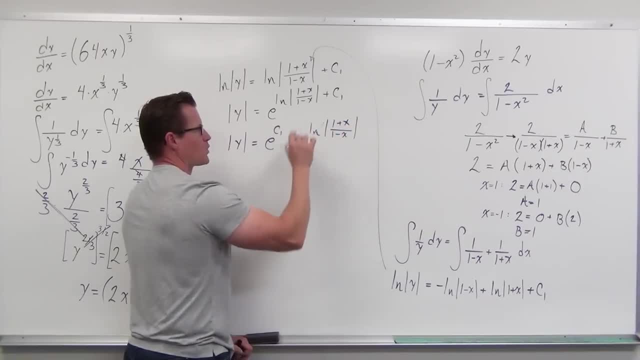 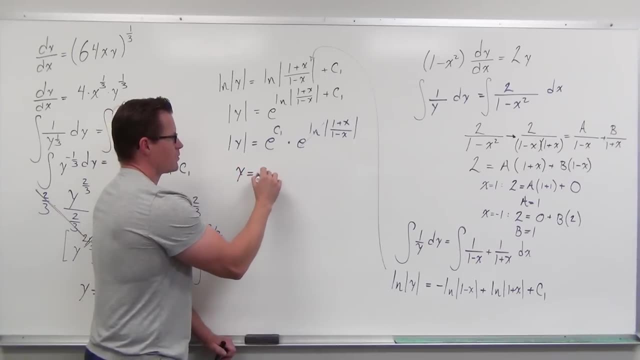 Those always go away, Gone. So let's do one more thing: Remember our absolute value. We don't want that. That's going to equal plus or minus e to the C1 times. Since that e and ln, they essentially cancel out. 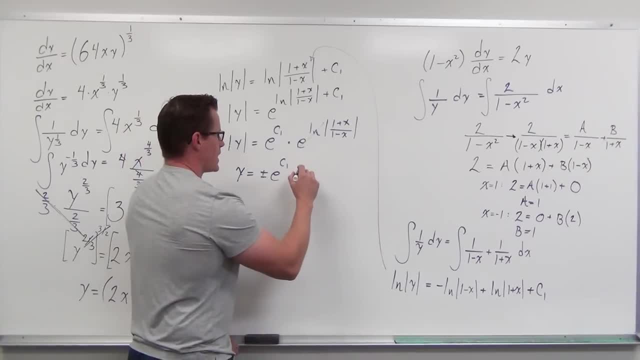 They undo each other. The inverse is there. We get just this: 1 plus x over 1 minus x. Let's wrap all of this up in a C. We're done. That's our general solution to that differential equation. That took a lot of work. 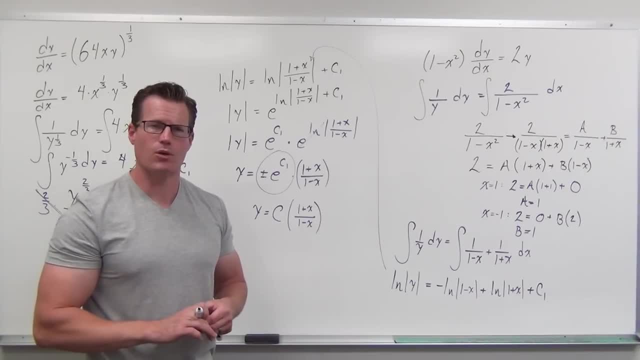 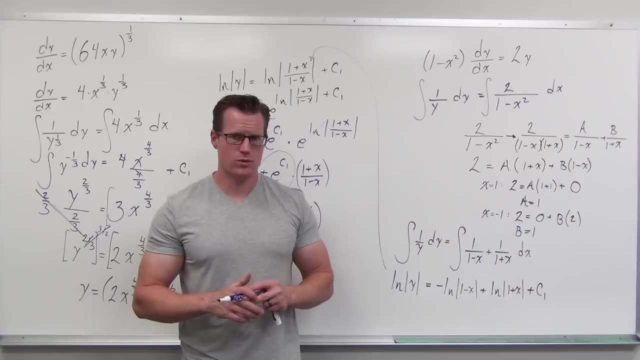 That's a lot of partial fraction stuff that maybe came out of nowhere. for you, When you see something and it doesn't fit and you go, how do I do that? Try to break it down. So we would try some basic things. 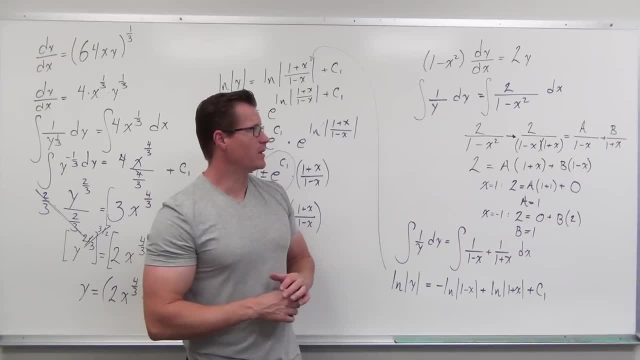 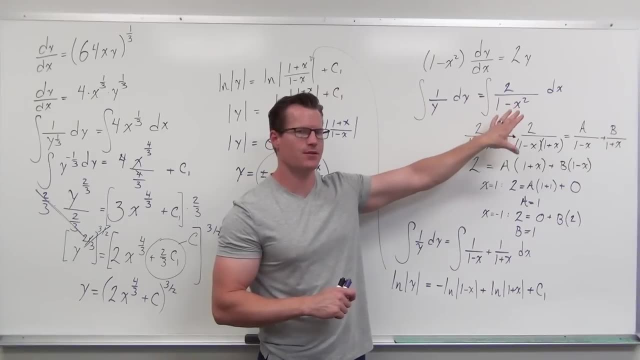 We would try ln a lot, But if you're getting something that looks like a trig sub or looks like something that you want to do for a trig sub and it's not fitting, maybe think about partial fractions. That might give you a hand. 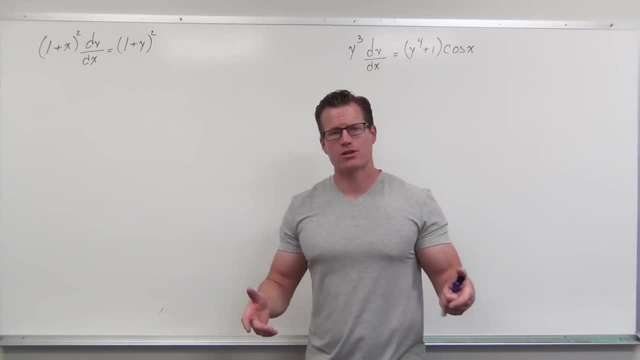 All right. So check it out through A couple more examples, a couple more integration techniques, making sure you see all that. So let's see if we can separate these variables, get our y's with dy, x's with dx. 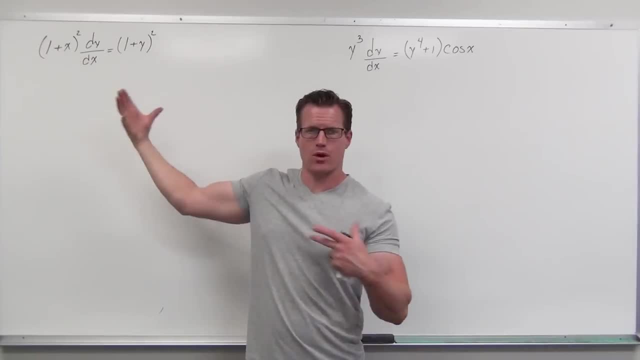 It looks like we can. If you were to move this over here, you'd have a product or a quotient. That's what we're really looking for. We don't really want to have to do that. We're going to do a lot of stuff at once. 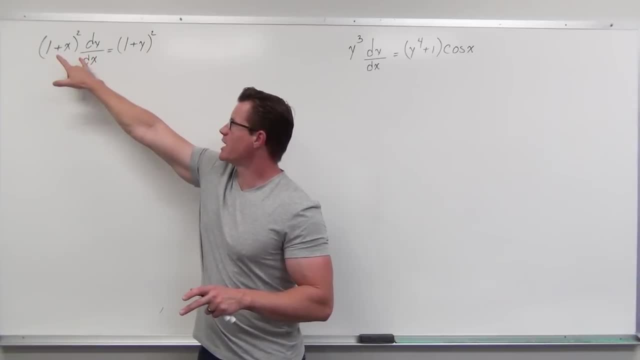 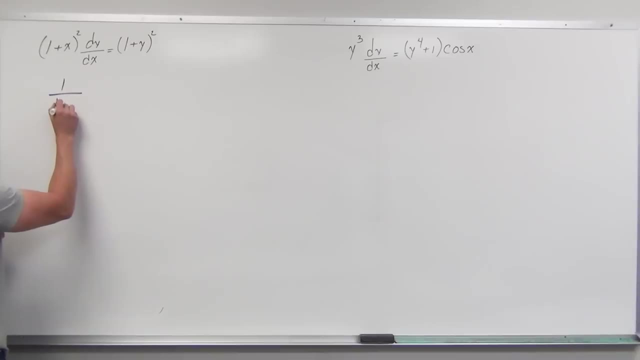 So we're going to divide both sides by 1 plus y squared. Divide both sides by 1 plus x squared and multiply by that dx. You know, at this point this stuff should just be kind of popping up in your head and go: yeah, I'm getting that. 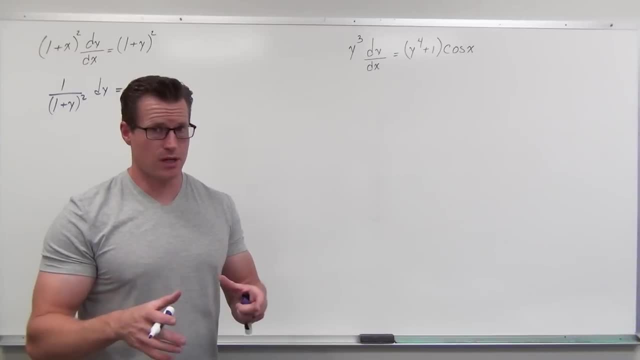 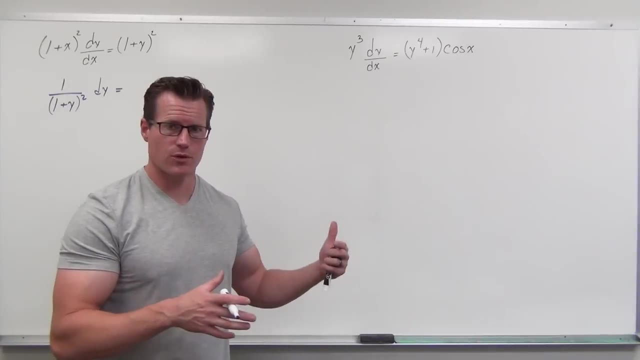 If that's great. if that's happening, that's great, That's really good. That means you understand the idea at this point, So that's perfect. You might want to just go and try some on your own right now, before we go any further, and see if you do run into a problem. 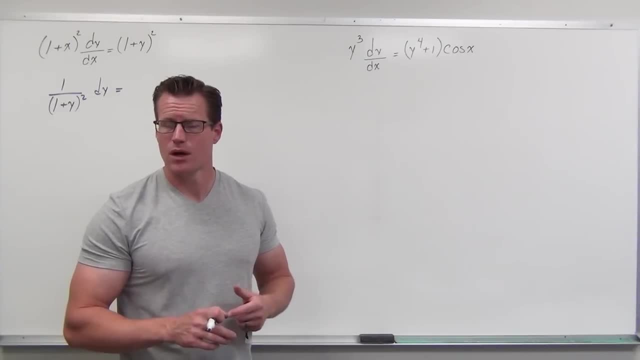 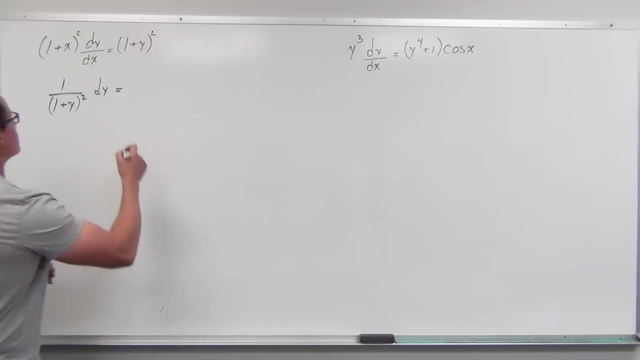 Maybe I'm going to cover it on these techniques also, But if you're getting it, man, I'm proud of you. That's excellent. You're solving differential equations. It's pretty cool. So y's got to divide. 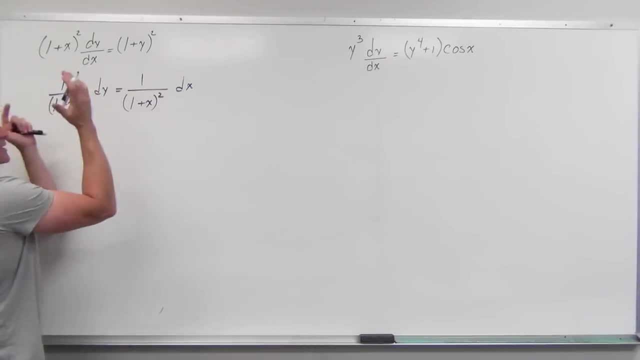 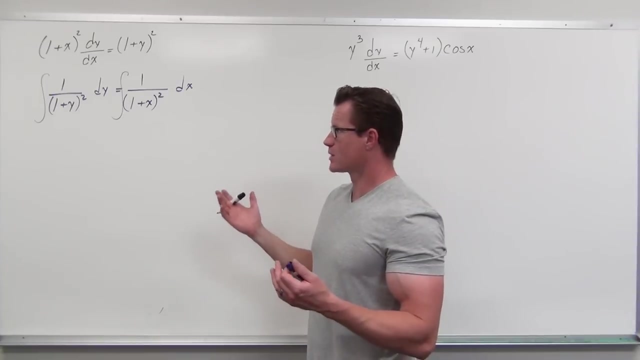 X's got to divide, We've got to get our dy on one side, dx on the other side, And now we're ready to integrate. Then we see that that doesn't really look like anything that we've seen before, at least not yet where it's not really a ln. 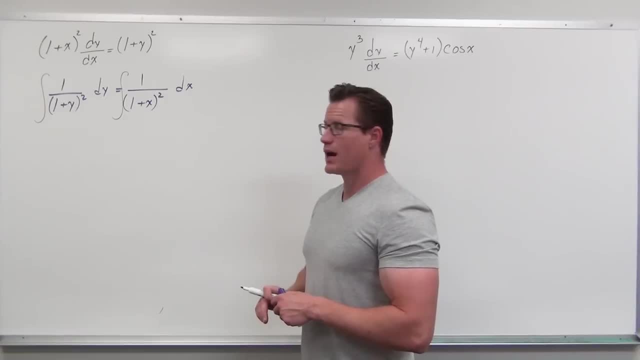 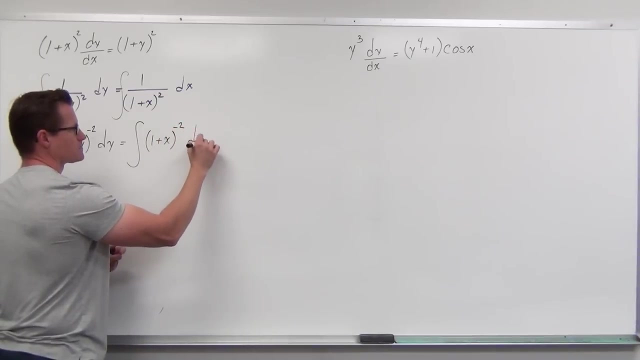 Man, I really don't want to have to do partial fractions- And it's not partial fractions, But just remember that when we have some simple linear inside of a power, oftentimes we can rewrite this and do a very simple u sub, if that. 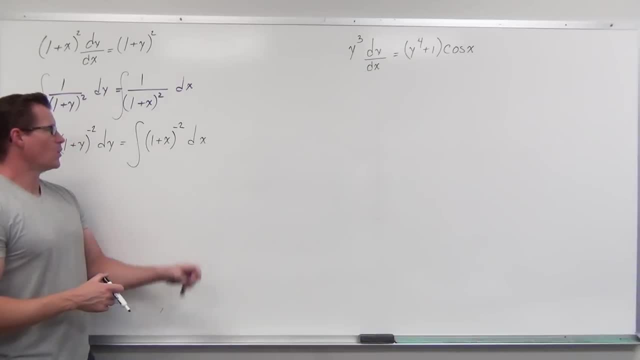 So they're the same integral twice. On the right-hand side we have well 1 plus x to the negative 2 power. If you called that, u you would get. You would get u to the negative 1 over negative 1.. 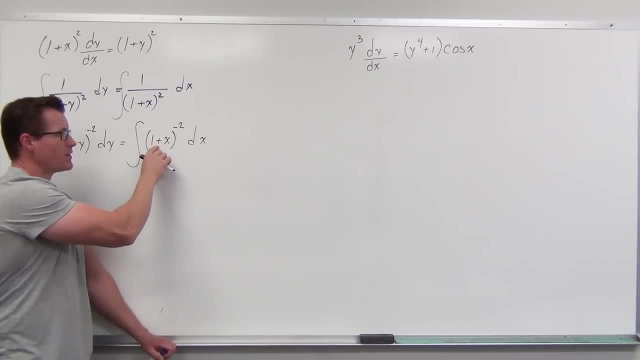 So negative u to the negative 1 divided by the derivative of that. But the derivative is just 1.. So if u equaled 1 plus x, then du equaled dx. That's just a straightforward substitution. That's excellent. 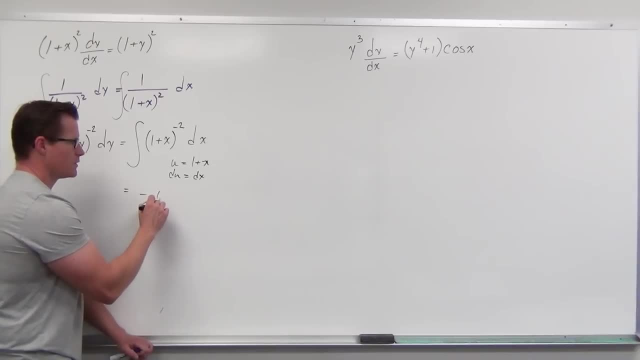 We would just get negative u to the negative 1.. But then we have 1 plus x being our u, And we're going to have a constant. Left-hand side is going to behave exactly the same, So let's make this a little bit nicer. 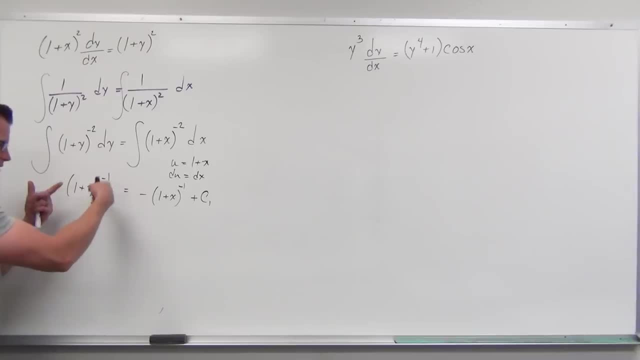 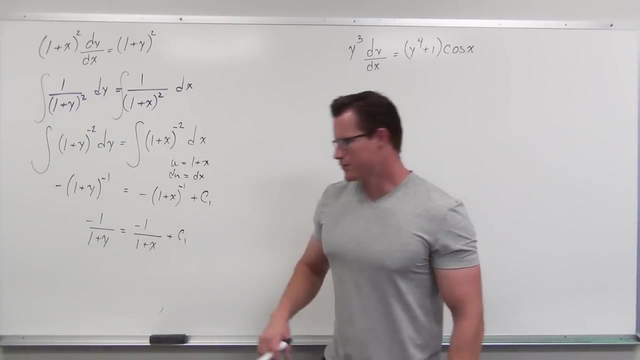 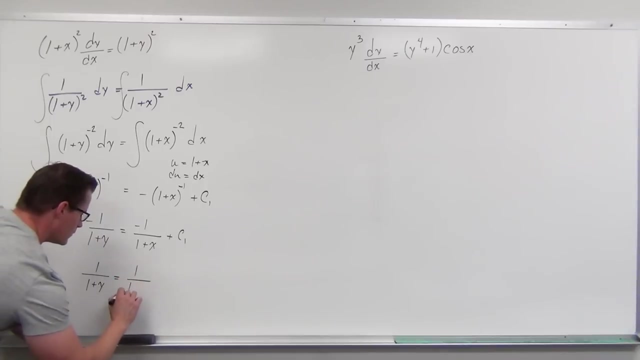 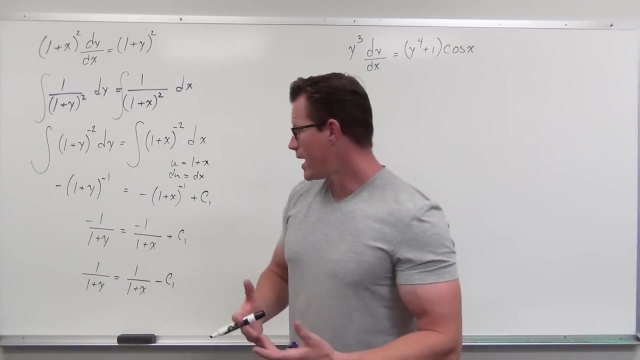 Right now it doesn't look very nice, So let's make this over a fraction, You go. well, that doesn't look nicer either. I don't really like the negatives, So let's multiply everything by a negative. Now we're going to have to solve for y. 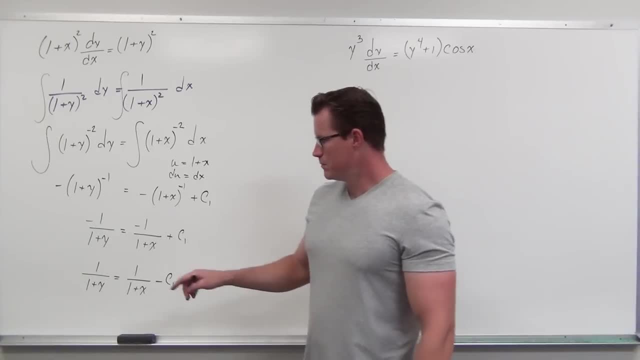 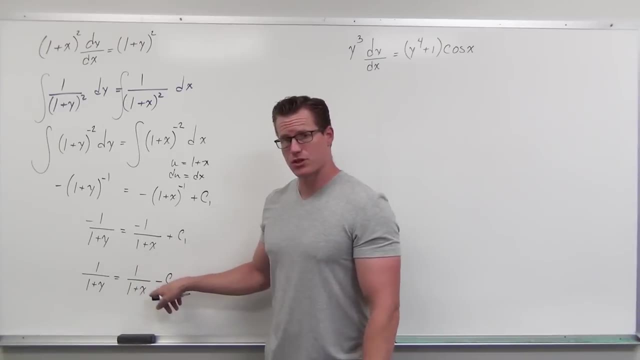 So how in the world are we going to do that? It would help- Here's the thought process. So it would help if this were all one fraction, Because if it were, then I could reciprocate both sides And then y would be on the numerator. 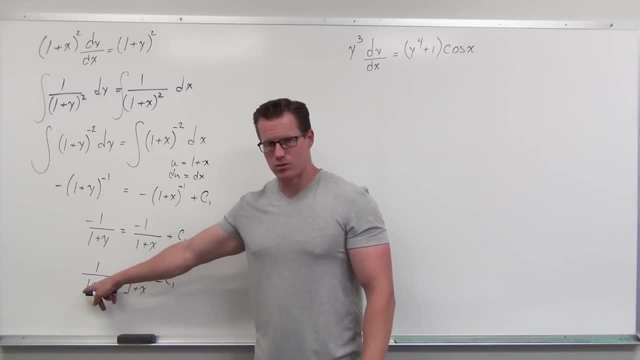 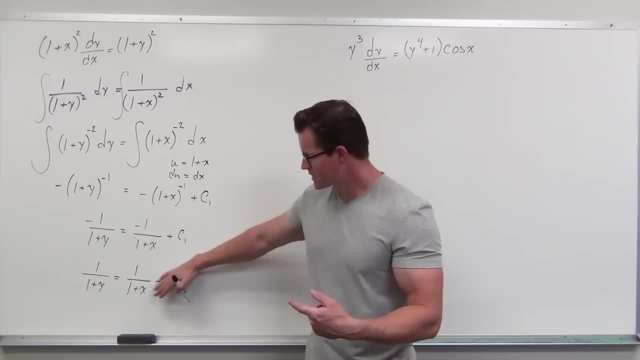 And all I would have to do is subtract 1.. Right now I can't really subtract 1.. So I want some mechanism where I can just reciprocate and reciprocate. I can't do it because of that. If that wasn't there, it would be easy. 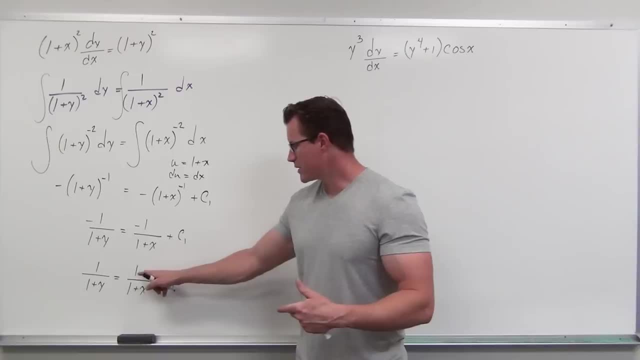 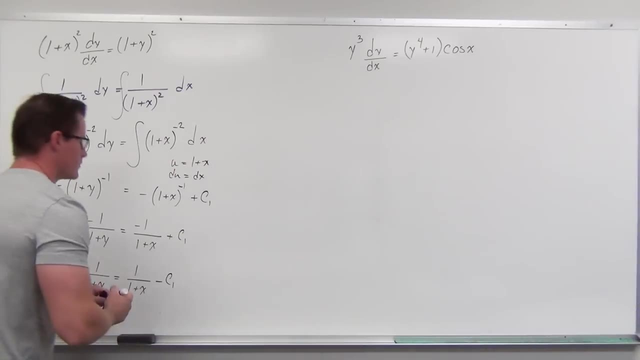 But I can't do it because of that. So let's find a common denominator here, Let's make one fraction, And then we're going to reciprocate. So 1 over 1 plus y, Because that's just a constant over 1,. 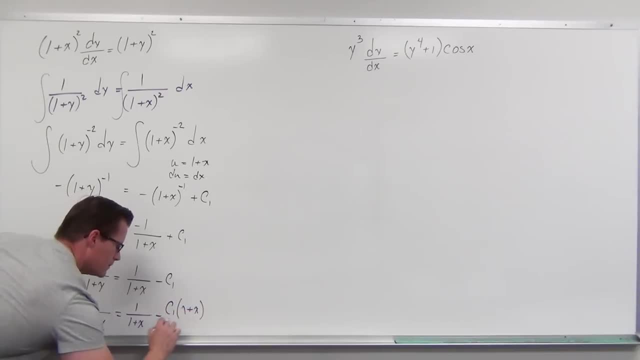 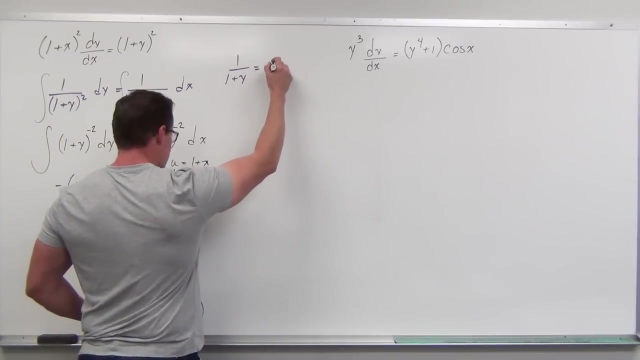 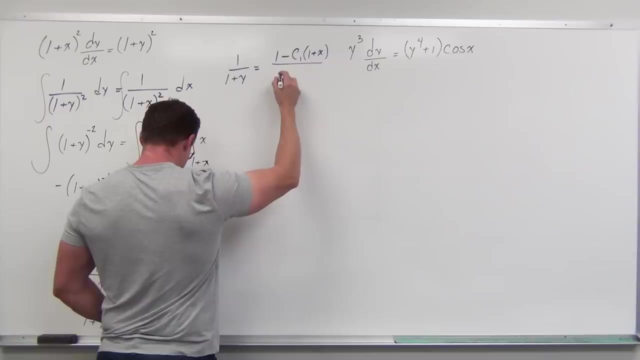 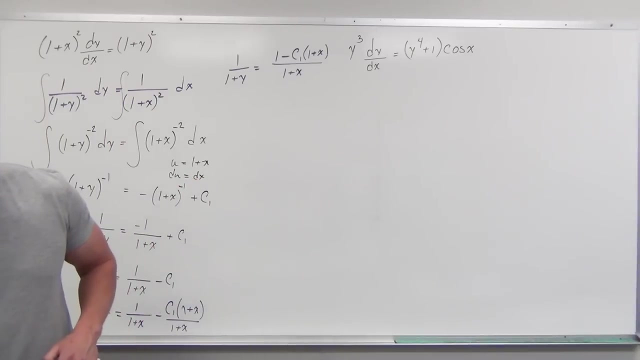 all we really have to do is multiply the numerator and denominator by 1 plus x, And then, when we join that together, that gives us something that we can actually reciprocate, And that's what we're going to do right now. So let's try it. 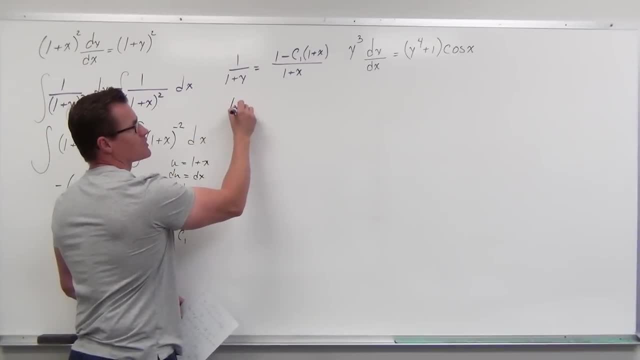 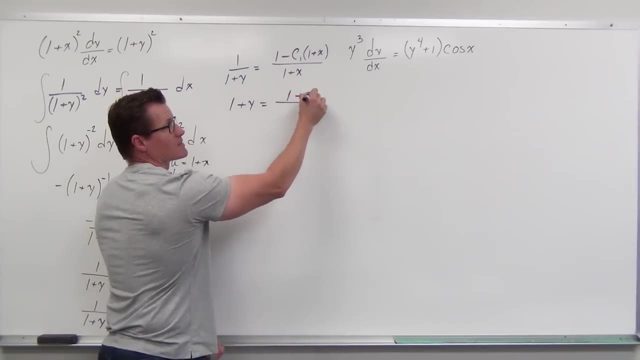 So if we reciprocate this, we have 1 plus y on the left-hand side. On the right-hand side we flip that fraction over. So x plus 1 or 1 plus x is on the numerator And 1 minus c sub 1.. 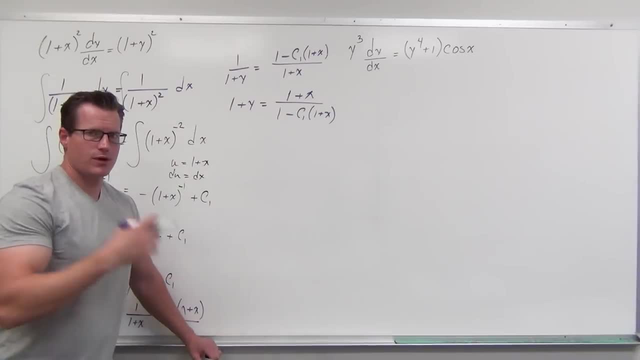 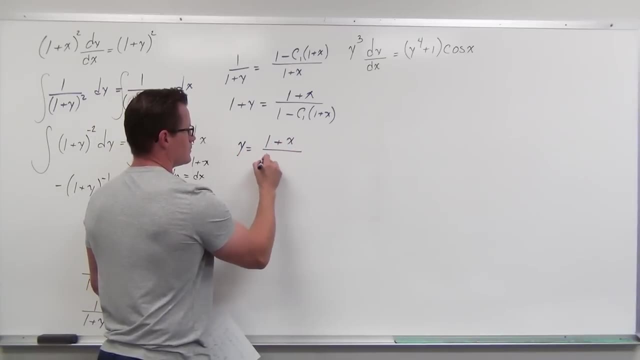 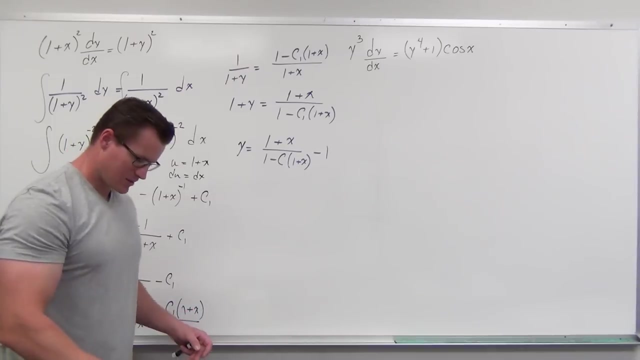 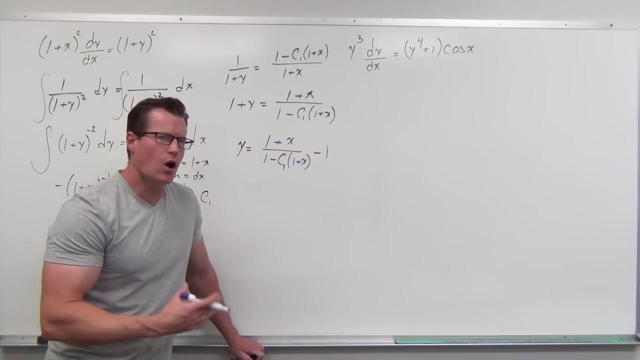 My 1 plus x is on the denominator, So we just reciprocate And then all we've got to do is subtract 1.. And that's good enough. I don't really want to leave this as c1.. So a lot of times, lots of times. 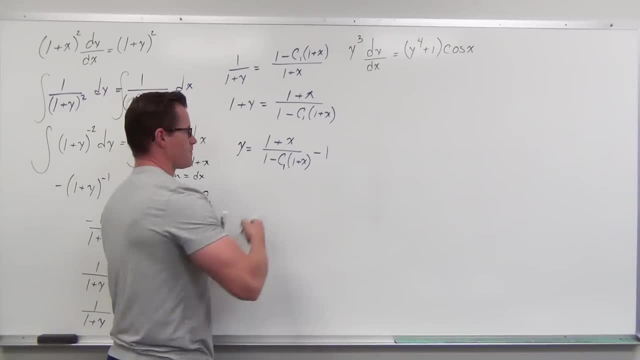 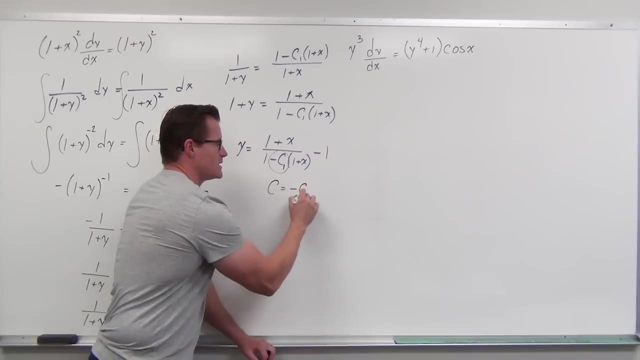 what we're going to do is we're going to call this piece that piece, with the sign we'll call c equal to negative c1.. That way we get rid of a minus sign and we get rid of that little subscript of 1.. 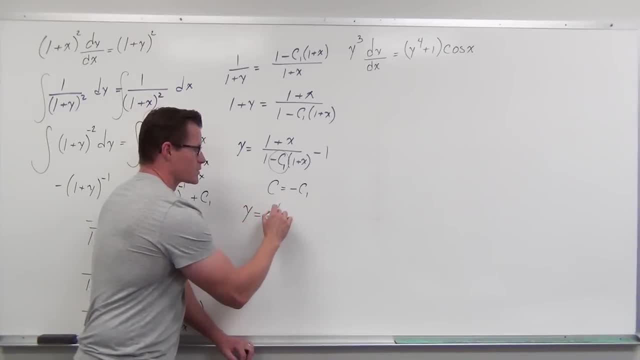 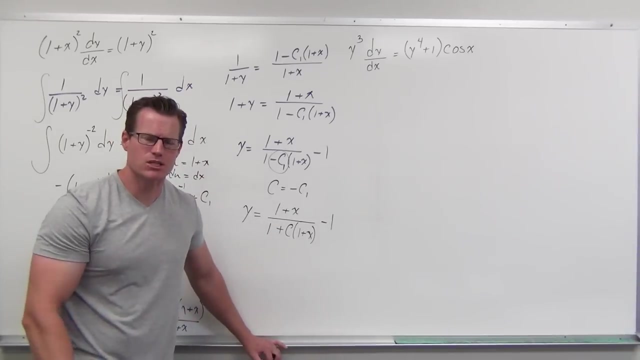 So if I call that negative c1, then y equals 1 plus x over 1 plus c, 1 plus x minus 1.. If your signs are wrong, like here, I did everything right. Darn you Leonard. 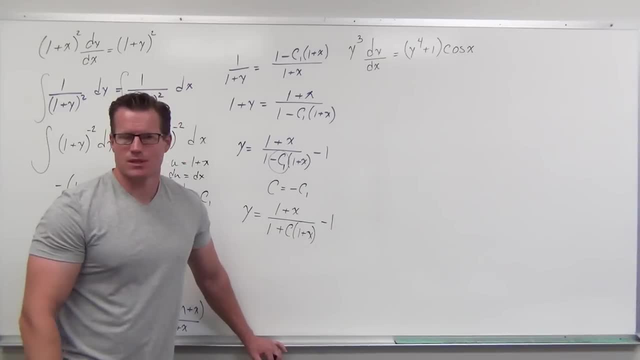 Don't darn the Leonard man. It's probably something like that, So don't worry about it. Don't get super frustrated if your signs are wrong. If it's revolving around a c, they're probably just redefining it. 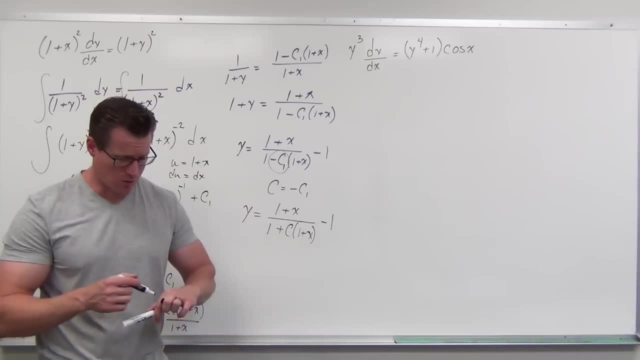 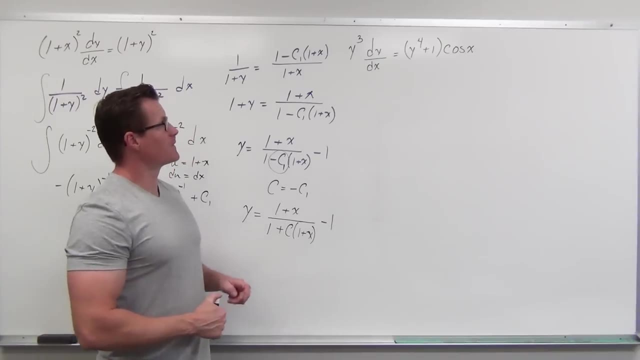 It happens a lot. That's it. It's nasty, That's a horrible looking answer, But that is a general solution to that differential equation. That's kind of cool. So let's do this last one before I give you some other ones. 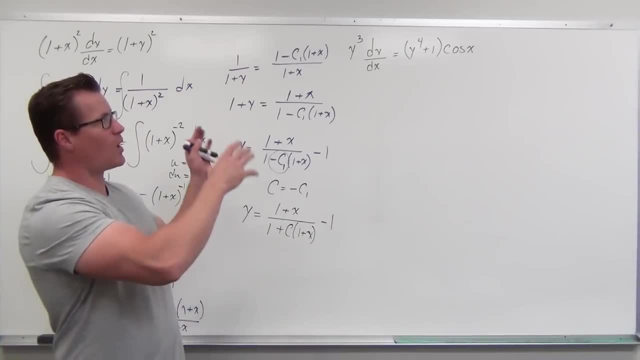 They're a little bit more advanced. So we got some y's. Hey, there's already y's on one side. We got some x's. They're already on the correct side. All we've got to do is move the rest of the y's. 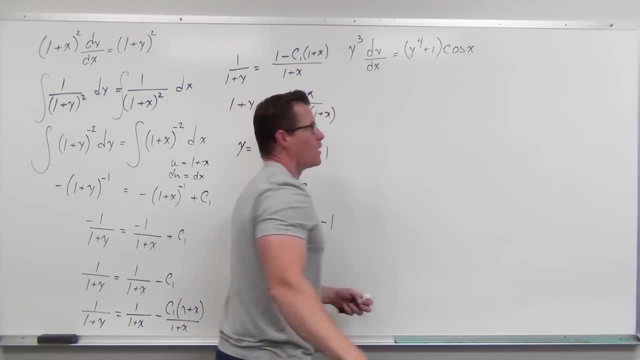 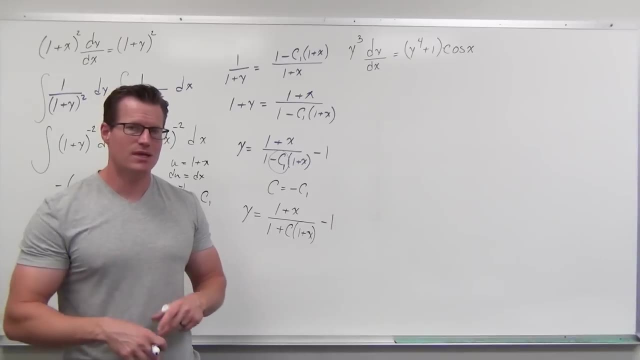 that's connected by a product on the left-hand side. Why don't you try that? See if you can go through it. Look at the left-hand side, See what you get. Look at the right-hand side. Maybe do that simple integral that you have. 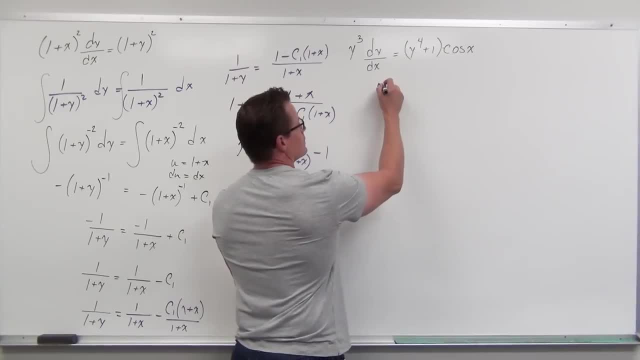 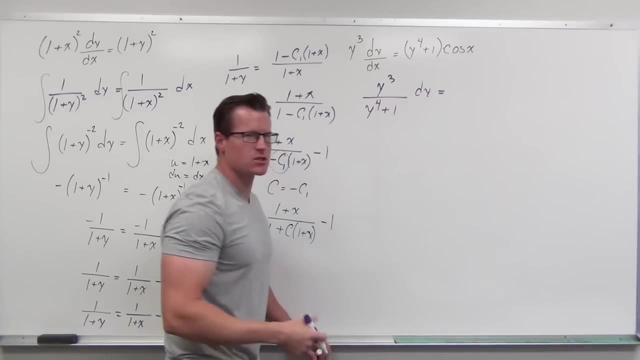 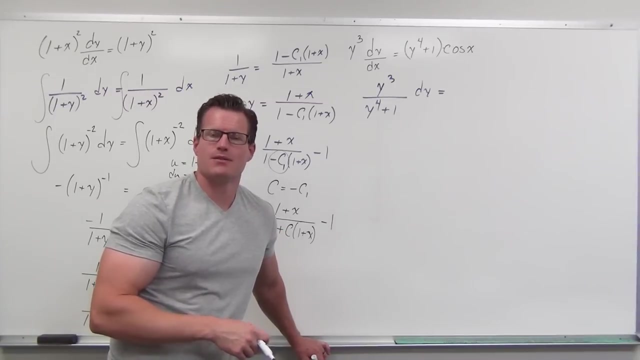 and see if you can practice that. I really hope you're doing that when I suggest it, Like, hey, give this a try, Because while watching me do math is super exciting, it's not benefiting you if you're not internalizing it. 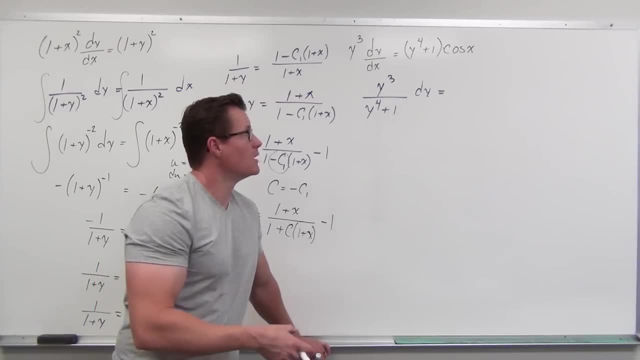 So one way that you can get better at this is: before I try the problem, try the problem. If you can do it, you don't need to study that problem anymore. If you can't, you need to watch me, That's okay. 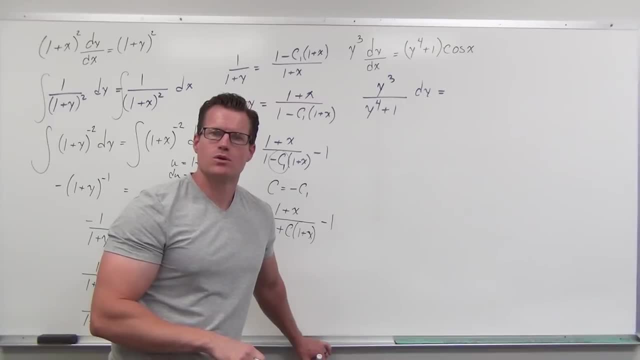 You're still learning it, But at the end, try again, See if you can do it after you've learned it And make sure that you have learned it. If not, try it again. Okay, And see if you can watch the video. 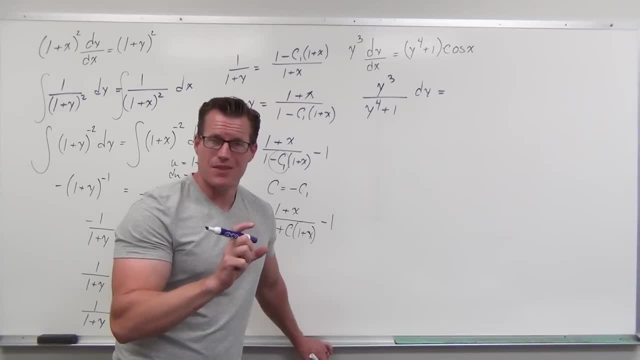 and pick up the small piece that you're missing. That's a good way to study, So don't just watch it all the way through. While beneficial for a little bit, it's not internalizing it, And I want you to know it. 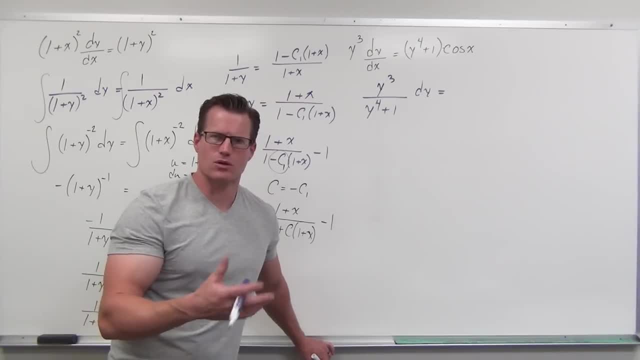 I don't want you to struggle with this stuff when you're in your class or learning it so much that you get mad. Getting mad at math is never helpful. It's like two people who are having a discussion and then they start yelling And then at that point no one's listening. 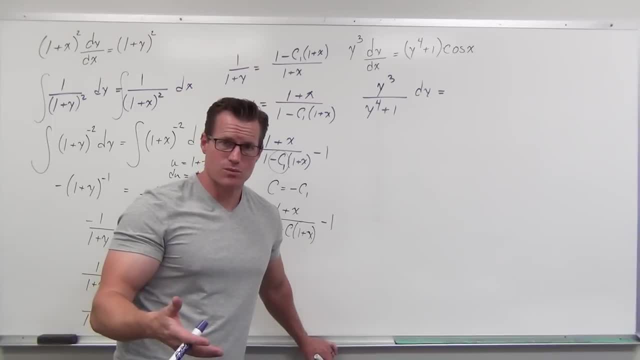 It's just beating your head against the wall. Frustration can produce perseverance and character. sure, It makes you a stronger person by having to go through trials like learning math. It's definitely a trial, But make sure that we're actually using our time wisely. 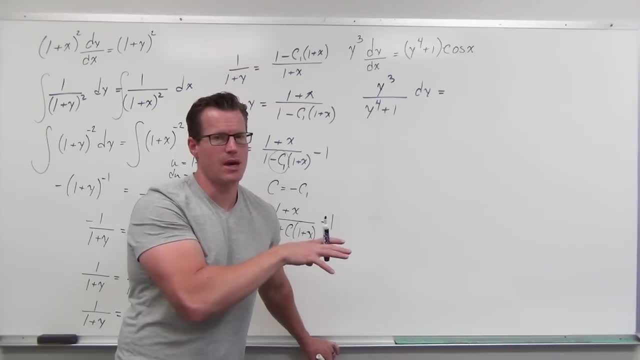 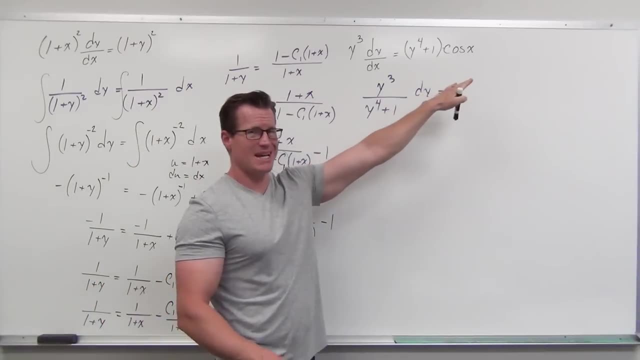 So one part of that is not just watching the videos but trying them out. Make sure you're trying them out. So on the left-hand side, we've divided by y to the fourth, plus one We've multiplied by dx. I haven't shown that yet. 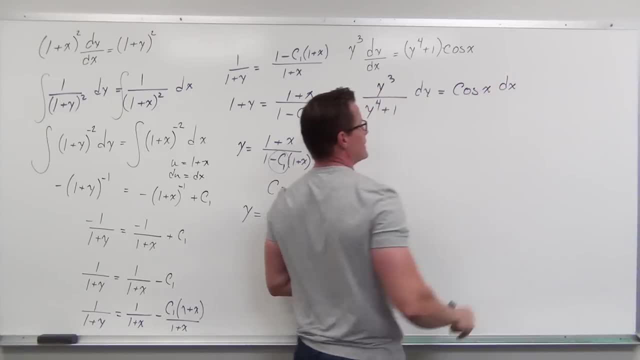 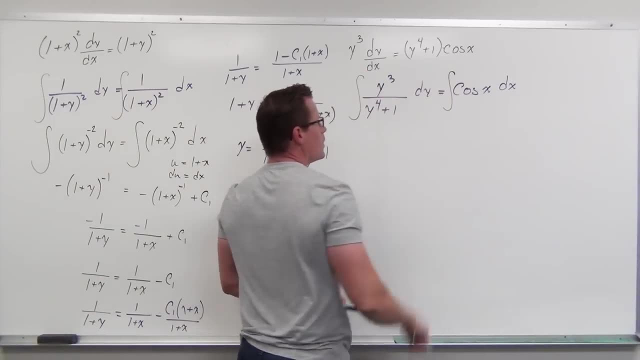 We have a cosine x and then a dx. Hey, we're ready. We're ready to do an integral, So we're going to integrate both sides. On the left-hand side, y cubed over y to the fourth plus one. 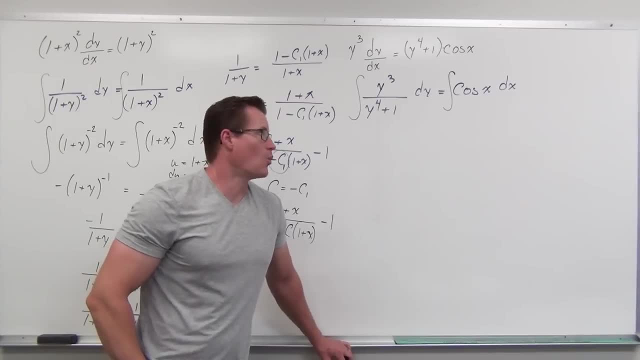 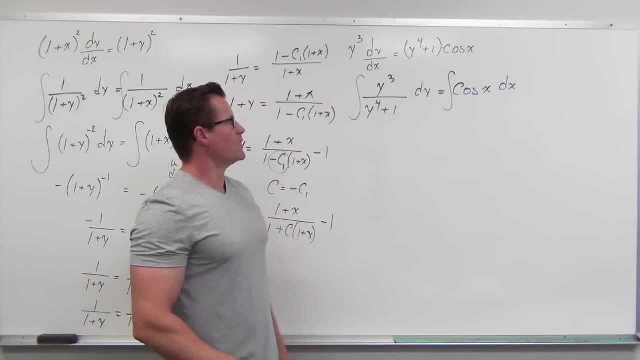 whenever your exponents on the numerator are one less than the exponents on the denominator. you're talking about a u sub and then an ln, And then you just have one term. So right here we're going to say: hey, u is y to the fourth plus one. 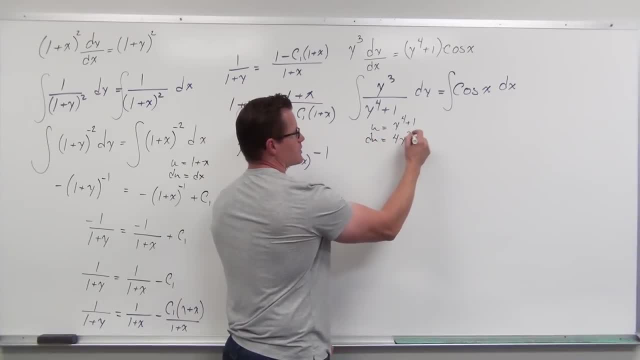 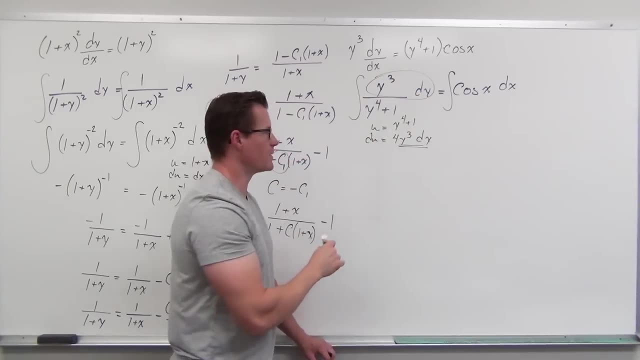 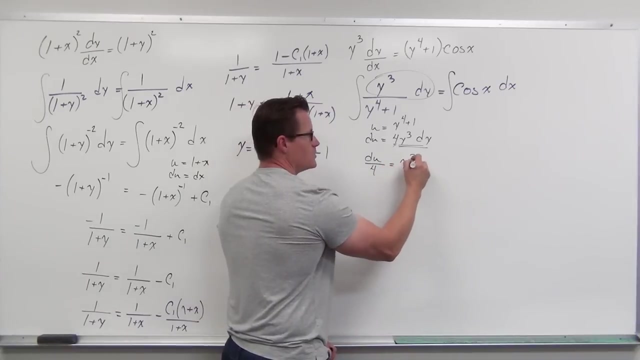 du therefore has to be four y cubed. Oh, that's perfect dy. This part matches this part. We're going to do a substitution. We do want to get rid of this constant right there. So du over four equals y cubed dy. 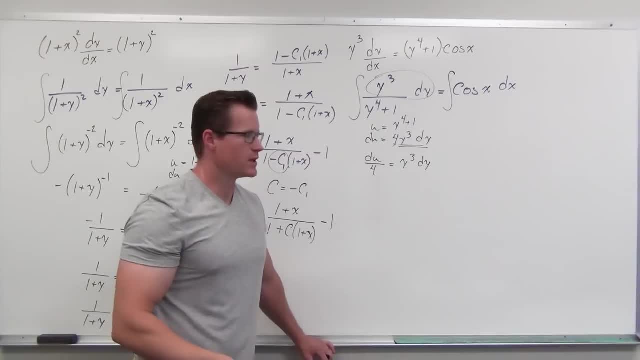 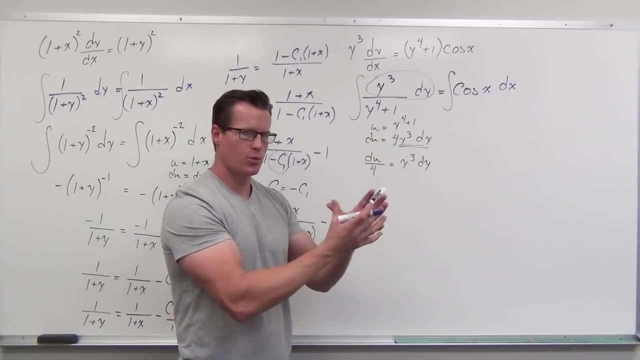 I've done this many different ways. I've shown it lots of ways in the videos. This is the one that lots of people prefer. You're looking for the piece that's the same and you're going to replace that whole piece with this stuff. 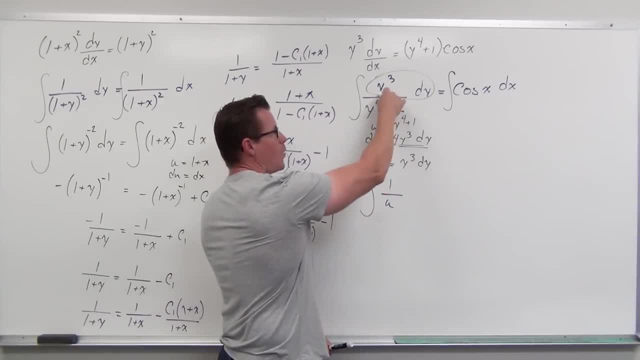 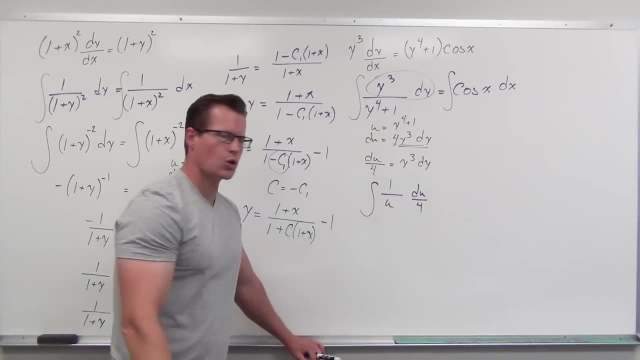 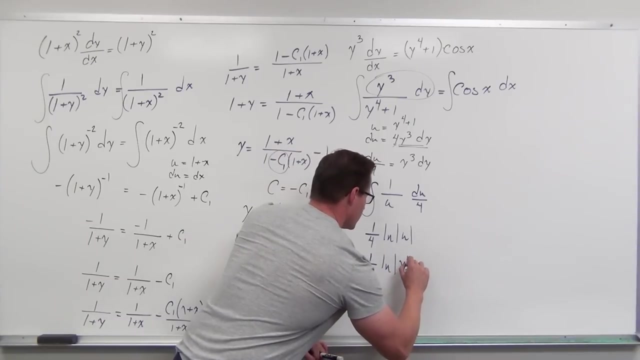 So y to the fourth plus one. we call that u y cubed dy. that whole piece gets replaced with du over four. No problem, because we know that we can just do a one fourth ln absolute value of u. We know what that is. 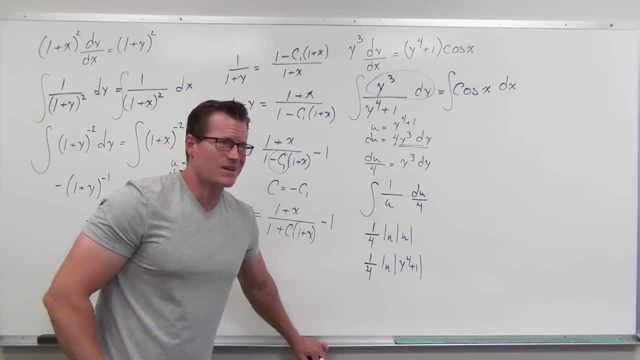 y to the fourth plus one. Let's talk about y to the fourth plus one. Is there any possible number you can plug in? That's not imaginary, That you can take to the fourth power, add one and get a negative, Then that absolute value is irrelevant. 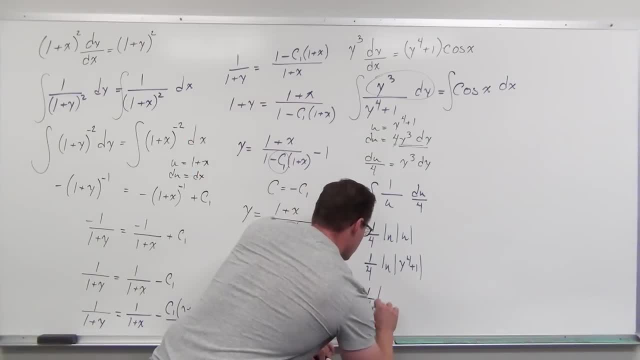 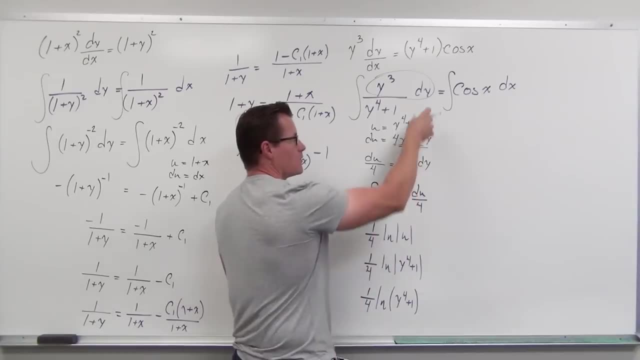 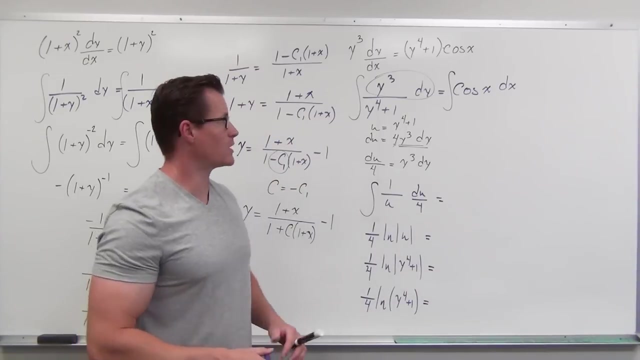 So we're going to drop that Now. we've just done a whole lot of work. All this was a use of. Let's see what's on the right hand side, So integral of cosine x. The x side happens to be an easy one here. 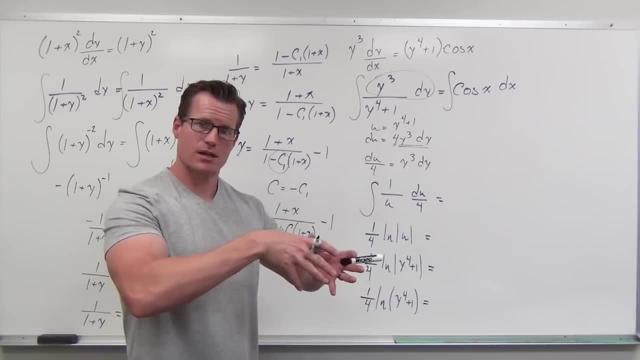 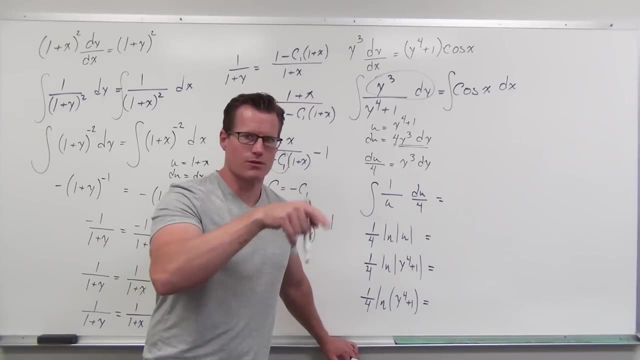 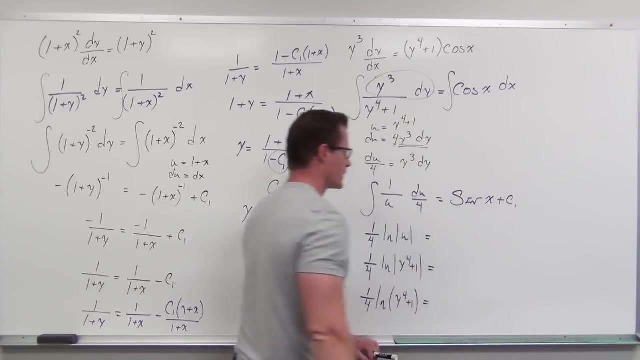 That's sine x. The derivative of sine x is cosine x, So the integral of cosine x is the integral going backwards is: Did I say that right? The derivative of sine x is cosine x, So the integral of cosine x is just sine x. 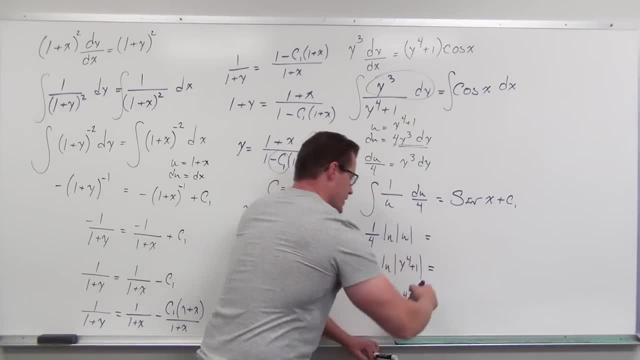 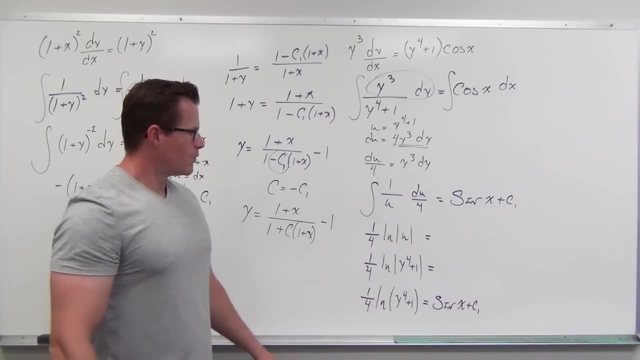 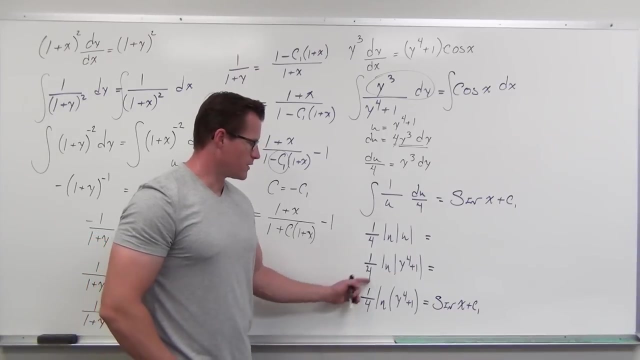 Plus c one, And that's going to follow us all the way down. Well, we definitely want to get rid of that one. fourth- And you do have options. Let's talk about what the better option would be. Would you want to create a fourth root? 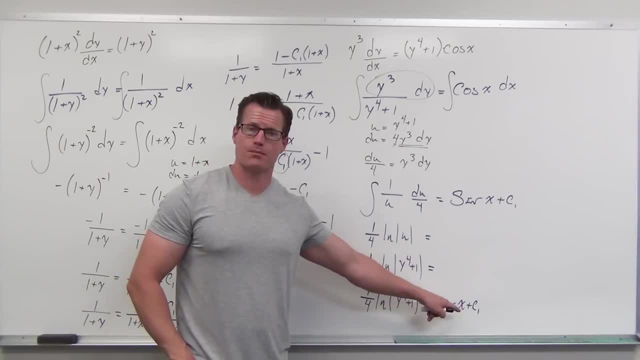 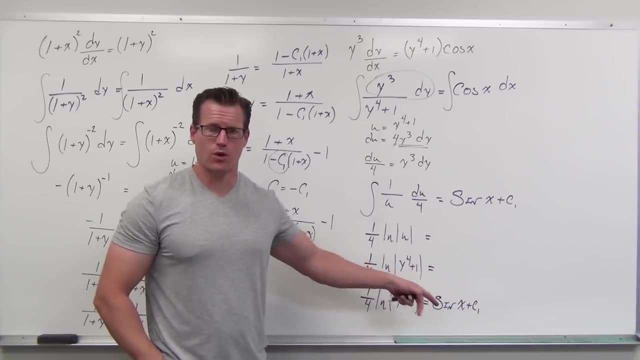 on the inside of a logarithm. Or would you rather just multiply both sides by four? Since we're trying to get as close to solving for y as possible, it's more beneficial to multiply both sides by four and at least remove that fraction. 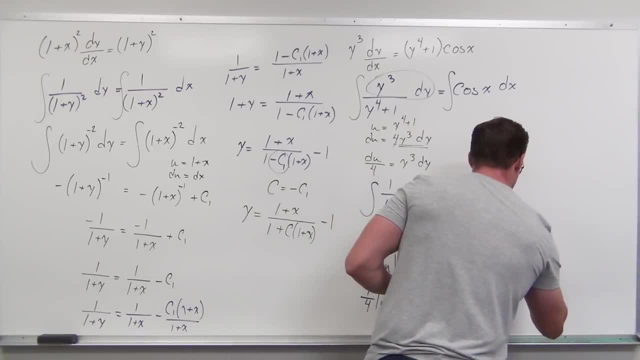 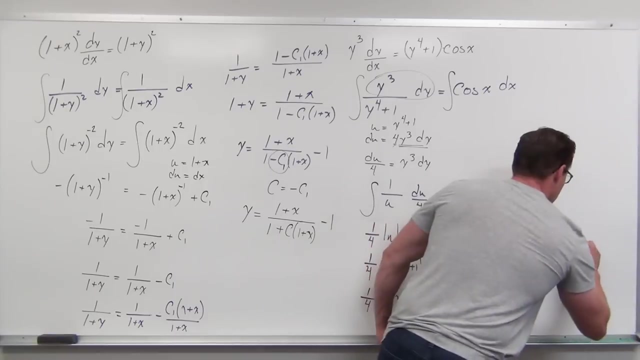 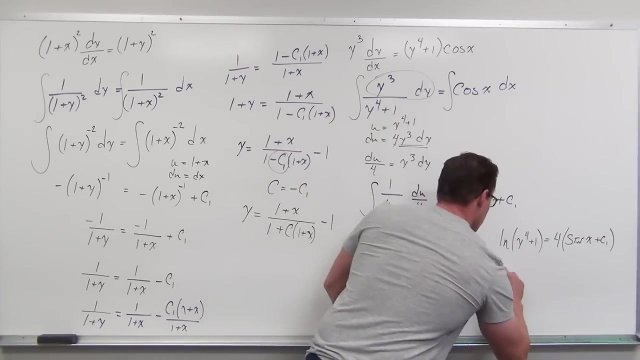 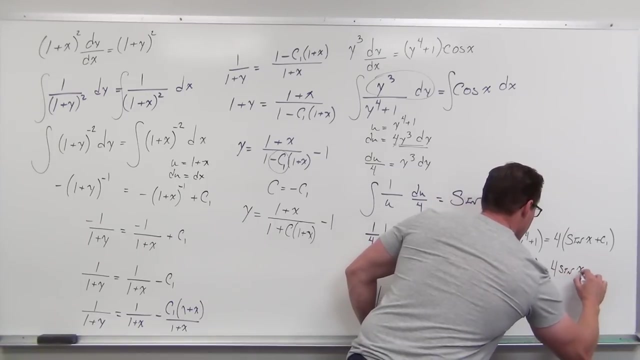 So we're going to get this whole ln y of the fourth plus one equals four, And we just want to write it like this: Four sine x plus c. If you do want to distribute, then we're going to replace that four c one. 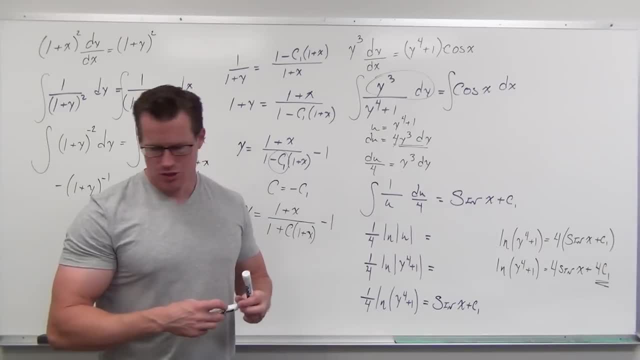 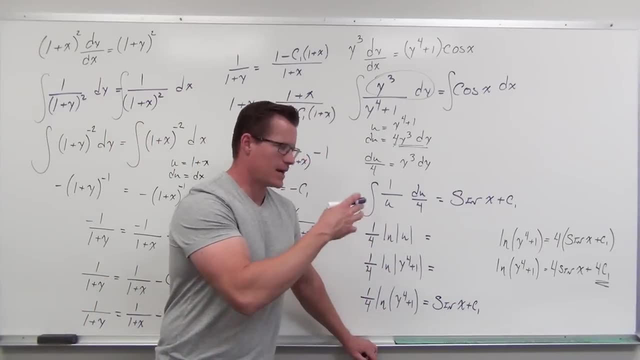 with just the arbitrary constant, And you can do that on your own. This is one that we really. we really want to start solving that for y. So we have to do an exponential on both sides. That's not fun, And then we'd have to subtract one. 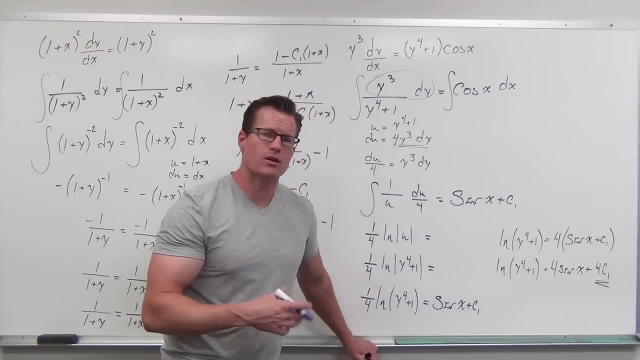 And then we'd have to take a fourth root. That's just too much work. So this is one of those cases where you're going to see it left implicitly. You're not going to be solving this for that y Especially since we get the whole non-function issue. 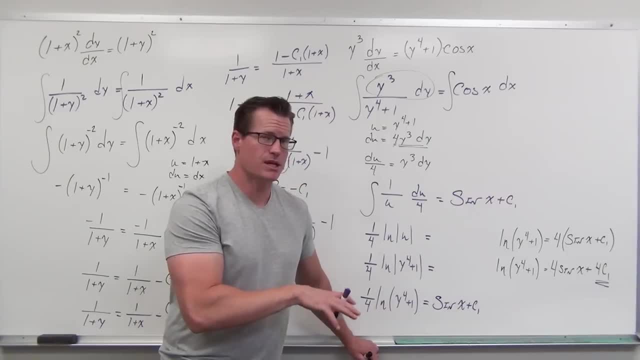 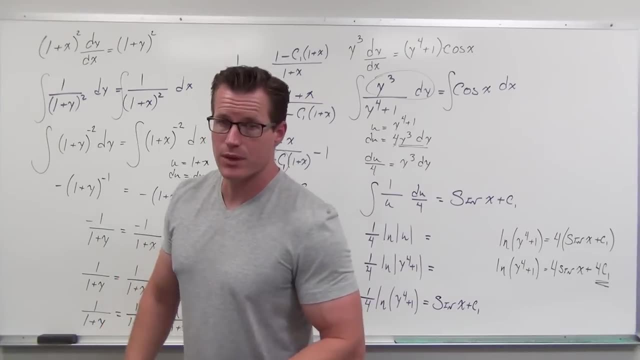 with the plus and minus when you take that fourth root. So anyway, I hope that's making sense. We have like four more to do. The last one again is probably pretty important for you to see, So don't skip out on the video without watching that. 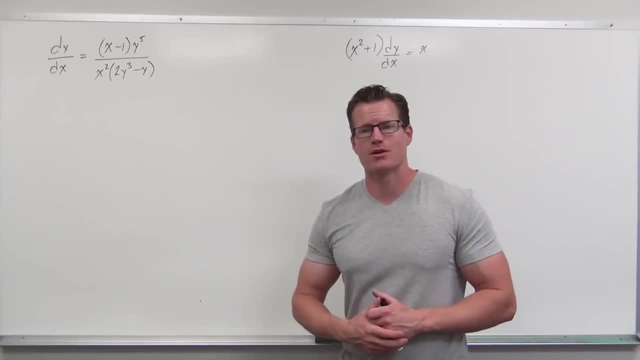 Okay, so two more Again. I am going to encourage you to try them on your own. See if you get stuck. If you do, that's okay. You're still learning it. It's probably an integration technique. If you're not getting stuck, that's awesome. 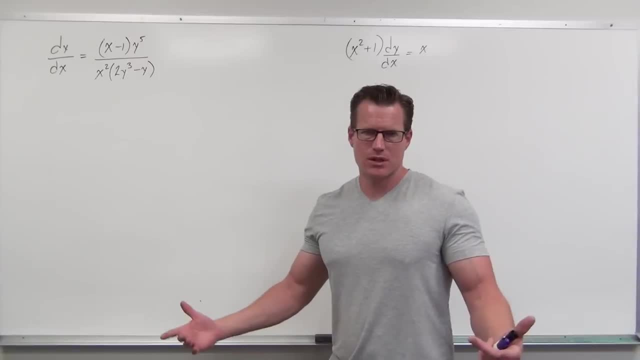 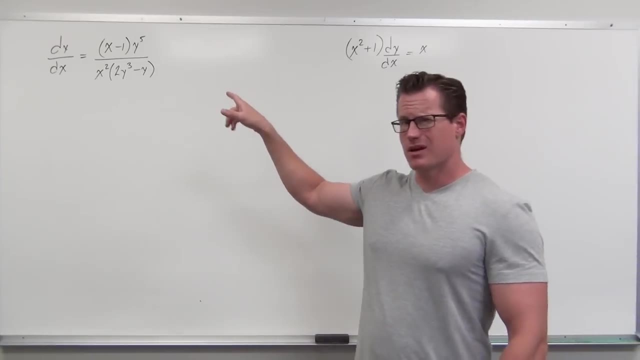 That should build your confidence. You guys should be really good at this, because you're putting in the time. You're already watching the videos. That's like number one, So perfect. So, as I was rambling, you'd probably hopefully pause the video and do that. 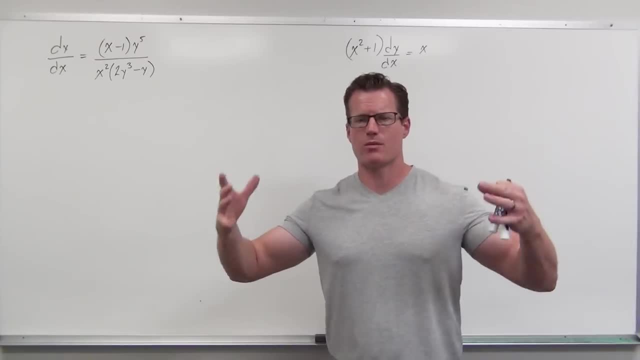 If not, we're going to get going right now Again the idea. I'm going to try to model my thinking here for you To get it in your head just a few more times. I'm kind of trying to brainwash you into doing it my way. 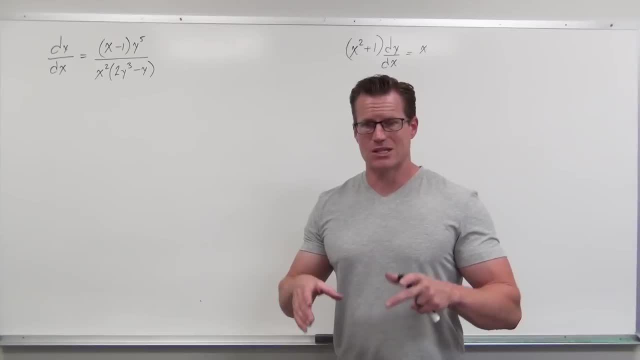 or separable equations. way here. Your first order of business is to look for separable equations. See if you can make it fit that. If you can't, it's just a matter of integrating and then solving for y, which is nice. 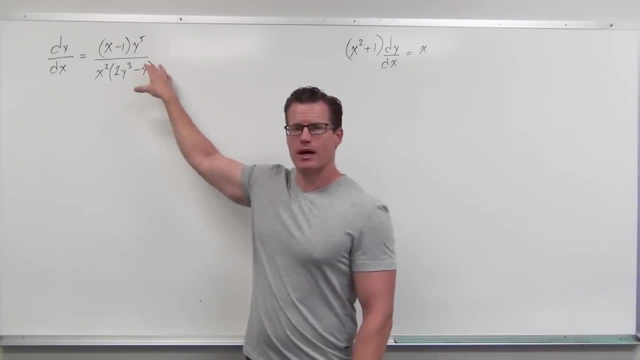 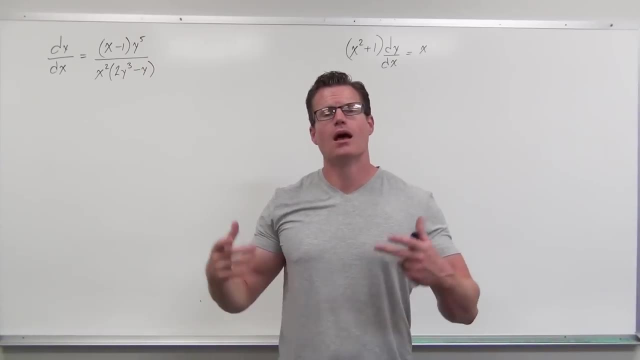 So here we have everything that's multiplied and divided. That's fitting. the model of differential equation equals separable equations or separable variables. in the right-hand corner, Let's get the y's on one side. Let's get the x's on the other side with a dx. 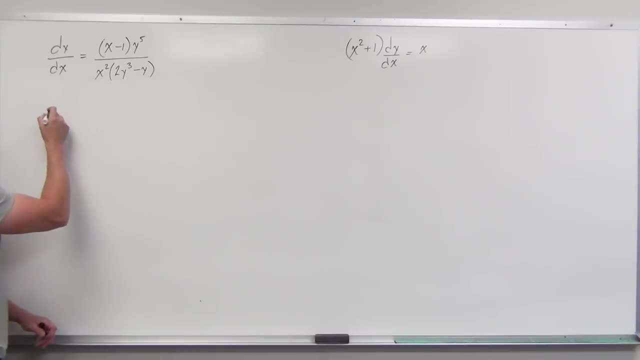 So that's got to move. So we divide. This has to move, So we multiply. On the right-hand side, all of our x's can stay. Nothing would need to move there. Now we've grouped our y's, dy's. 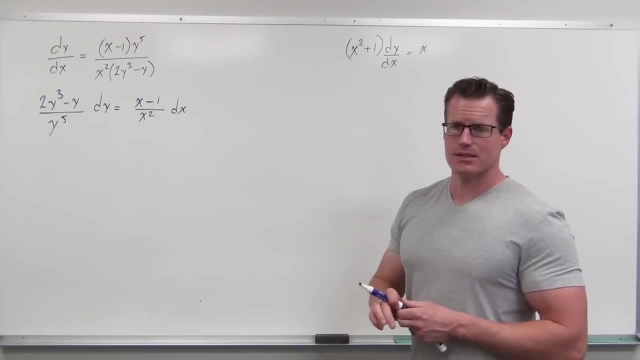 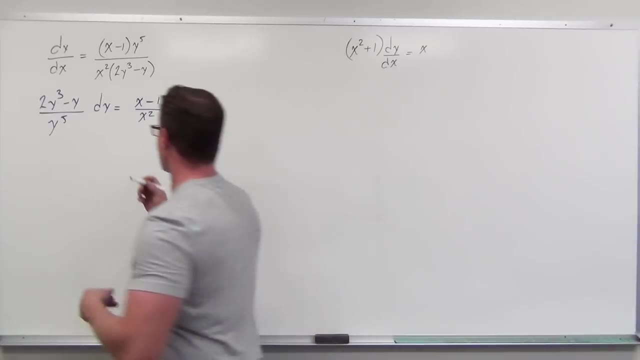 We've grouped our x's, dx's. It does not look very nice, does it? Well, not very nice, to me at least. But let's go through the process of seeing our integral. Just by writing the integral. hopefully, a little psychology comes into play. 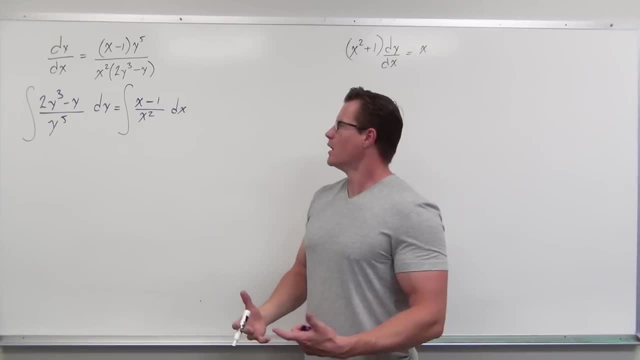 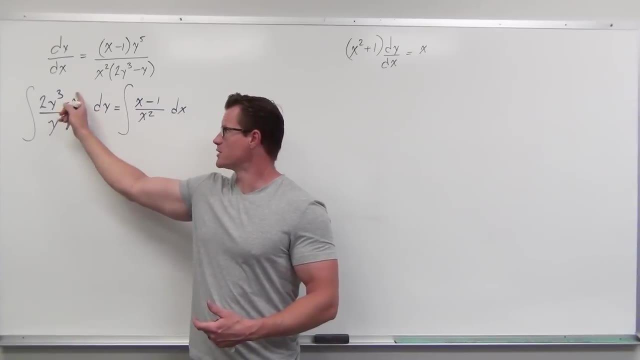 and you have some better recollection and oh, I'm integrating. Okay, how would I approach something like that Substitution? no, because there's too many. there's too many terms on the numerator, not enough on the denominator. 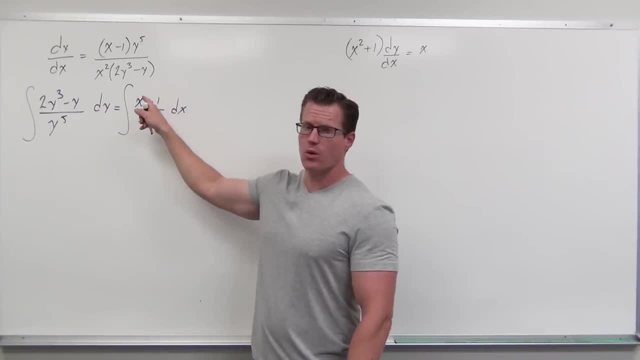 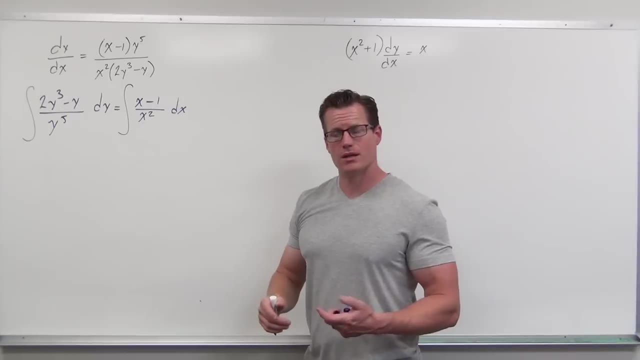 your powers don't match up. Substitution no. again for the same reason: Too many terms on the numerator power doesn't quite match up here. So not a substitution. But we also see that we're only dividing by one term. 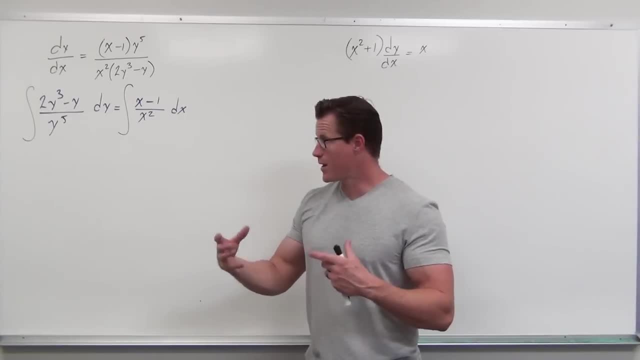 When you're dividing by one term on a fraction, split up that fraction. So we're going to make this 2y cubed over y to the fifth, minus y over y to the fifth. That lets us simplify, and the same thing happens. 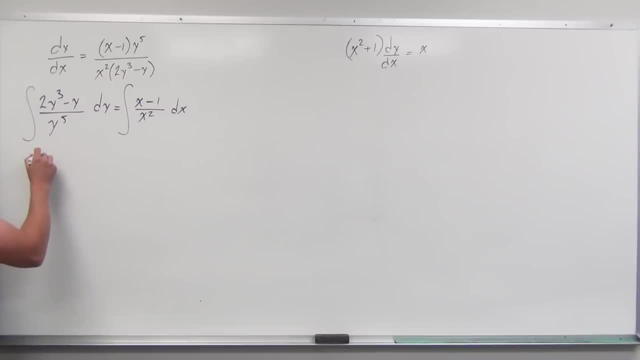 That's what the x is, And we simplify each little fraction and then we can integrate very easily. So, left-hand side, we're going to have an integral of 2y to the negative, 2. Minus y to the negative, fourth power: 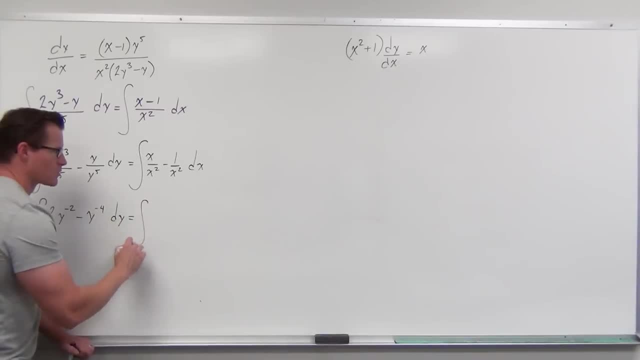 Hope you're sticking with me. On the right-hand side we get an integral of: we have to leave this as 1 over x, because x is negative 1.. Of course, we don't know how to integrate that with some basic technique. 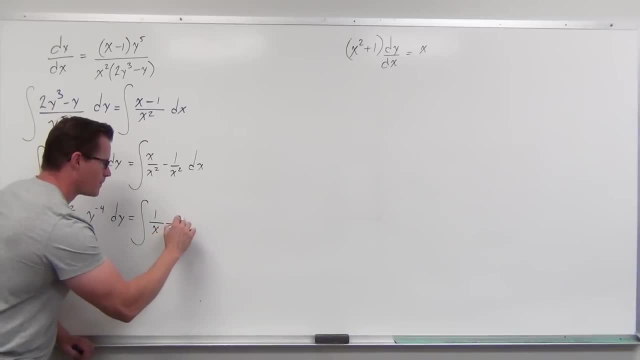 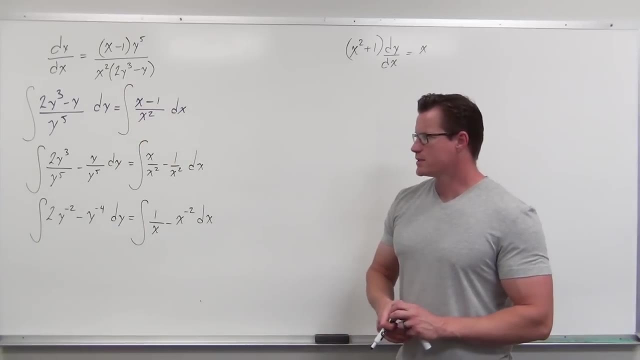 It's going to be a logarithm And right now, if you can integrate that, So 2y to the negative 2. Remember, we add 1 to our exponent, divide by the new exponent, So that's y to the negative. third power: 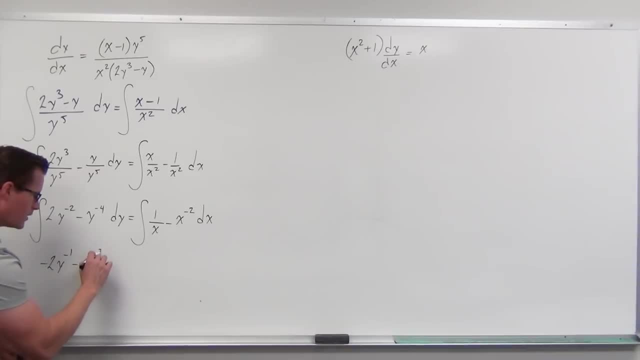 divided by negative 3.. Right-hand side: we've got an ln absolute value of x. Wait, something looks really bad. It's all nastified, So let's fix it First thing. well, we might want to make these. 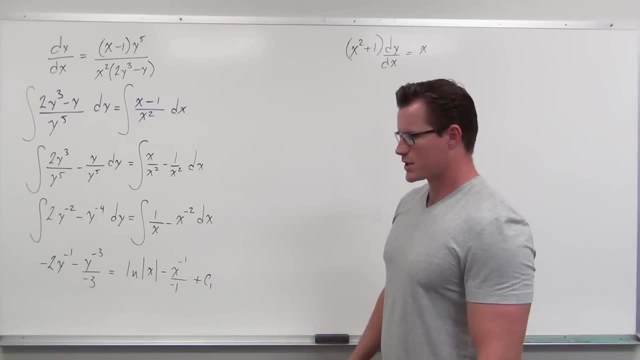 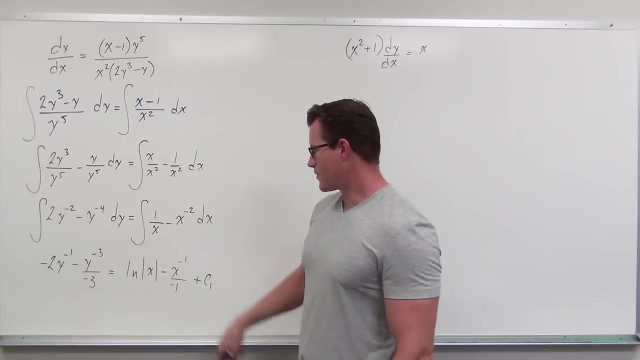 and we're going to have to do this. So what we're going to do is we're going to do this. Make these into fractions and see what our common denominator is going to be. Make this into fractions. see if we can change some signs. 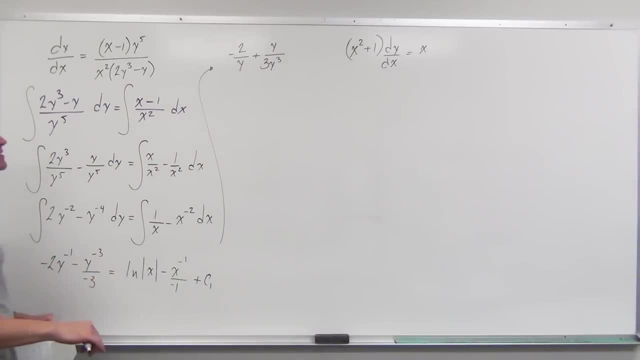 So negative 2 over y, we've got a plus And I set up 1 over y cubed plus 1 over y 3y cubed So that becomes our plus. Leave our 3. Move our y and negative 3 down. 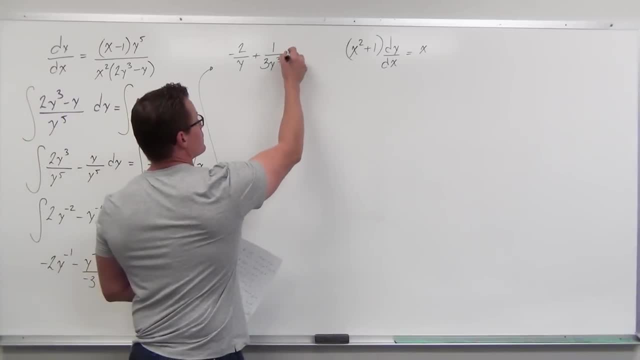 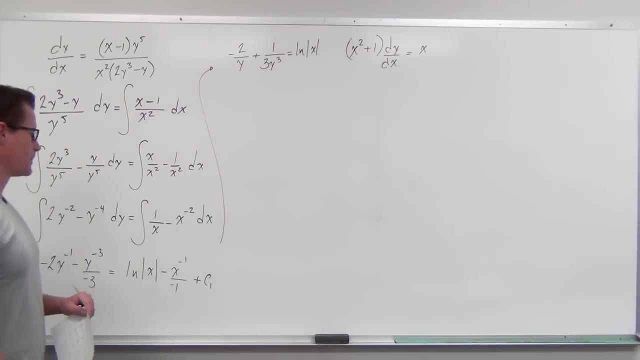 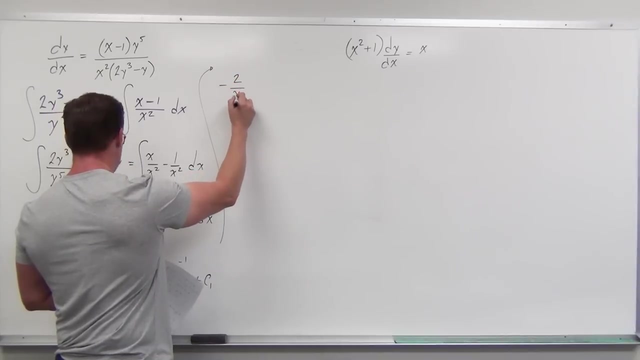 It becomes a positive exponent On the right-hand side. ln absolute value of x. I'm going to get too scratchy, So negative 2 over y, Just redoing it. Plus 1 over 3y, cubed. 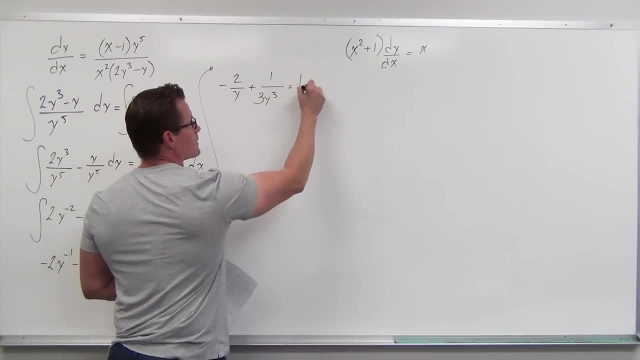 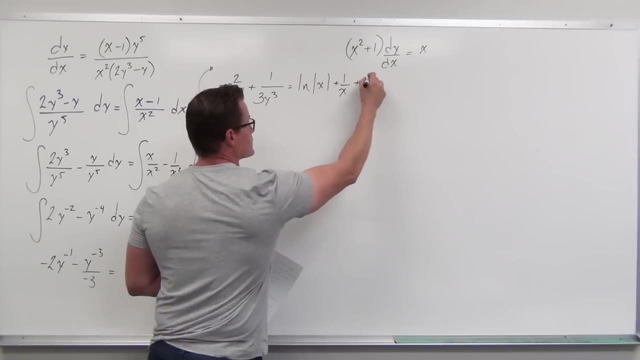 Looks good. Equals ln: absolute value of x. No problem, That's going to be a plus 1 over x plus c. I've got to be honest with you, That's way too nasty to try to solve for y, just to leave it. 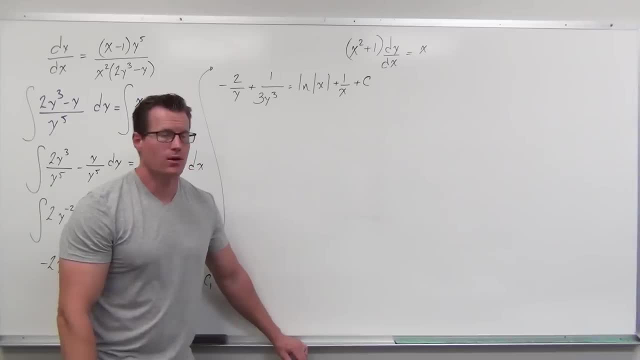 When it's that bad, you go. how am I going to do that? Well, you're not, Because you're going to start getting stuff like common denominator. You'll start getting y's up there, Even if you reciprocate. 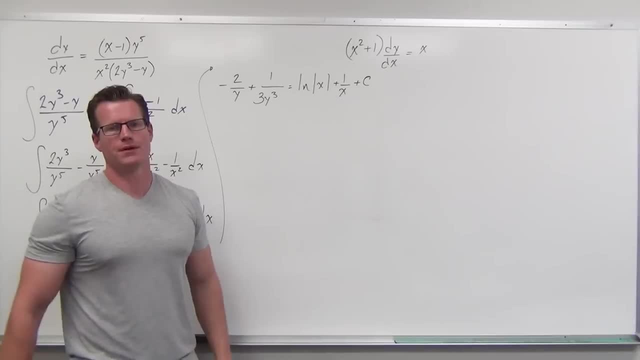 you'd have to distribute, Get everything on one side, Refactor and hope that you can solve for y and take a radical. It's not going to happen, At least not easily, So this is one that you'd be fine. Just leave it like that. 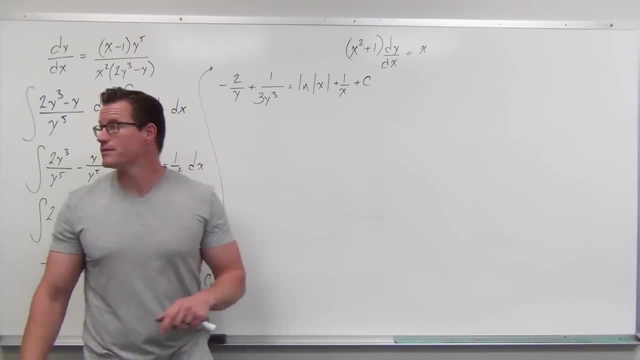 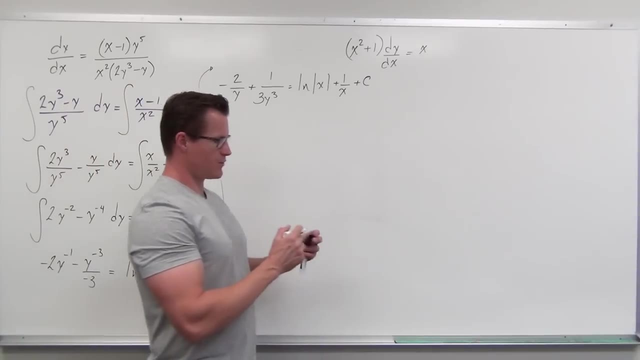 I know it doesn't look good, But that is a general solution to that differential equation. Let's try that next one. So next one says: if we have x squared plus 1 on the left-hand side, that's on the wrong side. 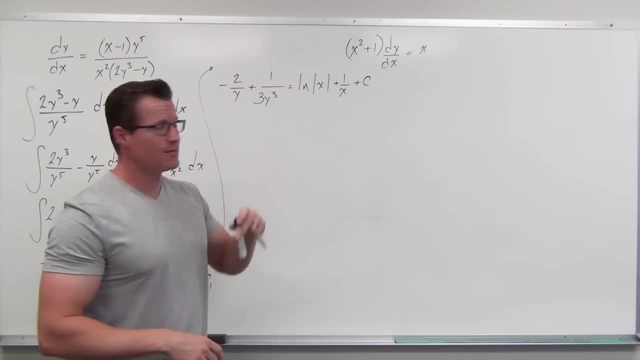 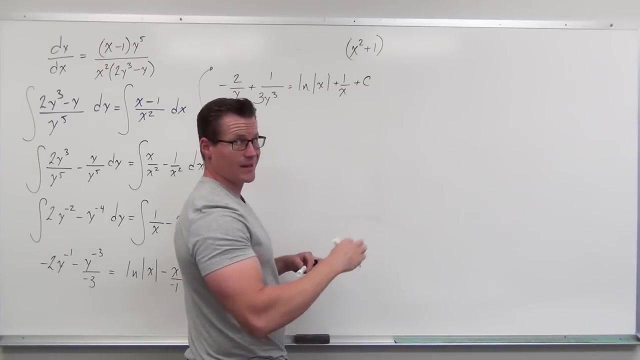 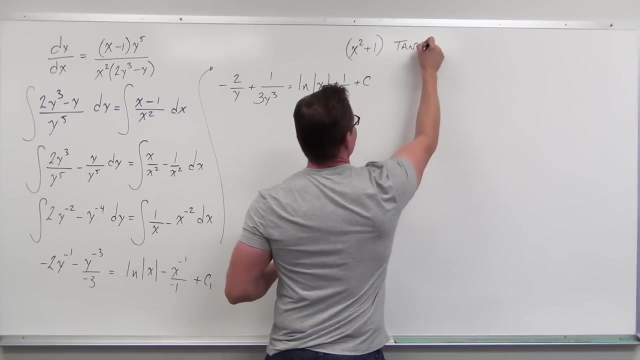 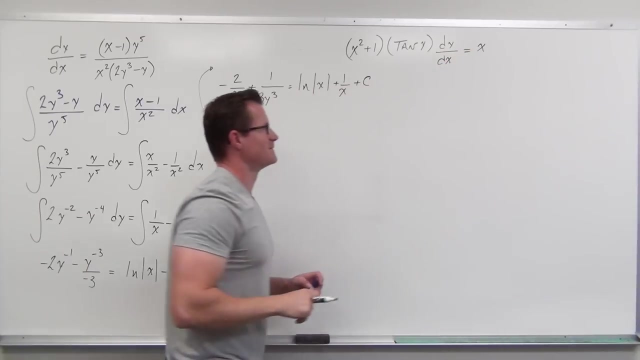 Let's move it. We already have an x over here. Let's leave that there. Oh, you know what? I forgot to write that. Sorry guys, I forgot something. It's kind of important. You tried to do that on your own. 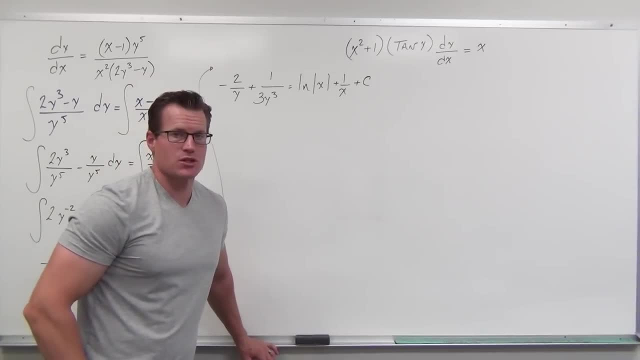 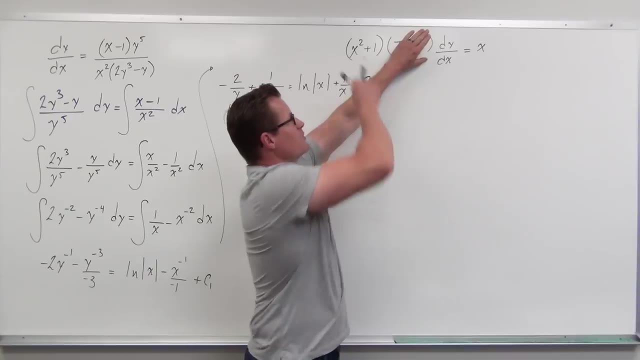 and you weren't able to, My bad. Actually, you probably should have been able to, because without that tan y, you just do the integral of dy and it's just y. So without that, you move that and that's going to be. 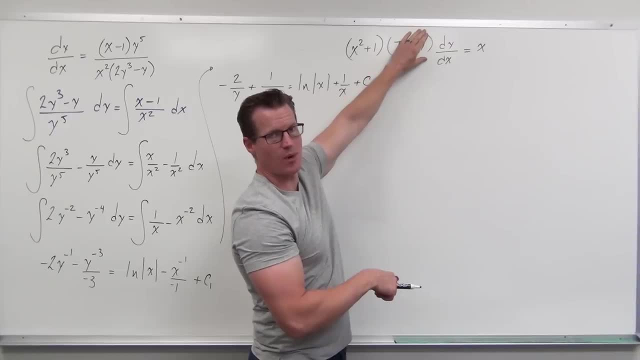 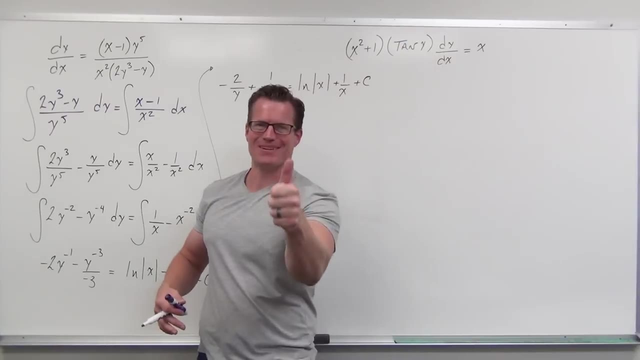 looks like a? u sub, And then take an integral of dy, you get y On the right-hand side. you get something really easy. So sorry if you did that on your own, But good job, Good job, You got it. 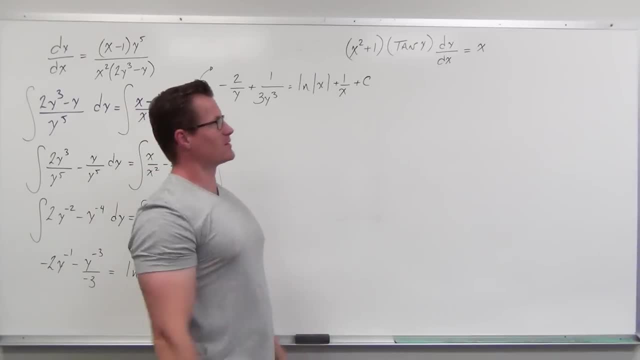 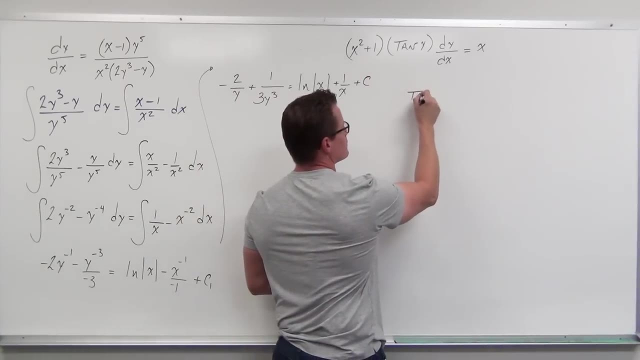 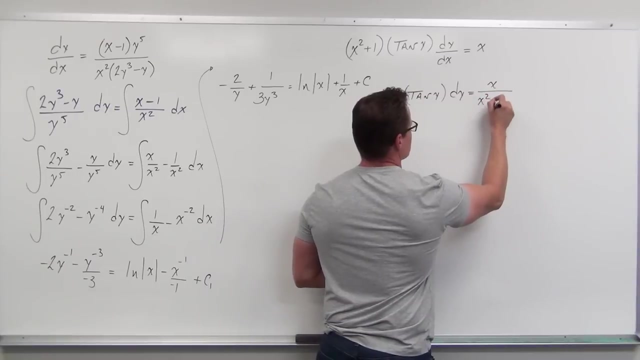 Now we have something a little bit different, Obviously. So let's leave the y's where they are, move our x's where they need to be by dividing by x squared plus 1 and moving our dx. Now we're ready to integrate both sides. 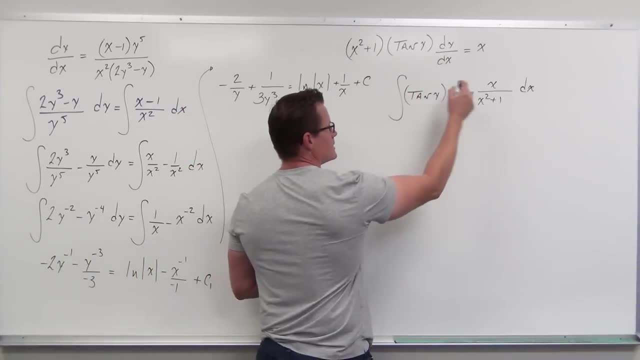 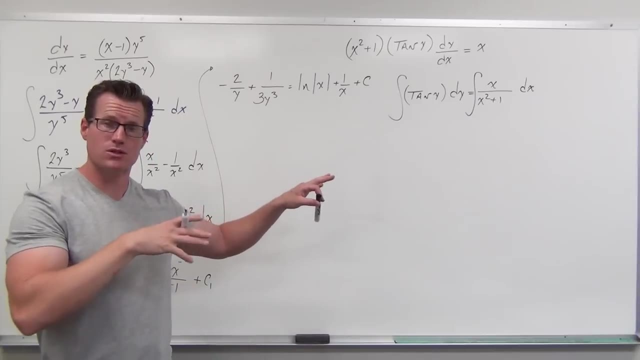 So let's take an integral of tan y, dy and an integral of x over x squared, plus 1 dx On the right-hand side. as I was saying, that's a perfect case for a substitution. So let's do that. 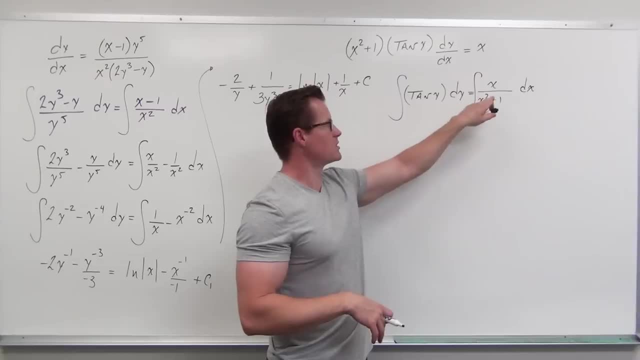 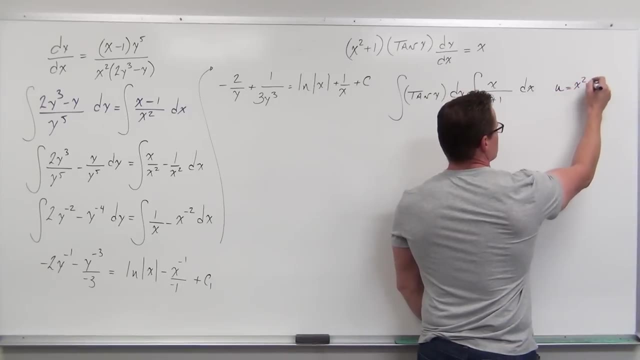 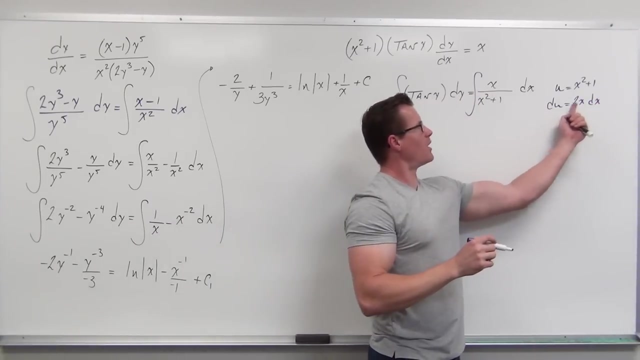 So we let u equal our denominator. The derivative is 2x, Our variables match up. We have a constant which we don't care super much about. So when we're doing this we're looking for: remember we want this piece. 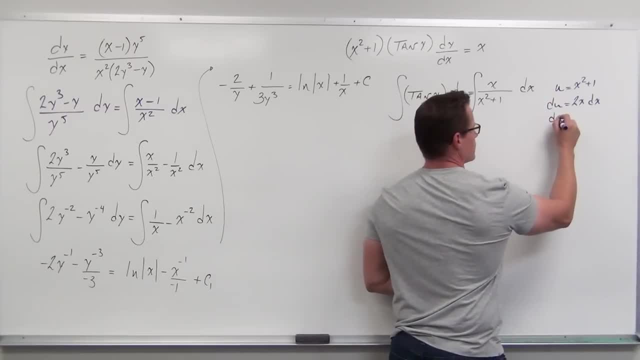 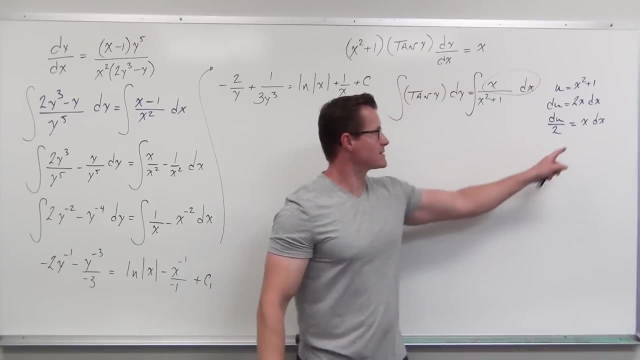 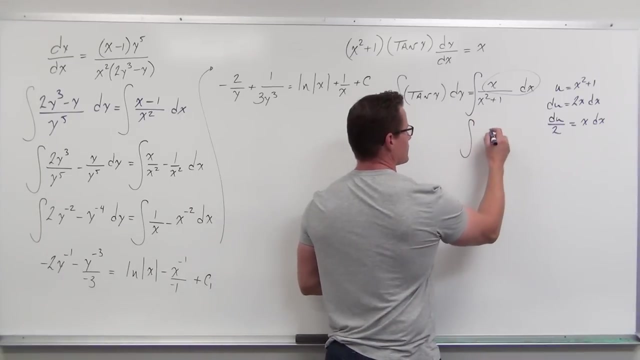 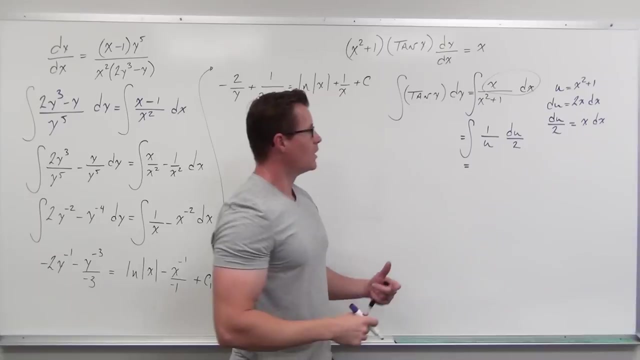 to match this side, You got to divide by 2.. Now we can replace that x dx with du over 2.. We know we're going to replace that with just u. That's what we call for our substitution. So we get our 1 half. 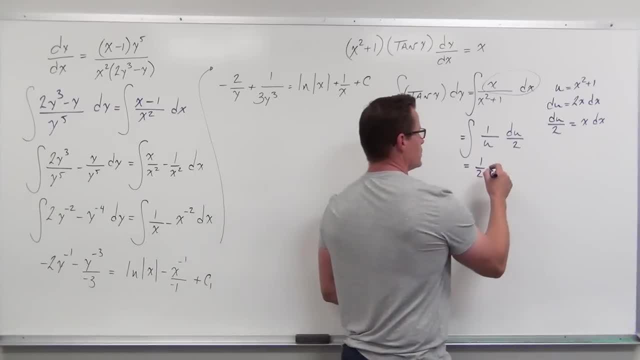 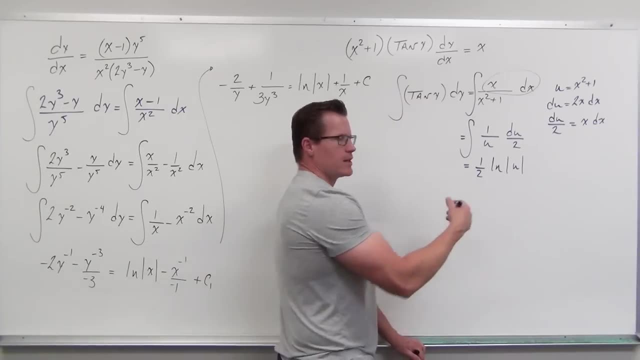 That's our du- over 2.. We're going to get an ln absolute value of u Now that u that u is x squared plus 1.. So we would normally do ln of absolute value whatever our u was, but because x squared plus 1, 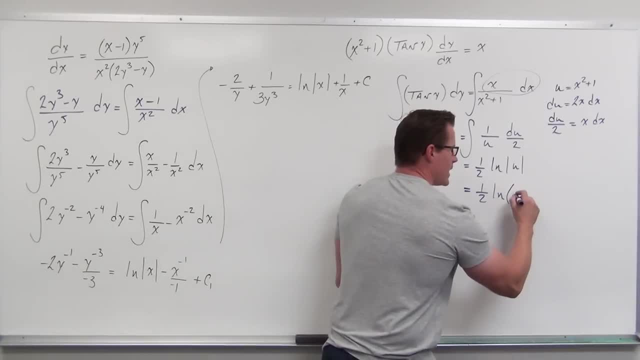 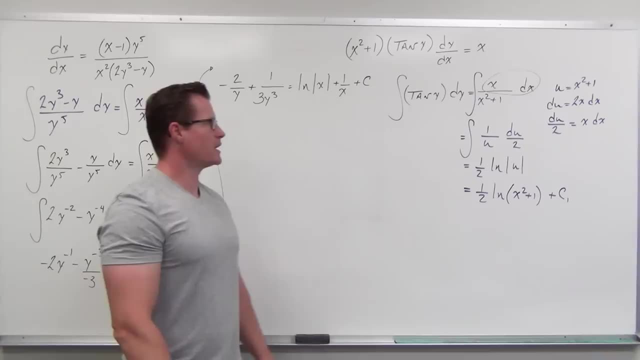 can't ever be negative. with real numbers, we don't need the absolute value anymore. We just do x squared plus 1, and then we have a c On the left-hand side. so the integral of tangent y. this is one that you're going. 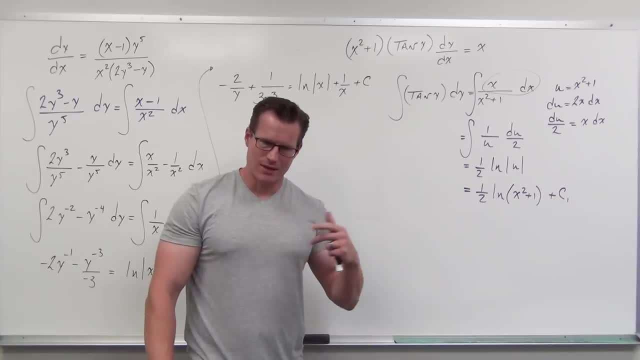 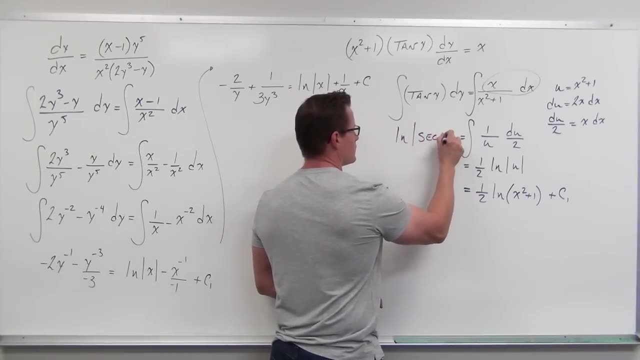 to want to use your table for. So the integral of tangent y gives you ln absolute value of secant y, And now we work our way through, just like we normally would. So let's write this down here: ln absolute value, secant y. 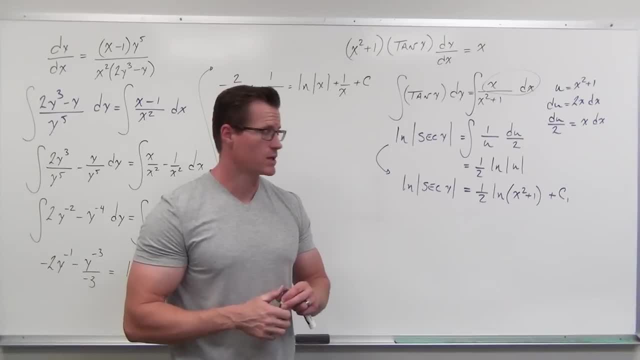 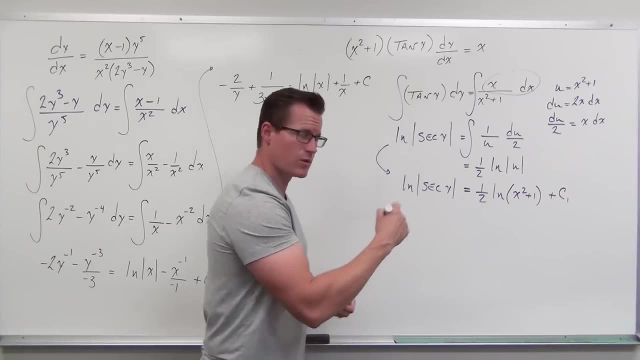 and then try to do the same techniques we've done a couple more times. Let's move this as a square root. Let's get rid of that coefficient. That way we can do an exponent on both sides. We're going to do that first. 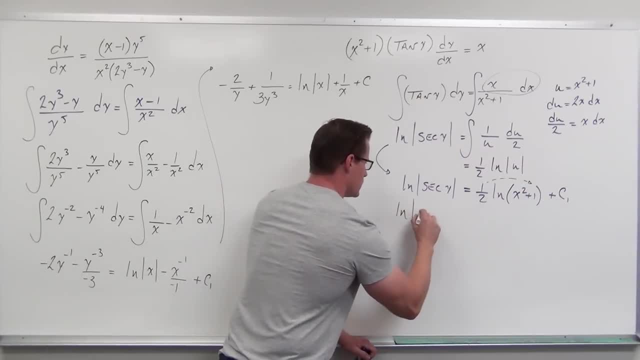 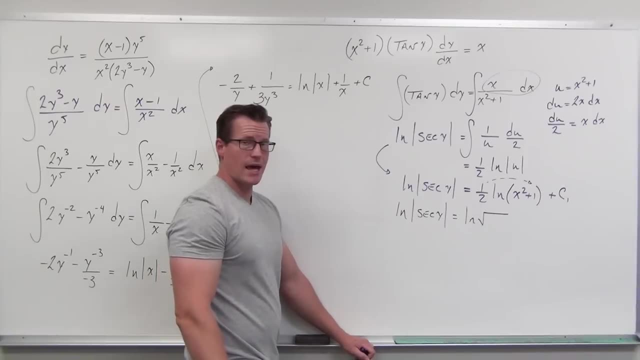 So we're kind of putting everything together right now: x squared plus 1 to the 1 half power is a square root. Now I've got an ln equal to an ln plus a c1.. Do you remember what happens when we do the e to both sides? 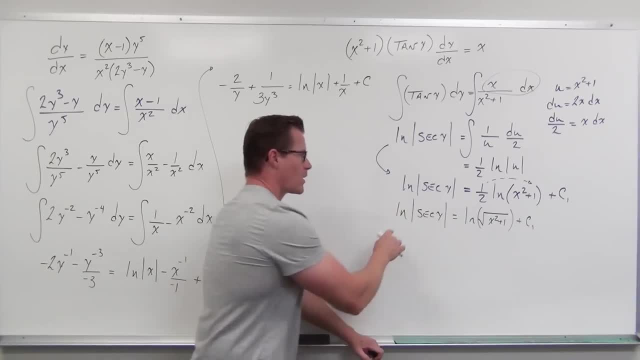 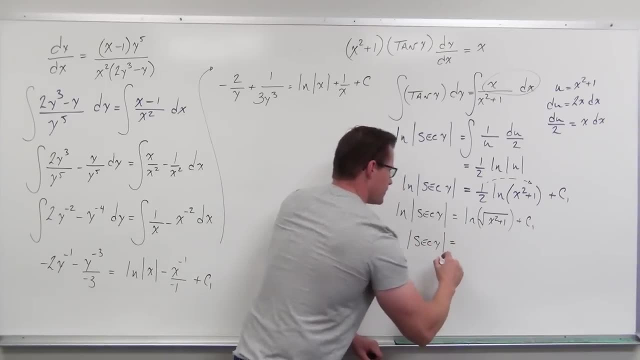 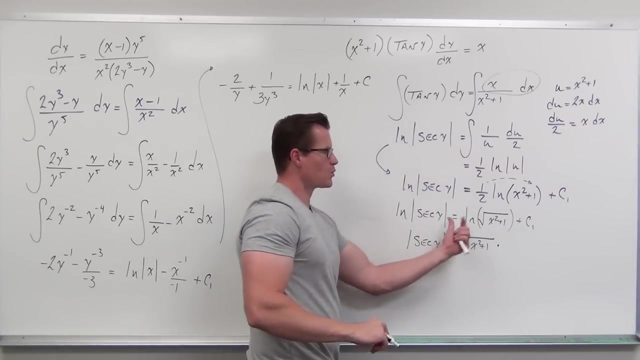 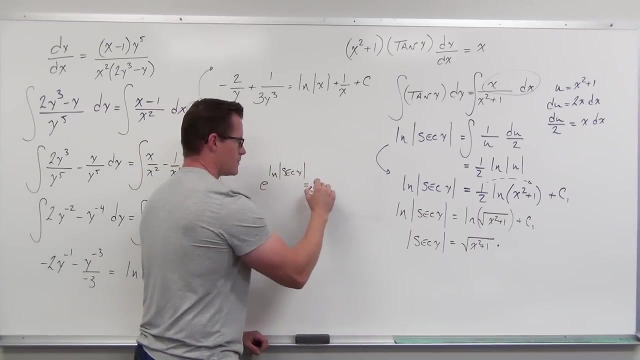 So we take both sides as an exponential on e, Our ln's are going to drop, But because what I'm really doing is this: that's going to go away, That's going to go away, but that right there, that plus c1, c sub 1,. 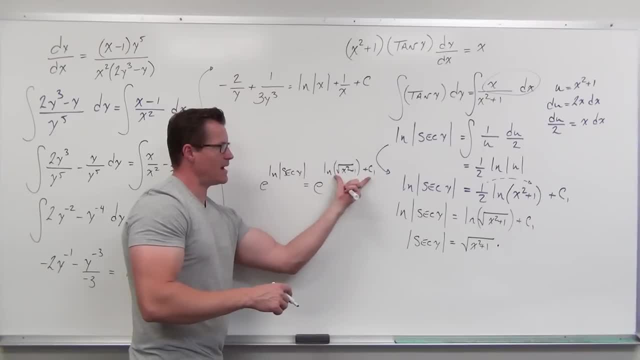 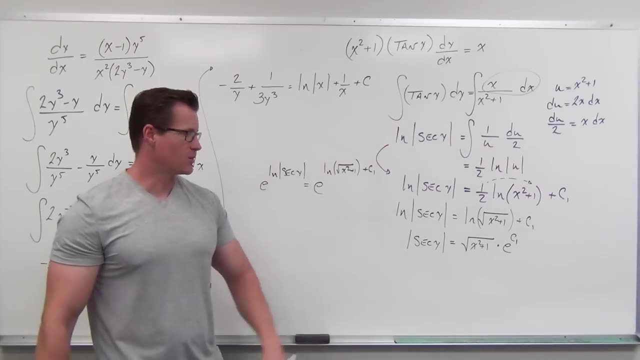 that's e to the c sub 1 being multiplied by this. Remember that when we have exponents being added, that's a multiplication common basis. So I'm still going to have an e to the c sub 1.. Now we know absolute value. 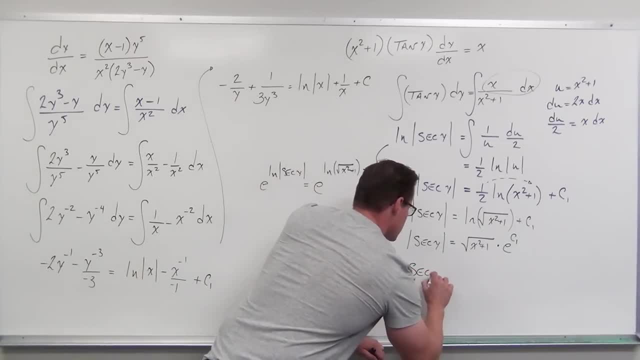 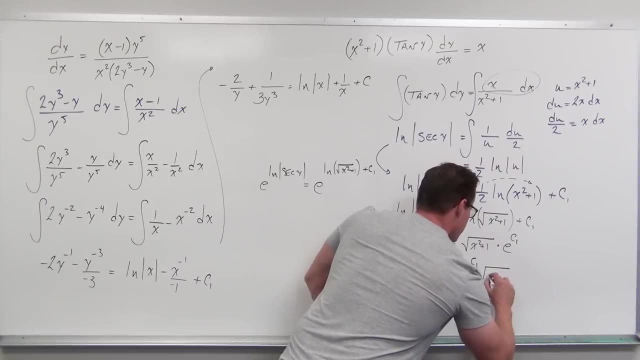 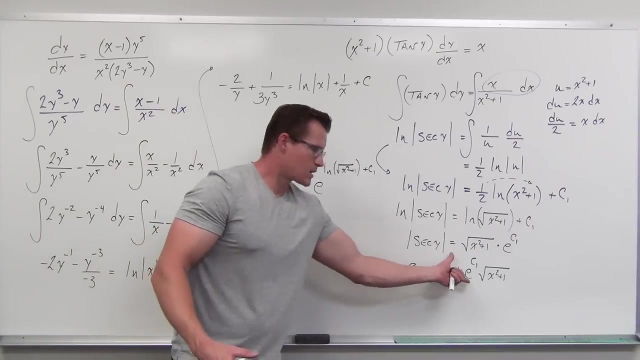 Well, we can take this as if we need to plus or minus e to the c sub 1 times the square root of x squared plus 1.. Now, that's a constant. We've done that many times, So that's going to be. 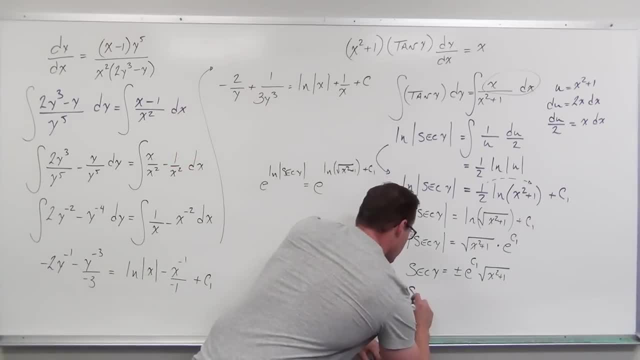 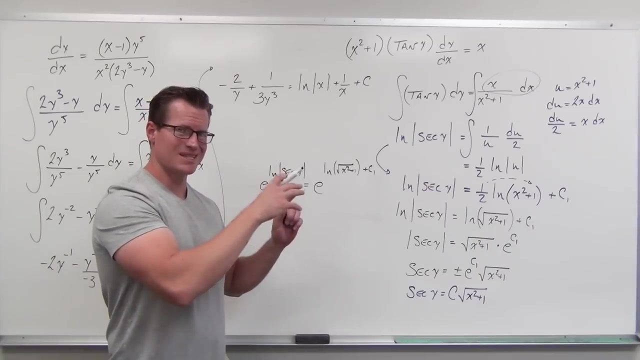 just a big C, the arbitrary constant. So secant y equals some constant square root, x squared plus 1.. And last step, Man, our last step. We're almost done. If secant y equals something, then y equals secant inverse. 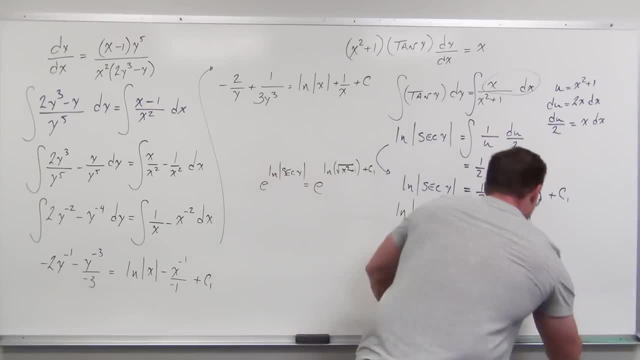 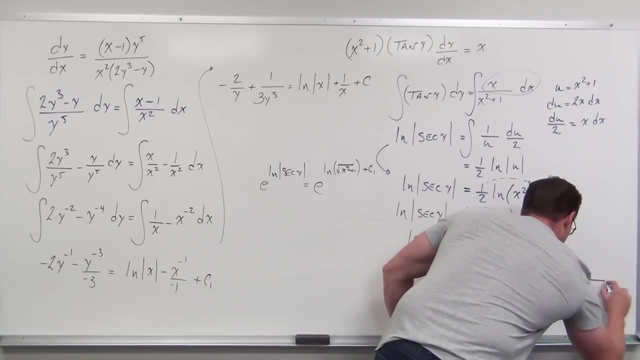 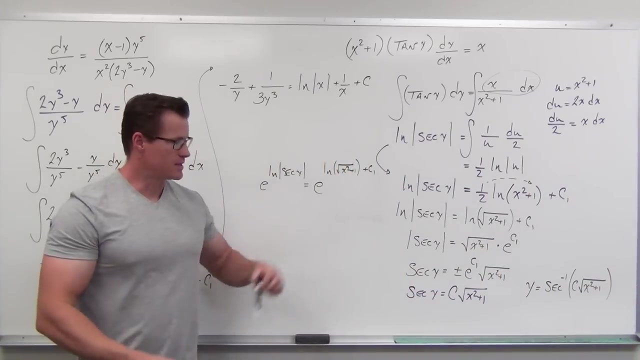 of that something And we're done. That's as good as we can get. That's our general solution for that differential equation. I'm really hoping that this is making sense to you, that you, at this point, are like. 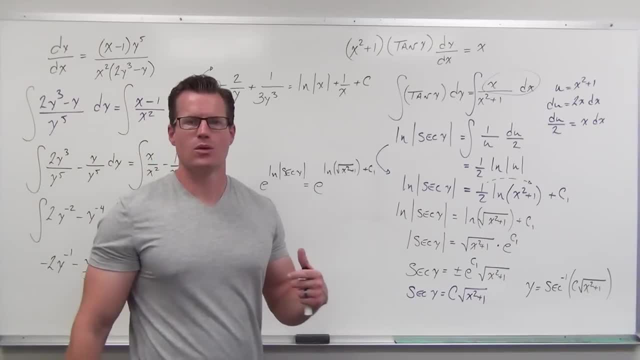 yeah, I get how to separate my variables. I understand that my y's and dy are here, My x and dx are here. We're going to do an integral, do lots of different techniques- There's lots out there- And then do our best to solve. 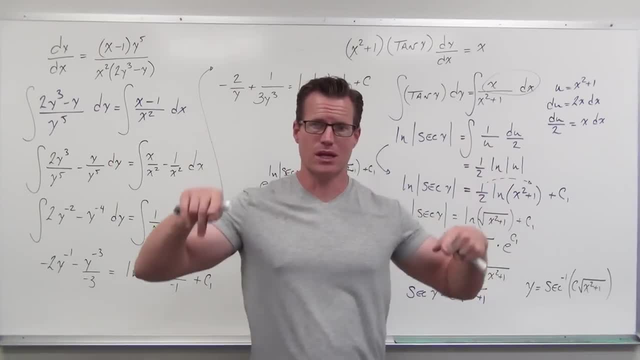 for y, When we get really nasty stuff, we're probably just going to leave it. If it's reasonable, then we're going to leave it. We're going to leave it for the next step, So we're going to leave it. 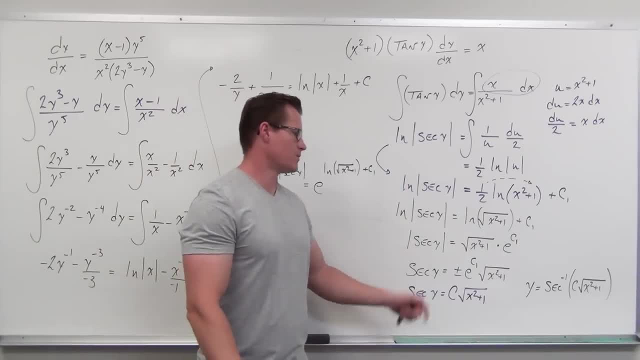 for the next step. We're going to leave it for the next step. If it's reasonable, then we solve for y. We have two more to do. They're not that bad. We're actually going to get a couple easier ones. 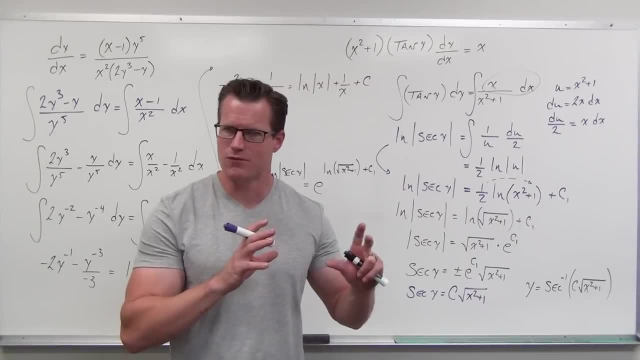 It's just one special case I need to show you at the very end And kind of a you need to pay attention to this when you get it for the next one. So we're going to do those two and then call it good. 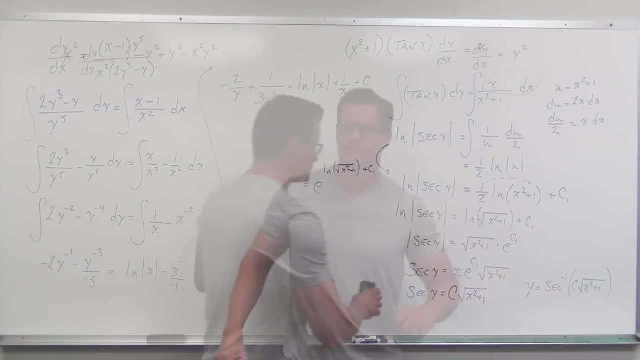 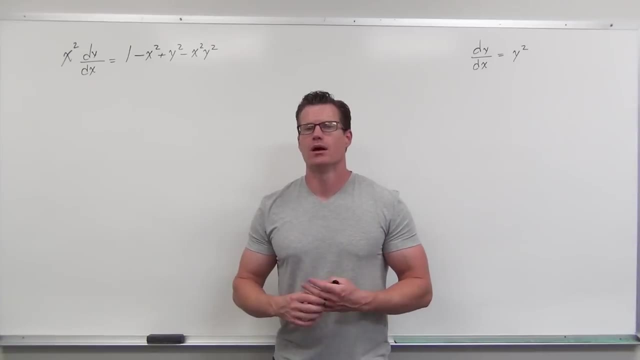 Two more. One's got some fancy-pants math on it, And one of them is just something that you need to be aware of. that can happen when you're solving differential equations, So we're going to do those two and then call it good. 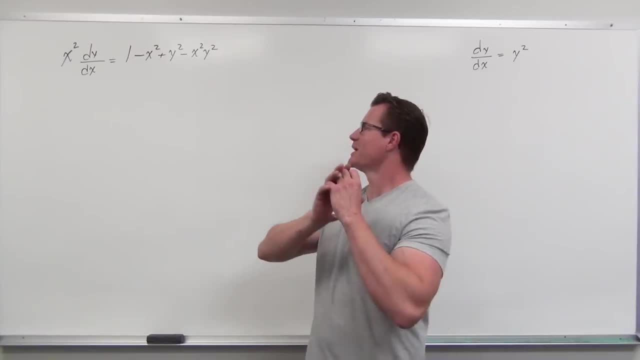 Two more. First, this one: When things don't look anything like what you're trying to make them. Sometimes they're not, But sometimes it requires you to think outside the box. So in our case, right here, 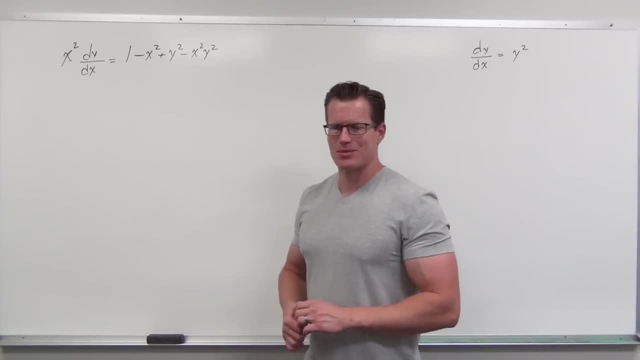 that doesn't come on. They can't possibly be separable. No, Well, what are we looking for? Stuff being multiplied. How do you get stuff that's multiplied out of stuff that's added and subtracted? Well, you want factors. 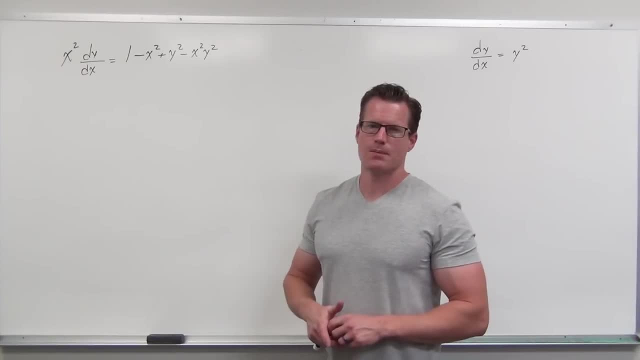 Oh my gosh, You've got to factor. Sometimes, rarely, these things are not factorable. So if you have four terms on the right-hand side, three terms is a diamond problem. four terms may be factored by grouping. 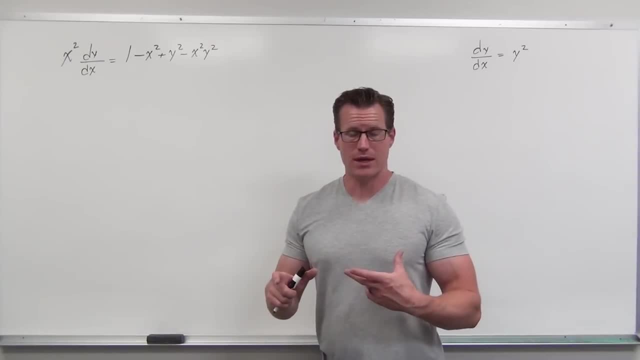 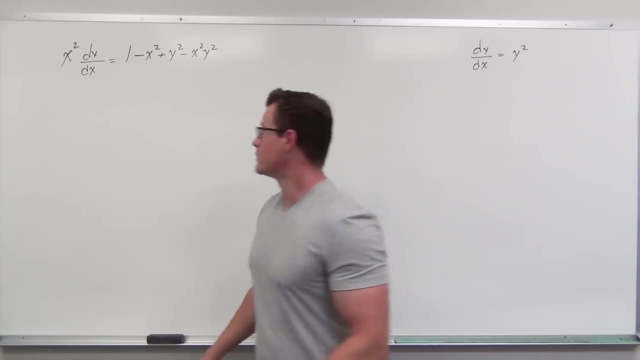 If you factor by grouping on that one, we can actually make this into things that are being multiplied. That creates factors. That creates this function equals stuff that's a product And that means that we can separate our variables. So it doesn't happen. 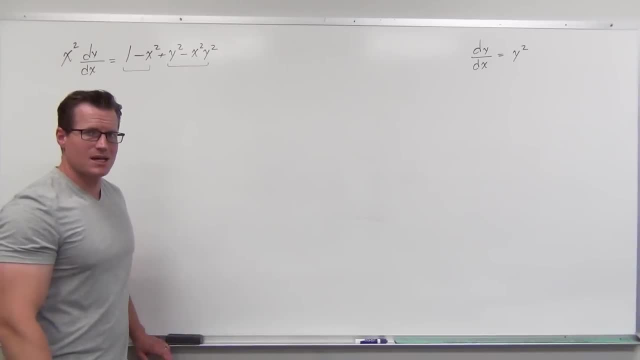 all the time, but sometimes you can group it. So the first two terms, one minus x squared. we're trying to factor a GCF. I'm talking about factoring a GCF. There's nothing besides one. So we can write. 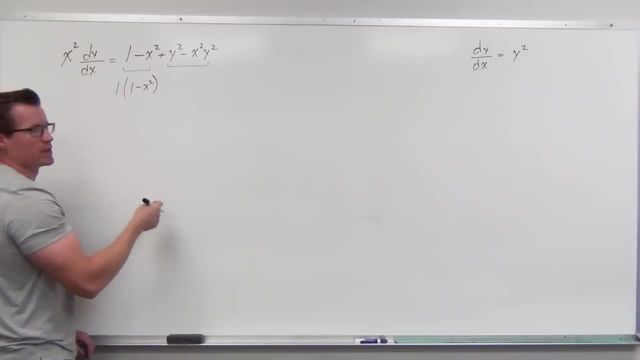 one One times one minus x squared gives you that back. Factoring by grouping always writes our middle sign between those pairs of terms, And then it factors the GCF out of the last two, which is y squared. This is what you're looking for. 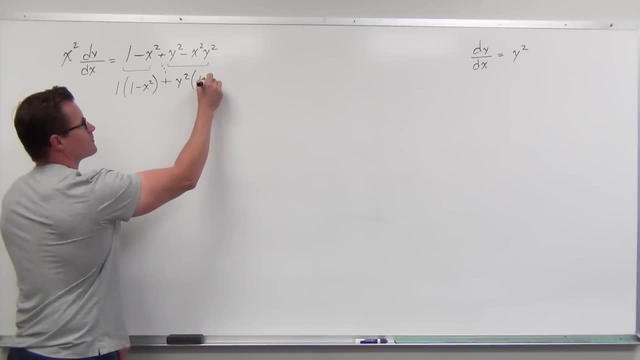 with factoring by grouping is two big fat terms that are equal to x squared. So that's two big fat terms that have a GCF that you can factor out again. So we factor out our one minus x squared. That leaves us with 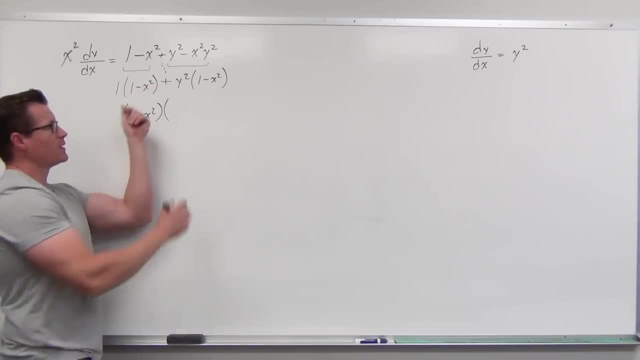 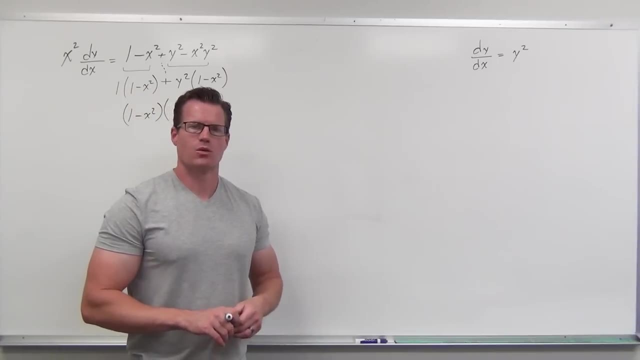 and the reason why we wrote the one. so when you remove this by division, you still have one That doesn't go away. Whenever you divide something, you can't ever get zero unless you start with zero. So when we're factoring, 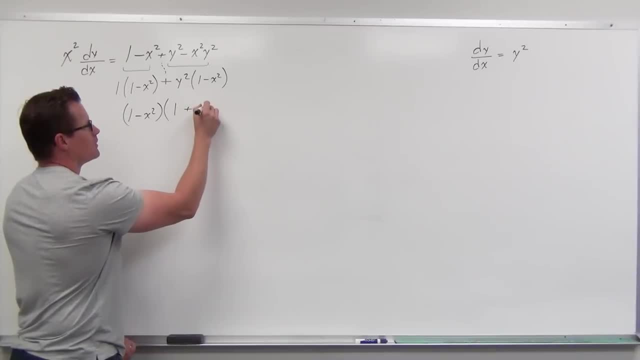 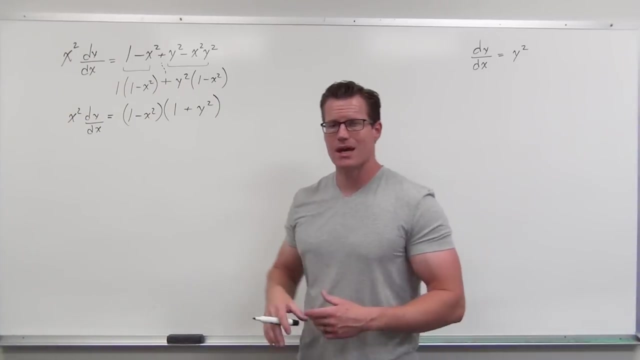 your terms never disappear. The smallest they can become is one. So y squared is one plus y squared, and that's something that we can separate the variables on. We can move our y's on one side, x on the other side, with a dx. 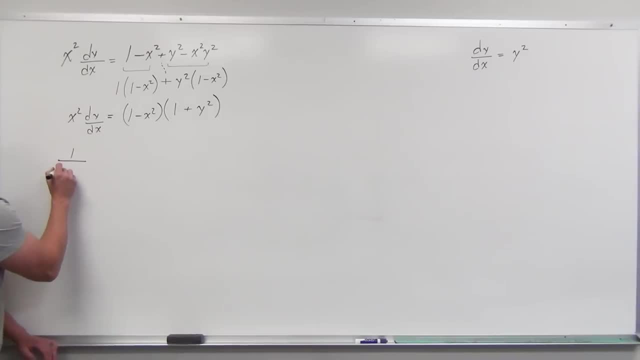 and integrate. Try it. I'm going to go a little quickly on this, because we've had a lot of experience with a lot of these differential equations and we're about ready to integrate. Use a table Whenever you get one over one plus y squared. 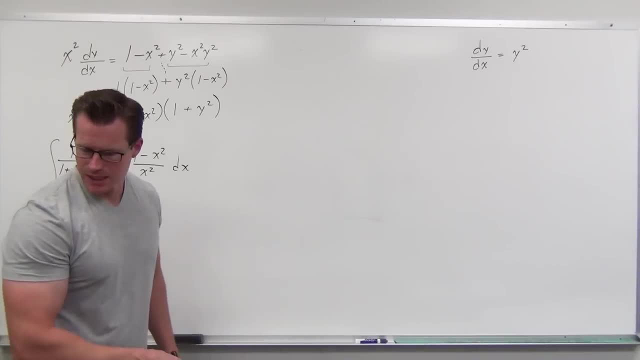 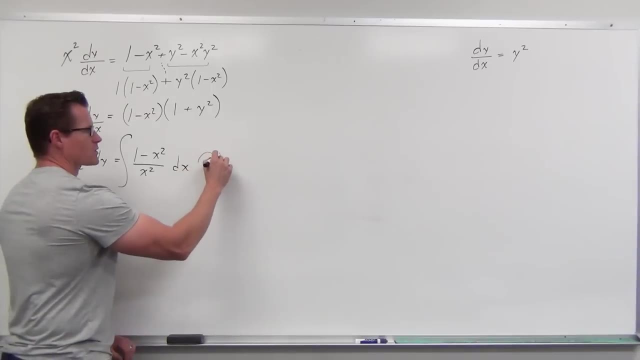 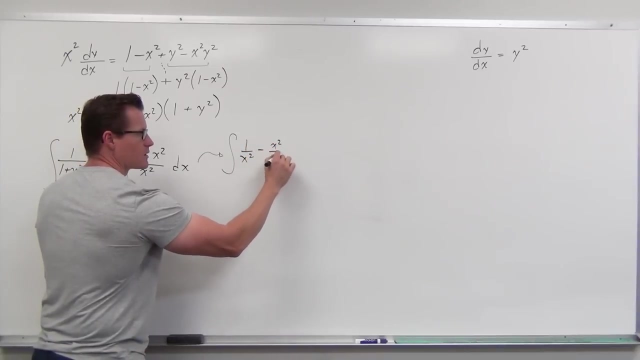 you can do trig sub if you really want to, but if at all possible, use a table. if you've memorized that This is a tan inverse On the right hand side, we'll certainly split this up as one over x squared minus. 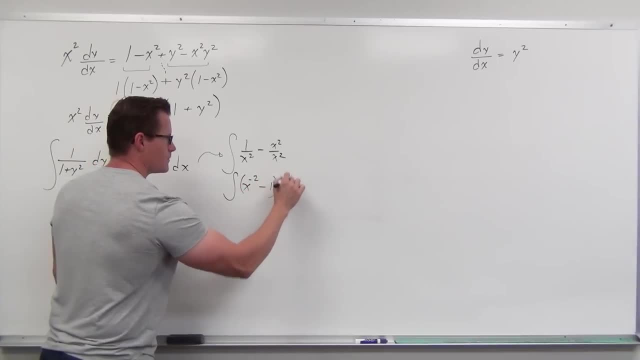 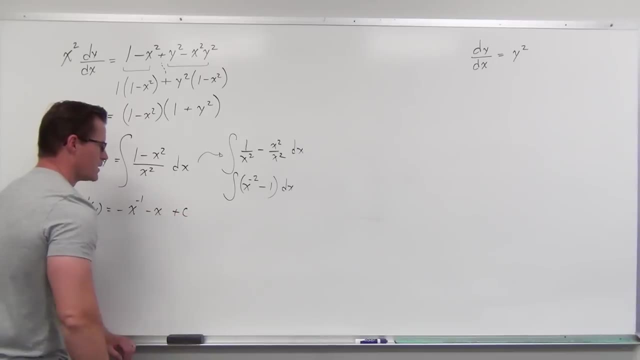 x squared over x squared, Which gives us negative x to the negative one, minus x, plus c one. We're going to leave it at c. We're not going to have to change it on this one. So if we clean it up just a bit, 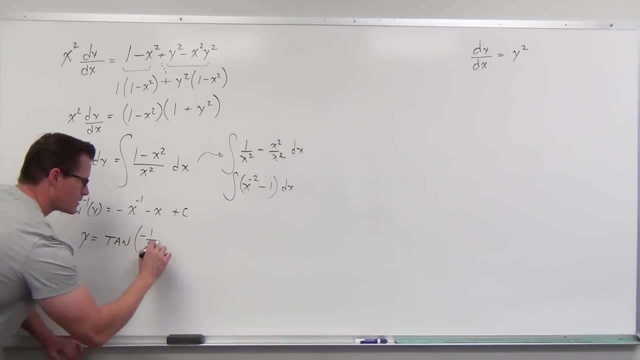 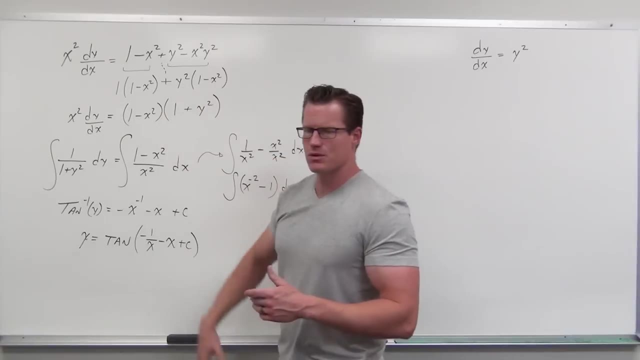 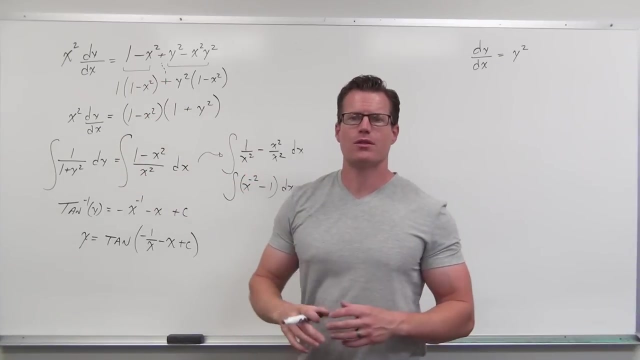 y would equal if tan inverse of y equals y. That's a really nice way to solve that. But the point of this problem wasn't this: We've done those techniques before It was. sometimes you can get stuff to fit, even when it looks like it. 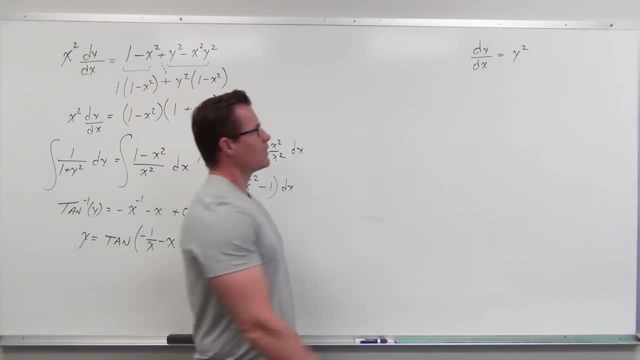 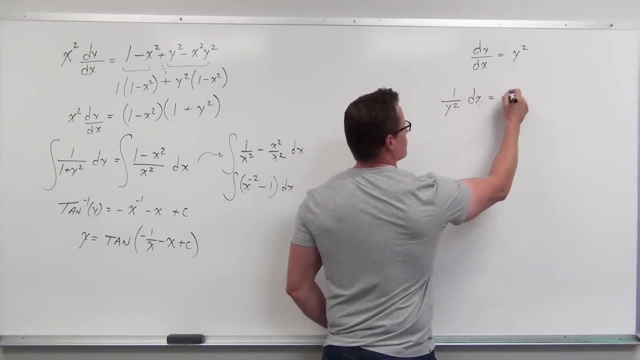 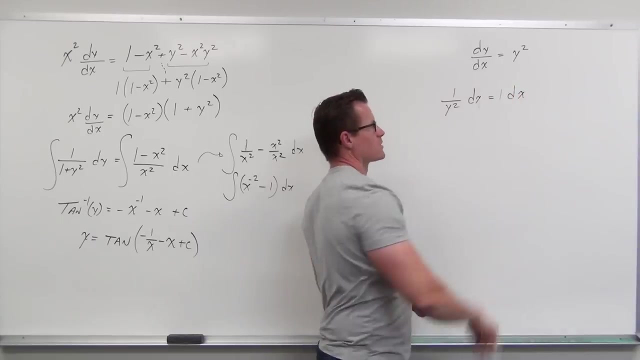 doesn't Think about factoring things that make a product for you. That's about all I need you to know on that one. So if we divide both sides, we get a one. y squared divided by y squared is one We get. 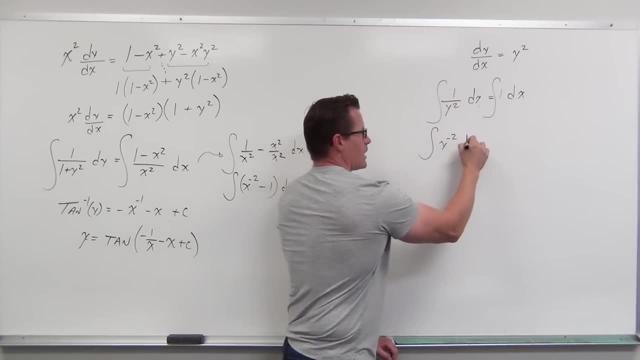 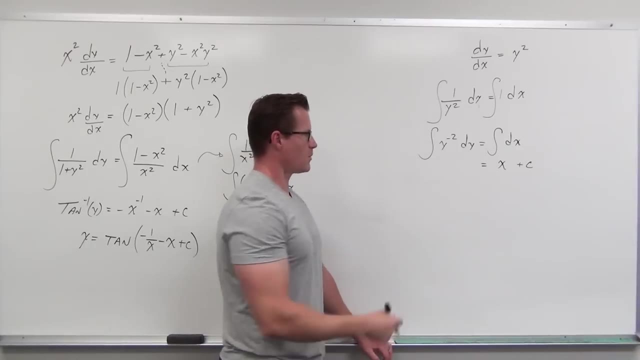 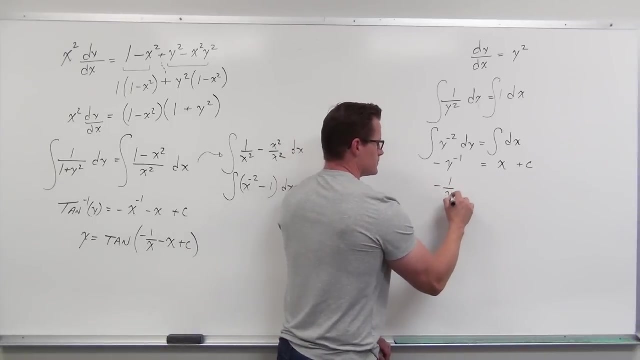 one over y squared dy. If we integrate we get the integral of y to the negative. two dy equals integral dx, which is integral of one, dx, which is one minus one. So we can get c-1 over y squared plus z squared. 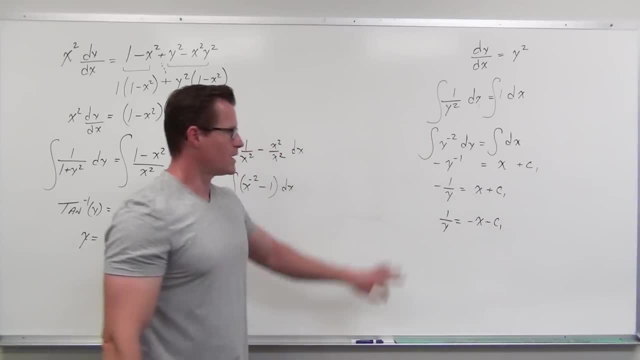 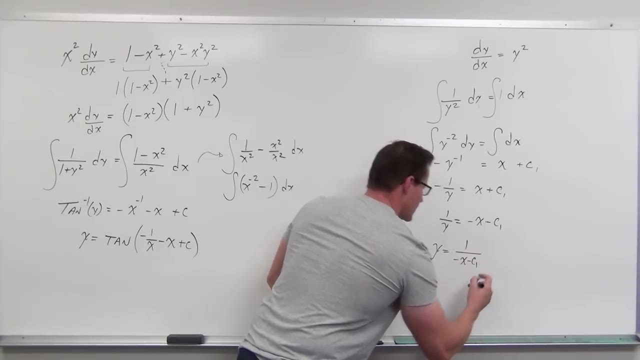 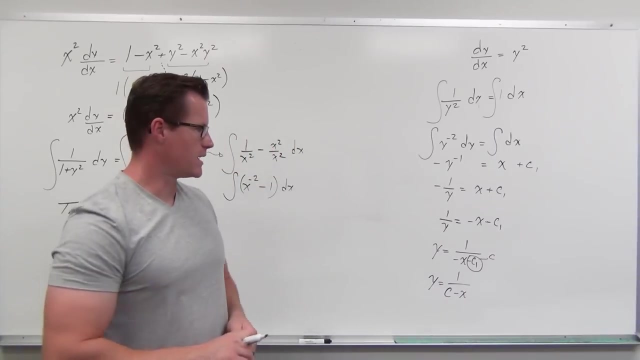 times x squared plus y, squared minus y, squared times y squared plus y, squared times 2 minus 1 minus x, squared times x squared times x squared minus, and get 1 over c, arbitrary constant minus x. That is a general solution. That is the general solution to that differential equation. 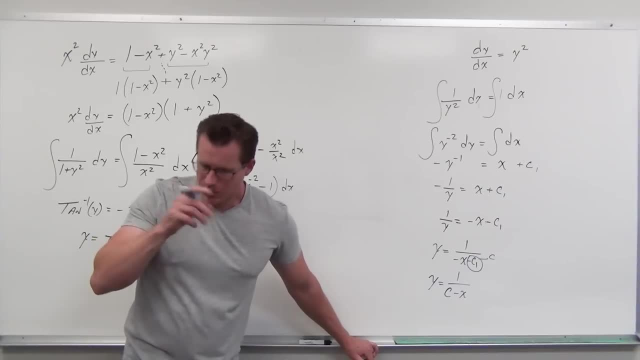 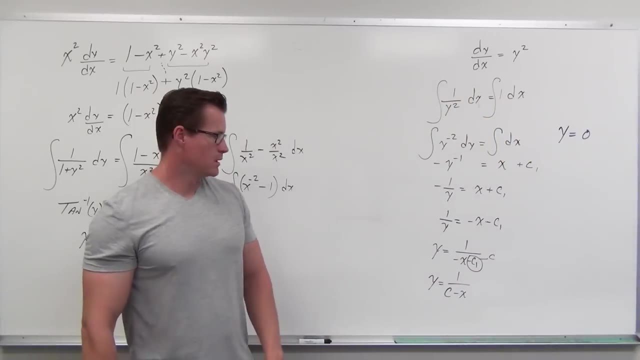 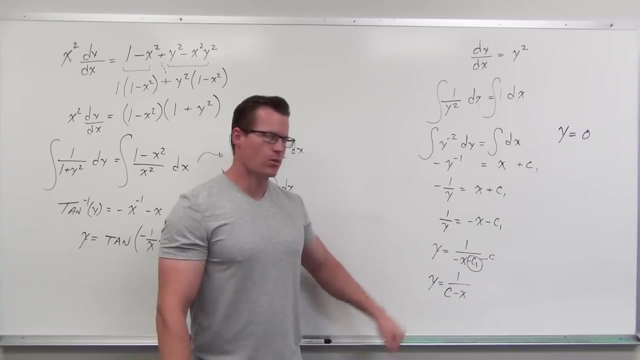 But I want you to consider something else. I want you to consider this: What about y equals 0? You can't get y equals 0 from here. It's impossible, because your numerator is 1.. There's no way that you're going to plug in any number and get y equals 0.. 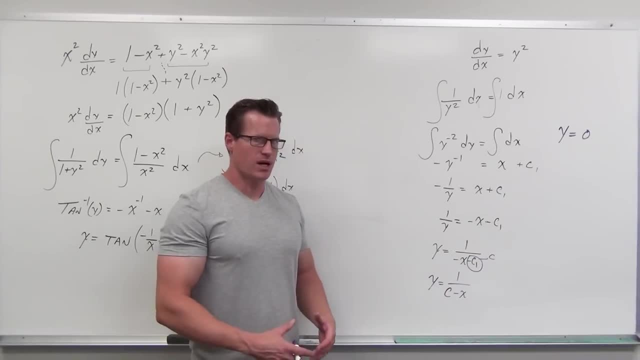 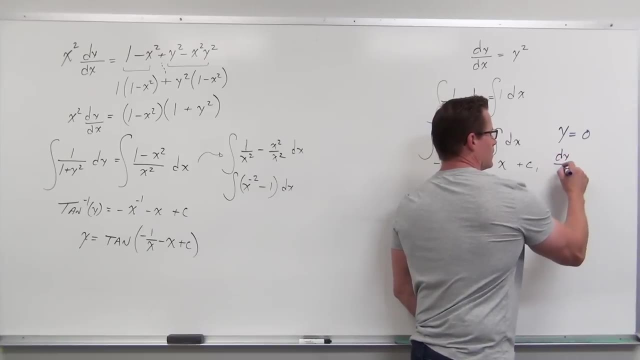 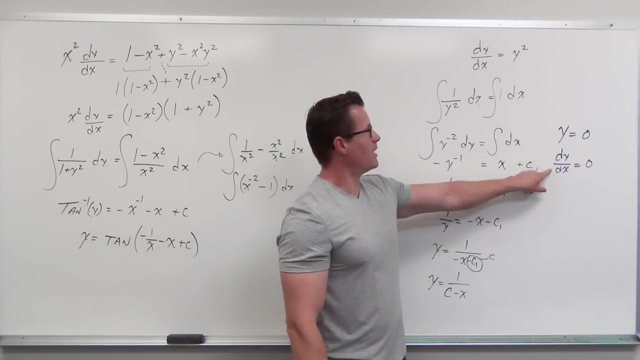 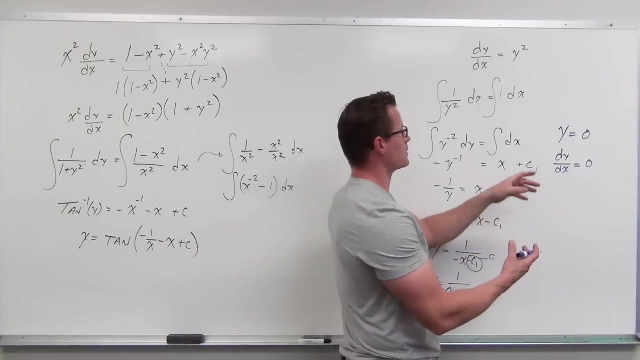 I'll verify that. You can't get it, So it's impossible. But consider this: If you took y equals 0, the derivative of y would still be 0. So we'd say, hey, does that satisfy this? Remember, the very first thing we did was plug in stuff to make sure it worked in our differential equation. 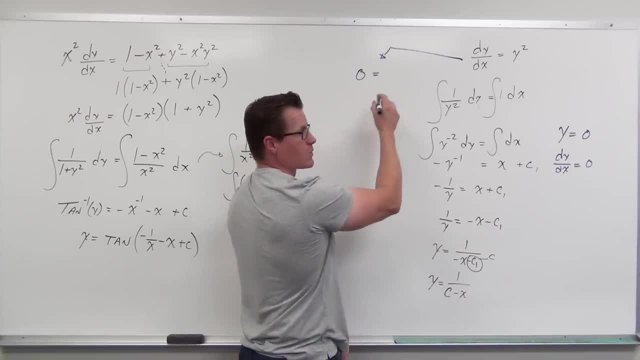 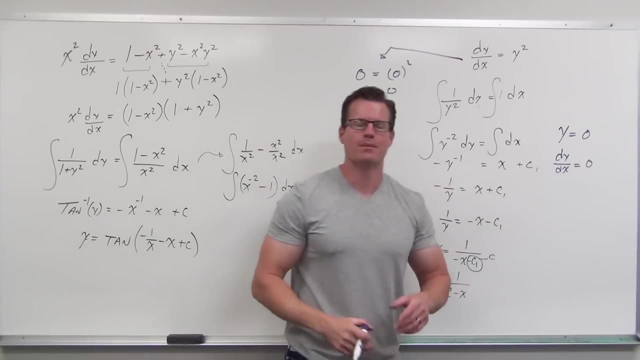 We'd say dy dx is 0.. y squared, It would be 0 squared because y is 0.. Yes, 0 equals 0.. Yes, that's a solution. There are sometimes solutions that do not appear in your general solution.